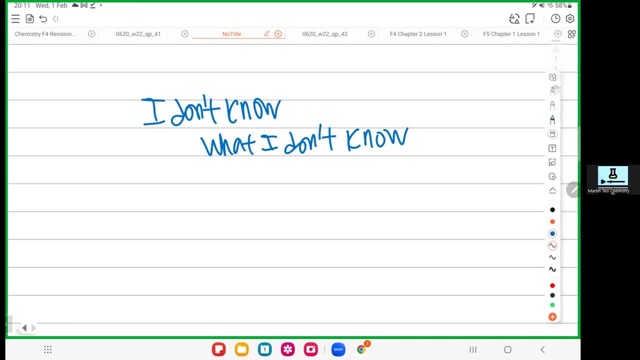 So one of the simplest way for you to identify your own weakness is that you must do good quality question. You must always do some good quality question. So what do we mean by good quality question? Okay, I want you all started from Form 5.. Try to do more on the trial exam paper. Do the question from trial exam paper or we call. 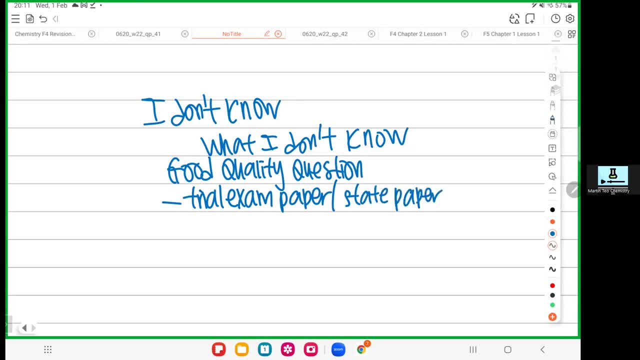 it state paper And also you want to do some past year question, PYQ, past year question. These are good quality question. Not advisable for you all to do the question from any reference book, okay, Because sometimes the question for reference book might be too easy or they might be too hard. all right, Some students. 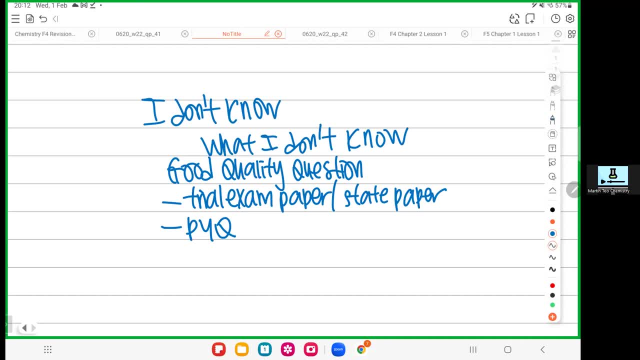 they can do all the questions from reference book, but they cannot do a single question in SPF. There are quite a number of students like that, okay, So if you really want to do the question, do some good quality question like what we will do today, like this, okay, Like the question from: 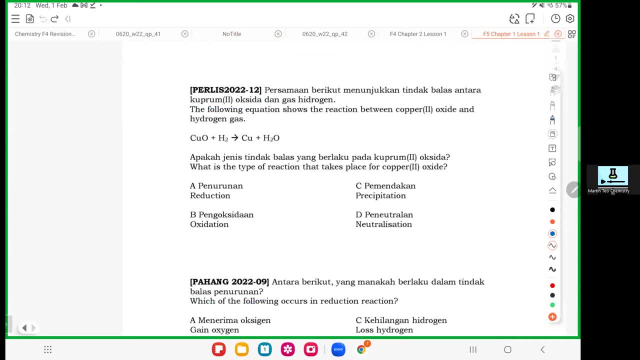 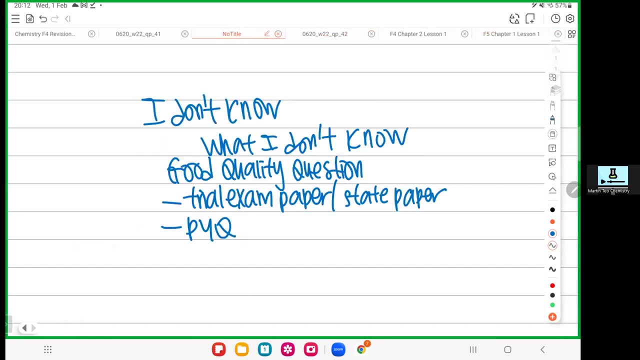 Perlis, the question from Pahang, all these state paper. So the quality is there, okay, So this is something very important, So don't keep on reading already when you come to your Form 5. You have to start doing question When you do the. 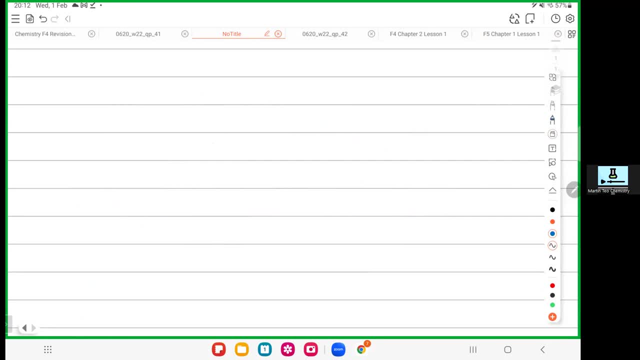 question, then only you know what is your weakness, Then only you can find some help. Like for example: if you keep on doing the question you found that you always start at sort okay, Then which means your sort is not good. Maybe you can ask your school teacher, you can ask me, you can ask your. 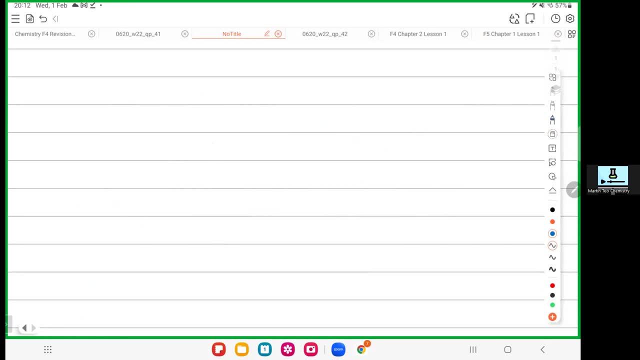 friend who know. At least you know what is your problem. okay, When you keep on doing question, you always start at more. You don't know how to do the more calculation, for example. Then you find a way out. Maybe you go to watch my YouTube video. 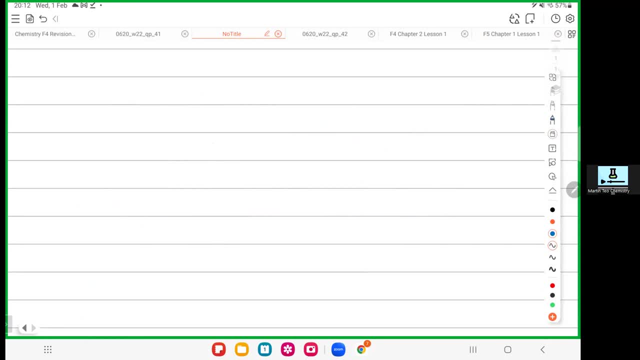 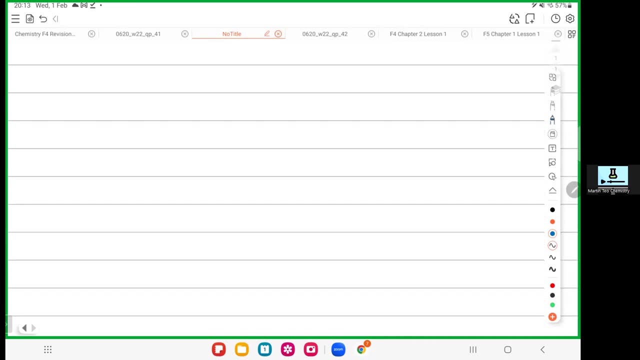 you ask your friend, you ask your school teacher, or what. So you must first understand: what is your own problem first, Because if you yourself don't know your problem, no people can help you. all right, Sorry for taking up so many time to talk about all this bullshit thing, but it's so. 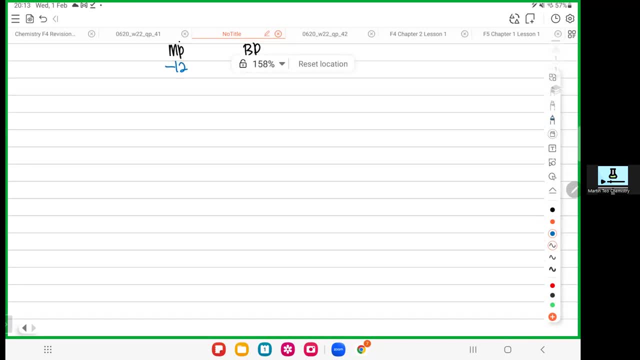 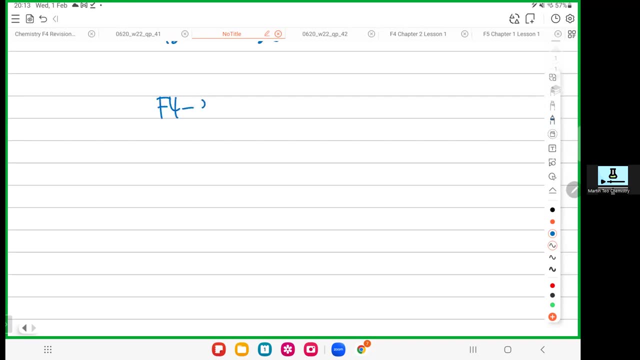 important, okay, Because many people were so lost. Many, many students were very lost, okay, Okay. so now let me give you the overview what we will learn in the Form 5.. So in your Form 4, there are total eight chapters. okay, When you come to Form 5, there is only five chapters. 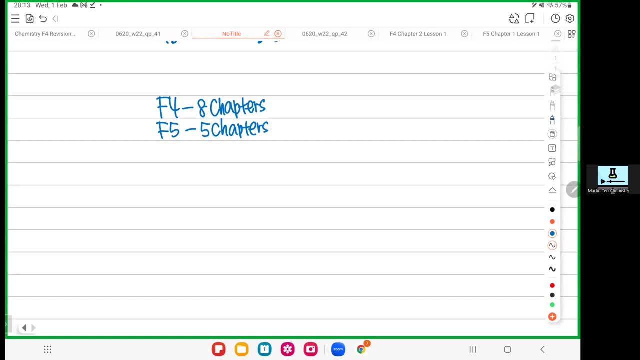 okay, There is only five chapters in your Form 5, okay, All right, So, but Form 5, the chapters will be more longer. okay, Form 5, the chapters? okay, might be a little bit longer. okay, Hold on. 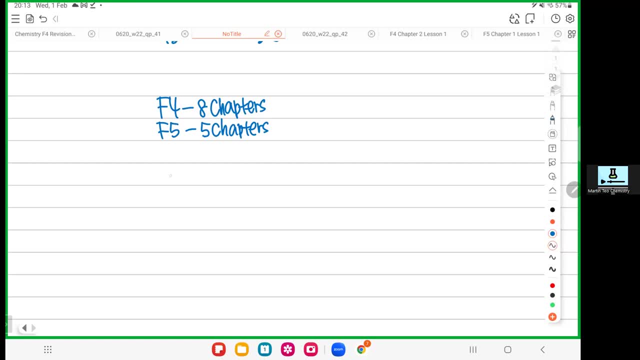 All right, All right, So we have Chapter 1.. Chapter 1 is called Redox Equilibrium. No need to copy all this thing out, I just give you a quick overview. I will tell you what we will do in this one year. 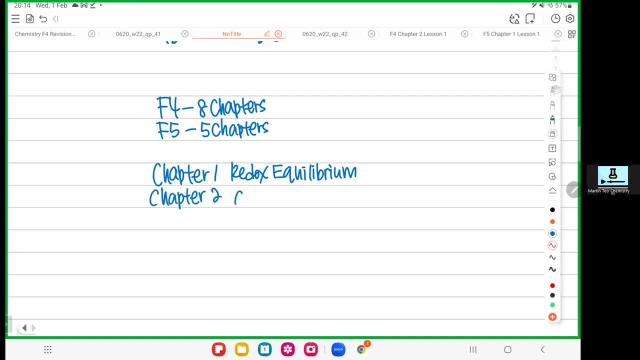 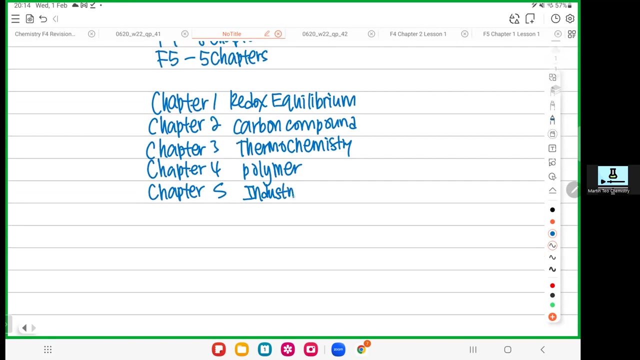 okay, Chapter 2 is called Carbon Compound. okay, Chapter 2 is called Carbon Compound, Chapter 3 is called Thermal Chemistry, Chapter 4 is called Thermal Chemistry, Chapter 4 is called Polymer And Chapter 5, okay- is called Industrial Chemistry. okay, All right, So your Chapter 1 will be the 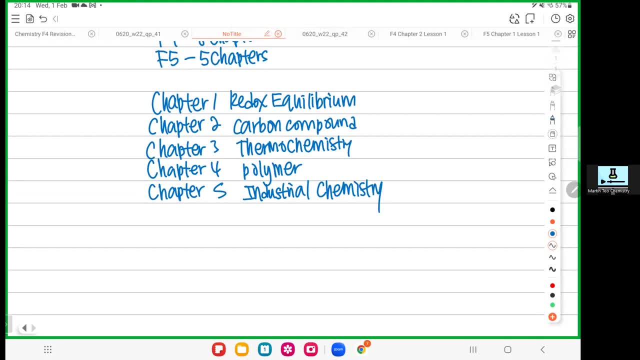 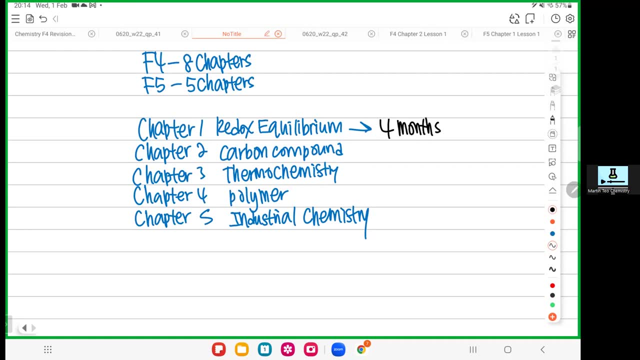 longest ever chapter you will encounter in these two years. okay, Chapter 1 itself, we will take a proximate four months. okay, We will Use a proximate four months just to learn about Chapter 1.. And Chapter 1 is the hardest chapter. 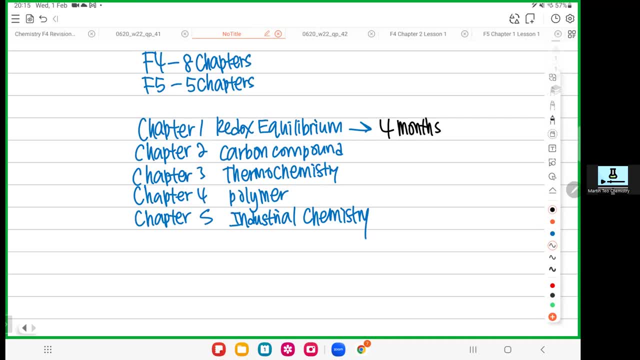 in the entire Form 4 and also the entire Form 5.. So I want you to stay focused and don't miss out any lesson, if possible. If you miss out the lesson, please, please, please get the recording, because if you miss out one lesson you might feel very lost already. okay, But don't get. 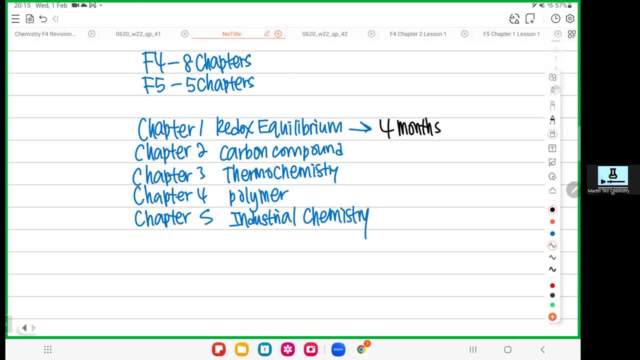 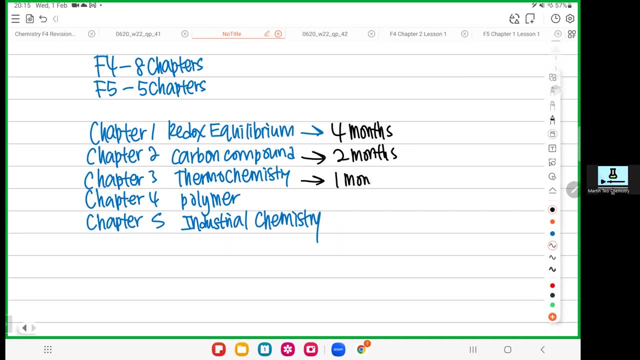 frightened by me. You follow my step one by one, step by step, you will be fine. So, Carbon Compound: we will spend about two months. Thermal Chemistry: we will spend one month. okay. Polymer: about one month. Industrial Chemistry. 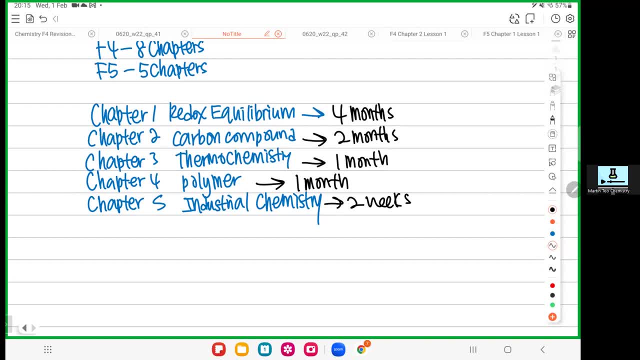 about two weeks. okay, So this is the basic planning. This is the basic planning for this year. okay, So we will spend a very, very long time on Redox Equilibrium. So, like what I say, so far, none of you actually, So far, none of you actually started with your How say So far. 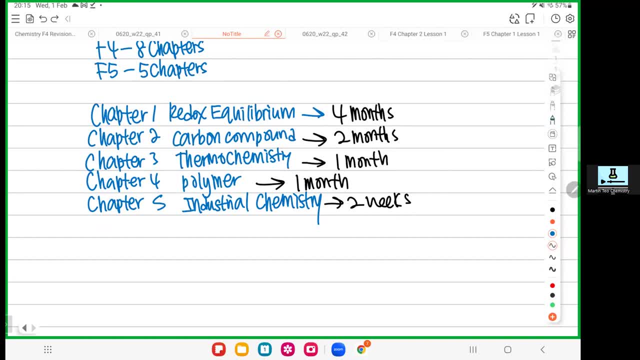 none of you actually already started with Chapter 1 in your school, So I assume you are just a white paper. You know nothing, which is good. That's why I'll teach you from scratch, and I'll teach you very, very slowly, okay, So that you can follow me. okay, So let's start. So the first thing that 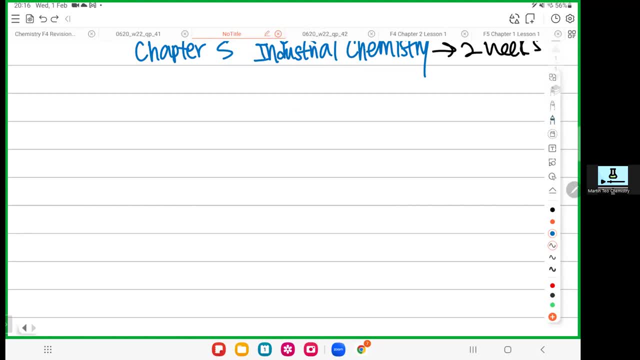 you need to learn today. the first thing that you need to learn today is this: You need to understand the word core, Redox. okay, So what is Redox? The word Redox comes from two words: The. the second word is ox, re and ox. so the re means reduction, so there is a chemical process called 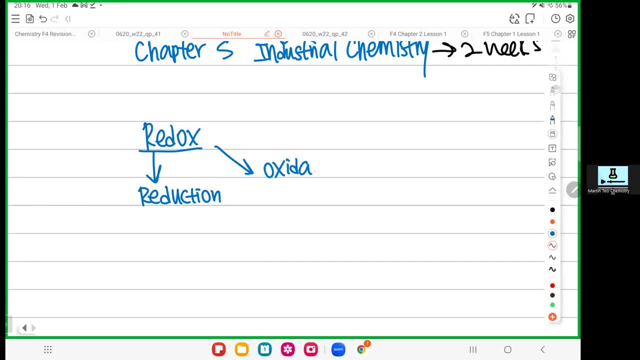 reduction, the ox means oxidation. so these two words, very important, you will keep on. you will be bombarded with these two words for the next four months. in the next four months, i'll keep talking about these two words until you want to vomit. yeah, reduction and oxidation. so what do we? 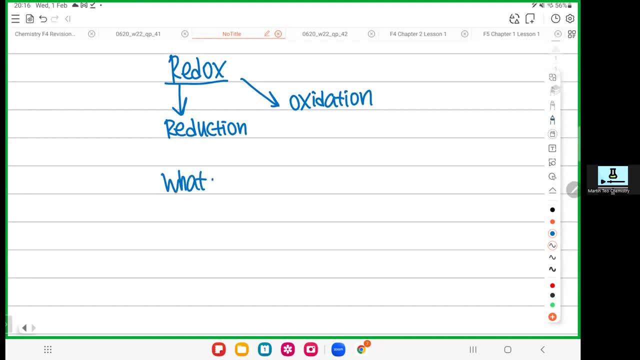 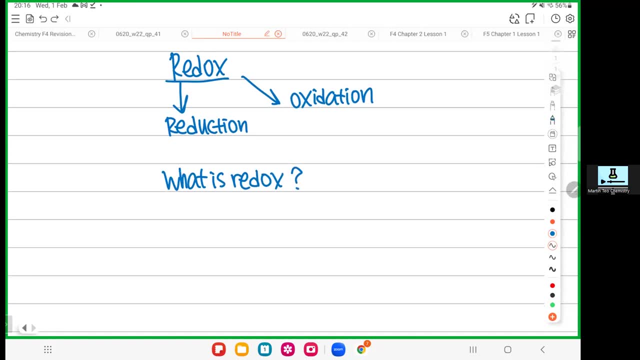 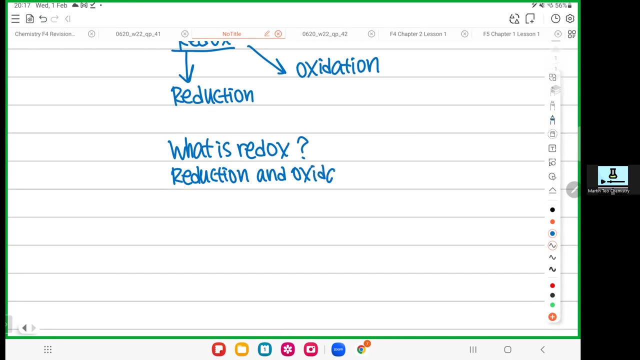 mean by redox. so sometimes spm can ask you a simple question: what is redox? hey, they can ask this: what is redox? and give you one mark in spm. so what is redox? redox means that you have reduction and also you have oxidation. these two process, they occur. you can use the word occur, you can. 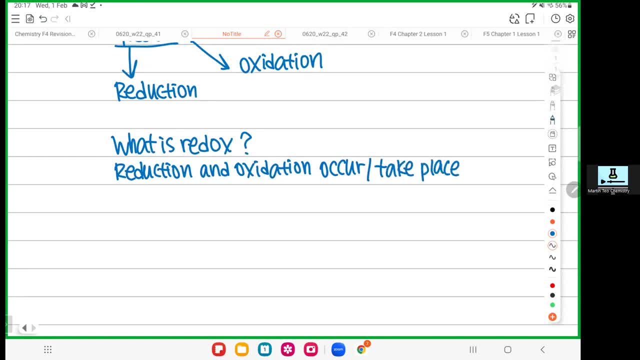 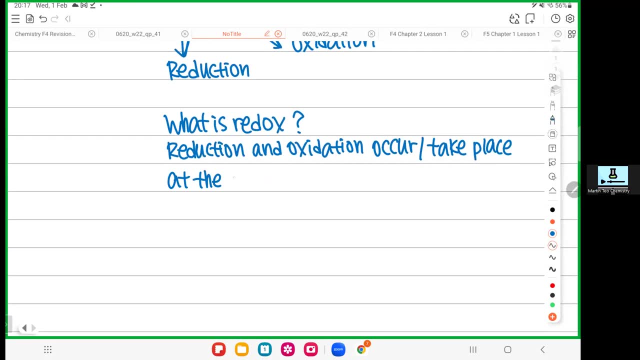 use the word take place. you can use a simple word: happen, doesn't matter. okay, all right, at the same time. okay, when you have oxidation process and reduction process, these two processes happen at the same time. that is called redox. you must have both. if, let's say, this chemical reaction only got reduction, don't have. 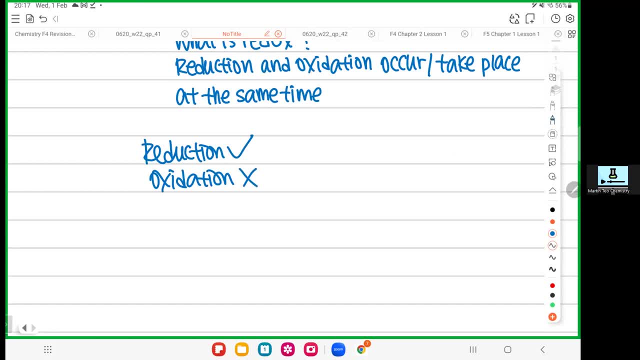 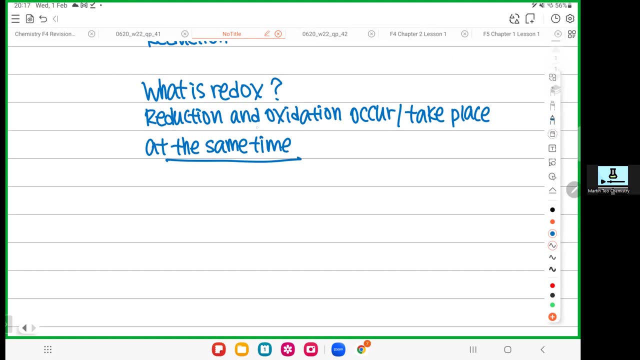 oxidation, it's not a redox. if this chemical process only have oxidation, don't have reduction, it's not a redox. redox must have reduction and oxidation happen at the same time. sometimes the school they do the, the textbook they don't use at the same time they use a very fancy word: they say reduction and 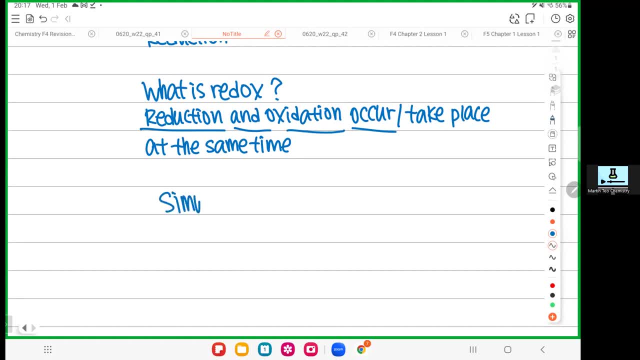 oxidation occur simultaneously. same thing: simultaneously means at the same time. okay, so make sure everyone know what the definition of redox. what is redox? they always ask this in your paper too. okay, you write this. you're going to get one mark, so that's the first thing, okay. 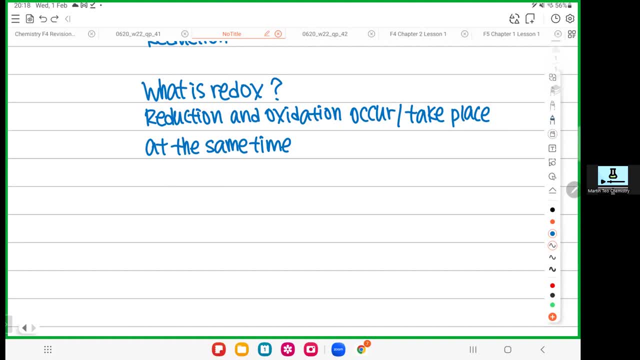 what is redox? oxidation and reduction happen at the same time. then some students ask, mr martin, can we write oxidation first, then only reduction? can we write oxidation and reduction happen at the same time? i put oxidation in front. can or cannot, can, the sequence doesn't matter. 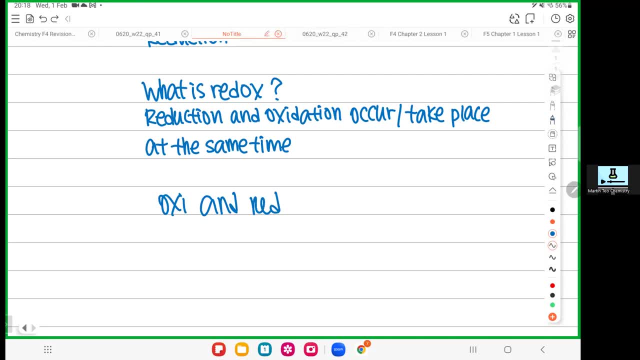 it doesn't matter, you write oxidation first, or, it doesn't matter, you write the reduction first, it doesn't matter. most importantly you write it okay. so that's the first thing we learned today. okay, up to this moment. can you guys please respond to me in the chat box? remember, send. 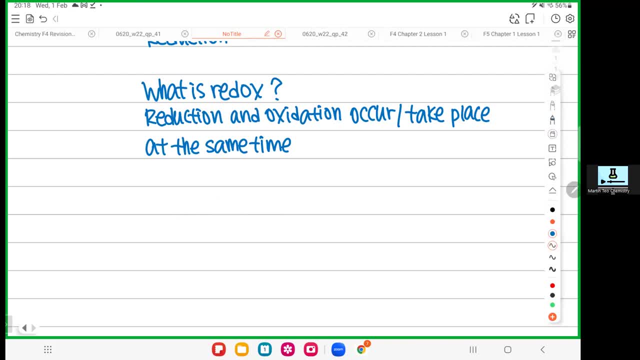 a message to the public space. are you guys okay with what is redox so far? okay, can, very good, okay, very good. so oxidation and reduction, these two process happen at the same time. it happened at the same time, so that is what we call redox, okay, so now the next thing we need. 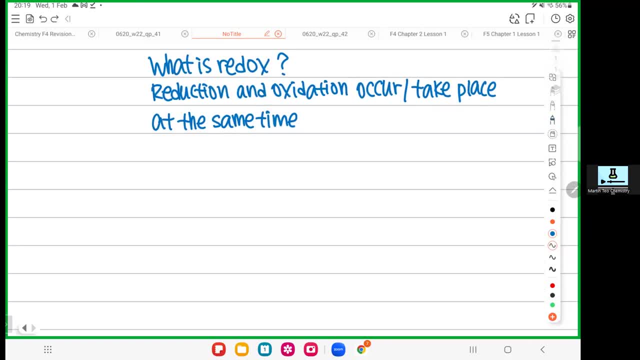 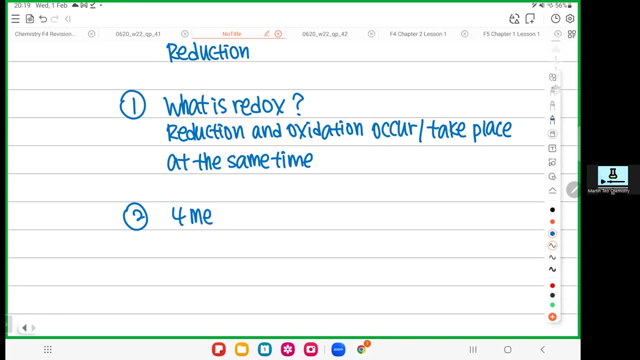 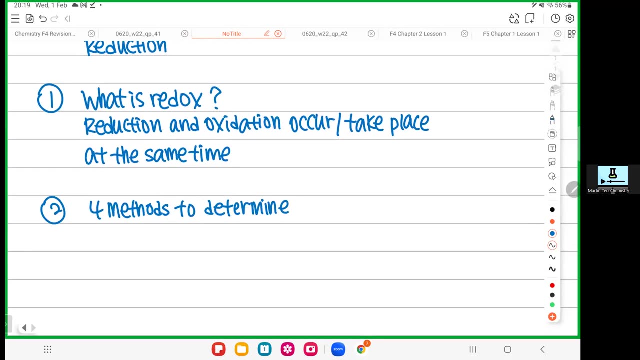 is this? what is oxidation? what is reduction? these two are something new for you. okay, so they are total four different methods. so we have four different methods in order to determine- okay, we have four different methods to know whether the process is oxidation or reduction. okay, we have four methods to determine this chemical process is oxidation or this chemical process? 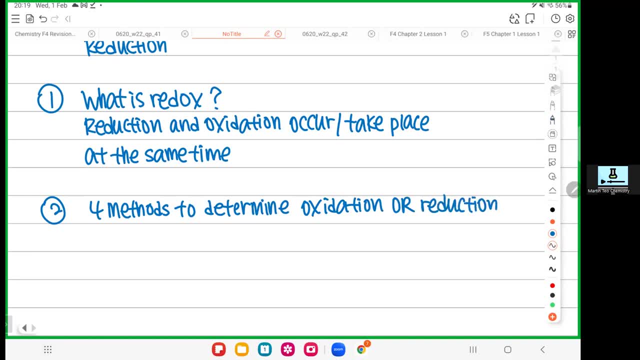 is reduction, because these two words is new for you in form four. maybe you heard about neutralization, you heard about combustion, something like that, okay, but you never heard about oxidation and reduction in form four. that's why it's something new for you. so how i, how am i going to know this? 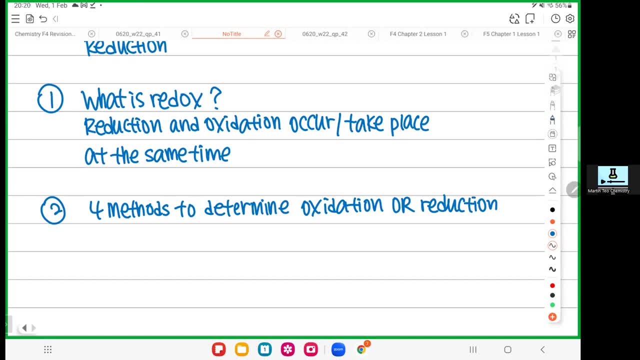 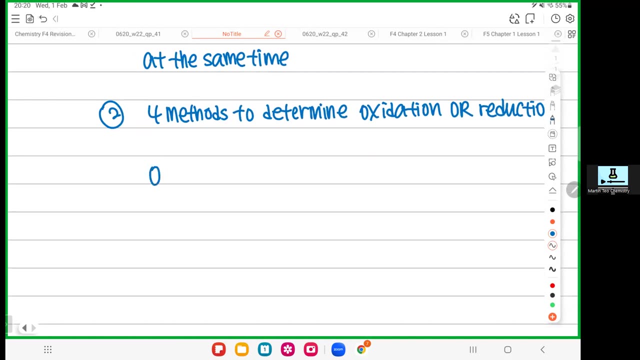 chemical process is oxidation or this chemical process is reduction, how to know? okay, let me teach you a very simple way and then we will do some past year question directly, so you know how to apply it. so let's look at it. so there is a very important table for you, okay, you see. so this is 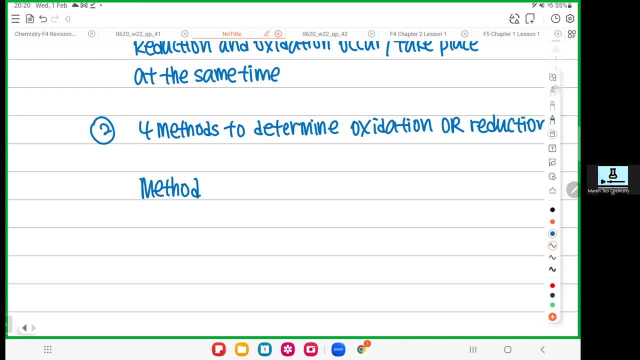 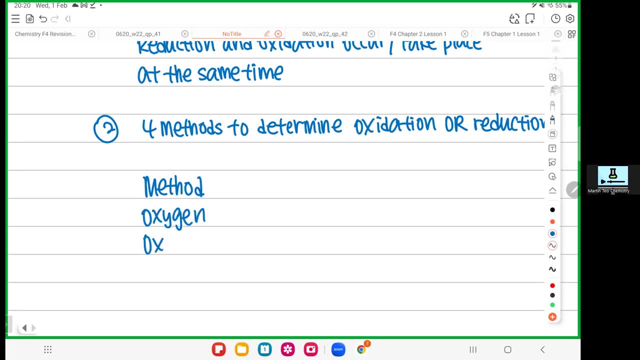 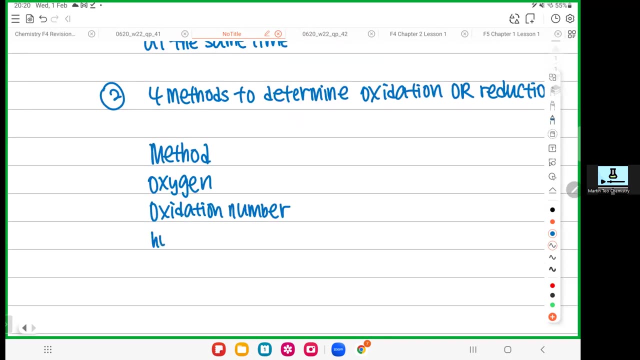 the method. okay, so you have four methods. okay, the first method is: you can look at the oxygen we call oxygen method. second method is called oxidation number method. okay, we will learn what is oxidation number, for no worry. then we can look at hydrogen method. then we can look at the last one called 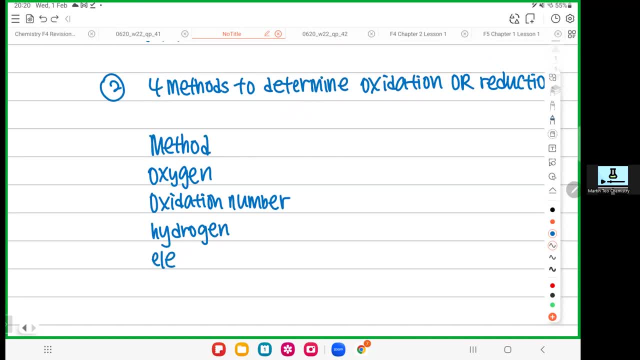 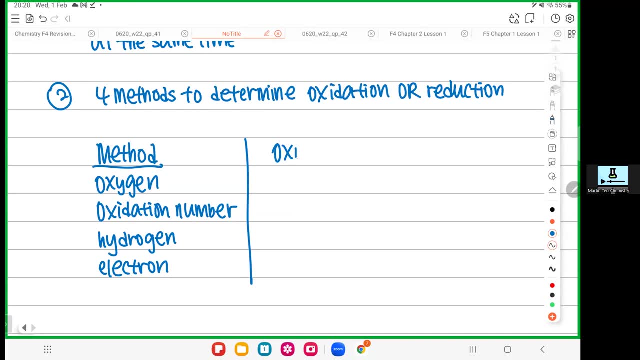 electron method. no worry, when you first started, of course, you'll feel confused, one which is completely normal. yeah, there are four methods we can use. okay, so i teach you a very simple way to memorize first. then i will explain to you one by one. okay, i teach you a simple way to memorize first. okay, so how to? 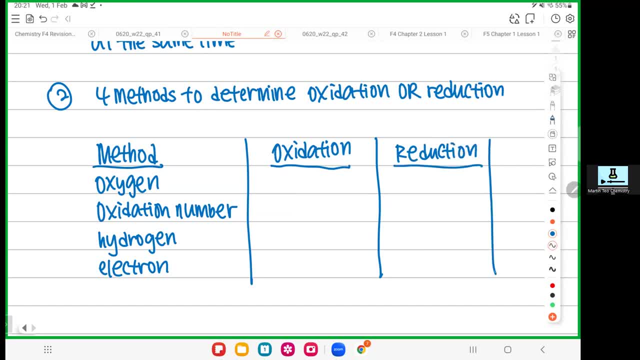 memorize it. so i teach you a simple way to cheat. so look at the first letter, so look at the first letter here you see, yeah right, this first letter is o. this first letter is o. if the first letter is the same, put a plus o and o. the first letter is the same plus o and h. the first letter is: 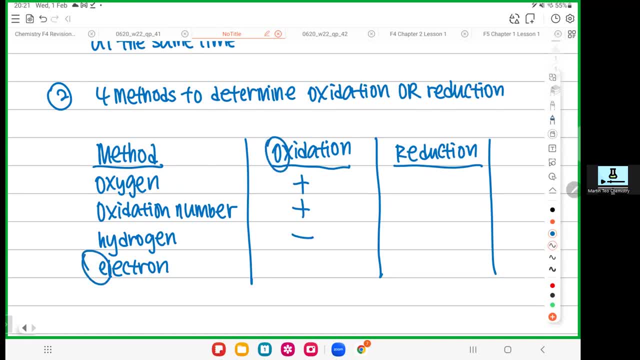 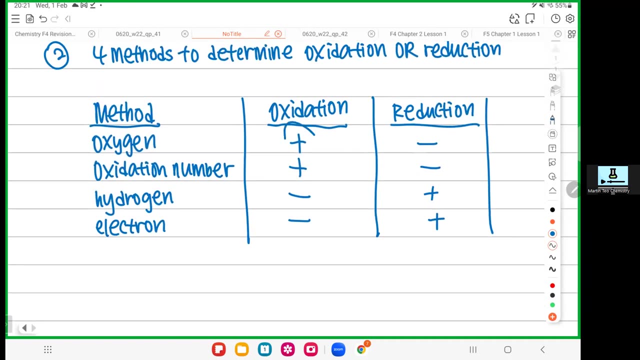 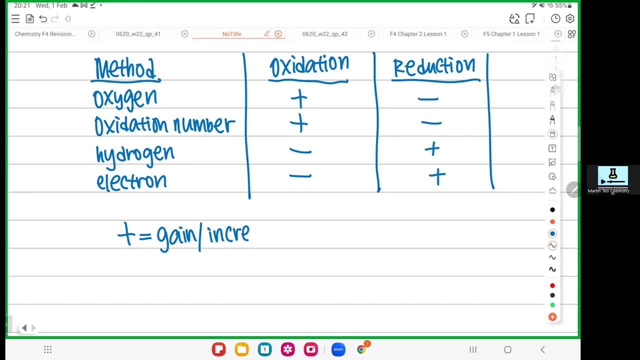 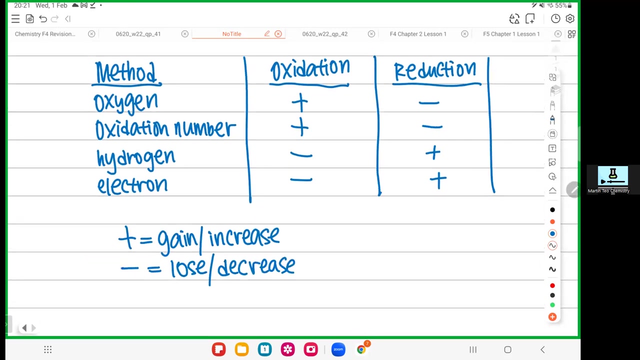 different. put a minus o and e. the first letter is different, put minus. so here everything: the plus plus, minor, minus. the ballet, minus minus, plus, plus. okay, what do i mean? if this chemical process plus means plus means gain, the plus means gain or increase, okay, the minus here means lose or decrease. so if this chemical process gain oxygen, 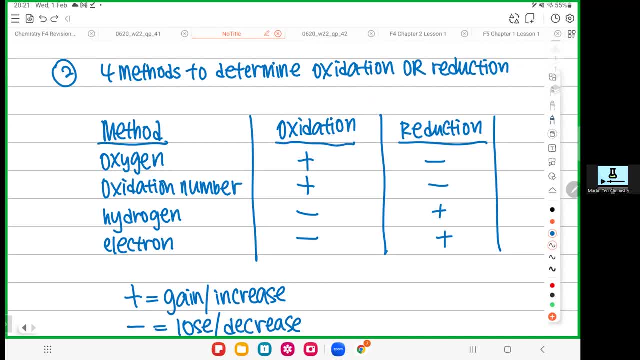 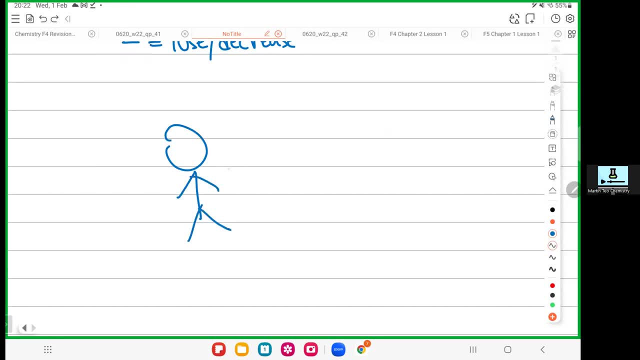 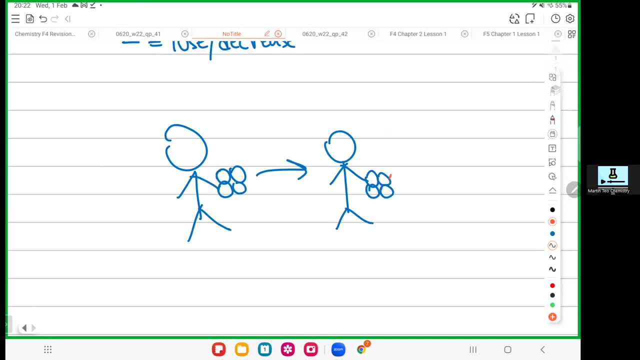 in my hand. so when i undergo a chemical process, process, process, now in my hand got seven oxygen already. now in my hand got seven oxygen already. now in my hand got seven oxygen already. okay, so now my oxygen increased. so when i? okay, so now my oxygen increased. so when i 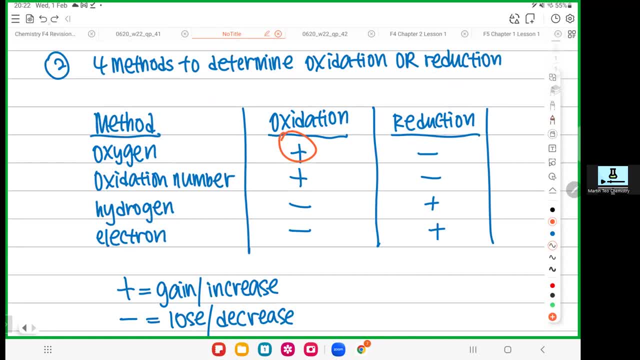 okay. so now my oxygen increased. so when i increase the oxygen, increase the oxygen, increase the oxygen. i undergo oxidation process. same thing, i undergo oxidation process. same thing, i undergo oxidation process. same thing, like the ballet if i decrease the oxygen. like the ballet if i decrease the oxygen. 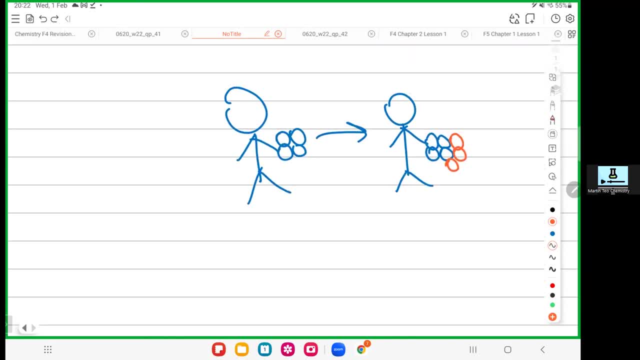 like the ballet: if i decrease the oxygen i undergo reduction. so let's say i undergo reduction. so let's say i undergo reduction. so let's say, initially i got initially. i got initially. i got four oxygen on my hand. four oxygen on my hand, four oxygen on my hand, so now four oxygen now all in sudden. 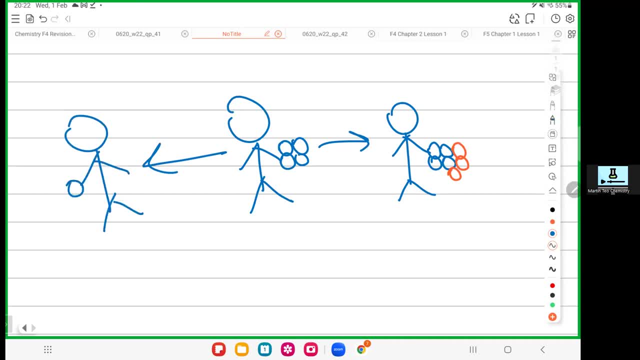 so now four oxygen, now all in sudden. so now four oxygen, now all in sudden. become only one oxygen, so i lose oxygen. become only one oxygen, so i lose oxygen. become only one oxygen, so i lose oxygen. right from four, right from four, right from four oxygen, now only left one, i lose oxygen. so 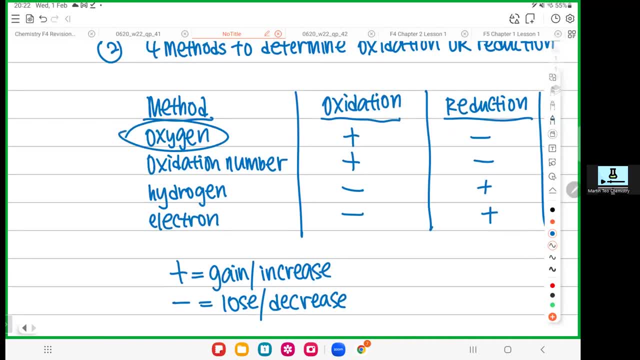 oxygen now only left one, i lose oxygen. so oxygen now only left one, i lose oxygen. so that is reduction, that's it. so. this is that is reduction, that's it. so. this is that is reduction, that's it. so this is oxygen method. we will learn more later. 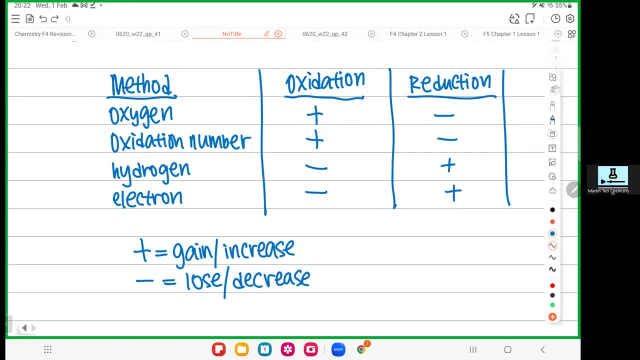 oxygen method: we will learn more later. oxygen method: we will learn more later. next one, next one, next one: oxidation number: oxidation number we oxidation number, oxidation number we oxidation number, oxidation number. we will learn later also. ah, no, worry okay, will learn later also. ah, no, worry okay. 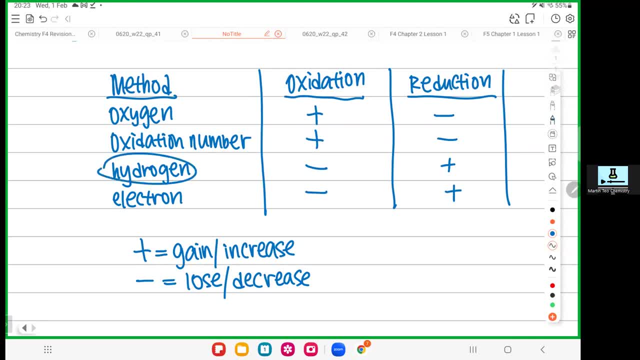 will learn later also. ah no worry, okay. so this one a little bit tricky, we'll so this one a little bit tricky, we'll. so this one a little bit tricky, we'll learn later. okay, next one same thing, learn later. okay. next one same thing, learn later. okay, next one same thing: hydrogen. so if you lose, minus means. 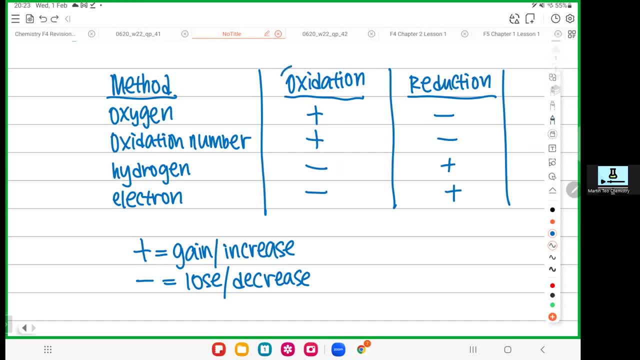 hydrogen. so if you lose minus means hydrogen. so if you lose, minus means lose. if i lose hydrogen, i undergo lose. if i lose hydrogen, i undergo lose. if i lose hydrogen, i undergo oxidation, oxidation, oxidation if i, if i, if i gain gain, gain, sorry if i, sorry if i. 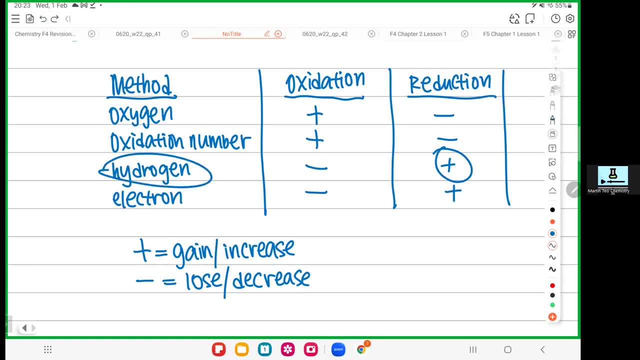 sorry, if i gain hydrogen, i undergo reduction. so same hydrogen, i undergo reduction. so same hydrogen, i undergo reduction. so same thing, thing, thing. let's say initially, i have a substance. let's say initially, i have a substance. let's say initially i have a substance. okay, on the left hand side, let's say i. 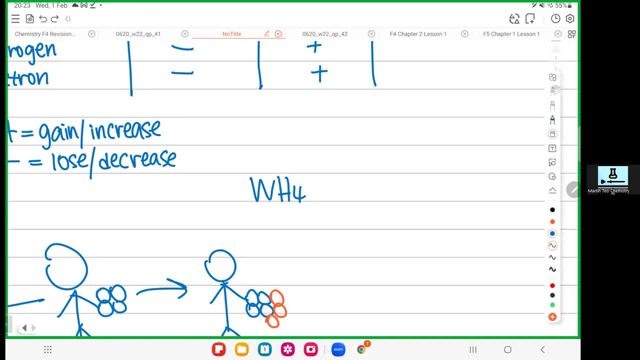 okay on the left hand side. let's say i. okay on the left hand side. let's say i got wh4. i got four hydrogen on the left, got wh4. i got four hydrogen on the left, got wh4. i got four hydrogen on the left hand side. go to right hand side become. 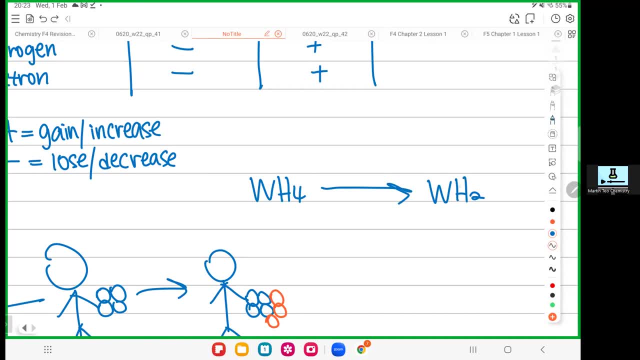 hand side. go to right hand side, become hand side. go to right hand side, become wh2, wh2, wh2. from four hydrogen become two hydrogen. so from four hydrogen become two hydrogen, so from four hydrogen become two hydrogen. so what happened? i lose oxidation. what happened? i lose oxidation. 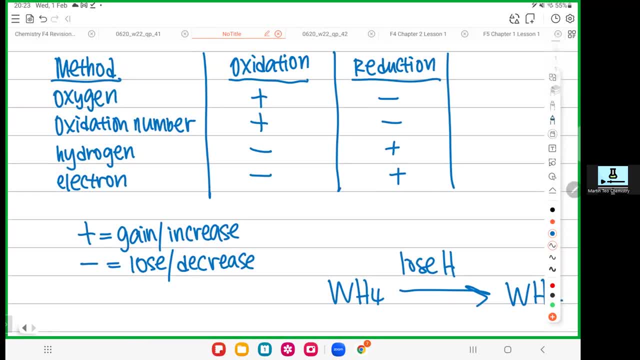 what happened? i lose oxidation, okay, i loses hydrogen already. so when i- okay, i loses hydrogen already. so when i- okay, i loses hydrogen already. so when i lose hydrogen, so look at hydrogen lose, lose hydrogen, so look at hydrogen lose. lose hydrogen, so look at hydrogen. lose means minus, so lose hydrogen means. 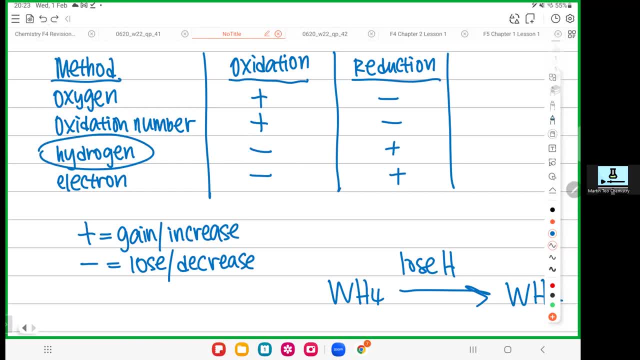 means minus, so lose hydrogen means means minus, so lose hydrogen means oxidation process, so that's it okay. so oxidation process, so that's it okay. so oxidation process, so that's it okay. so by looking at these four different, by looking at these four different, by looking at these four different perspective, then you know already. 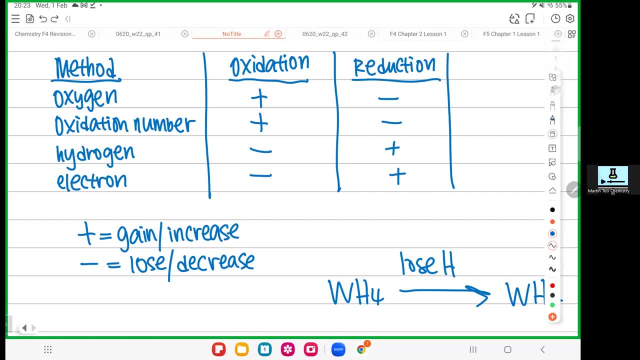 perspective, then you know already perspective, then you know already whether the reaction is oxidation or whether the reaction is oxidation, or whether the reaction is oxidation or reduction, so same thing if i reduction, so same thing if i reduction, so same thing if i gain electron, if this chemical reaction 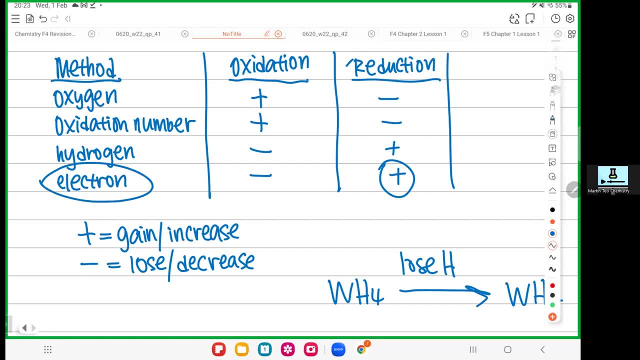 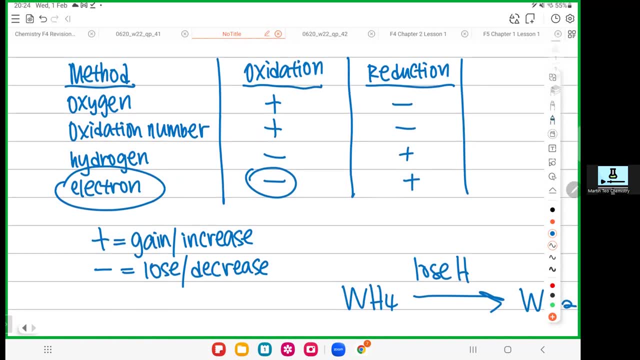 gain electron. if this chemical reaction gain electron. if this chemical reaction gain electron. if i receive electron from gain electron. if i receive electron from gain electron. if i receive electron from other people, i undergo reduction. other people, i undergo reduction. other people, i undergo reduction, oxidation. okay, so this table is the most. 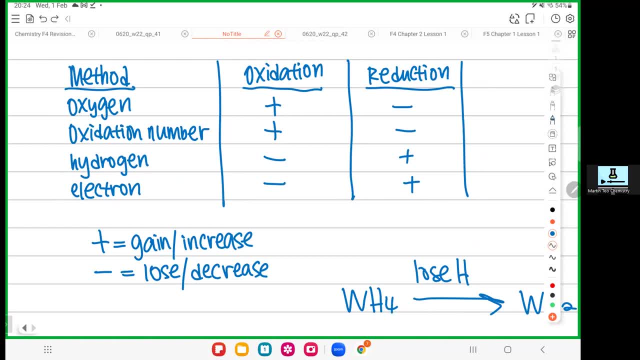 oxidation. okay, so this table is the most oxidation. okay, so this table is the most important thing in your entire chapter, important thing in your entire chapter, important thing in your entire chapter one. if you don't know this table you one. if you don't know this table you. 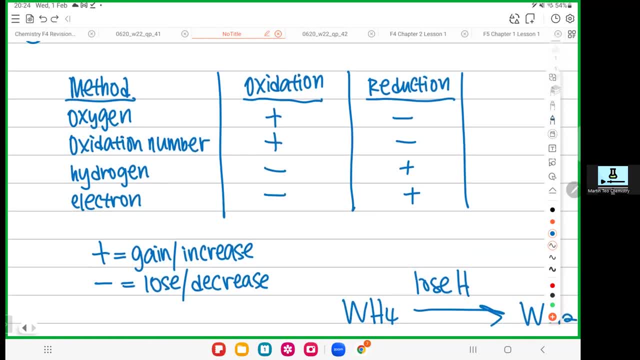 one. if you don't know this table, you cannot move on with chapter one anymore. cannot move on with chapter one anymore. cannot move on with chapter one anymore. so of course, when you first started you, so of course when you first started you, so of course when you first started, you feel confused, which is okay, which is. 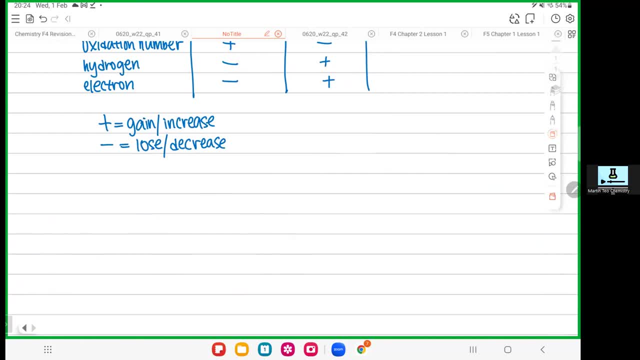 feel confused, which is okay, which is feel confused, which is okay, which is normal, okay. so, how are you going to normal, okay? so how are you going to normal, okay? so how are you going to familiarize yourself easier and faster? familiarize yourself easier and faster. familiarize yourself easier and faster. take a piece of paper, this table copy. 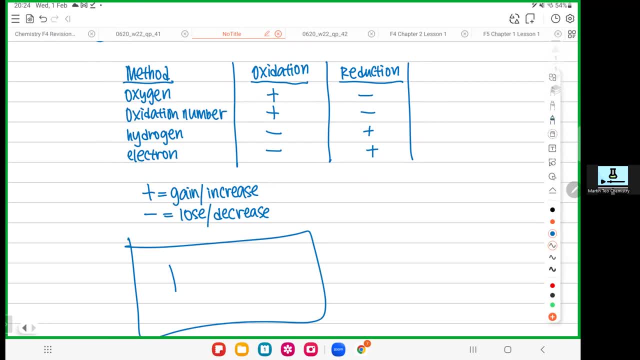 take a piece of paper. this table copy. take a piece of paper. this table copy for a few times every day. copy this for a few times every day. copy this for a few times every day. copy this table for one time. table for one time. table for one time. do it continuously. maybe one week you. 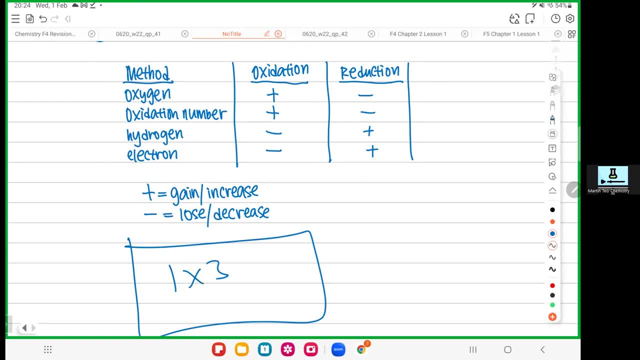 do it continuously, maybe one week. you do it continuously, maybe one week. you copy three times, copy three times, copy three times. do it continuously for one or two weeks. do it continuously for one or two weeks. do it continuously for one or two weeks. then you will be able to remember you. 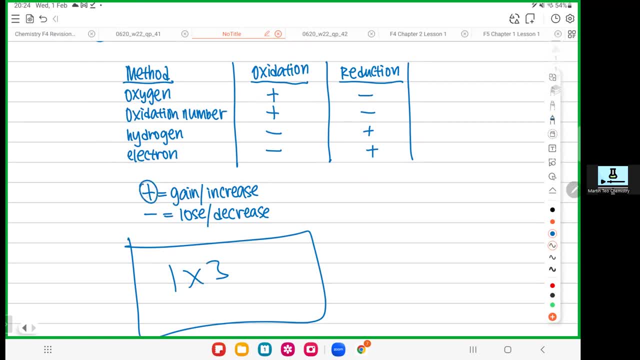 then you will be able to remember you, then you will be able to remember. you won't forget already. okay, this is very won't forget already. okay, this is very won't forget already. okay, this is very, very important. okay, you must know this, very important. okay, you must know this. 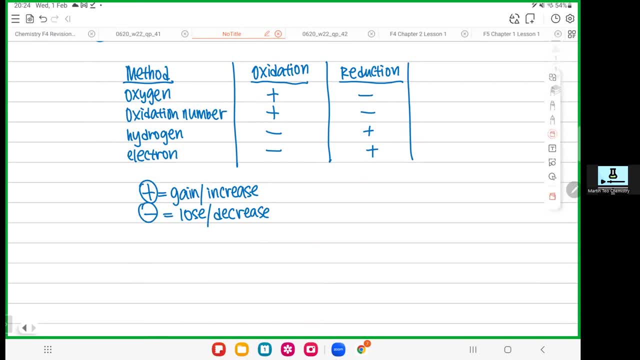 very important. okay, you must know this table. okay now, why this table, so table. okay now, why this table, so table. okay now, why this table so important and how the question can be important and how the question can be important and how the question can be tested in the real examination. how. 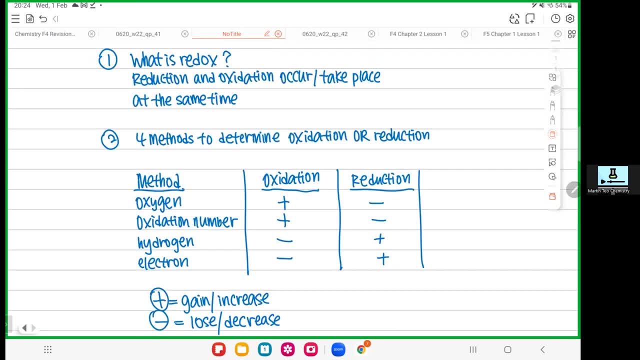 tested in the real examination, how tested in the real examination, how actually they can ask us the question. actually they can ask us the question, actually they can ask us the question. okay, right, so let me show you, uh, how the. okay, right, so let me show you, uh, how the. 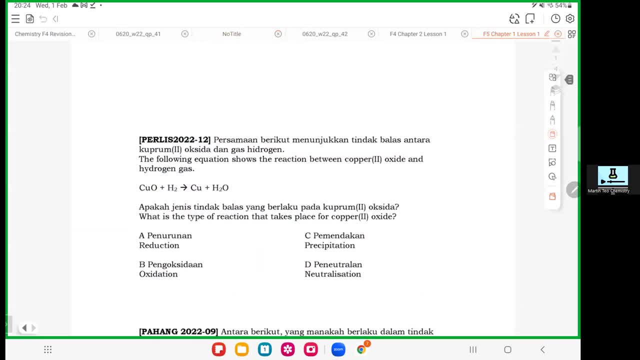 okay, right, so let me show you, uh, how the question can be asked. so let me show you question can be asked. so let me show you question can be asked. so let me show you the question here. okay, so this question. the question here. okay, so this question. 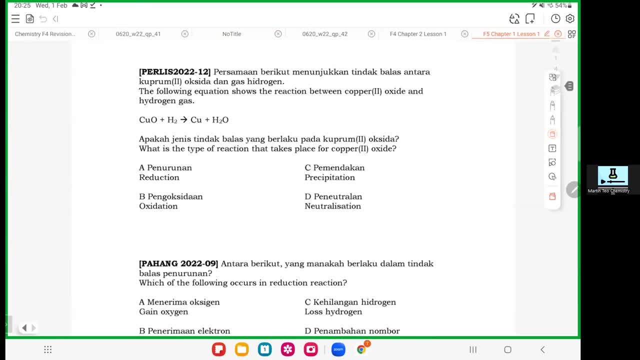 the question here. okay, so this question is all coming from good quality question, is all coming from good quality question, is all coming from good quality question. all the questions i'm showing you today, all the questions i'm showing you today, all the questions i'm showing you today, they are coming from trial exam paper. 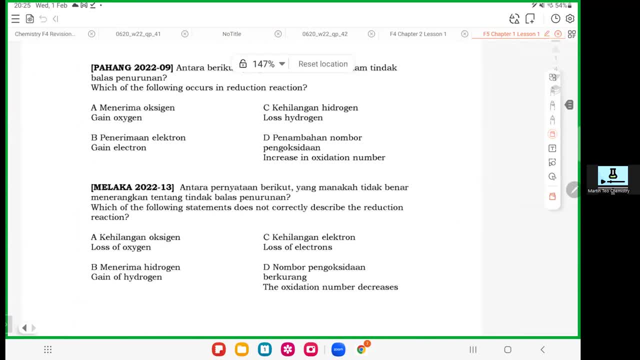 they are coming from trial exam paper. they are coming from trial exam paper. okay, they are coming from trial exam. okay, they are coming from trial exam. okay, they are coming from trial exam paper. so let me show you the first one paper. so let me show you the first one. 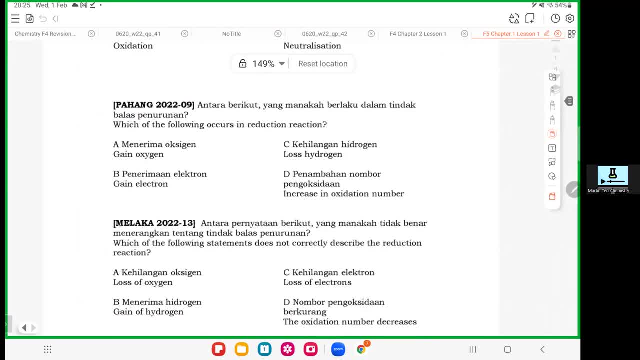 paper. so let me show you the first one. this is the first question coming from. this is the first question coming from. this is the first question coming from pahang, and also this is coming from pahang and also this is coming from pahang and also this is coming from malacca. okay, so what they want, so they. 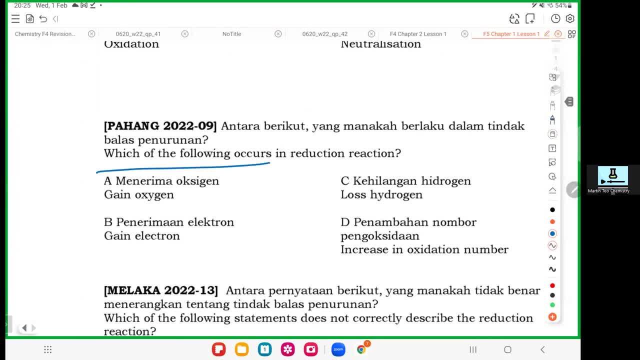 malacca. okay, so what they want. so they malacca. okay, so what they want. so they say: first one question. which of the say first one question? which of the say first one question? which of the following occur in reduction reaction? following: occur in reduction reaction: 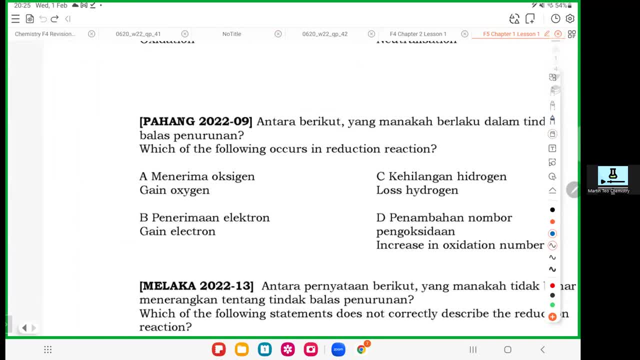 following occur in reduction reaction. which of the following occur in the which of the following occur in the which of the following occur in the reduction reaction: so reduction. so how i reduction reaction, so reduction. so how i reduction reaction, so reduction. so how i do it. so remember, let's do a table. 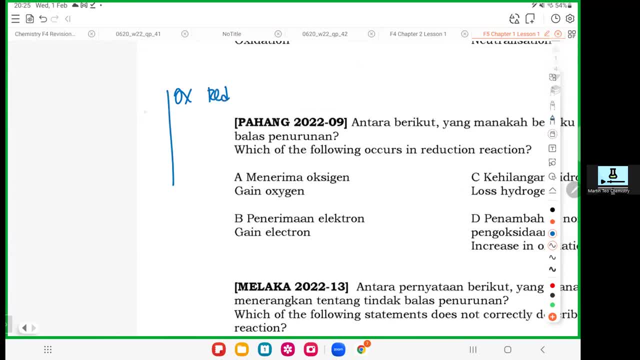 do it, so remember, let's do a table. do it, so remember, let's do a table. oxidation reduction. so there are four oxidation reduction. so there are four oxidation reduction. so there are four methods. first, method: oxygen method methods. first method oxygen method methods. first, method oxygen method. second method: oxidation number method. 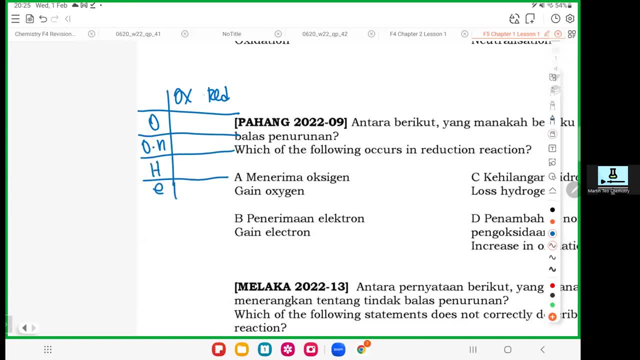 second method: oxidation number method. second method: oxidation number method. third method is hydrogen method. fourth third method is hydrogen method. fourth third method is hydrogen method. fourth method is electron. okay, four method. so method is electron. okay, four method. so method is electron, okay, four method. so how to remember? look at the first. 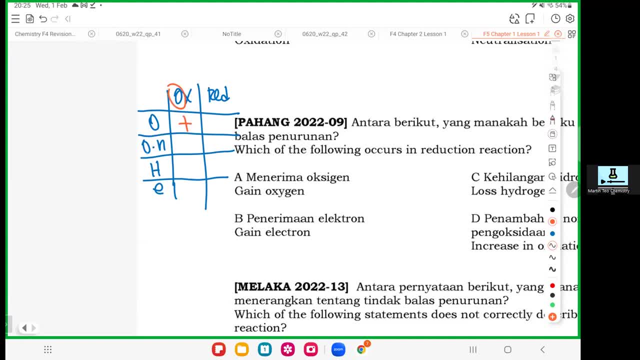 how to remember. look at the first. how to remember. look at the first letter: o and o plus o and o plus letter o and o plus o and o plus letter o and o plus o and o plus o and h. different letter minus o and e. o and h. different letter minus o and e. 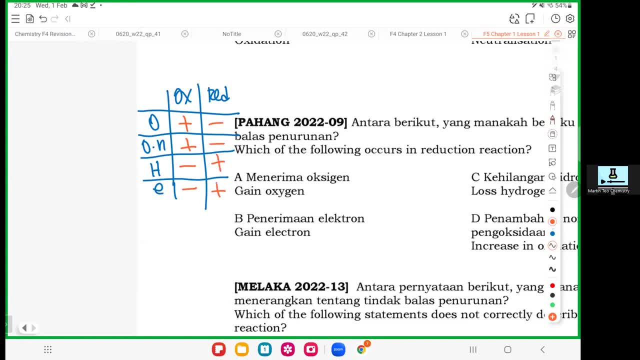 o and h different letter. minus o and e different letter. minus the valid minus different letter. minus the valid minus different letter: minus the valid minus. minus plus plus, so what they want. they minus plus plus, so what they want. they minus plus plus, so what they want. they want reduction, so focus on reduction here. 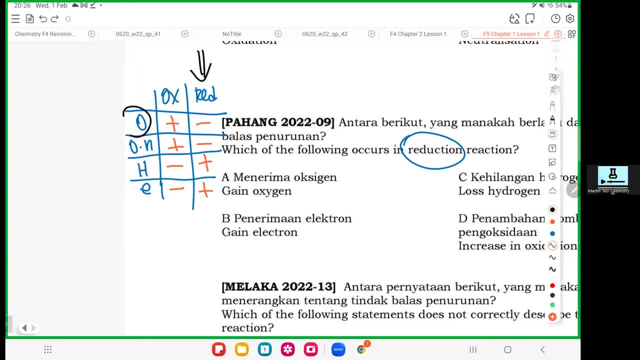 want reduction, so focus on reduction here. want reduction, so focus on reduction here. so reduction gain oxygen, yes or no. so reduction gain oxygen yes or no. so reduction gain oxygen, yes or no. oxygen reduction is what minus minus oxygen reduction is what minus minus oxygen reduction is what minus minus means lose. so it's wrong. 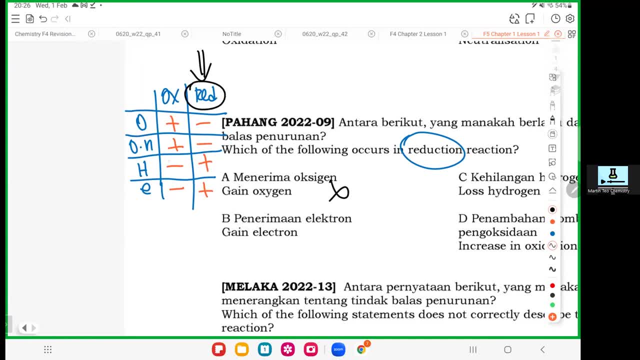 means lose, so it's wrong. means lose, so it's wrong. so let's look at b gain electron. so so let's look at b gain electron. so so let's look at b gain electron. so reduction electron electron is plus reduction electron electron is plus reduction electron electron is plus plus means gain, so the answer is b. 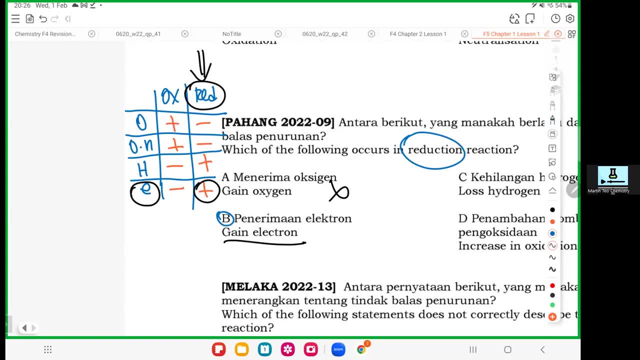 plus means gain, so the answer is b. plus means gain, so the answer is b. so can you guys please type in the chat? so can you guys please type in the chat. so can you guys please type in the chat box and let me know. are you okay with? 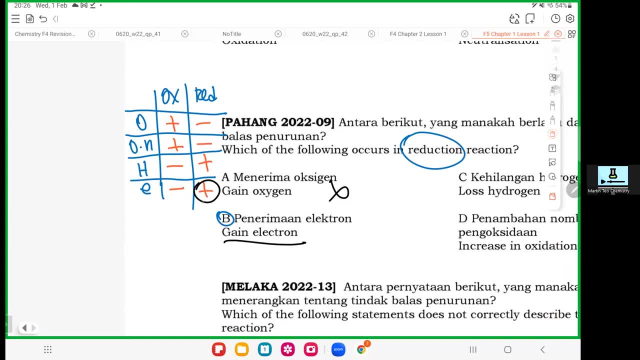 box and let me know, are you okay with box? and let me know, are you okay with this concept so far? so this question is very straightforward. so this question is very straightforward. so this question is very straightforward if you, if you, if you understand, understand, understand the table, if you can memorize these. 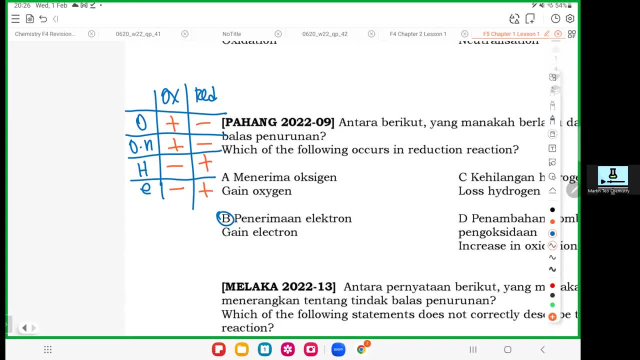 the table if you can memorize these, the table, if you can memorize these. table is super, super straightforward. table is super, super straightforward. table is super, super straightforward. same thing if you don't know this table. same thing if you don't know this table. same thing if you don't know this table at all. you cannot do if you don't know. 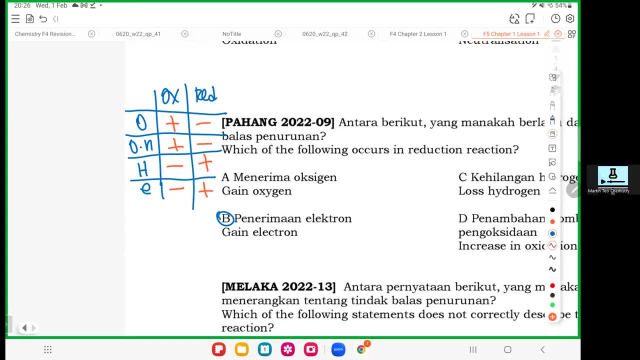 at all. you cannot do if you don't know at all. you cannot do if you don't know this table at all. you cannot do. that's this table at all, you cannot do. that's this table at all, you cannot do. that's why this table is so important. yeah, this. 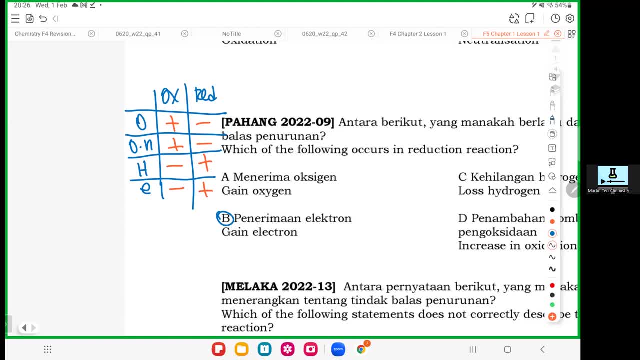 why this table is so important. yeah, this, why this table is so important. yeah, this table it is so important. okay, so now table it is so important. okay, so now table, it is so important. okay, so now let's move on. let's try, let's move on, let's try. 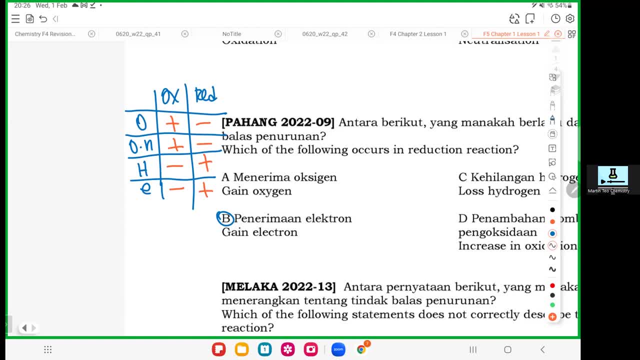 let's move on. let's try: i do a few more, then i let you try. okay, i do a few more. then i let you try. okay, i do a few more, then i let you try. okay, i do a few more with you all. then i do a few more with you all then. 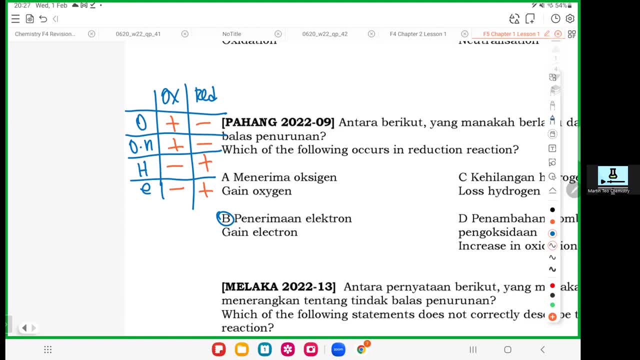 i do a few more with you all, then, okay, okay, okay, i let you try, okay, i let you try, okay, i let you try. okay, okay, come, okay, come, okay, come, yeah, yeah, yeah, this is malacca paper same thing. this is malacca paper same thing. 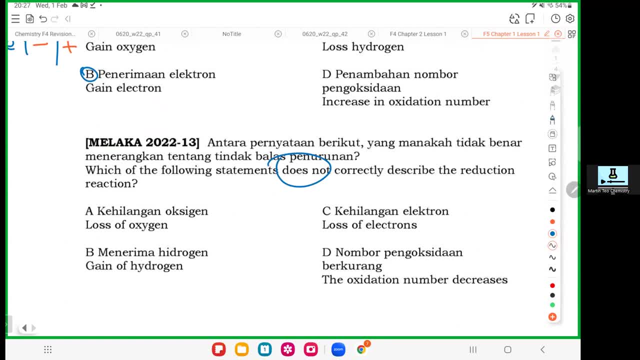 this is malacca paper, same thing. which of the following statement does not? which of the following statement does not? which of the following statement does not: correctly describe the reduction? so correctly describe the reduction. so correctly describe the reduction. so that's not means: do you want something? 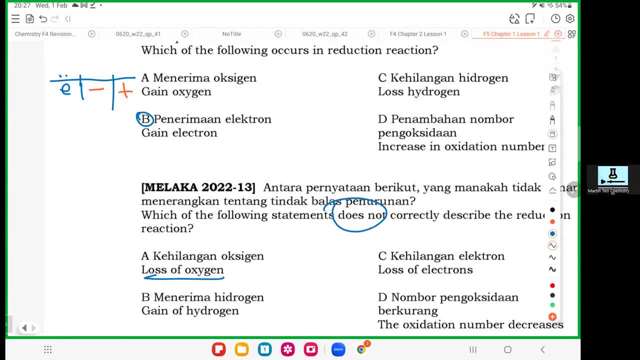 that's not means do you want something. that's not means do you want something wrong, something wrong wrong, something wrong wrong something wrong. lose oxygen- yes or no oxygen. lose oxygen- yes or no oxygen. lose oxygen- yes or no oxygen. lose oxygen. it is reduction, yes, but we're. 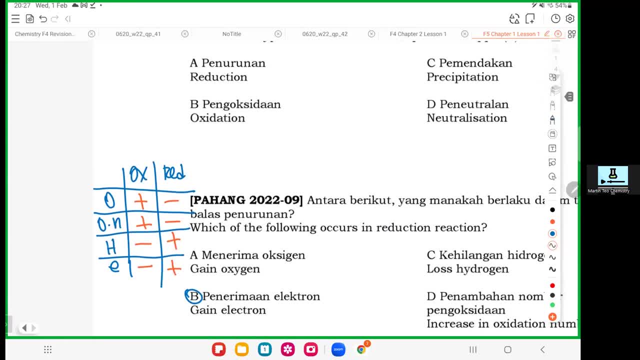 lose oxygen. it is reduction, yes, but we're lose oxygen. it is reduction, yes, but we're looking for something wrong. looking for something wrong, looking for something wrong. gain hydrogen: yes or no. hydrogen gain gain: hydrogen: yes or no. hydrogen gain. gain hydrogen- yes or no. hydrogen gain- hydrogen reduction: yes. 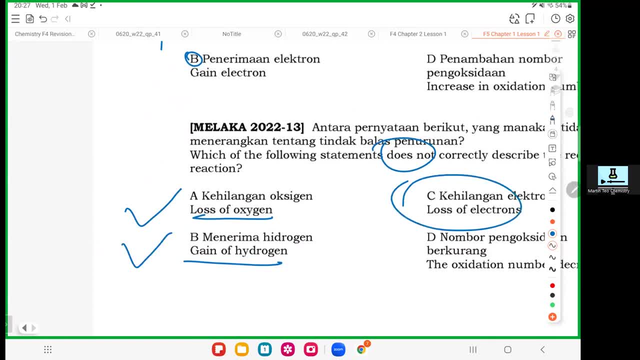 hydrogen reduction: yes, hydrogen reduction, yes, but we want something wrong. but we want something wrong, but we want something wrong. lose electron, so let's look at electron. lose electron, so let's look at electron. lose electron, so let's look at electron, electron, electron, electron lose, it should be oxidation, so wrong. 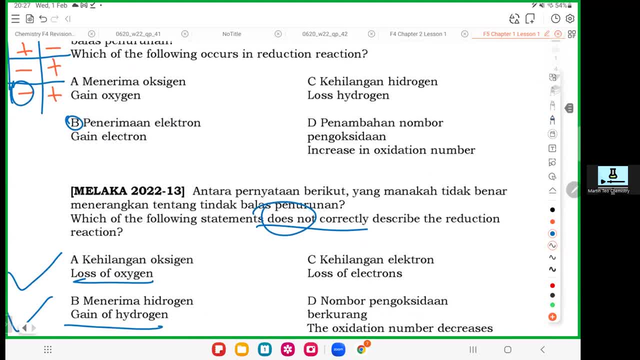 lose, it should be oxidation, so wrong. lose, it should be oxidation, so wrong. because we are looking for something does. because we are looking for something does, because we are looking for something does not correct. so the answer is c okay, so not correct. so the answer is c, okay, so 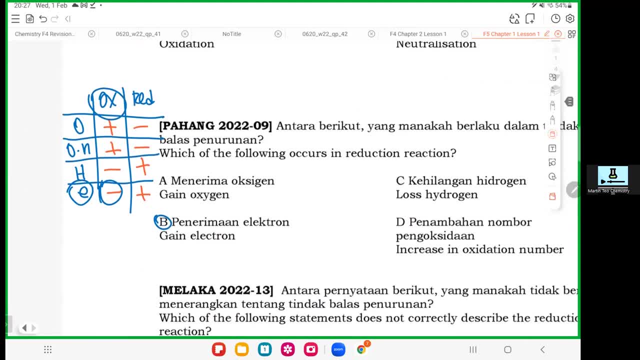 not correct. so the answer is c. okay, so actually it is very, very straightforward. actually, it is very, very straightforward. actually it is very, very straightforward. you know this table, you know this table. you know this table- uh, you are good to go. okay, you know this. uh, you are good to go. okay, you know this. 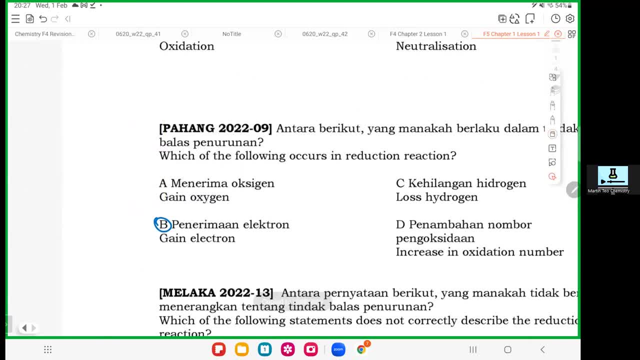 uh, you are good to go, okay, you know this table. you are good to go, okay, so let me table. you are good to go, okay, so let me table. you are good to go, okay, so let me copy this table first. huh, okay, so now. copy this table first. huh, okay, so now. 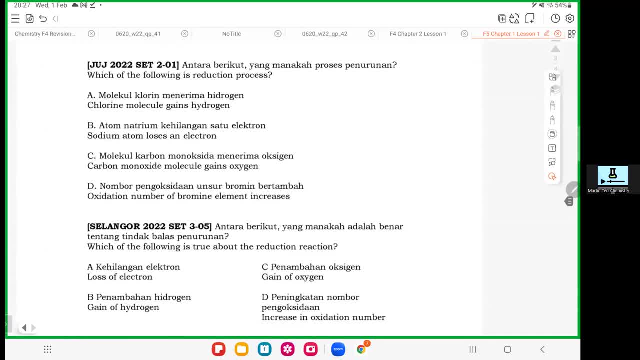 copy this table first. huh, okay, so now let's try another one, let's try another one, let's try another one. okay here, okay, okay here, okay, okay here. okay, this one, this one, this one. so this is a question from joho, this is so. this is a question from joho. this is. 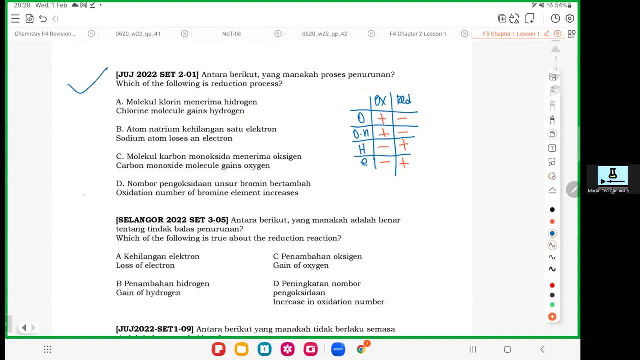 so this is a question from joho. this is the question from joho. probably you want the question from joho. probably you want the question from joho. probably you want to try this. try these two questions to try this. try these two questions to try this. try these two questions. type in the answer in the chat box. uh, 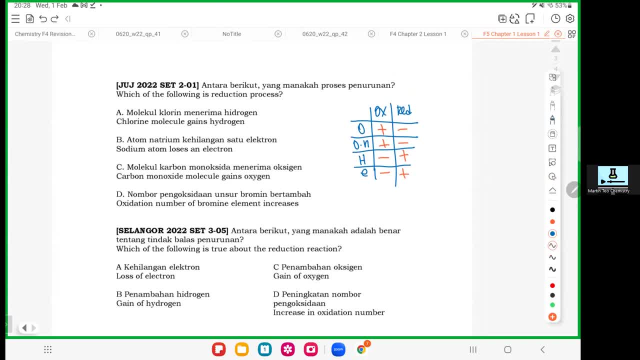 type in the answer in the chat box. uh, type in the answer in the chat box. uh, let's say for the first question, the let's say for the first question, the let's say for the first question, the answer. simply say, answer, simply say, answer. simply say: let's say the first question, the answer. 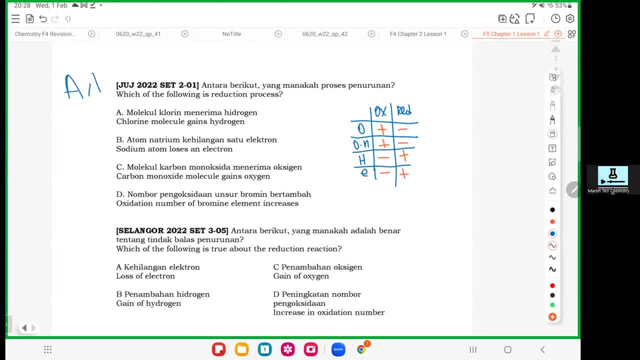 let's say the first question, the answer. let's say the first question. the answer is a second is b. simply say you type a is a second is b. simply say you type a is a second is b. simply say you type a, comma b in the chat box. okay, let's say: comma b in the chat box. okay, let's say: comma b in the chat box. okay, let's say: the first answer is c, second is donkey. the first answer is c, second is donkey. the first answer is c, second is donkey. you type in the chat box. okay, let's say: 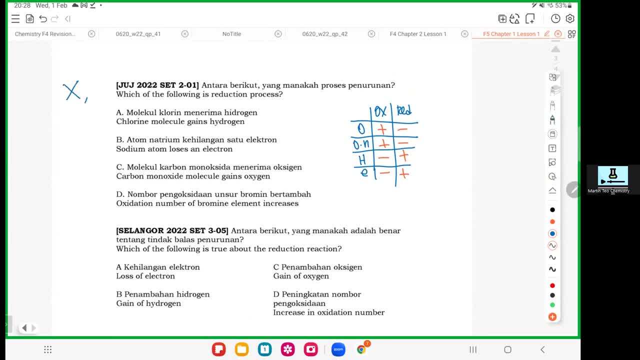 you type in the chat box. okay, let's say. you type in the chat box. okay, let's say you don't know how to do the first, you don't know how to do the first, you don't know how to do the first question. you type cross second one: you. question: you type cross. second one: you question: you type cross. second one: you know how to do. you can type b if both know how to do. you can type b if both know how to do. you can type b if both questions you don't know, you type both. 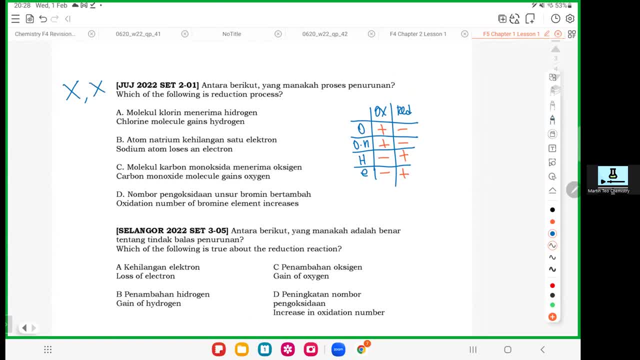 questions you don't know. you type both questions you don't know. you type both. process. okay, i want at least you reply process. okay, i want at least you reply process. okay, i want at least you reply me. i want you all to reply me, come on me. i want you all to reply me, come on. 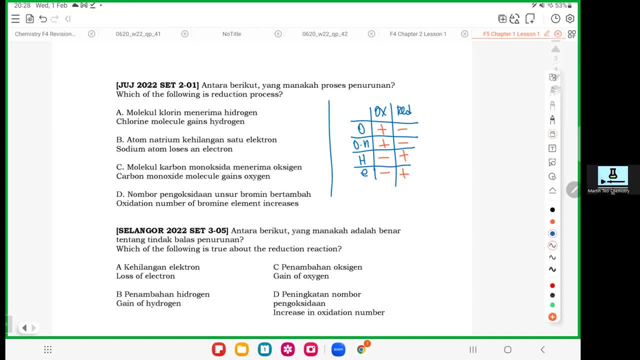 me. i want you all to reply me. come on, let's try. let's try this. you are allowed. let's try. let's try this. you are allowed. let's try, let's try this. you are allowed to refer to this table by today. okay for to refer to this table by today. okay for. 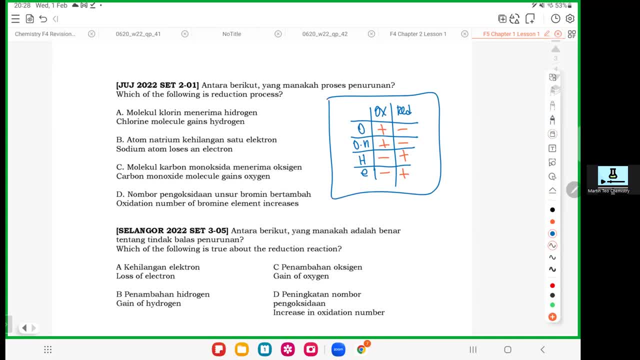 to refer to this table by today. okay, for today, this table i will give you. but in today, this table i will give you. but in today, this table i will give you, but in another one or two more lessons. you need. another one or two more lessons you need. 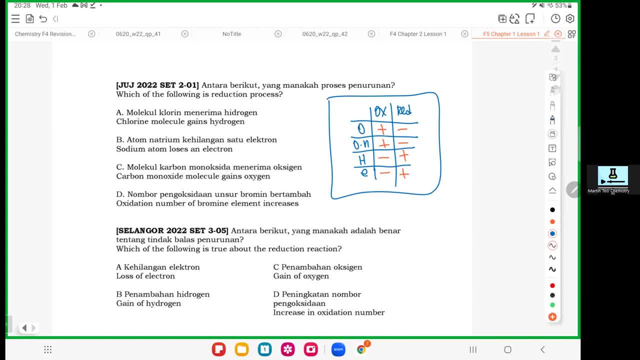 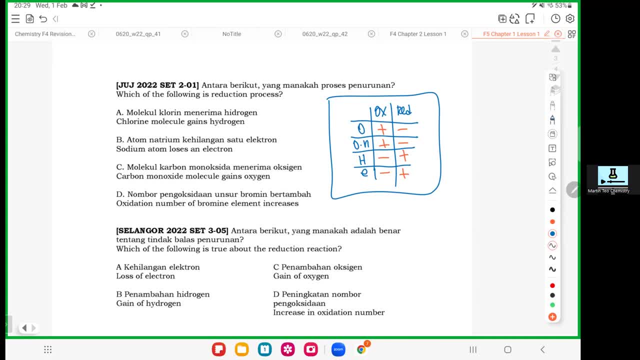 response: so far fantastic guys. response: so far fantastic guys. a and b are a and b are All right, fantastic. So just refer to the table: gain: hydrogen, Hydrogen gain reduction. that's what they want. Okay, so the second one: it's reduction also. 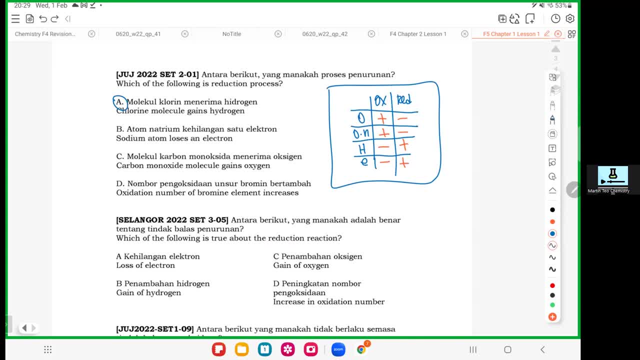 So reduction. so let's focus on this role. So what they do is that gain hydrogen. okay. So reduction, hydrogen plus plus means gain. So it is very, very straightforward, okay, If you understand this table. 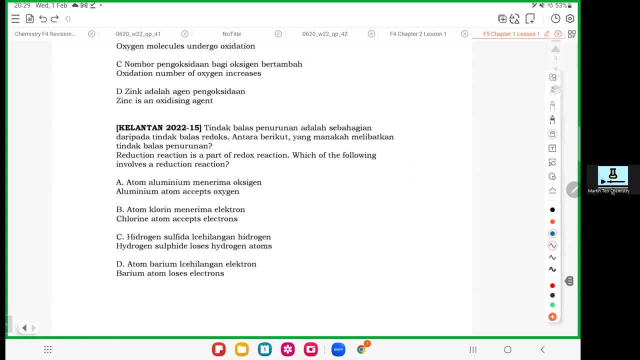 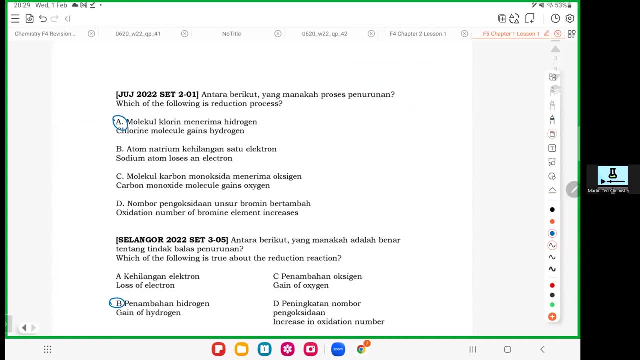 if you understand this table, everything will be easy for you, okay, Everything will be easy for you, okay. So that's the first thing that we learned today. Okay, come on, let's move on and learn something new. So this is first part for today, okay. 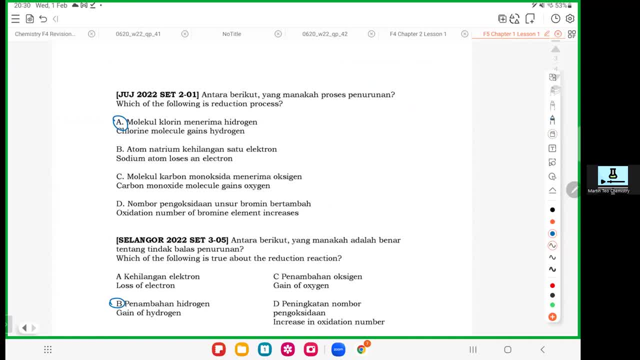 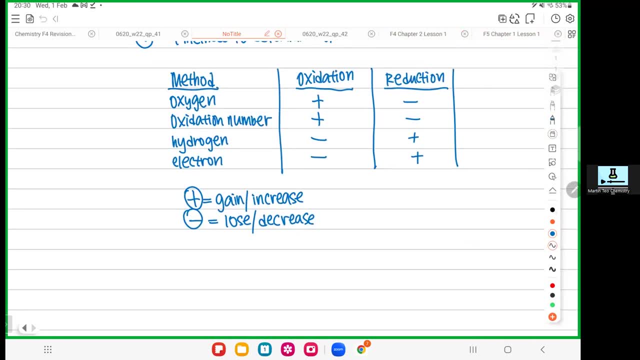 So the second part for today, the second part that we need to learn today, is this: okay, Let me move you back. Okay, so the second thing you need to know is this: okay, All right, so now, today, I'll teach you. 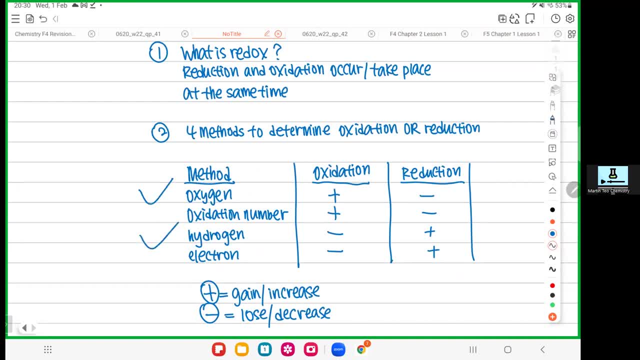 probably two methods: oxygen and hydrogen. If we got time, then I teach you oxidation number method as well. So we see this four method. this one is easy, this one is easy, this one is hard and this one is hard okay. 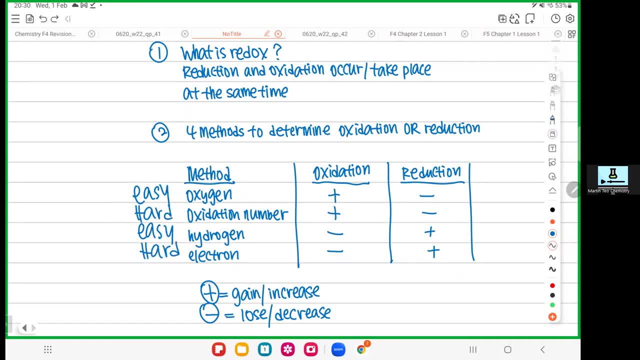 So in chemistry you see, this is the one easy, easy and hard, hard huh. So SPM normally will ask you the hard one, the easy one. they seldom ask, all right, But we have to start from the easy one. 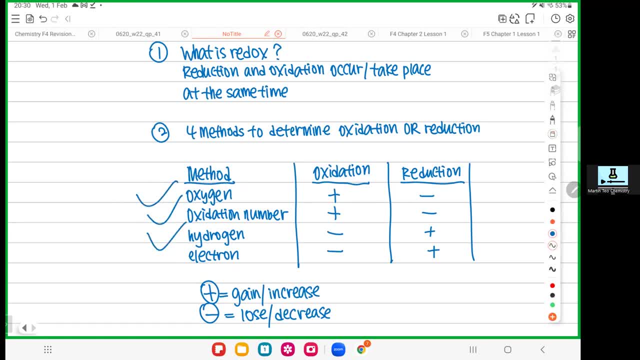 So today I'll teach you these two method first, If we got time, we learn this method as well. okay, One by one. we learn slowly. no rush, We are not rushing. okay, First lesson is always the most okay. 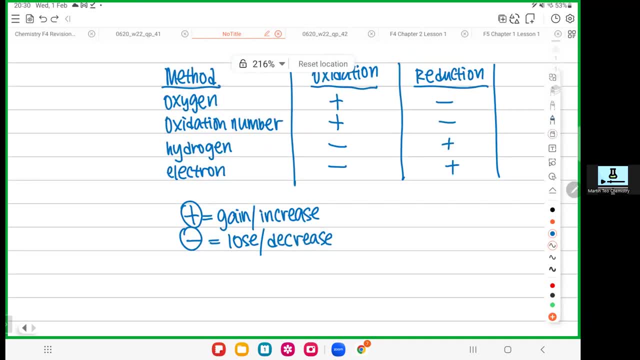 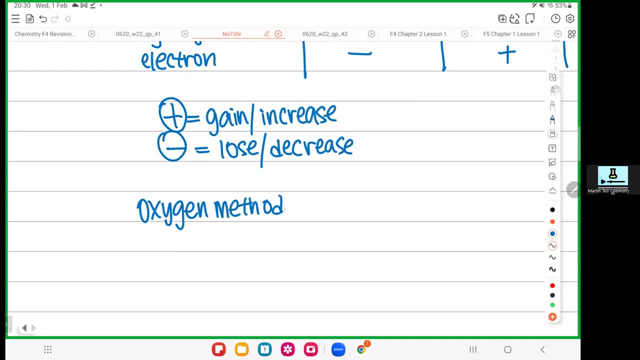 Okay, so let's go. I do super slow so that you all can follow me. Okay, let's start with the first one. huh, Come on. The first method is called oxygen method. okay, So listen carefully. So if you guys understand oxygen method, 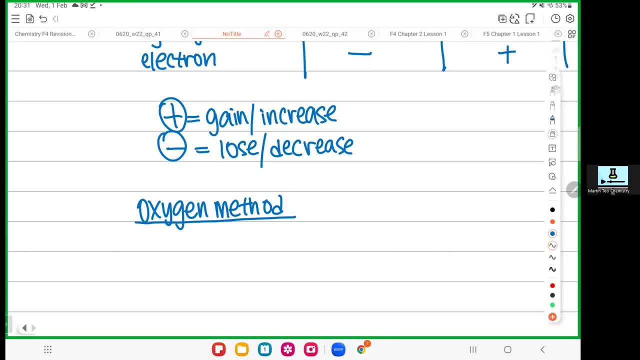 then the remaining part will be easy. okay, Because many, many method. they are very similar one. There are many method actually. they are very, very similar one. So if you understand the first method, the other method would be quite 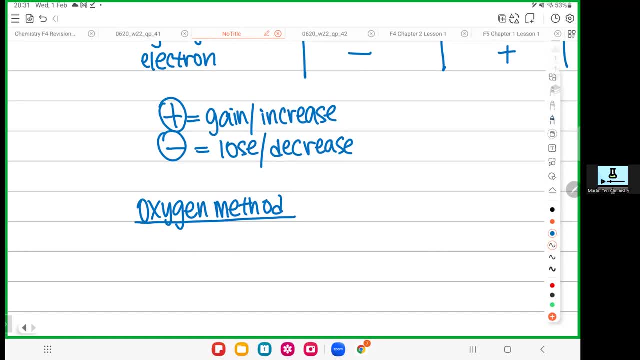 quite easy for you, okay, So let's start with it. huh, So for oxygen method. so what we need to do, okay, How to do oxygen method and what is it. okay, So let me show you now. okay. 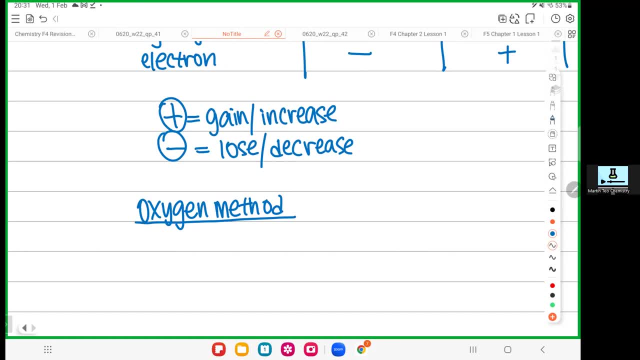 So if you want to do the oxygen method, okay, First of all you need to understand a very important thing. We call it as apple to apple comparison. okay, We need to do a very important thing called apple to apple comparison. okay. 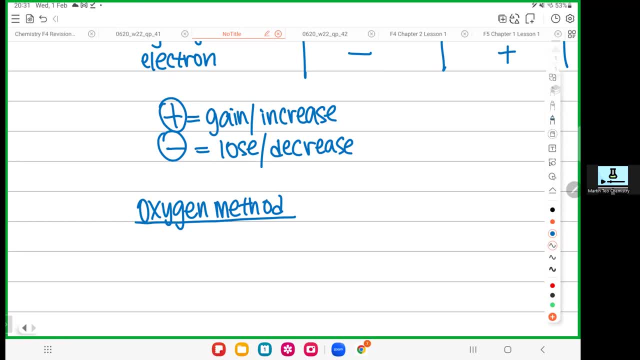 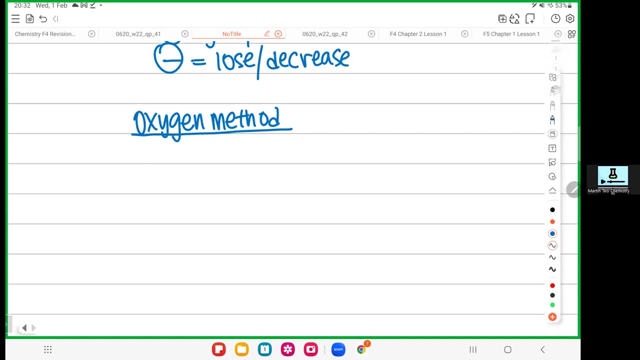 So what do we mean by apple to apple comparison? Okay, so let me show you something first. huh, Let me show you something first. okay, All right Here. Okay, So oxygen method: we only focus on oxygen. So we only focus on whether we gain or lose. 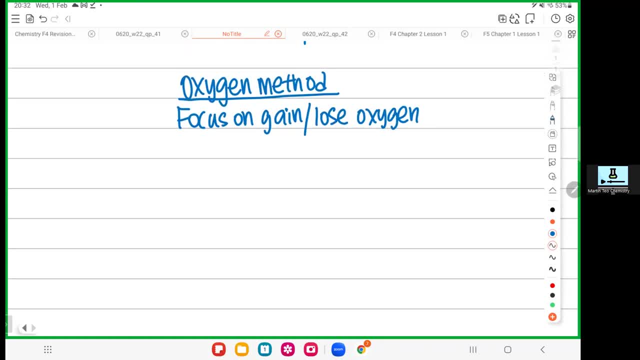 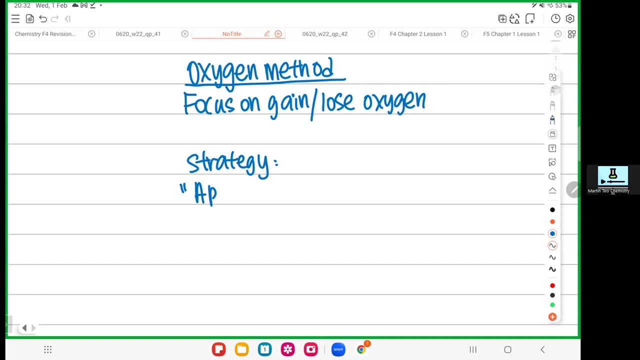 Oxygen. okay, We don't look at other things. okay, So what is the strategy that you need to use? Okay, this strategy can use for any other method. We call it apple to apple comparison. Okay, what do we mean by apple to apple comparison? 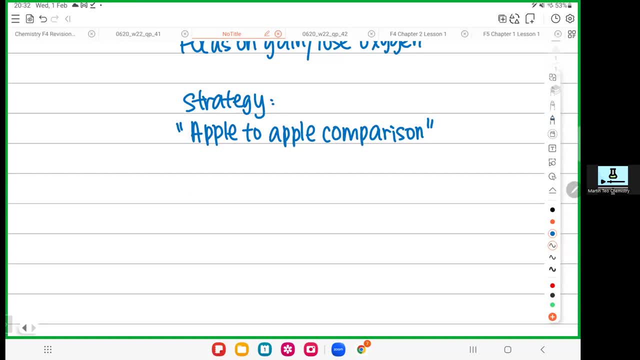 Okay, listen carefully. Yeah, So when you do apple to apple comparison, you must always, always choose the right person to compare. Okay, you must always compare the right apple. You cannot take apple compared with durian. You cannot take apple compared to rambutan. 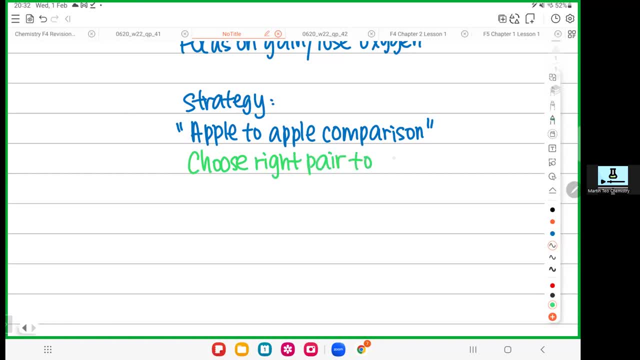 So how to choose the right apple, Okay. how to choose the right pair to compare, Okay. so listen carefully. So there are three things you need to do here. First thing: you always need to choose one fellow from the left, And then you always choose one from the right. 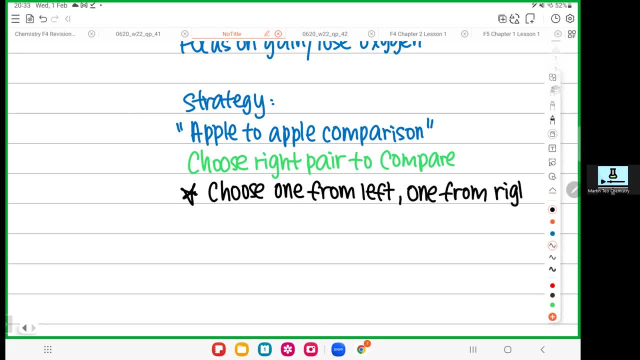 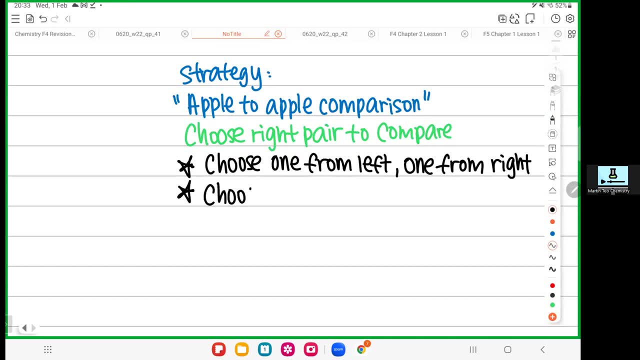 So must be one left and one right. You cannot choose two from the left. You cannot choose two from the right. Must be one from the left, one from the right, Okay, Okay. so you must always choose something that is related. 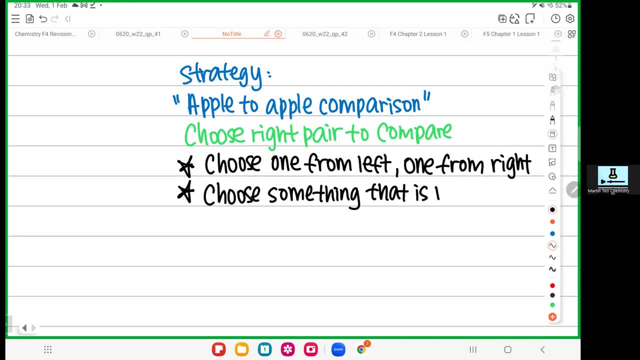 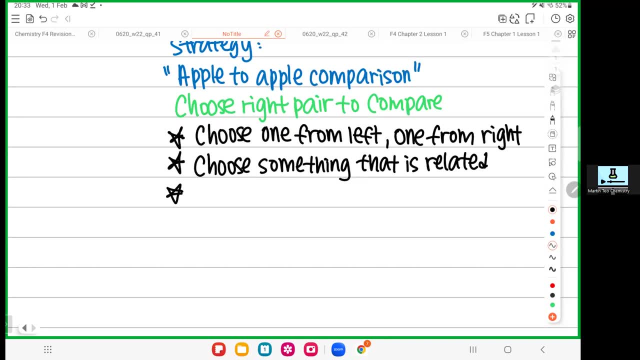 Choose something that is related. No worry, later I'll use two to three examples to show you, So you will have a better idea. Okay, so then you have to be careful with the sequence. Okay, so you have to be very, very careful with the sequence that we are doing. 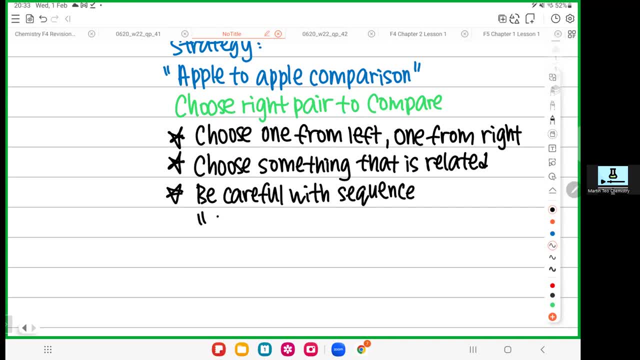 When you're doing the comparison is always left, go to the right. You cannot the balik. You cannot go the other way around. You cannot compare right to the left. Okay, what do I mean? Okay, the best way to learn is by example. 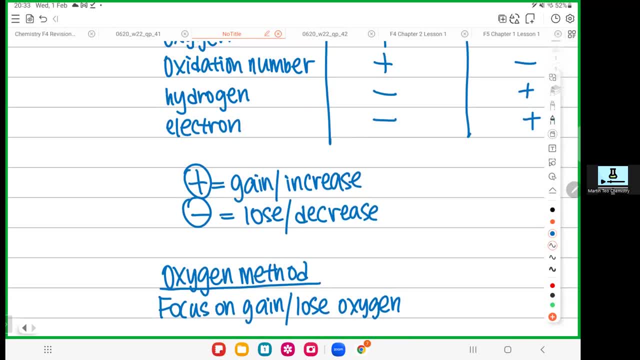 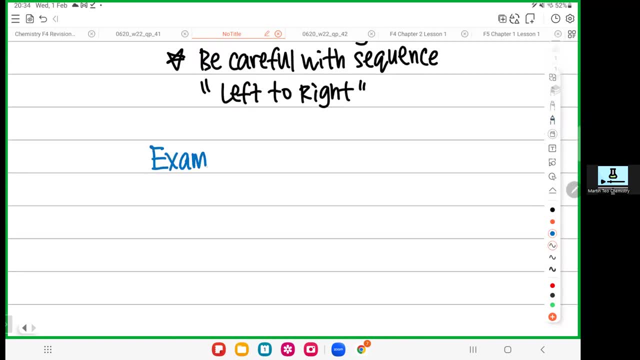 I will use three examples to show you so that you have a better idea. So if, after three examples, you still very blur, please ask me. Okay, so the first example. let me teach you this. So the first example. we have something like this: 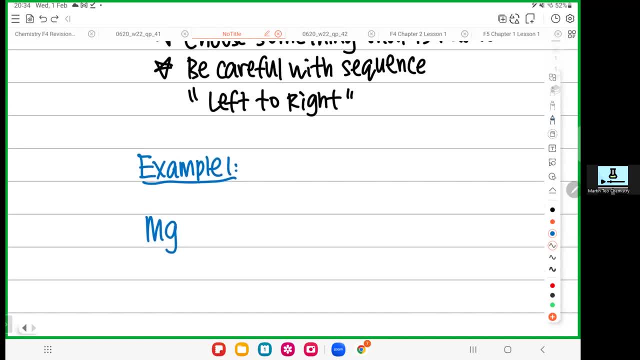 This is a magnesium and then this is a copper oxide. This is magnesium oxide And this is a copper. Okay, All right. So how are we going to use oxygen method to do this question? So first of all, look at the step. 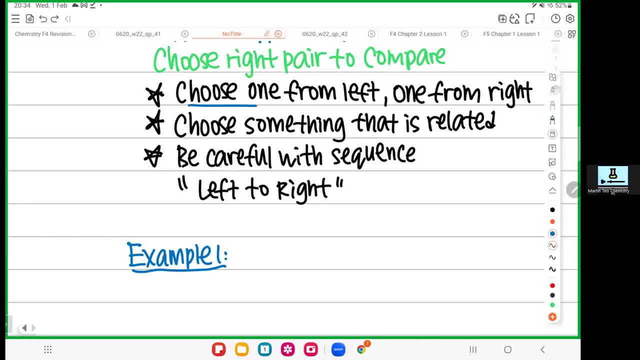 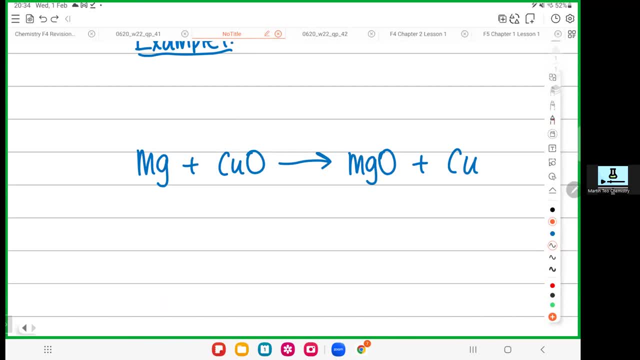 First go to choose the right. one fellow from the left and one fellow from the right. Choose something that is related. Okay, let's say I choose one Apple from the left. The first Apple I choose is magnesium. So can I choose copper oxide already? 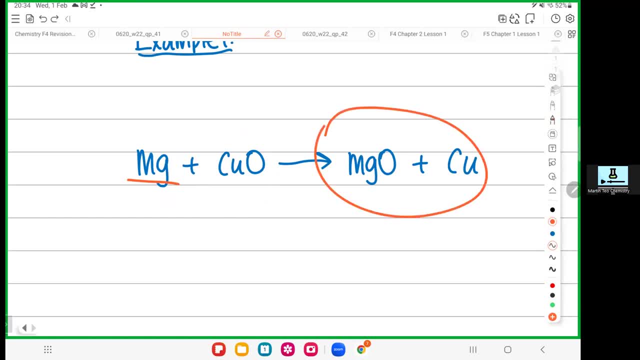 Cannot. You must choose one Apple from the left and one Apple from the right. So now the right Hand side got two apples. right, The right hand side got two apples. Which Apple we should choose? They must be related to the left. 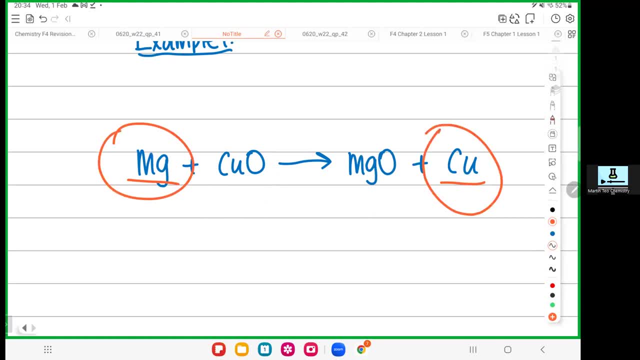 Can we choose copper, Cannot Magnesium, and copper has nothing related, No common thing, Nothing related at all. Magnesium, copper, totally different. You will choose magnesium oxide, Why They got relationship. This is magnesium, This is magnesium oxide. 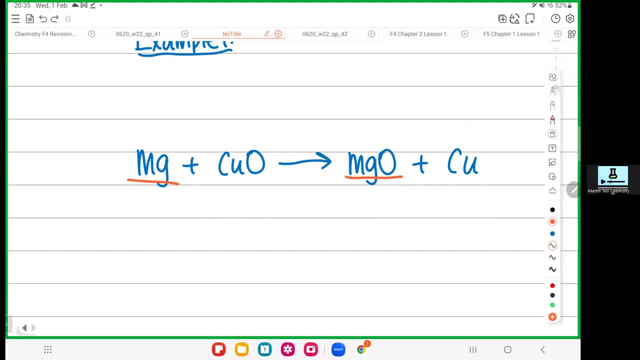 Both of them got MG, So at least you can see they are related. Okay, So these are the Apple that you want to compare. Let me know in the chat box: Are you okay so far? Okay, Always choose the right pairing for comparison. 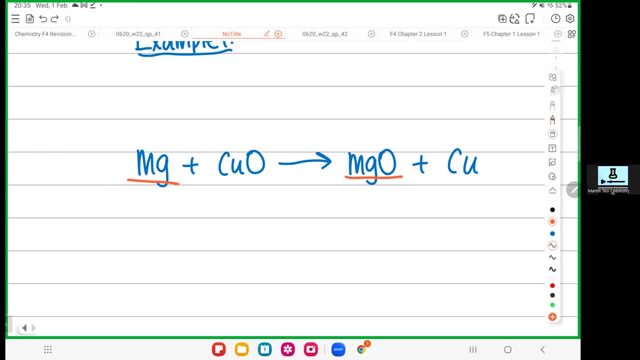 So can we do a comparison now? Yes, Let's look at it. Let's look at the right color arrow. Would you compare? always left to the right, Not right to the left. So let's say now, I compare the left to the right. 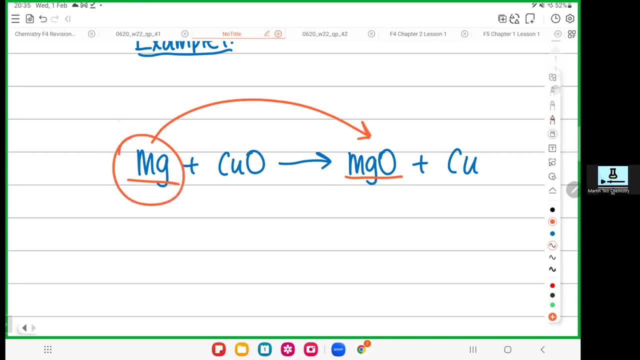 So left to the right, What you can see on the left hand side, Magnesium is alone. on the right hand side, Magnesium sticking with oxygen: here Magnesium, but other oxygen, here The magnesium, other oxygen. So from no oxygen become got oxygen. 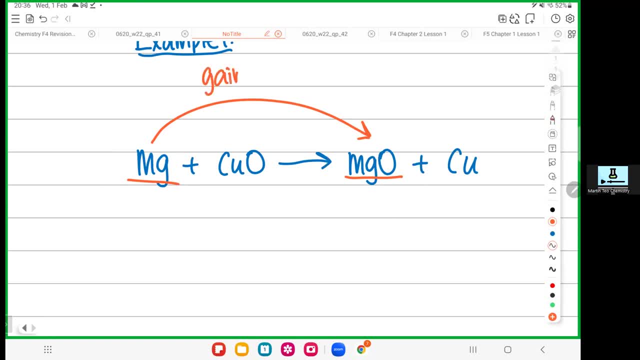 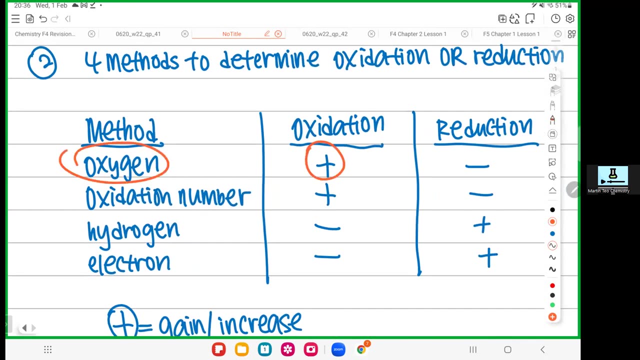 What happened? Gain oxygen. Okay, So now you can see already: magnesium gain oxygen. So magnesium increase oxygen. So, as what we learned today, the four different methods, So when I gain oxygen, what process that is happening? Oxidation- 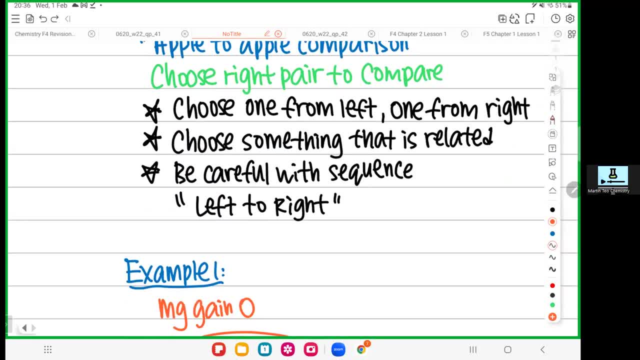 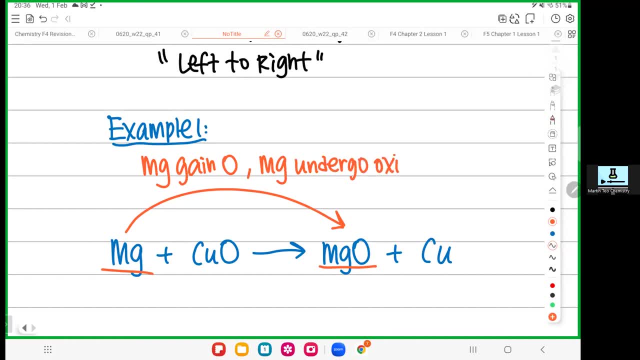 Okay, So magnesium undergo oxidation. So magnesium undergo oxidation. If you don't want to say magnesium undergo oxidation, you can put a past tense like this. You can also write: magnesium is oxidized. Make it a past tense. Same meaning: Magnesium is oxidized. 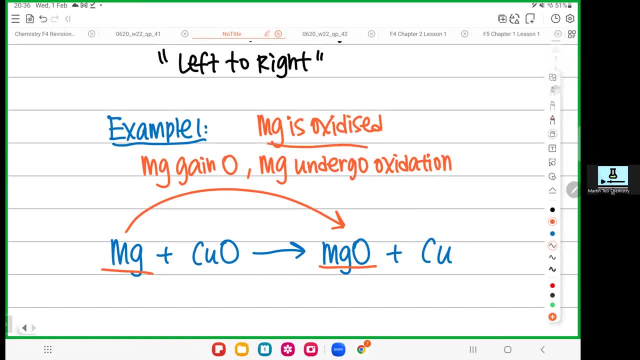 Okay, Magnesium Suda undergo oxidation. Same meaning. what So you can write either way. You can write the first one or you can write the second one, up to you. Okay, So magnesium undergo oxidation already. Okay, Now let's choose the second Apple to do comparison. 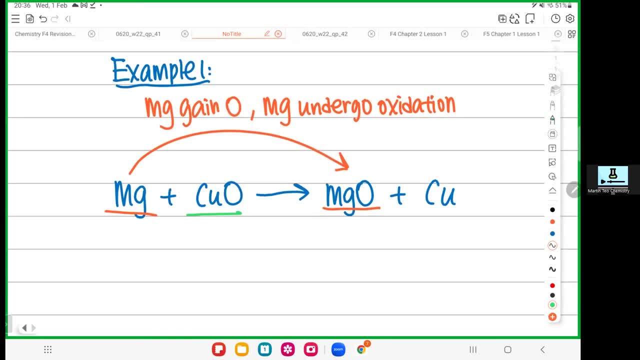 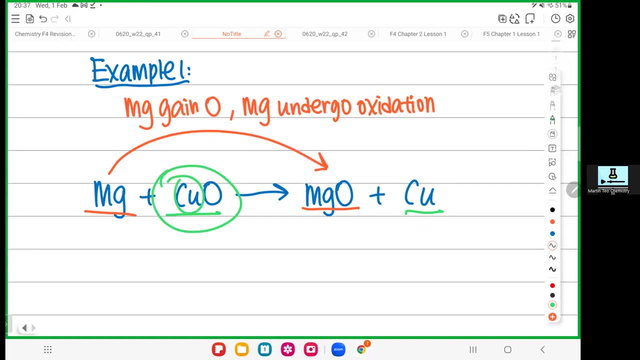 So now the second Apple is copper oxide. So now, compared to another Apple, this one, copper oxide and copper, they are related, right? Why? This fellow got seal, This fellow got seal, So they are related. So from here to here, remember left compared to the right. 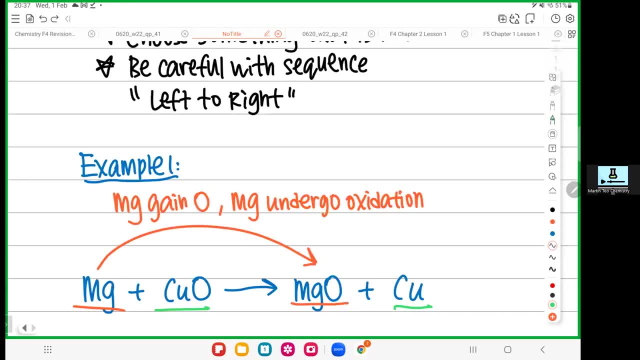 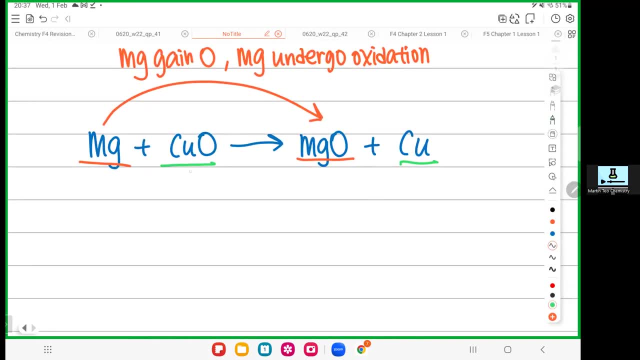 not the right compared to the left. The sequence is important. The sequence is very important. Left to the right. So left hand side Apple compared to the right hand side Apple. So what you can see on the left hand side, the copper got oxygen. 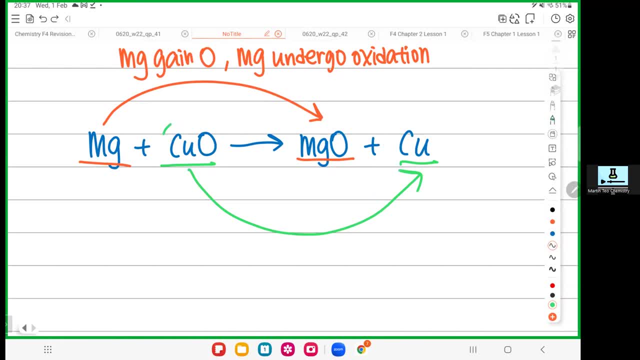 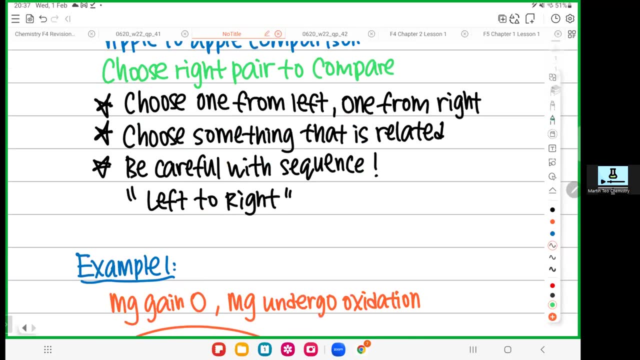 On the right hand side, copper, don't have oxygen. So what happened? This fellow copper oxide lose oxygen. So when you lose oxygen, what happens? So that's what we learn: Oxygen If you lose it. So it is reduction process. 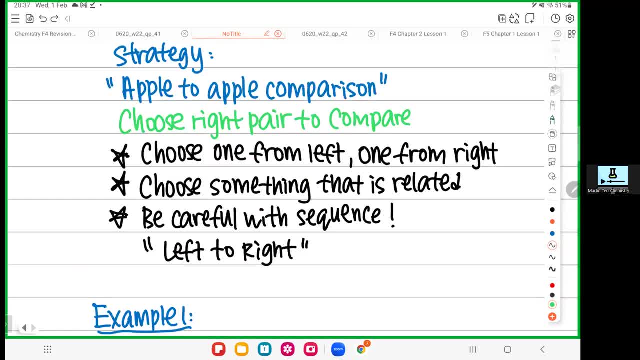 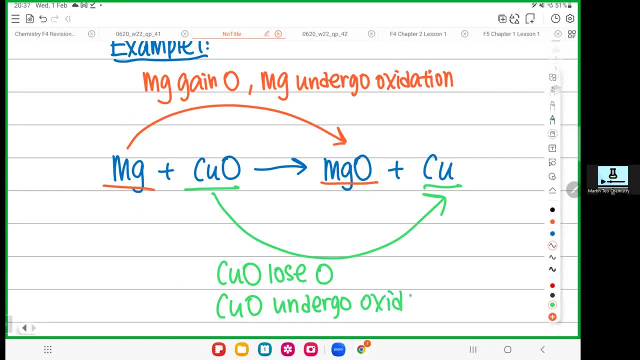 So it's reduction process. So you can say that this fellow copper oxide lose oxygen, copper oxide undergo reduction. If you don't want to say the word undergo reduction, I read wrongly. Sorry guys, my bad, My bad. You can say undergo reduction. 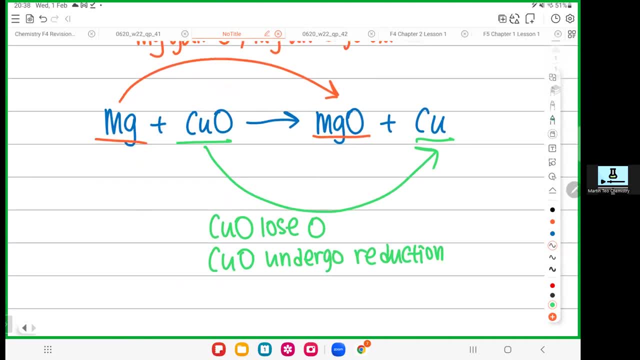 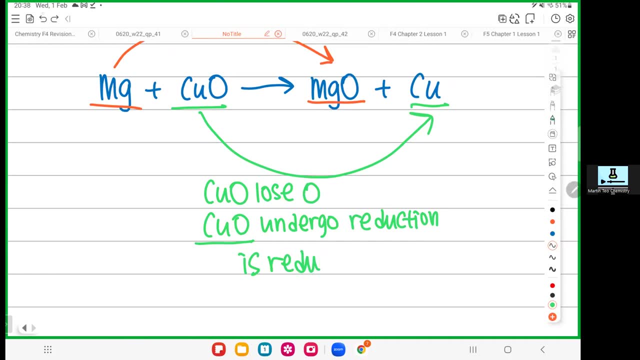 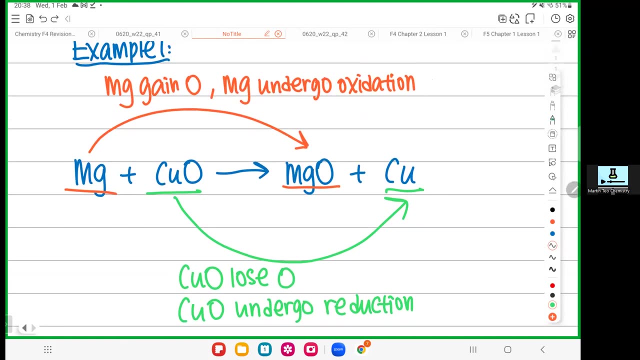 If you don't want to say undergo reduction, you also can use a past tense: Copper oxide is reduced Suda undergo reduction also can. So now look at it. So in this chemical reaction you have oxidation. In this chemical reaction you also got reduction. 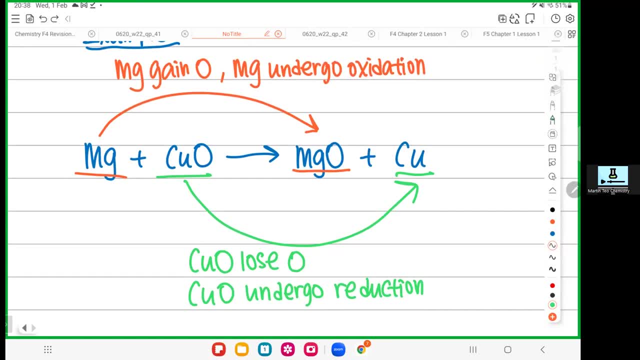 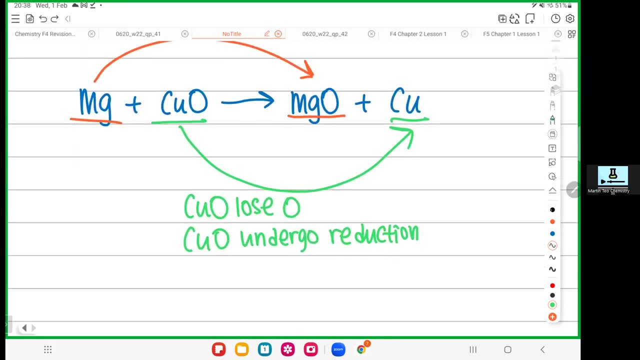 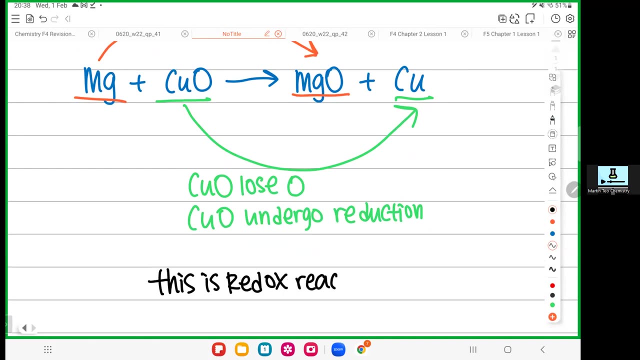 So when oxidation and reduction, these two process, happen at the same time, this whole chemical reaction is a redox. So this is redox reaction. So guys up to this point is it okay so far, So it's not very hard. 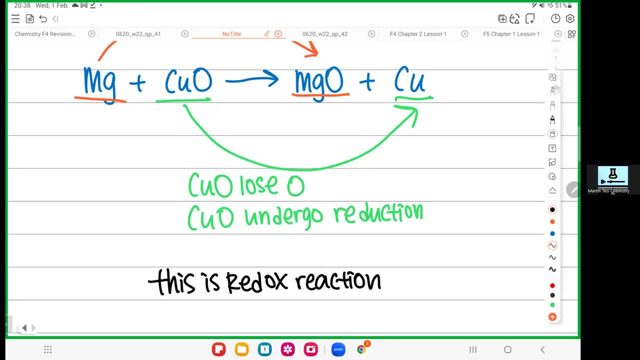 Like what I say. you just need to make sure you choose the right Apple. If you choose the right Apple, you do the right comparison. Everything is easy. Everything is easy if you're able to do this, Okay, All right, Not very hard one, but it all begin with choosing the right Apple. 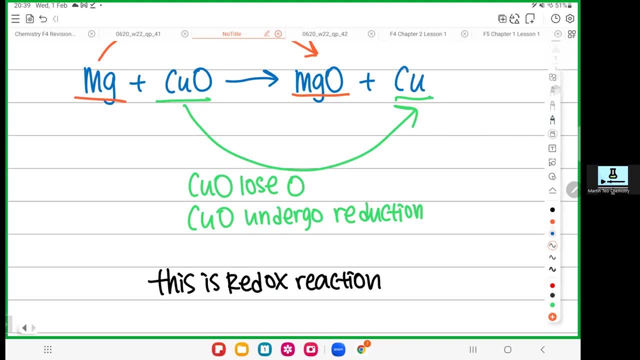 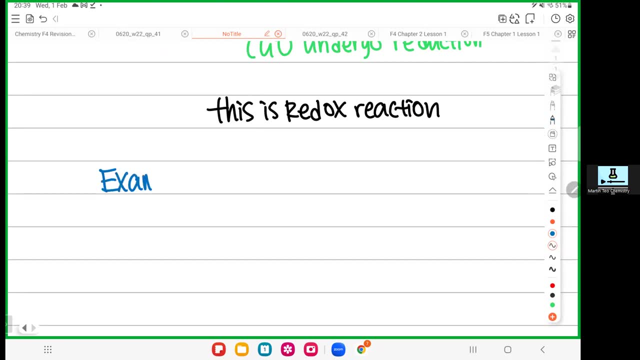 It's all begin with choosing the right Apple first. Okay, so we're done. Come on, So let's do a few more. Let's do another few more. Example number two: Okay, Later I would like you all to try. 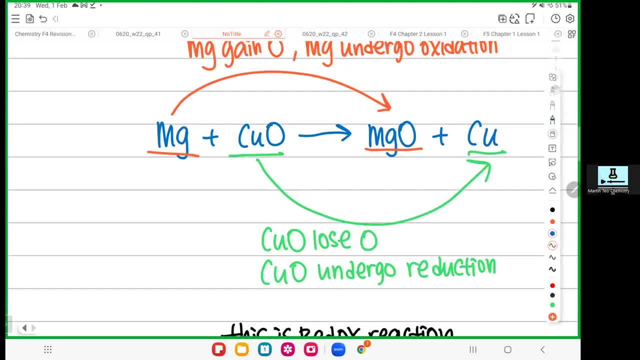 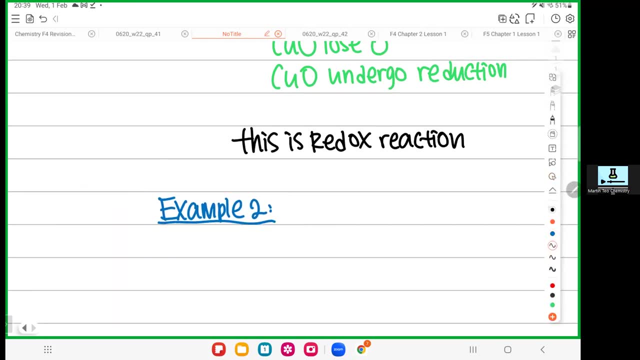 Later. I would like you all to try some questions later, But now just follow my footstep. Let me guide you first. Let me guide you step by step. Okay, Example number two. Okay, So let's say I go for another example. 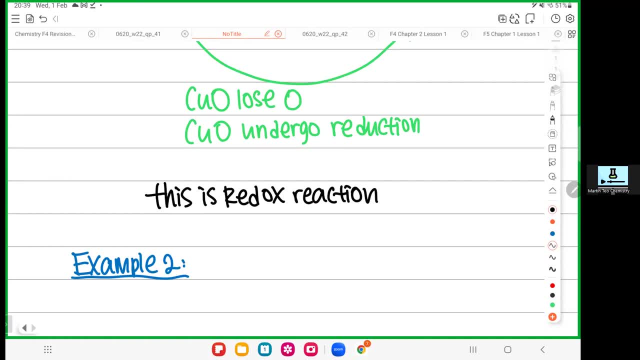 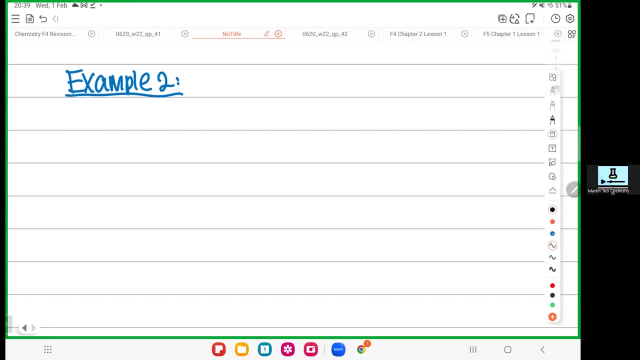 It looks like this: Okay, All right, Here we have. let me read like this: Okay, He be all two. Sorry, He be all two plus C, become he be all plus CO. Okay, Same thing. We are now still focused in oxygen method. 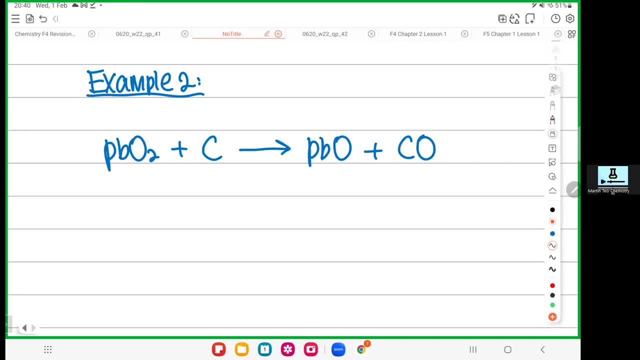 Other method. Don't bother, Don't bother yet. So let's choose the first Apple. So the first Apple I choose is what? This one? One Apple from the left. So we choose one Apple from the left. You need to choose another one Apple on the right. 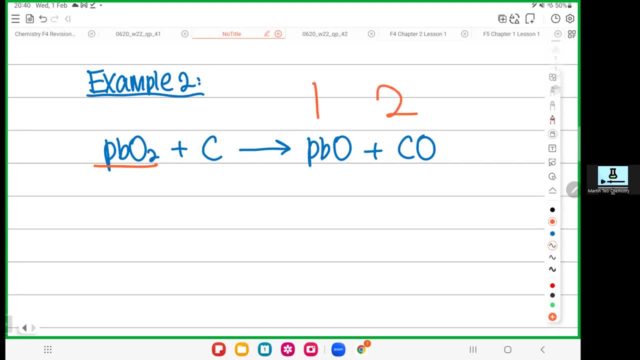 So among these two Apple on the right, you will choose the first or the second one to compare. Guys, you choose the first or second one to compare with the Apple. Okay, Very good, You choose the first one, right, Because at least you see something related, right? 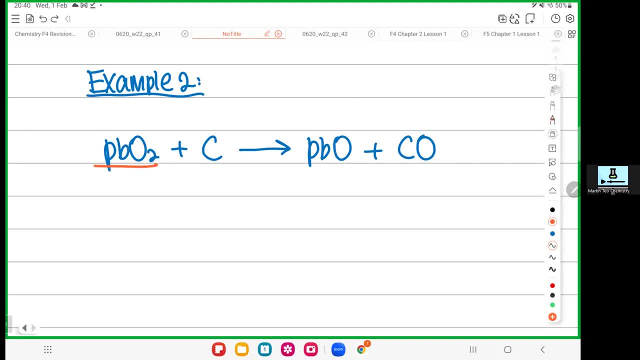 Throw. not Okay, This fellow got PB, This fellow got PB. You can see they got relationship, They got relationship. So that's it. So compare left to the right, Left hand side. The PB got Two oxygen right hand side. 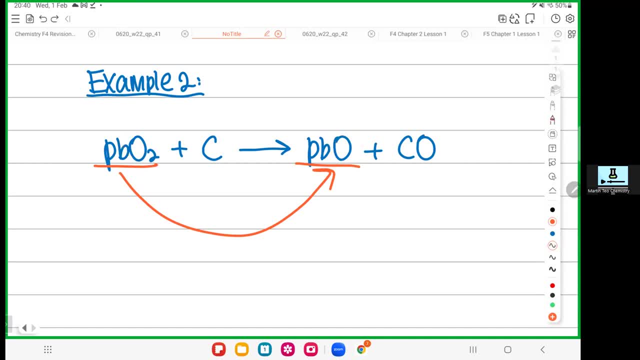 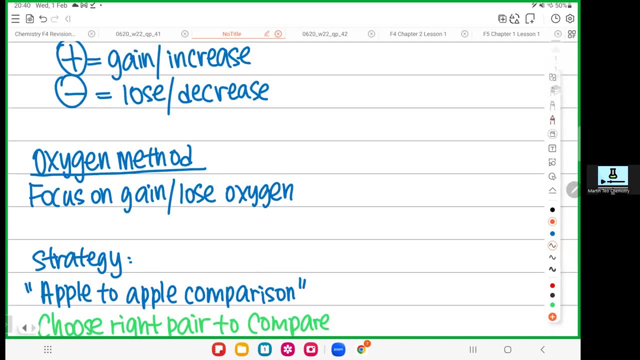 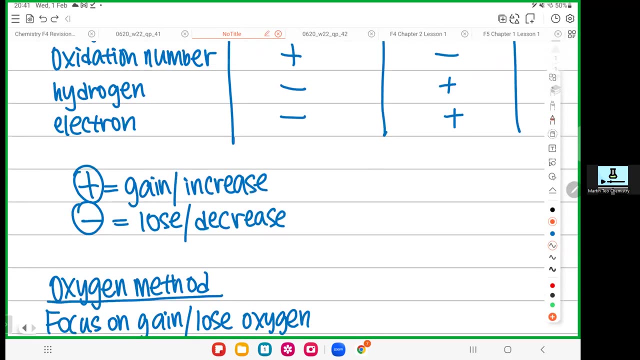 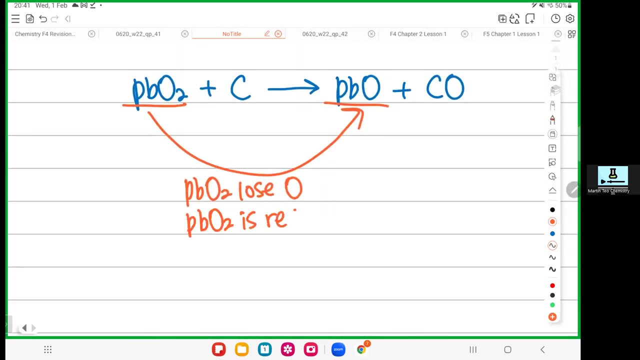 The PB got one oxygen. Two become one oxygen become lesser, So lose oxygen. Pb O2 loses oxygen. So that's what we learn today: When we lose oxygen, the process is reduction process. The process, it is reduction process. So reduction of Pb O2 undergo reduction or you can say is reduced. 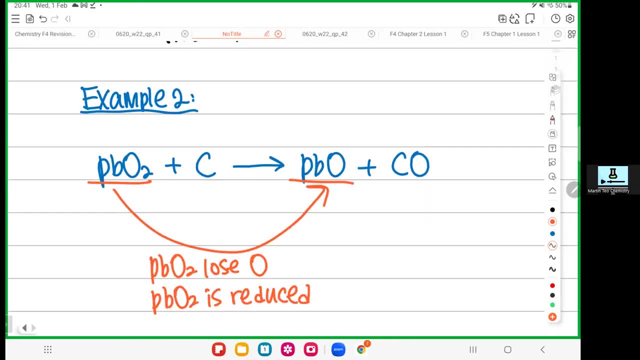 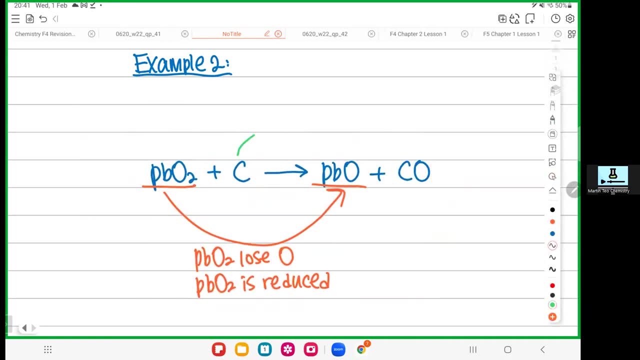 Let's say I use the past tense- settle. So now let's choose the next Apple to do the comparison. So the next Apple that we want to do the comparison is here. Carbon is another Apple compared with CO. So these two are related, right? 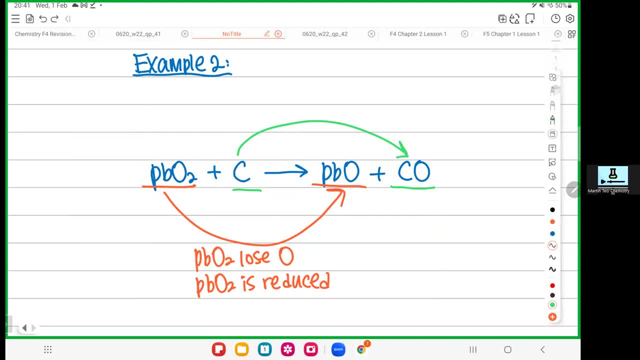 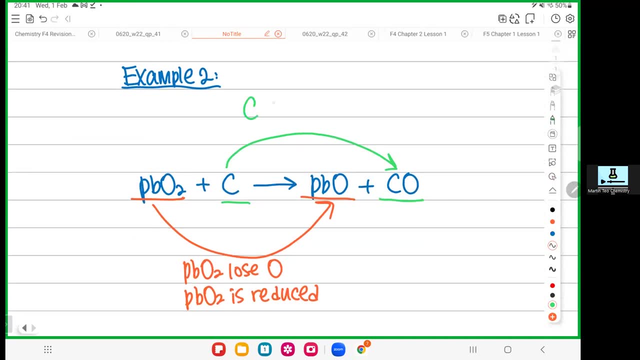 You got C. You got C. So on the left hand side the carbon come alone, On the right hand side the carbon sticking with O. So no, O got O. So increase in oxygen for the carbon, gain oxygen. So when you gain oxygen you undergo oxidation. 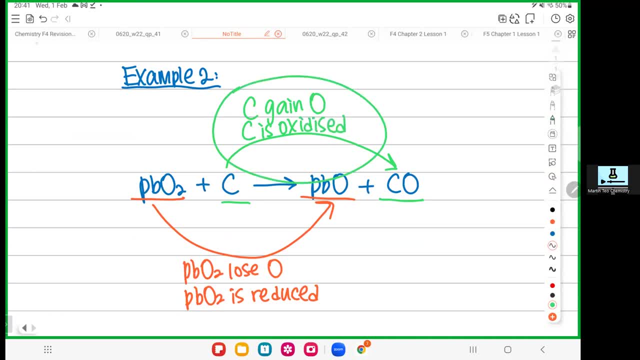 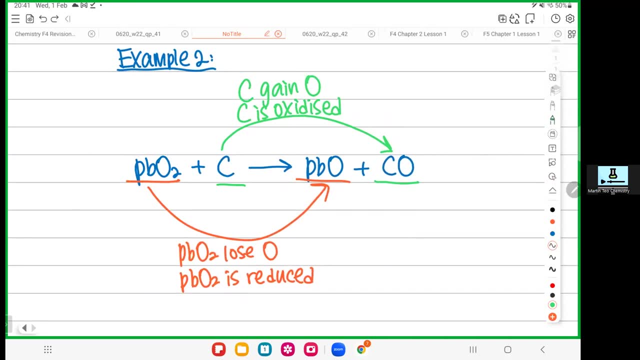 You can say: undergo oxidation, Or you can say: is oxidized. So this chemical process, is it a redox? Guys, is this a redox process, Yes or no? Is this chemical process a redox, Yes or no? Yes, Right, 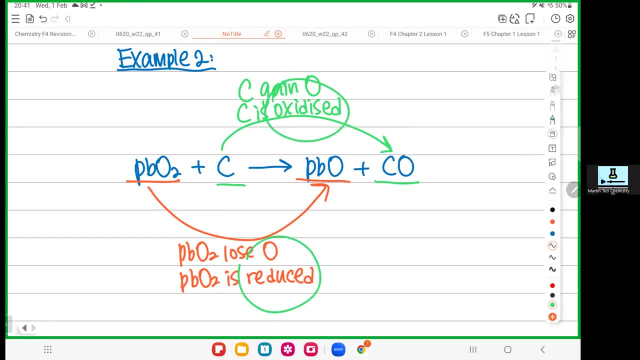 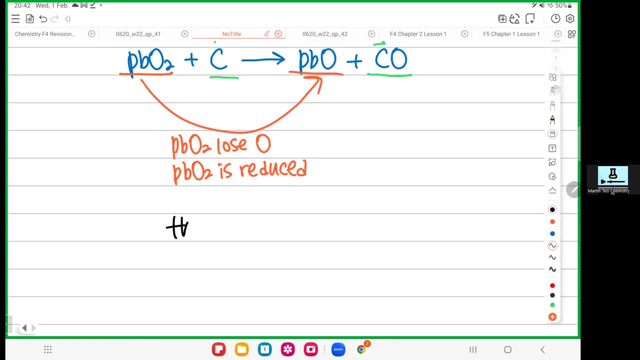 Because ada oxidation, ada reduction. When you have oxidation, you have reduction. These two process happen at the same time. Yes, it is redox. Yes, Okay, so settle So it is redox, So done. Okay, So I don't think very hard, right. 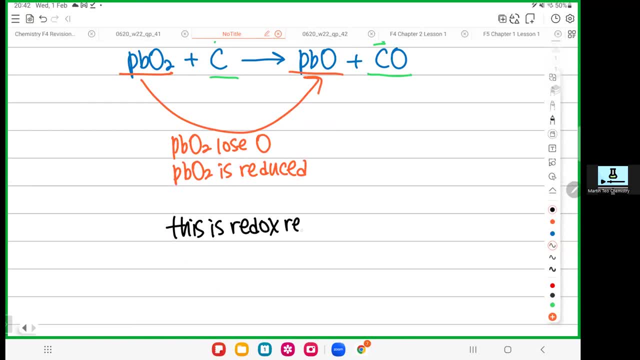 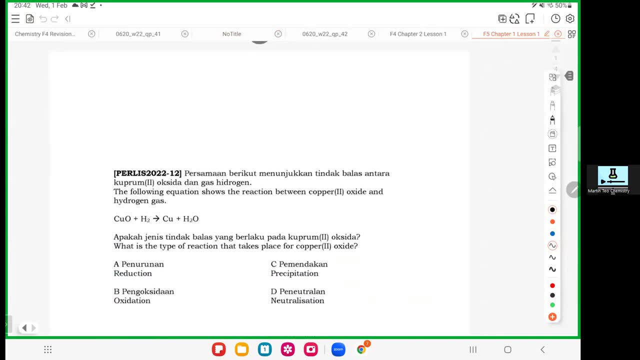 So, as long as you understand the logic, as long as you understand the logic, you are good to go. Okay, you are good to go. It's not very hard, actually. Okay, Right, So now let's look at here. 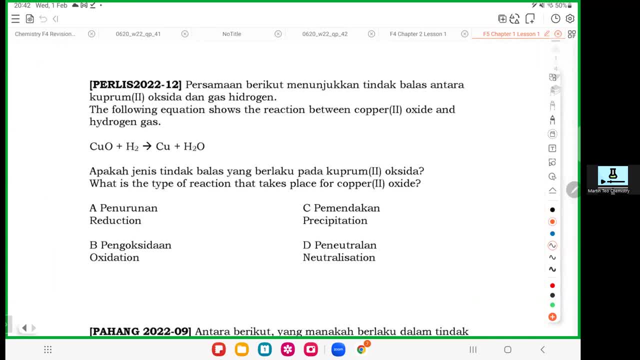 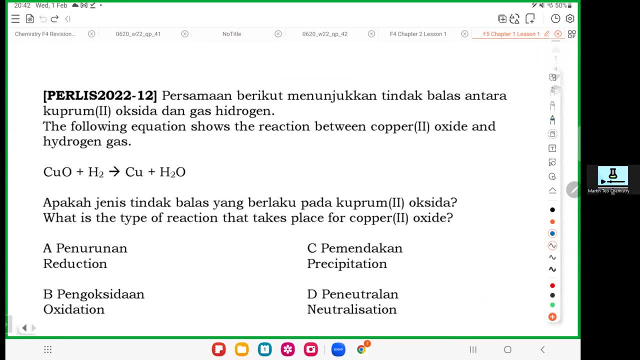 Let's look at one past year question. So no past year State paper. Let's do one state paper. This question is from 2022. police trial exam paper: Soalan per cubaan police. So they give you this Chemical equation. 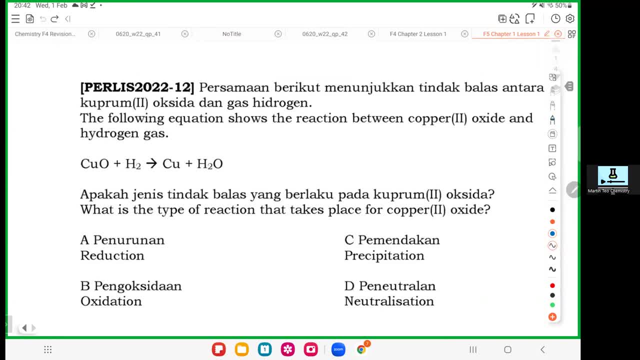 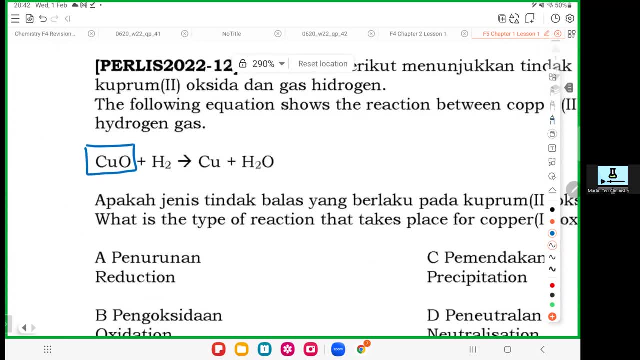 They give you this chemical equation, They ask: what is the reaction? happen on copper oxide. So copper oxide is this fella. So when you want to know what happened, you must choose the right Apple for the copper oxide compared with the Apple. 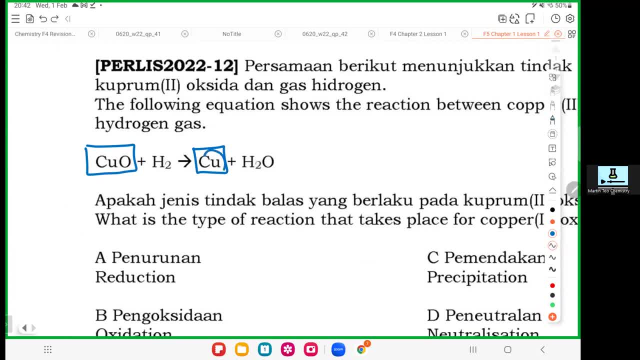 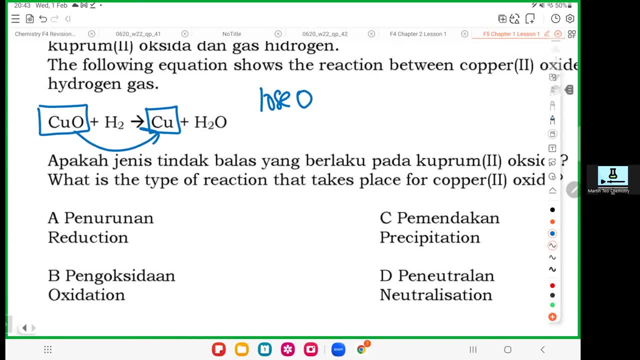 Copper left hand side: This copper got old. right hand side: This copper don't have old. So what happened here? Loose oxygen. So loose oxygen is what process. anyone can type in the chat box to let me know Loose oxygen is what process. 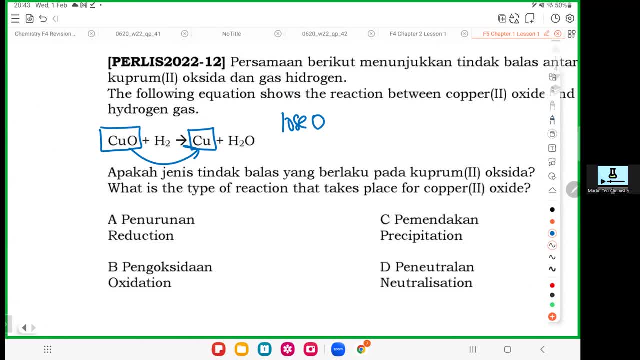 Okay, fantastic. Loose oxygen is reduction, So the best answer is quite easy, isn't it? Okay, that's exactly how the question can be tested in the real exam. Is that easy? Only choose the right Apple, Do the right comparison. 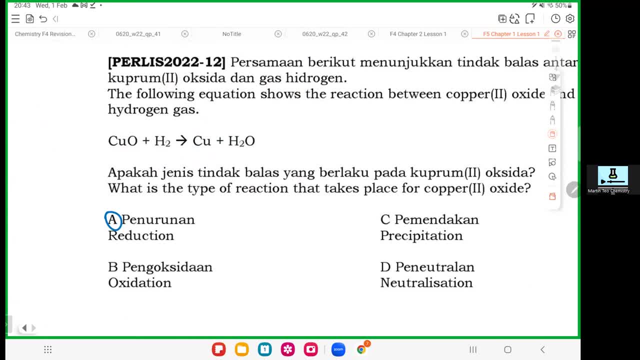 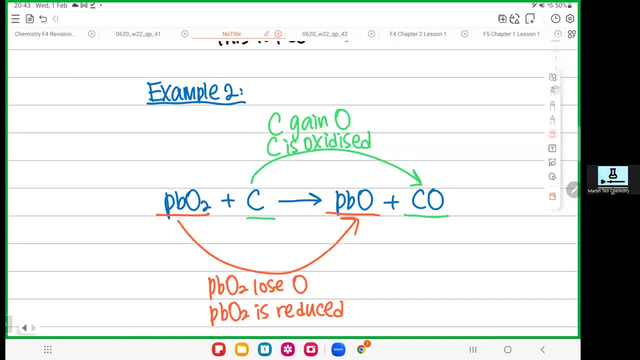 You are good to go, As simple as that. Okay, that's it. Okay, now let us increase the difficulty. Let us increase the difficulty A little bit more. Okay, when you come to chemistry, another very important words is this: 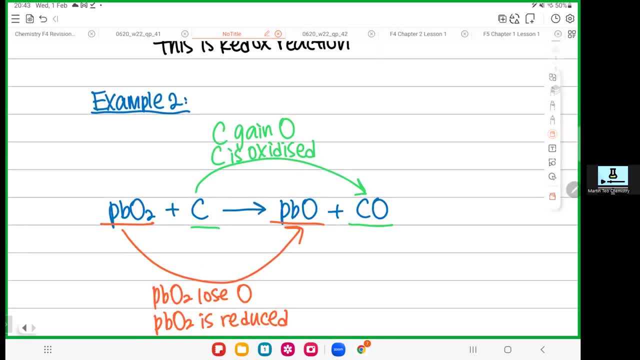 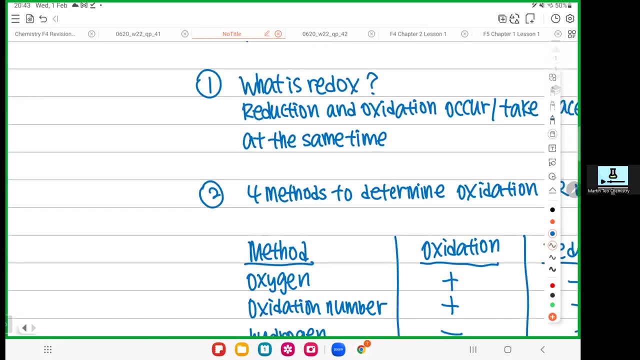 In chemistry you will see this one, these important words, This one might be a bit confusing, So I'm going to go very, very slow to make sure that you really can get the idea. I'm going to go very slow to make sure you can get the idea. 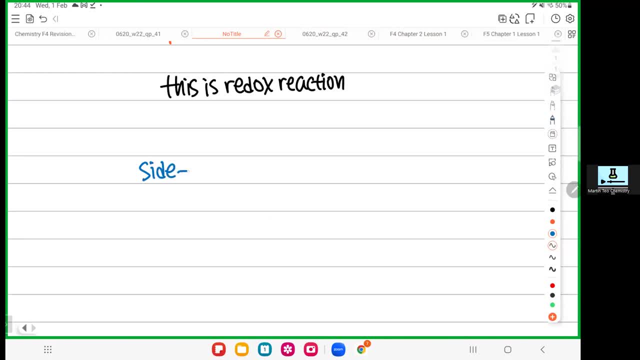 Okay, so listen carefully. So this is the side notes. Okay. so in chemistry, okay so we have some super agent, We have some special agent. Okay. so you see, when you watch some super hero, you watch some movie. 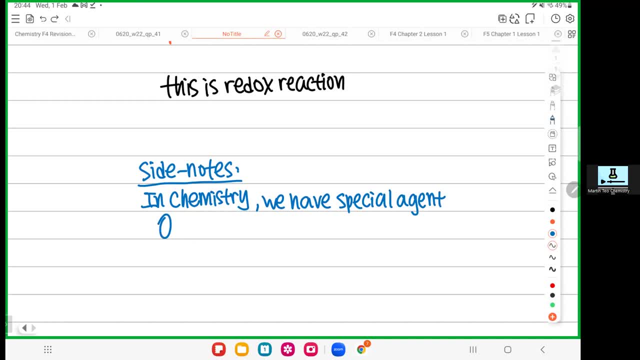 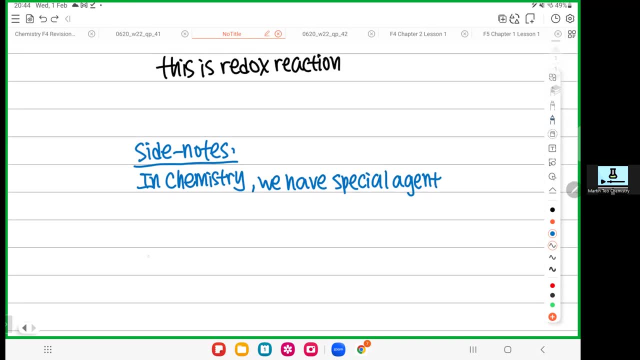 Okay, you can have 007.. Those like secretive agent, isn't it? So chemistry also got some secretive agent. Okay, so you have two agents. Listen carefully. The first agent called oxidizing agent. The second agent is called reducing agent. 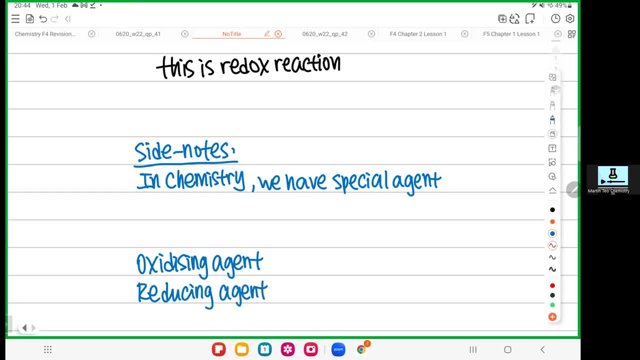 What do we mean by oxidizing agent and reducing agent? Oxidizing agent means what you are, the agent to oxidizing. Oxidizing means you let other people to undergo oxidation, So you go to let other people or other substance to undergo oxidation- you oxidizing. 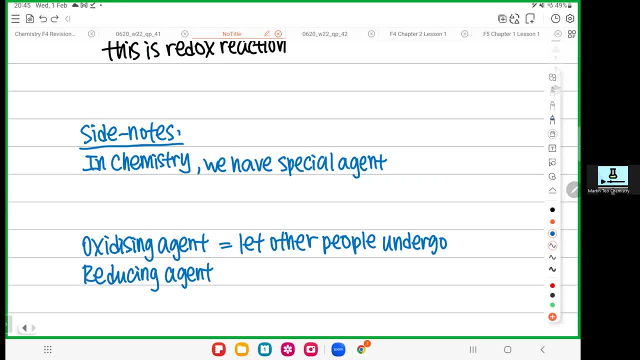 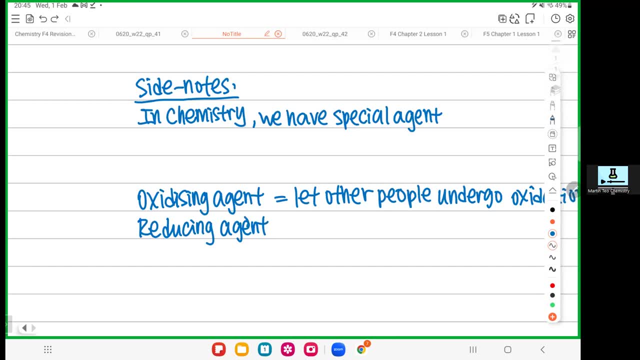 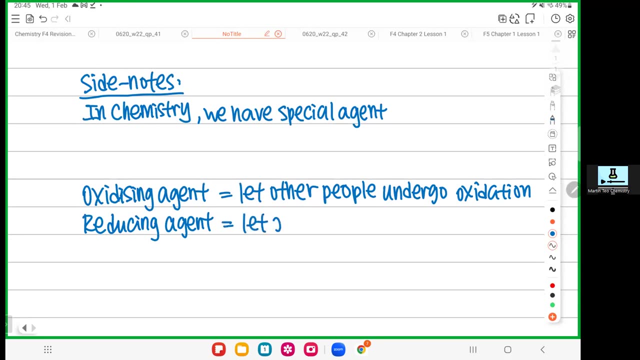 Oxidizing means you let other people to oxidation, undergo oxidation. This will be a bit confused. No worry, I go very, very slow. reducing agent. I am the agent. What I do reducing let other people to undergo reduction, So I go to let other substance undergo reduction. 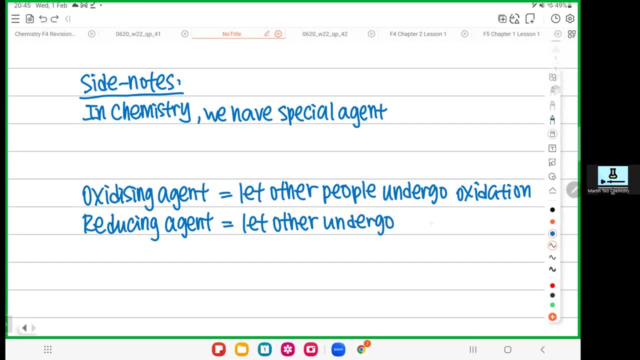 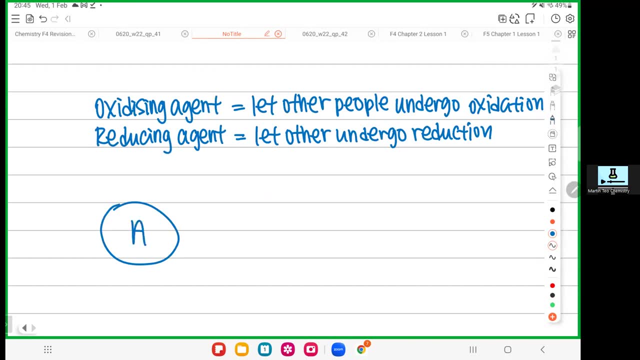 Okay, what do I mean? Okay, you see. So everyone, take a look on this today. This is substance A, or this is me. This is me. You mix me with oxidizing agent. You mix me with a fellow. This fellow is called oxidizing agent. 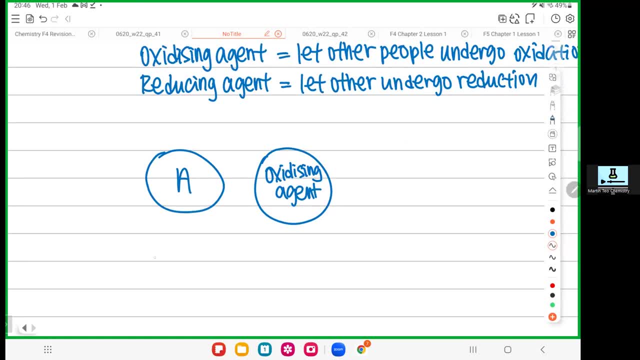 Okay, some people say it's Mr Martin. Why Sometimes in the books I saw they write oxidizing agent. Some they write Oxidizing agent the S and the Z, It doesn't matter. This has nothing to do with chemistry. 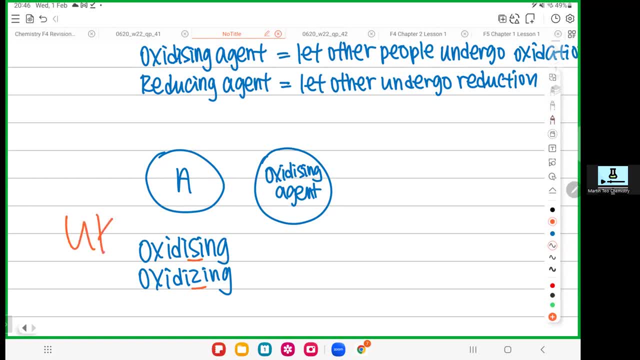 This has something to do with English. Whether you are learning the UK English or you're doing the US American English, It's okay. One, both also acceptable. It's just English only. No matter you write S or Z, both are okay. 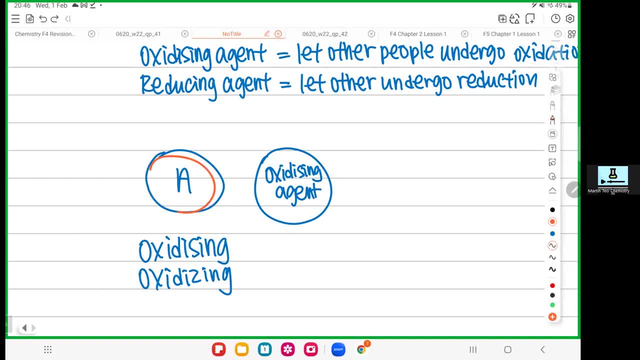 Yeah, So if I am a substance called A, I mix with oxidizing agent. So what happened? Oxidizing agent? what they will do, they will let me undergo Oxidation. So they thought on, the A will undergo oxidation. 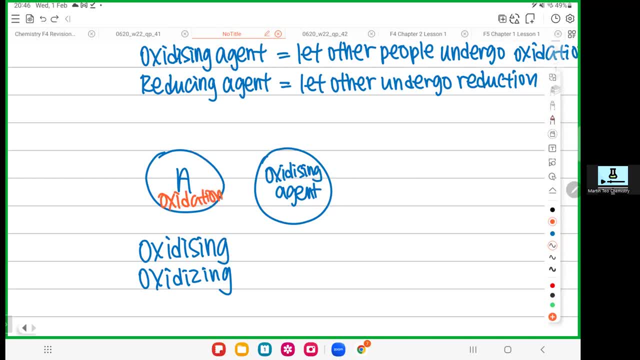 So oxidizing agent, let other people undergo oxidation process. Same thing today If this is a reducing agent. if I mix with reducing agent, reducing agent will make me undergo reduction process. Okay. so when I say agent means what you want to help other people. 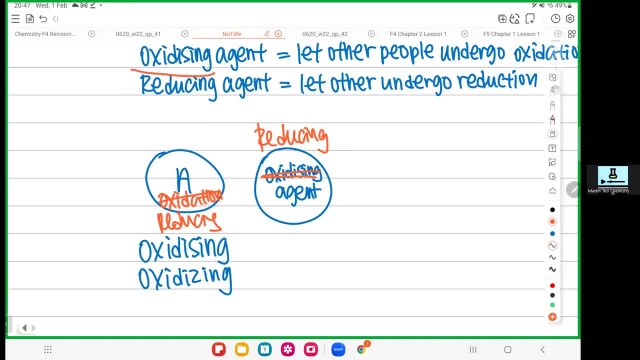 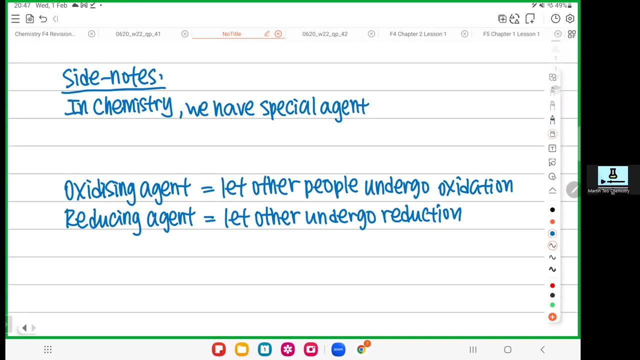 Agent means you want to help other people. Oxidizing agent: you help other people undergo oxidation. Reducing agent: you help other people undergo reduction, Reduction process. Okay, so this is something very important. Now the next thing: how on earth we can know the substance? 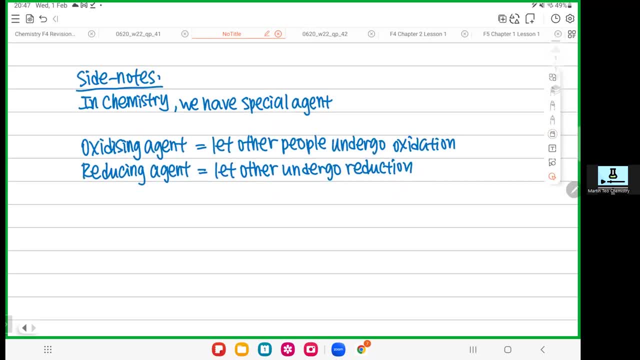 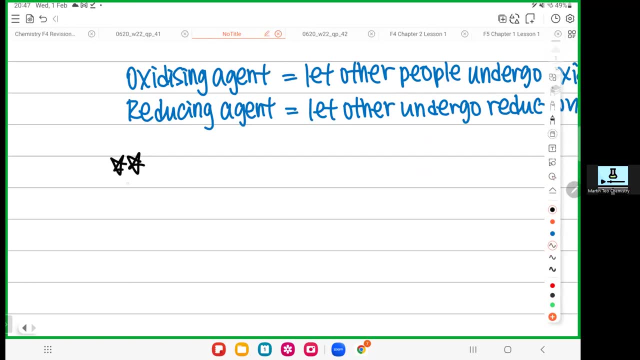 is oxidizing or reducing agent. this will be very tricky already. This will be very tricky already, So I put five star here so that you know how important it is. Not one star, not two star, not three star, five star. 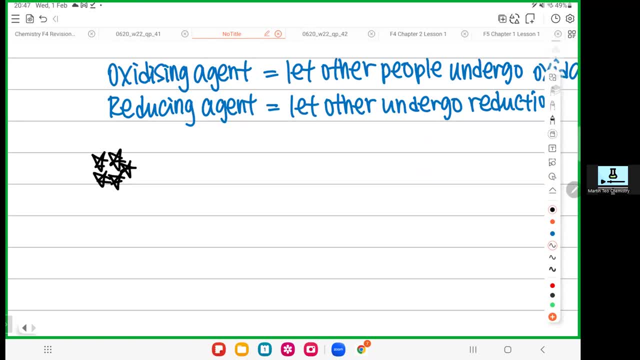 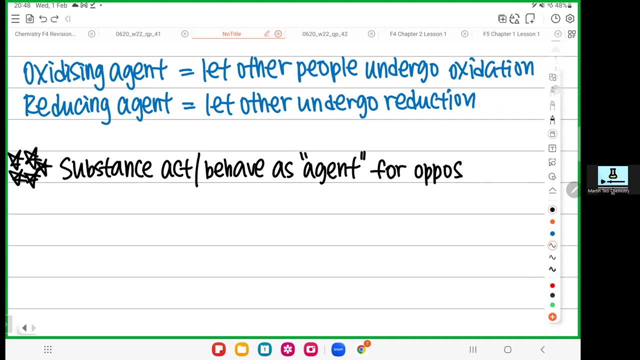 So this concept very important. So what is it? So listen carefully When you come to chemistry. you need to understand this. You need to understand that all the chemical substance, they will always act or they will always behave as the special agent for the opposite process. 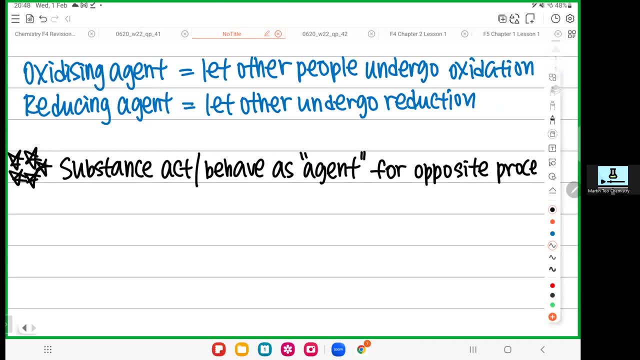 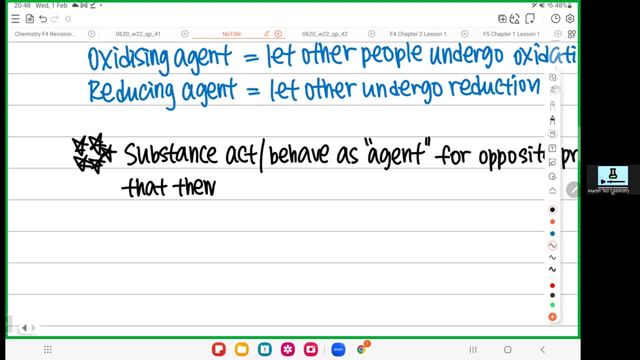 Okay, that themselves undergo. okay, this will be very tricky. This one will be very, very tricky. So you will be the agent for the opposite process that you yourself undergo. Okay, All right. So what do I mean? Okay, what do I mean? 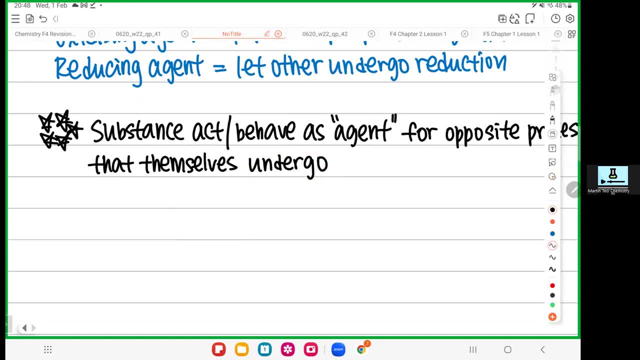 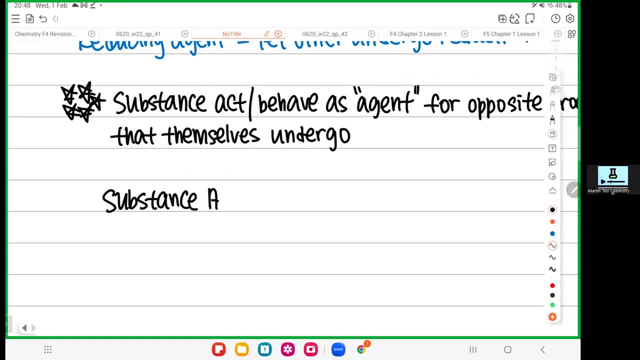 Okay, let's say I am a substance A. So let's say I am substance A, me myself undergo oxidation process. I undergo oxidation process. Okay, I undergo oxidation process, so I will be agent. also, When I undergo oxidation, I am qualified to be agent. 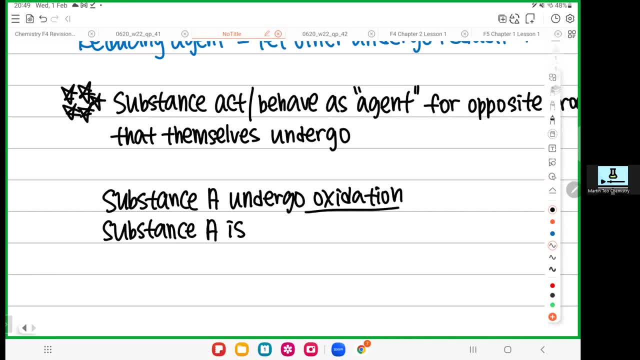 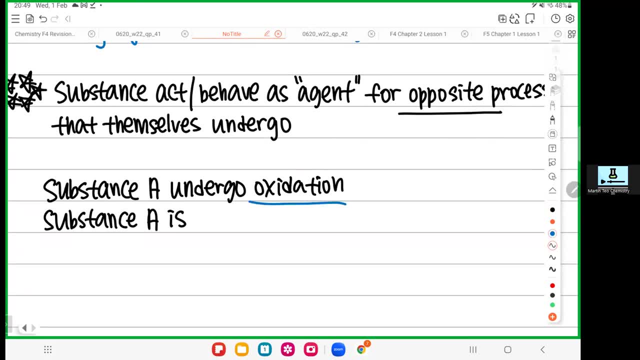 So the agent will be opposite of this. So if I undergo oxidation, I will be the opposite agent. So I will be reducing agent, because the opposite of oxidation is reduction. So I am reducing agent. So you will always be the agent for the opposite process that you yourself undergo. 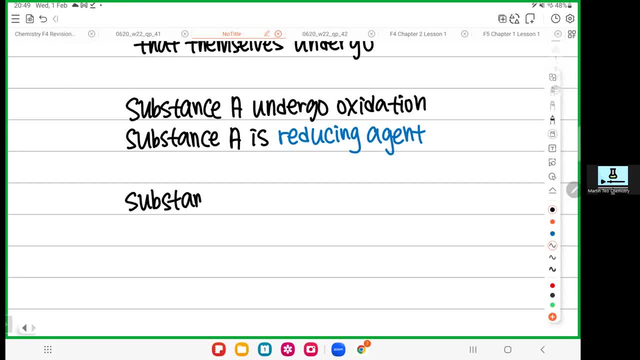 Let's say I have another substance called substance B. So I have substance B, Substance B. this substance undergo reduction. So if I undergo reduction process myself, so who am I? So if I undergo reduction process, I'll be opposite, So I will be the opposite agent of this reduction. 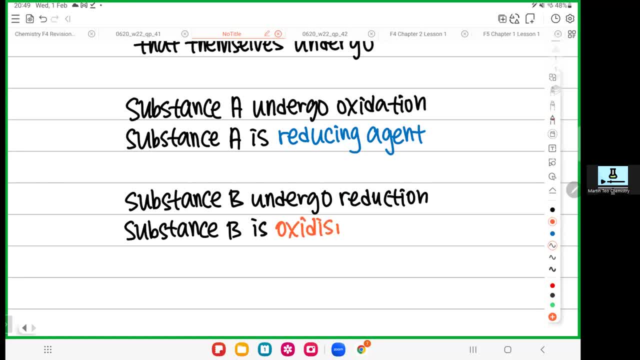 Opposite is oxidizing. So I am oxidizing agent. Okay, So when you know what process that you yourself undergo, you will know exactly what agent you are. So I undergo reduction, I am oxidizing agent. I undergo oxidation, I am reducing agent. 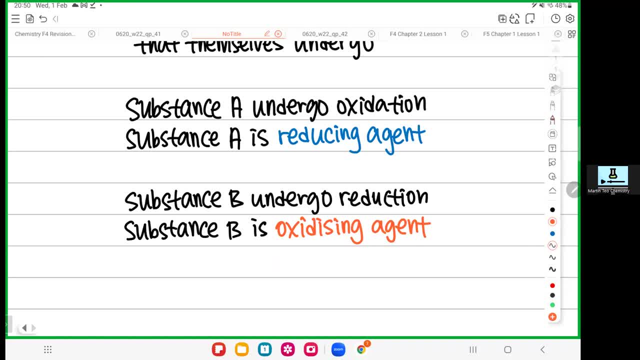 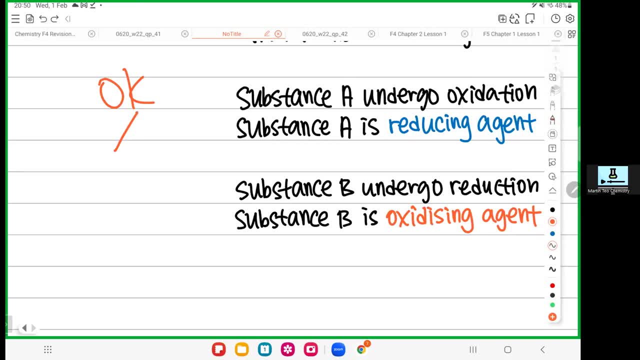 So this part, This part might be a bit confused. Let me know, Are you guys okay? If you are okay, can you type? okay, If you don't understand, put a cross in the chat box. Let me know. It's okay to say not, okay. 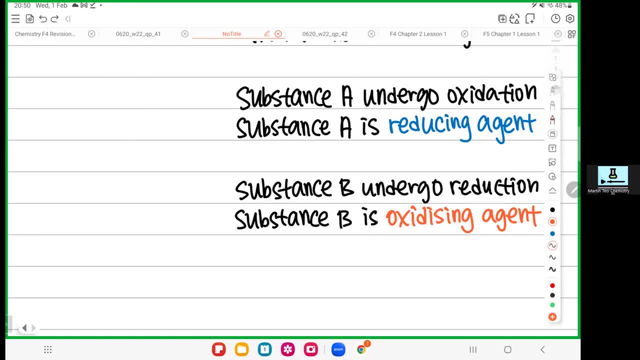 All right. So you have to be very, very careful with this. Okay, All right. Good, So I can see. probably so far got one. Okay, You got one student. I just don't really understand. Okay, Never mind. 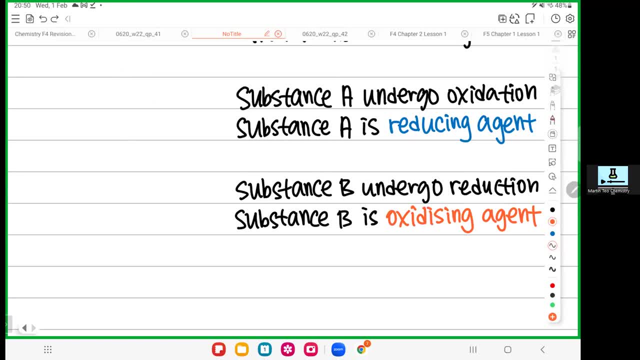 Is there any other don't understand? Is there any other student don't understand? Okay, So, let me go one by one, All right? Okay, So, I hope I pronounced your name correctly, Jerry Harshan. Okay So, Jerry Harshan. 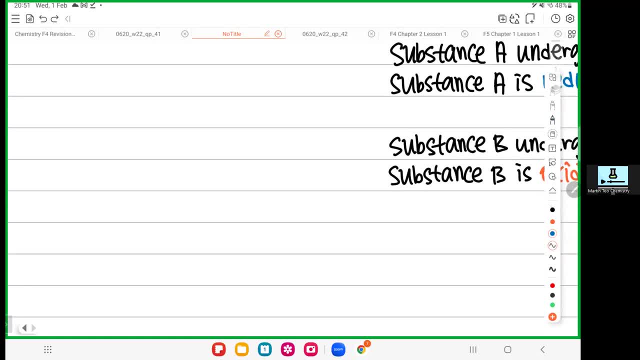 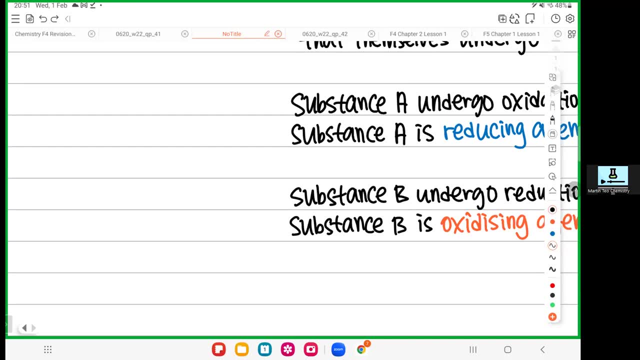 So let me go through this one, Okay. So I want you to follow me. I want you to follow me, Okay. First of all, do you understand what is oxidation reduction? The basic thing first. Do you understand basic oxidation reduction first? 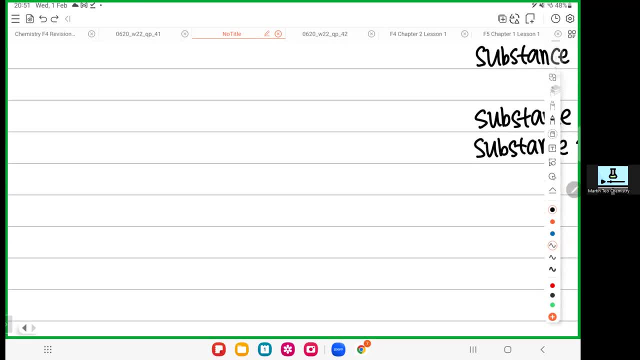 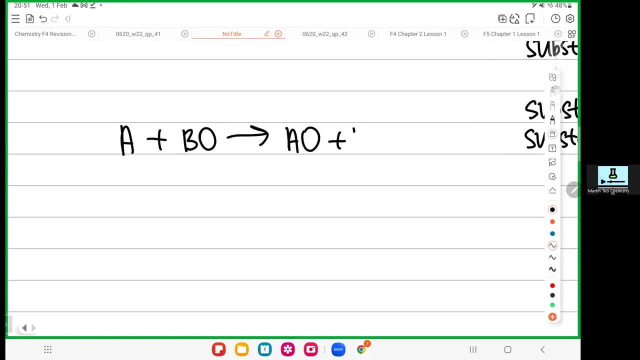 Okay. So now allow me to ask you a simple question. Let's say now, A plus B O become A, O and B. Okay, So I want you to answer me, Jerry Harshan. So now I want to do Apple to Apple comparison. 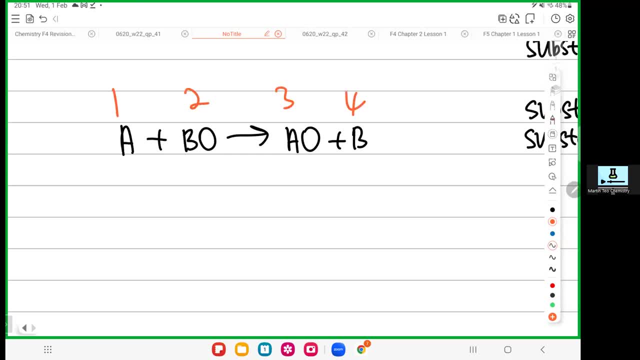 So which one I should compare? You let me know the number, who and who I should compare. When I do Apple to Apple comparison, let me know which pair I should compare. If I choose A here, I should compare with who? Okay, Three, one and three, two and four, Very good. 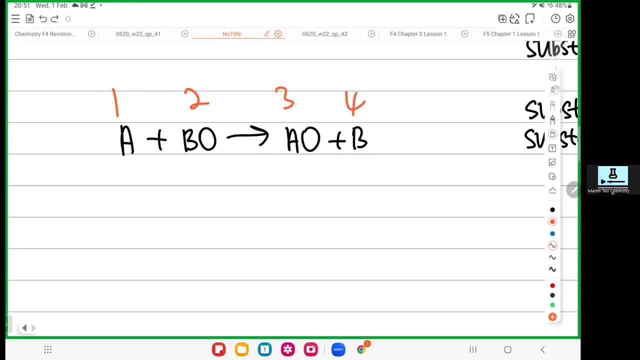 Okay, I choose one and three, two and four. Okay, Let's say I one and three. I compare Apple to Apple. Okay, So can you let me know A to A O, What is the process happen on A? What process A undergo? 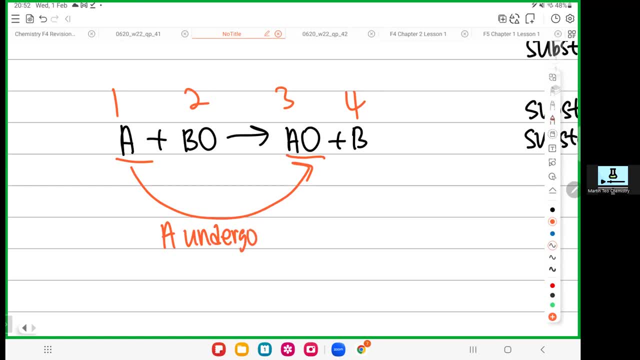 What process A undergo? Very good Oxidation. That's it Why, For the other students, you can see A become A O. What happened? Gain oxygen. So when A gain oxygen, according to the table that we learned today, gain oxygen means oxidation. 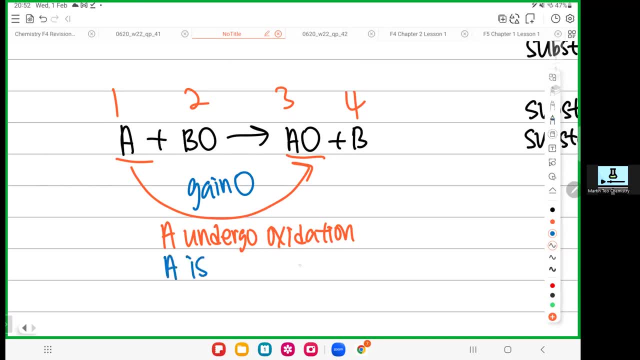 So, when you undergo oxidation, what is the agent you are? So remember, you will always be the agent for the opposite process that you undergo. If you undergo oxidation, you will always be the agent for the opposite process that you undergo. If you undergo oxidation process, what agent you are? 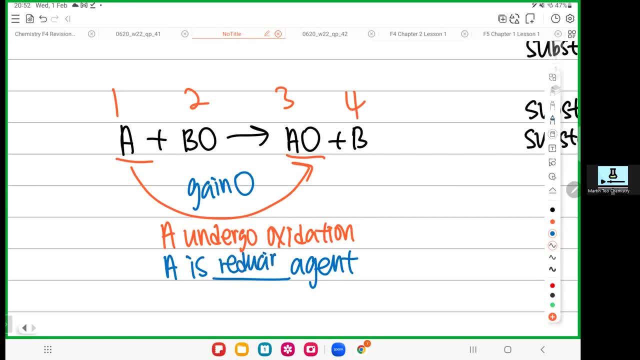 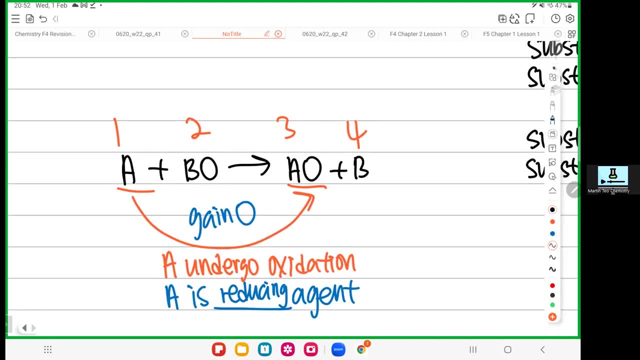 That's it, Reducing agent. So do you get some idea now? Okay, Let's try another one. Okay, guys, come on B O to compare with B. Apple to Apple comparison. B O to B. got O, don't have O. 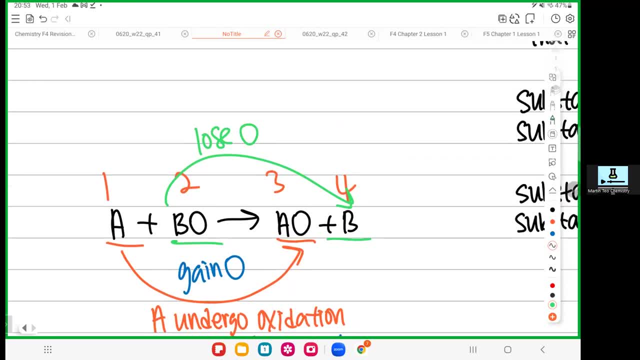 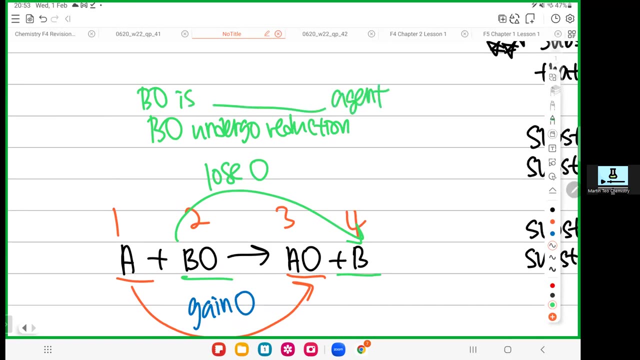 What happened? Loses oxygen. So lose oxygen. What happened? B O undergo reduction, isn't it? Lose oxygen is reduction. So, guys, can you type in the chat box, if B O undergo reduction, what agent it is, What agent it is? 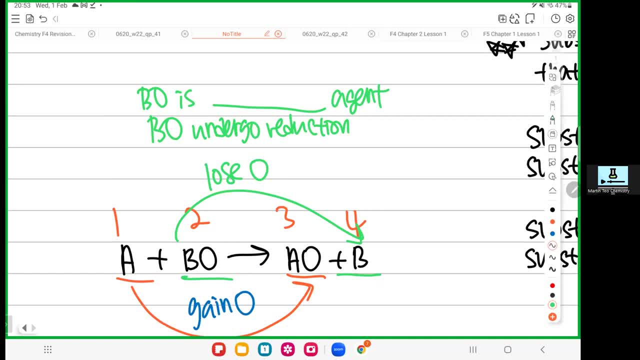 Fantastic, Very good. Haida, All right, Very good. Duncan, All right. Joey, Eliza, All right, Very good. Oxidizing: You get it Okay, As simple as that, So don't mess up. 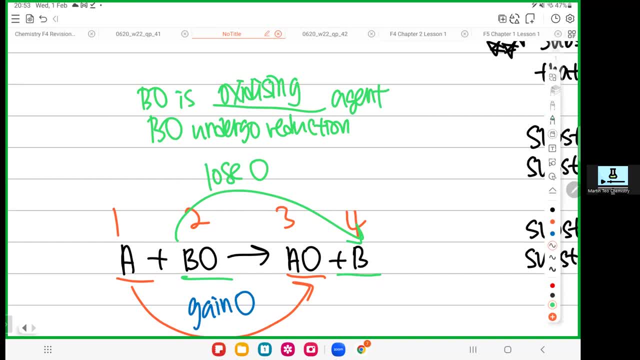 Okay, I'm talking about two things. First of all, I tell you all what do we mean by agent. Agent means what I can help other people to undergo a specific process. If I am oxidizing agent, I help other people undergo oxidation. 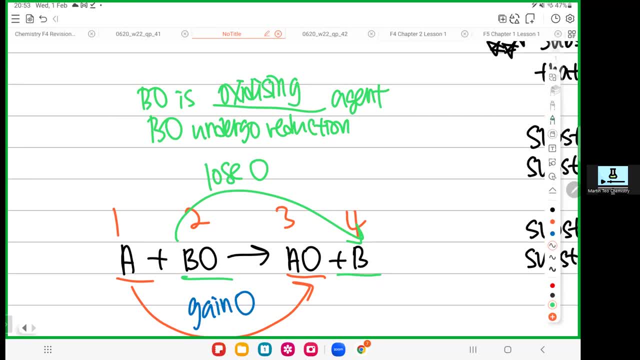 If I am reducing agent, I help other people undergo reduction process. That's it, So that's what the agent do. Then how on earth I know this filler, this substance is what kind of agent? So I must know what process they undergo. Because whatever process you undergo, you will be the opposite agent. If you undergo oxidation, you will be opposite. Opposite of oxidation is reduction: reducing agent. If you undergo reduction, you will be opposite agent. Opposite of reduction is oxidation. 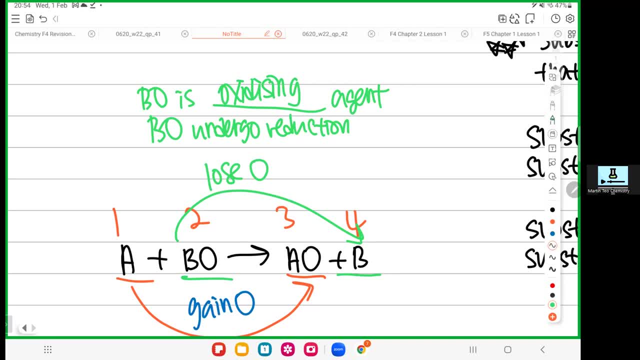 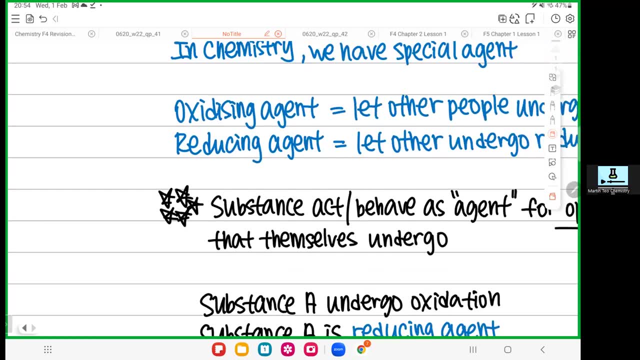 Oxidizing agent. That's it. You will always be the opposite agent for whatever process that you have undergone. That's it. Okay, So simple, As simple as that. So now we can come back here and we can complete the remaining thing already. 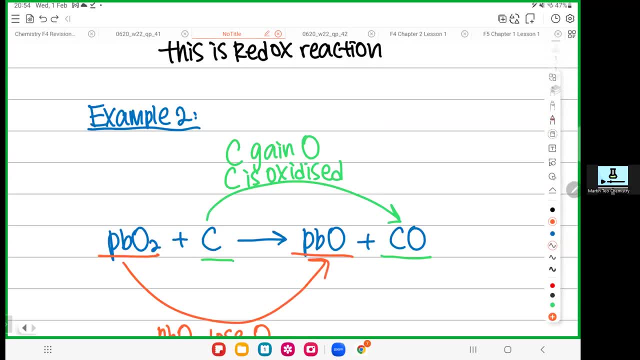 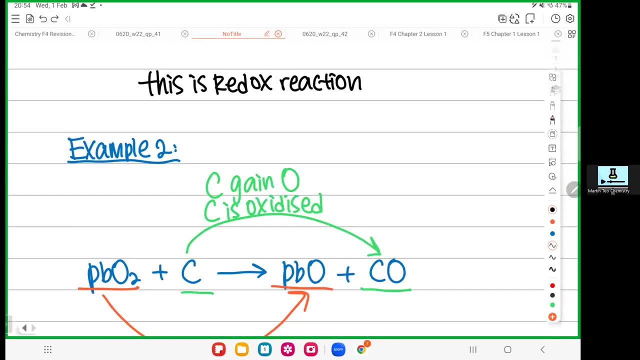 Come Example number one just now. So come on, Maybe we'll open up a new one, We open up a new one, and maybe I give you two minutes for you to try together, For you to try together with me. Okay, So I do example number three with you all. 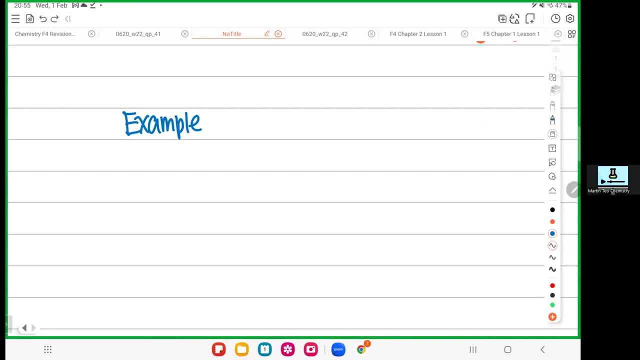 I do example number three with you all. Okay, All right, Example number three: Okay. So let's say example number three. We have this zinc and zinc react with oxygen or two to become full zinc oxide. This question is not hard, but it's a bit tricky for some people. 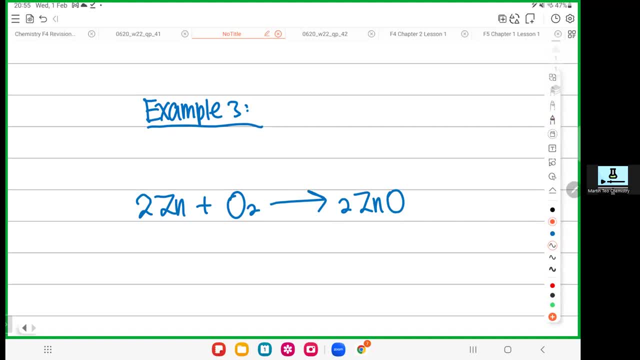 It's a bit tricky for some people. Listen carefully, Listen carefully. How are we going to? How are we going to do this question? How are we going to do this question? Okay, First of all, same thing: Choose the Apple and Apple comparison first. 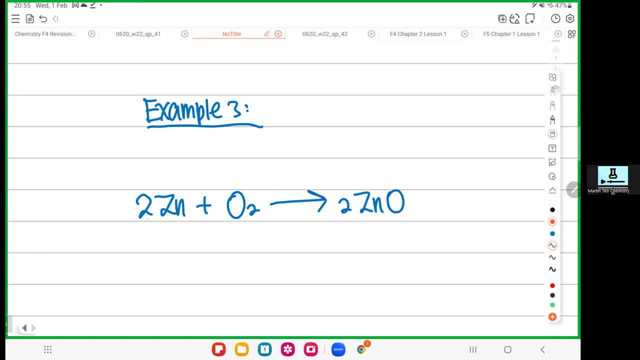 Always choose one Apple from the left, one Apple on the right. So first Apple on the left, Let me choose this fella. So Apple on the right, No choice, There's only one here, Of course. I choose this one. 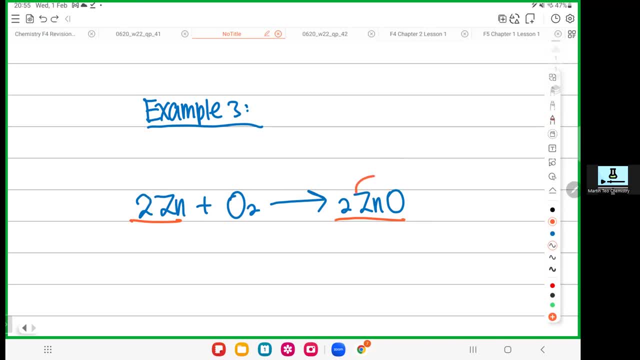 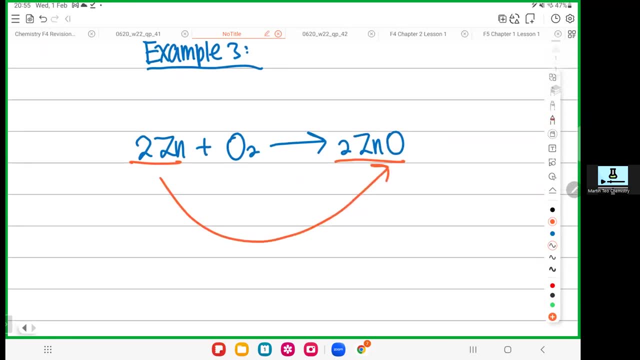 So when you compare the left hand side, the zinc, right hand side, the zinc come with O, Quite easy. No O got O, So here to here. So what happened? The zinc actually gained oxygen. So gain oxygen, Gain oxygen means reduction. 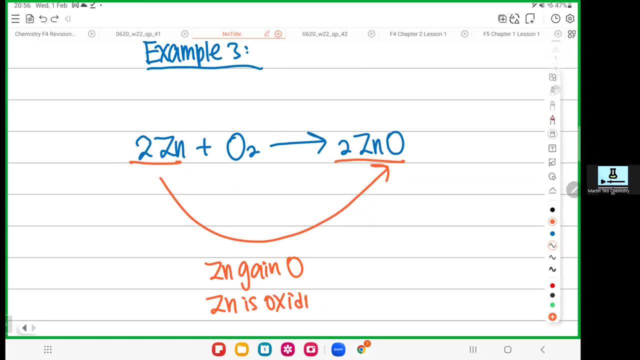 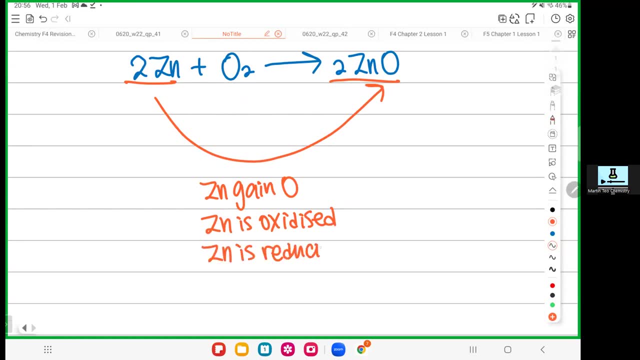 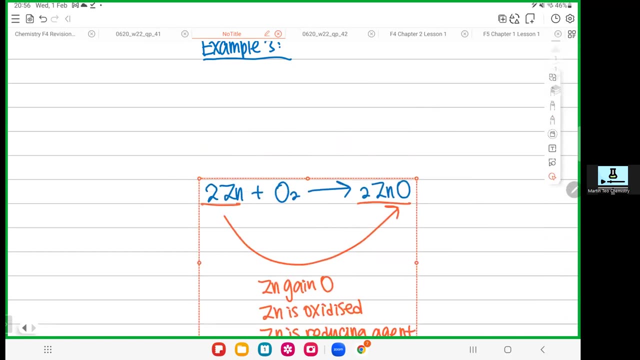 So when zinc undergo reduction, it will automatically become the opposite agent. So the zinc itself become reducing agent. Remember, when I undergo oxidation, I will be reducing agent. It always go opposite. It always go to Bali. So settle. Now let's look at the another one, another Apple. 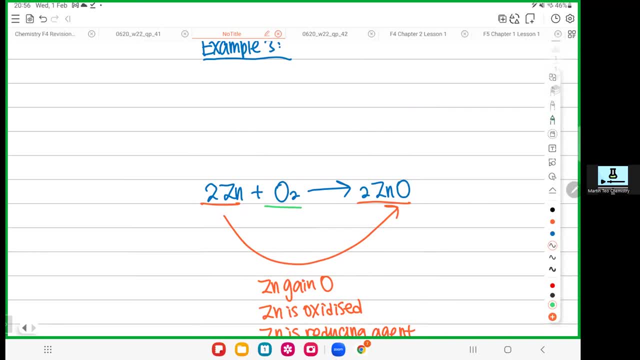 So now I choose another Apple on the left. So which Apple I want to compare? the right, Same thing. So I still compare with this fella. So, sir, I thought just now you compare already. I didn't say you cannot repeat, right. 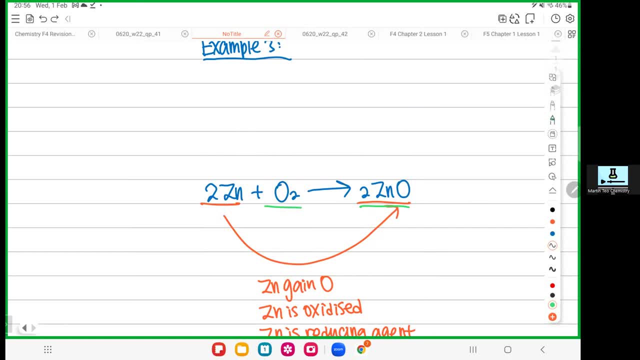 I only say you must compare the left and the right. Choose one Apple on the left and one Apple on the right. I didn't say you cannot compare back to the same Apple, isn't it? You can compare back to this Apple, Although this Apple just now compare with here already. 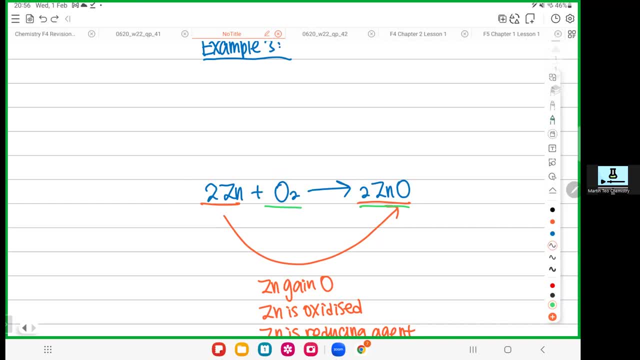 You can reuse the Apple and compare with this fella. It's okay. So let's do it. Left hand side- O2, two oxygen. Right hand side: one O. Now be careful, Many students they will start to say, sir, you got two O right. 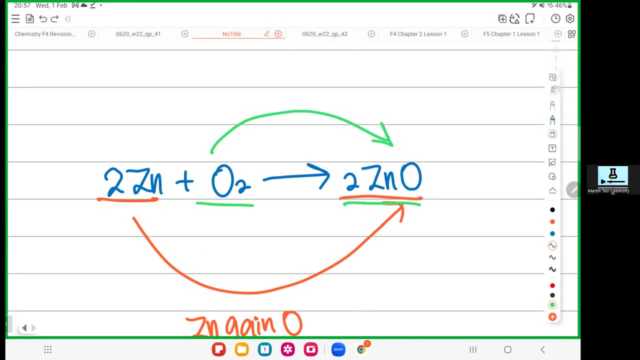 Here got two O By right. oxygen doesn't change. Okay, listen carefully When you do Apple to Apple comparison, please don't bother. the number in front, All the number in front here only used to balance the equation. All the number in front here only used to balance the equation. 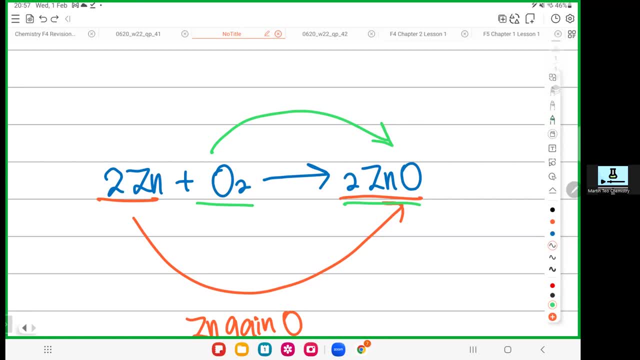 When you do that, when you do the Apple to Apple comparison, do not bother the number here. Don't look at the number in front. So only look at O2 and ZNO- This number two don't look at it. So O2 got how many O? 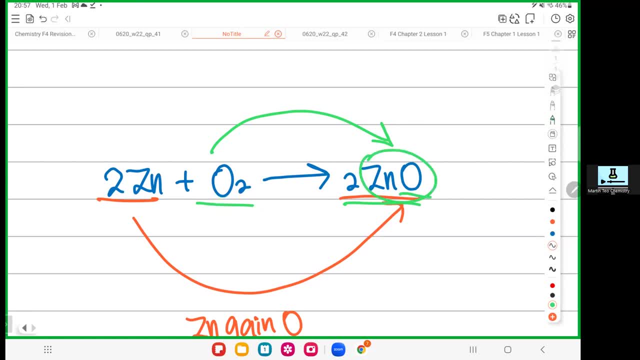 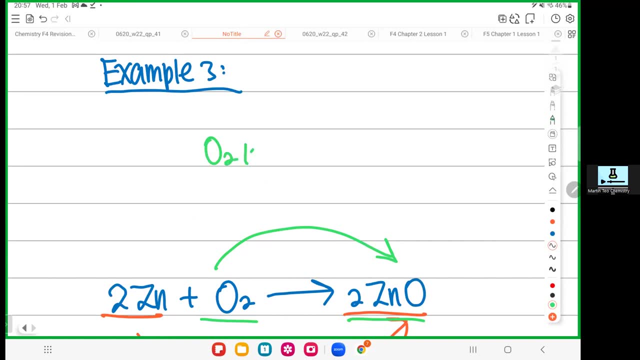 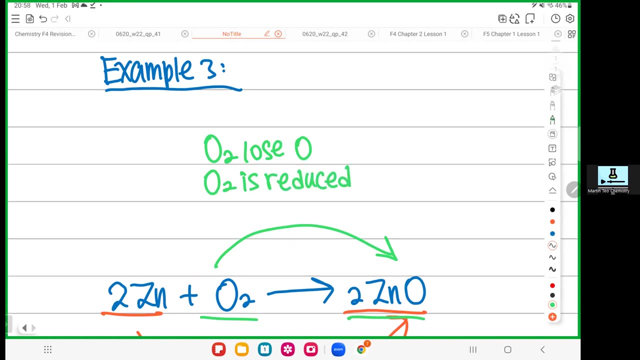 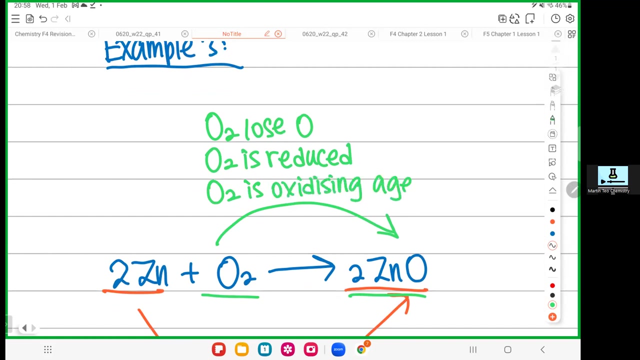 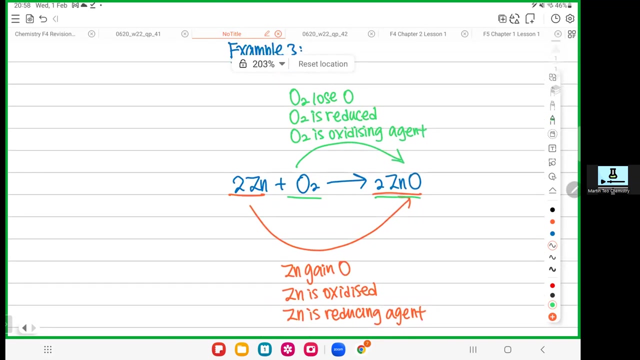 Two ZNO got how many O One? Two O become one O. So what happened? Lose oxygen, So the O2 loses oxygen. So lose oxygen means reduction. When you undergo reduction you are opposite oxidizing agent. Okay, so guys now, based on this question up to now, is it okay? 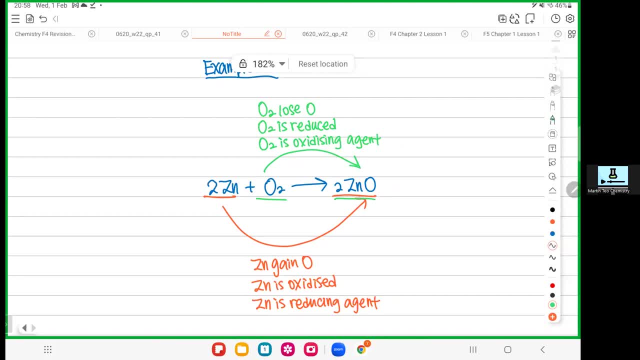 So far so good. Is it okay? If not okay, same okay. So far, so good, Okay. so I want you all to be honest with me. Not okay, just say not okay, Don't feel bad. 40 people say okay. 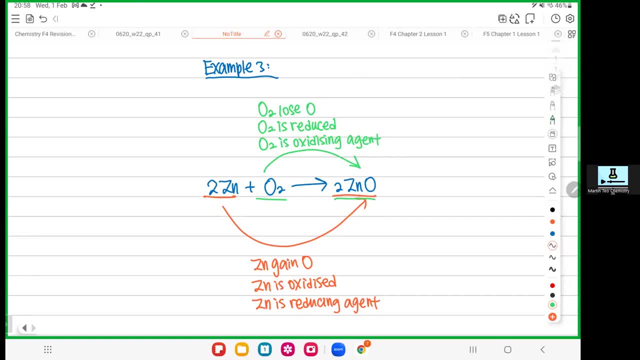 I am the only one who say no. Okay, I feel bad. No, don't think like that. Please don't think like that. Okay, I'll try my best to help you, but you just need to be honest with me. 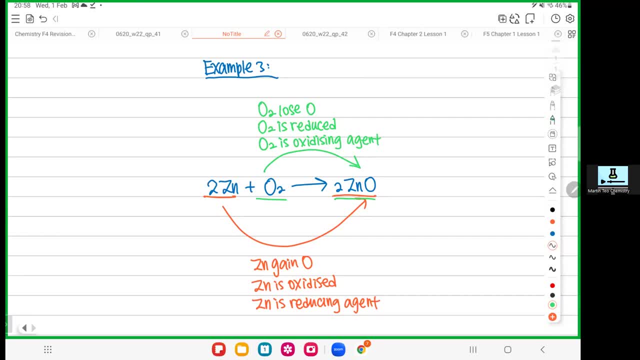 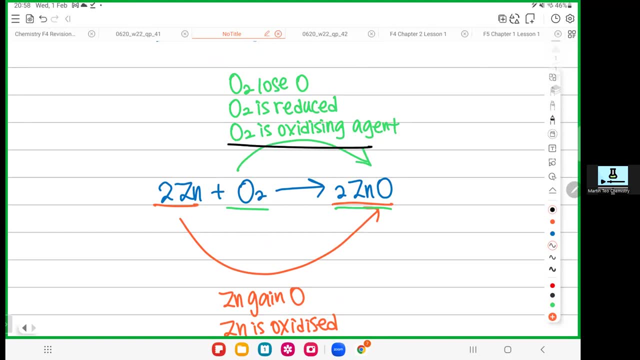 Can I? All right. So you see, guys, it makes perfect sense. What do you see? You see, it makes perfect sense. One Why I say O2 is oxidizing agent. Oxidizing agent means what You help other people to undergo oxidation. 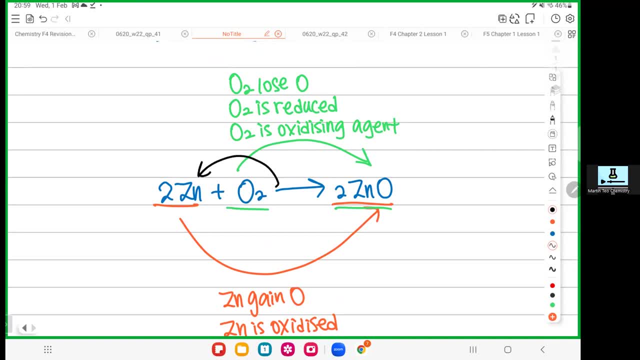 Make sense. O2 gives one O to the zinc right. O2 gives one oxygen to the zinc so that it becomes an N. Also, when I give oxygen to the zinc, I let the zinc to gain oxygen. When I let the zinc to gain oxygen, I help the zinc to undergo oxidation, isn't it? 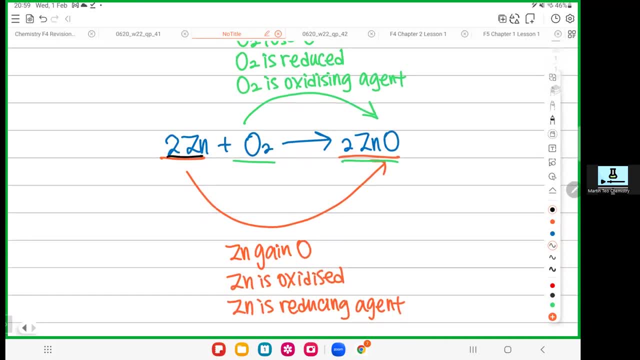 That's what I do. Okay, same thing. The zinc will take one oxygen from O2.. So when zinc Take one oxygen from O2, zinc will let the oxygen to lose. O. Zinc will let the O2 to lose. O. when I let other people to lose oxygen, 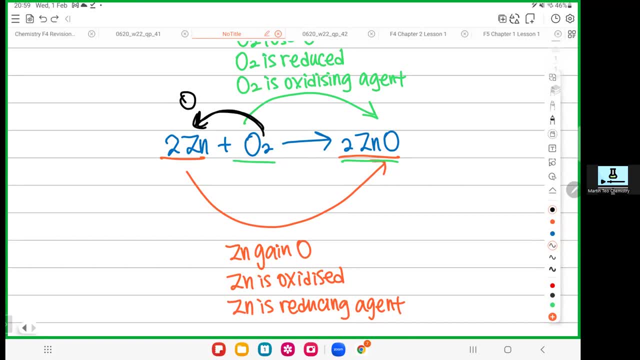 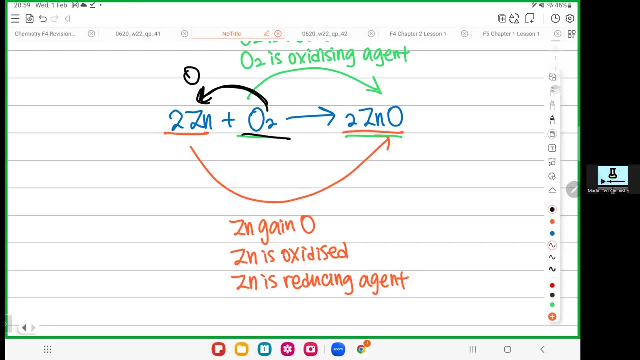 Okay. so what is it? I let other people to lose oxygen. I let the oxygen to undergo reduction When I help this oxygen to lose the oxygen. so I am reducing agent. Makes sense, right? Zinc is reducing agent Why I let the O2 undergo reduction. 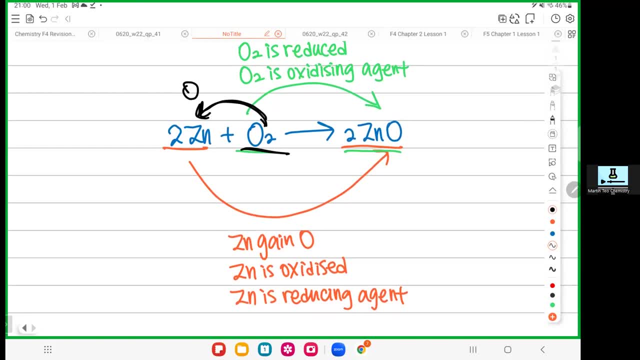 How I let the O2 undergo reduction. I take away O from the O2.. When I let the oxygen to lose the oxygen, When I let the O2 to lose oxygen, the O2 undergo reduction. That's it. So that's what happened. 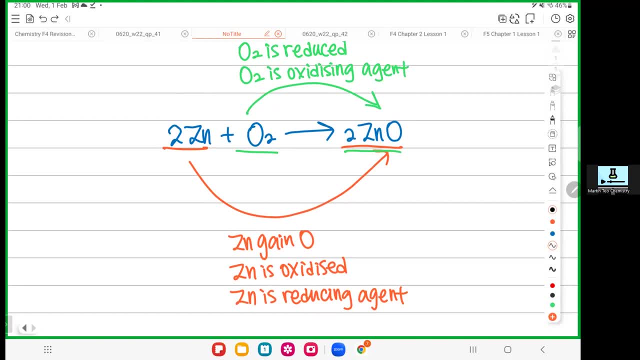 Okay. so when I am agent, I help other. Okay. so that's why don't confuse. First of all, you must know what the agent do. Oxidizing agent: what you do. You help other people undergo oxidation. Reducing agent: what you do. 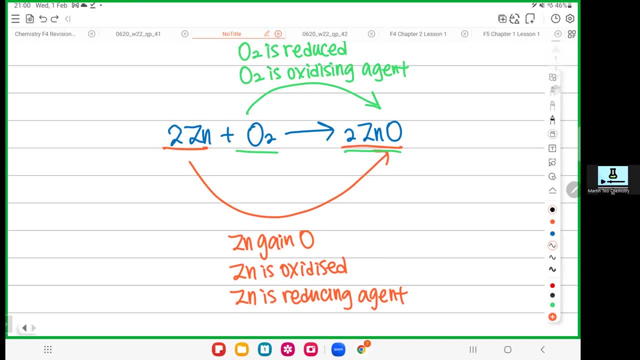 You help other people undergo reduction. How to know who is oxygen, Who is oxidizing agent, Who is reducing agent? You just need to know what process it happens. If you undergo oxidation, you become the opposite agent, Reducing agent. If you undergo reduction process, you become opposite agent. 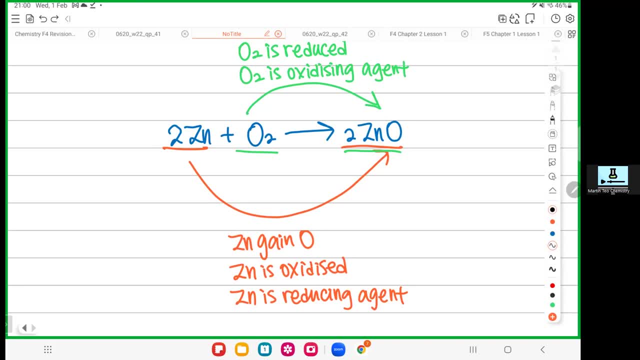 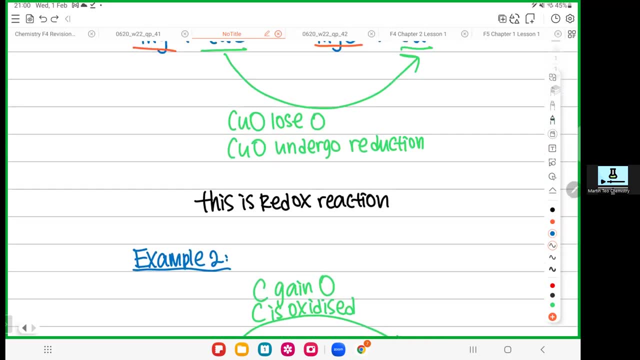 Oxidizing agent. I keep on repeat, repeat, repeat, repeat and repeat, because this is so important. This is very, very important. Okay, that's it. So that's how it works. Okay, now the last example. this is for you. 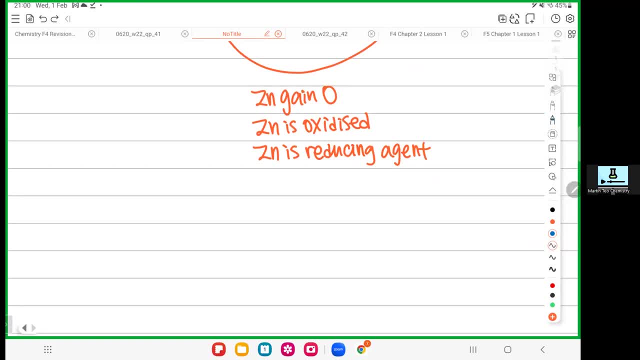 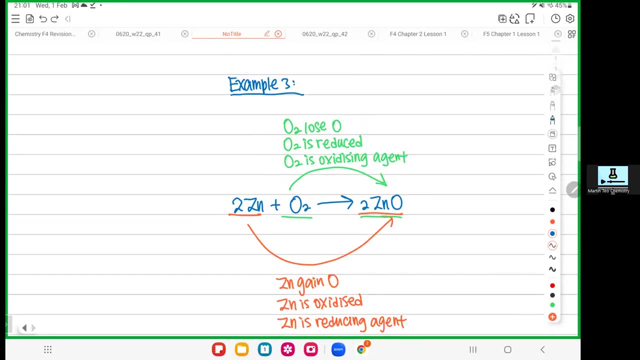 Maybe you can try to do. Okay, I would like you all to try to do this question. You can try to do this question. You do like what I did. Okay, you must know who gain or lose oxygen, what process it undergo and what agent you are. 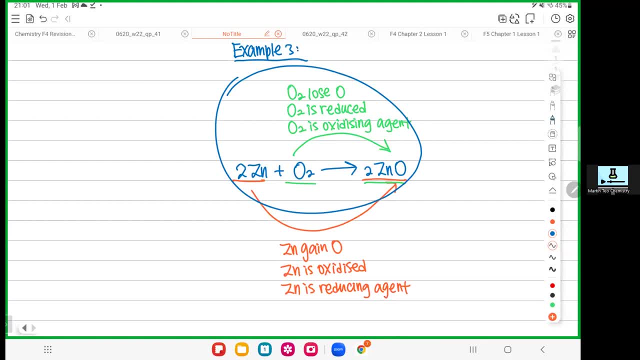 So tell me three things. Okay, follow exactly what I do. Okay, draw the proper arrow, Choose the right apple, Do the right comparison, Tell me who gain or lose oxygen, Tell me who undergo oxidation and reduction, and tell me who is the oxidizing or reducing agent. 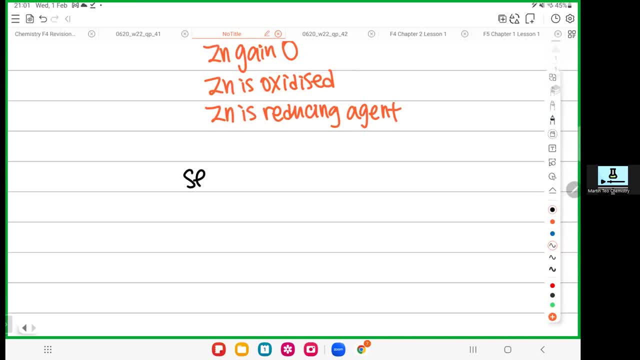 So this one is a self test For you all. Okay, so after this self test, then we will move on to the hydrogen method, because I believe if you understand oxygen method, you shouldn't have a big issue when you move on to hydrogen method, because they are very, very similar. 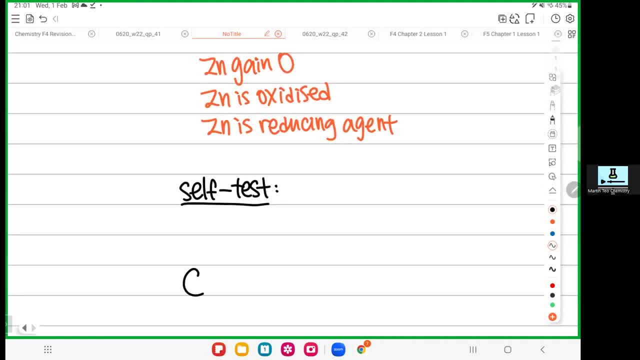 Come on. So this is a self test for you all. This is a carbon, This is a carbon dioxide and this is a carbon monoxide. So, guys, all right, you can try. So you just need to tell, you just need to follow exactly what I do. 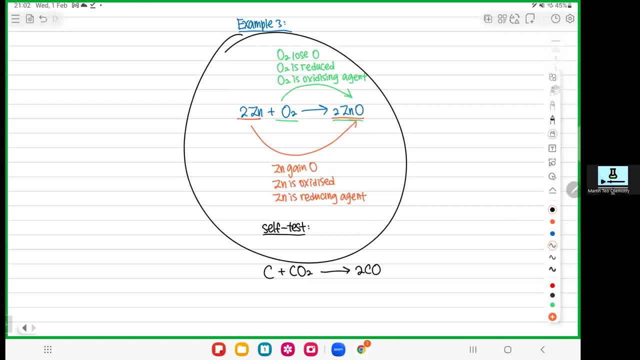 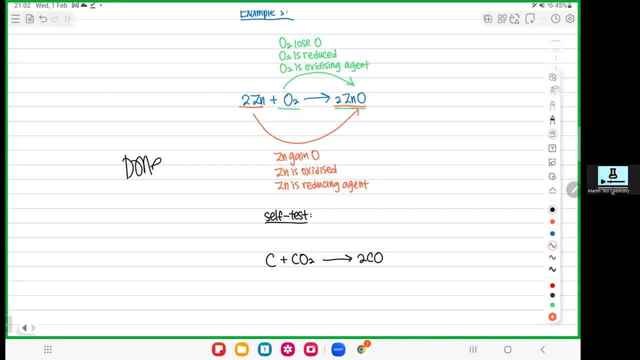 Something like this: Okay, you try first, Come on. Okay, so once you are done, you type done for me. If you finish, already type done. So I want you to do exactly what I do: Choose the right apple, Do the right arrow. 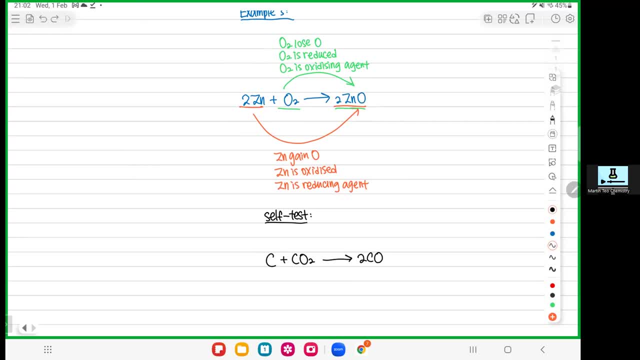 Tell me what process it happens. Tell me what agent it is. Okay, come on, Take your time. All right, Some might do it very quickly, Some might take a longer time. It's okay. Don't compare with others. Okay, follow your own pace. 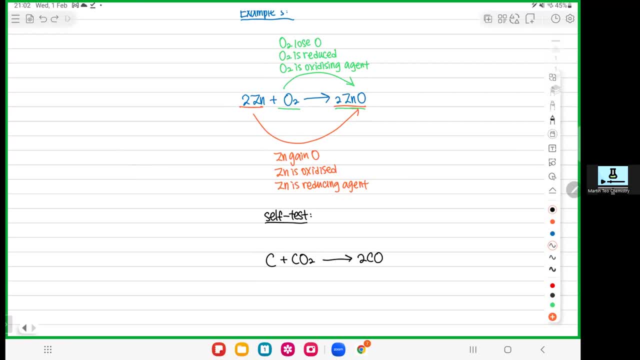 Follow your own pace. Yeah, All right. So I'm going to do my first step, which is take one. So I'm going to do my first step, which is testing. I'm going to do the first step with my sample. 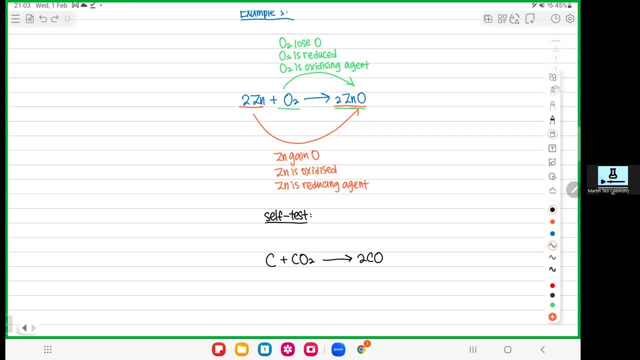 I'm going to do my sample So you can see how long this takes. Now I'm going to tell you what I'm going to do, How long it takes. If you want to do this test, just follow my instructions, Okay. 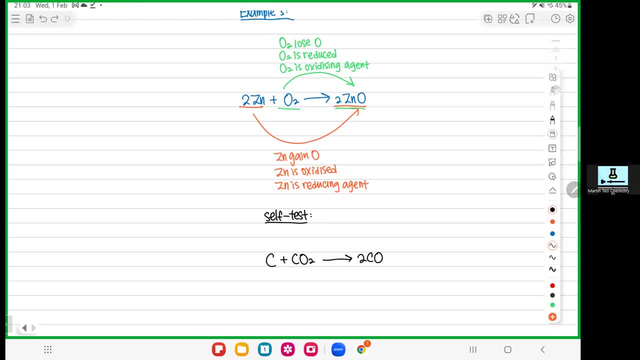 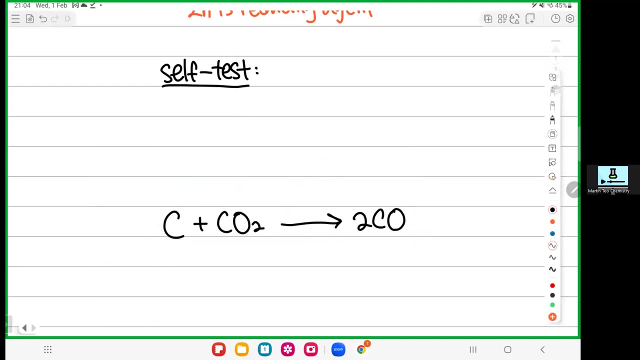 Thank you. Okay, guys, Okay, let's discuss on this question. yeah, Okay, first of all, please choose your apple. okay, Always choose one apple on the left first. Always start from the left. okay, The apple on the left, let's say carbon. 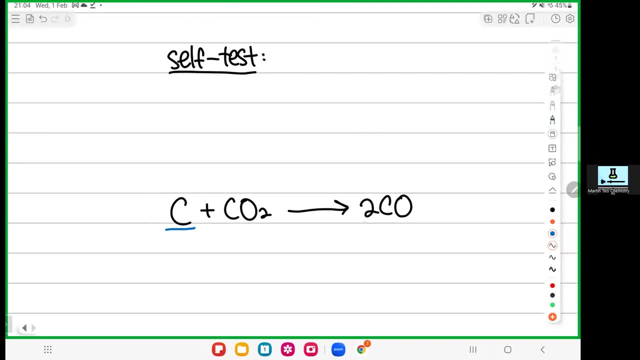 So you must choose one apple on the right, Right-hand side. you don't even have a choice- Must be this one. So left to right. So you want to go top, you want to go bottom, up to you It's okay, one huh. 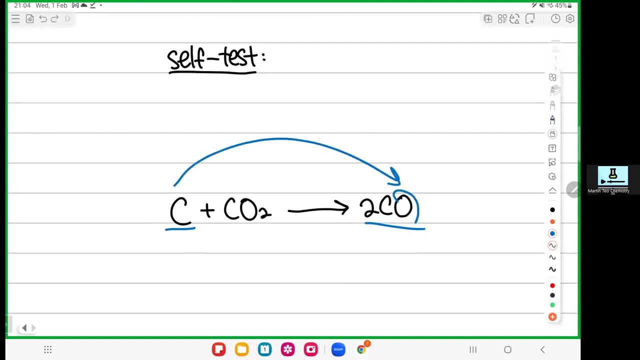 So let's say, go top, This carbon got no. oh, this carbon got one. oh, Remember, when you compare this number two, don't bother, huh, Don't bother. number two in front, Only compare the formula, the number in front only for balancing. 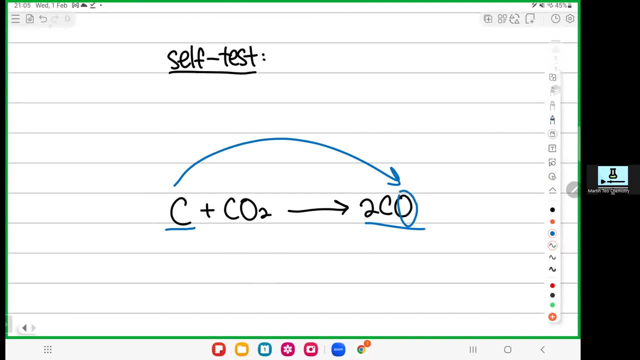 C becomes CO, You gain one additional oxygen. So you gain oxygen. huh, So carbon gain oxygen. So carbon undergo oxidation. So carbon it's reducing agent, End of story. So another apple to apple conversation. Comparison. Choose another apple on the left- CO2.. 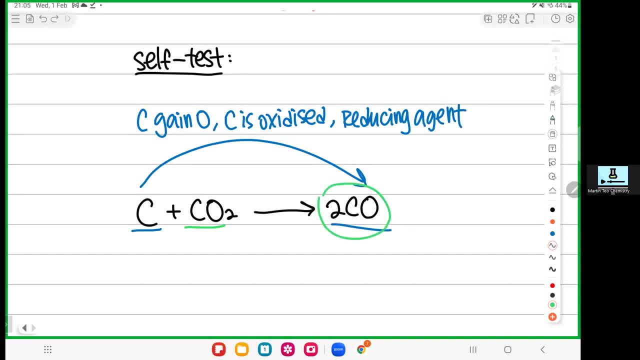 So you must choose one apple on the right. So this apple, although just now you use, already now you can use back the same apple. Okay, nevermind, CO2 become CO1.. Remember the two, don't bother If you put a two, you're confused already. 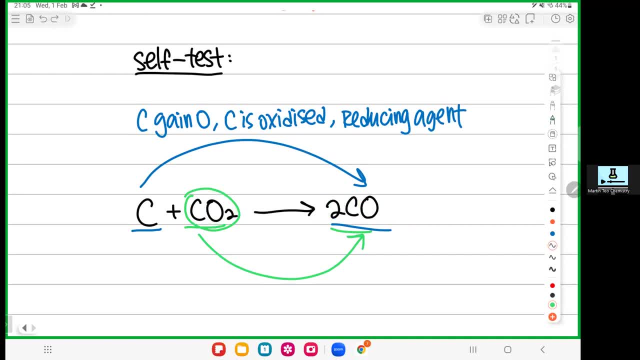 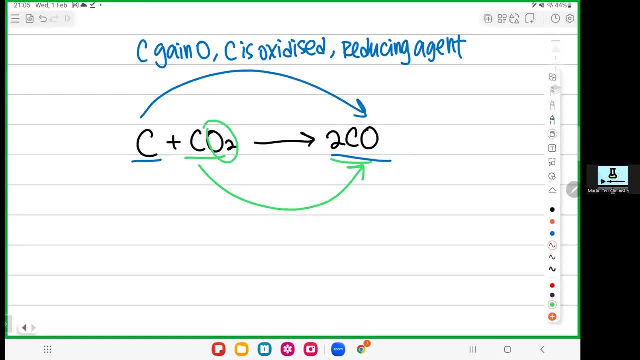 Here got two O, here got two O. Cannot the number in front? don't bother, Okay, don't bother. CO2 to CO. So what happened? CO2 got two O, CO got one O, So one oxygen went missing. 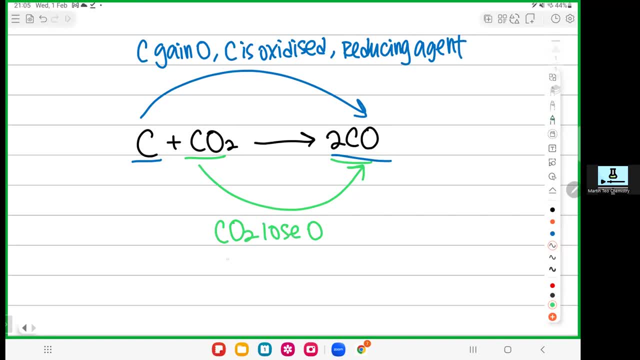 So CO2, lose oxygen. So lose oxygen, undergo reduction process. When you undergo reduction, you'll become the opposite agent: oxidizing agent. End of story, okay. So with that being said, we are all done with the oxygen method, okay. 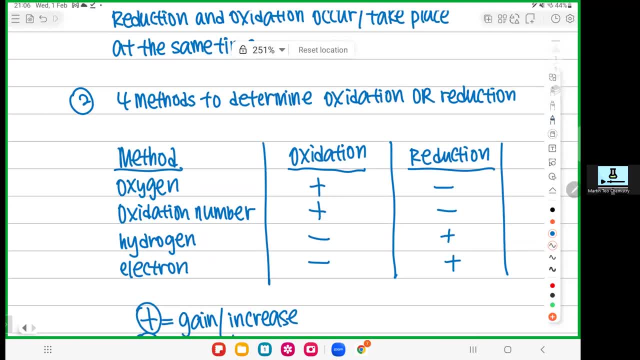 So the first method is all done. Let me know in the chat box: guys, So far, are you guys okay with oxygen So far? I want to make sure everyone okay for stay only and move on. Okay, guys, very good. 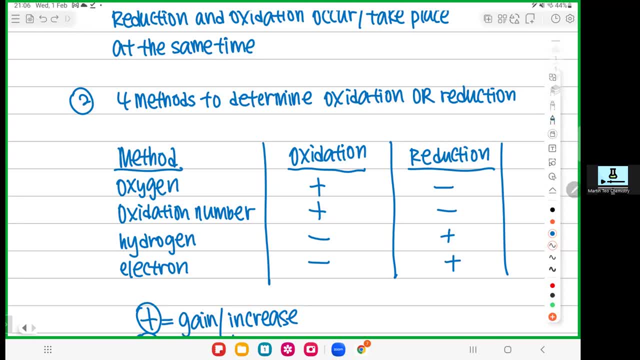 Very good, So you guys can follow right. Okay, So I memang want to go so slow, I memang want to go this slow And I memang purposely go very slow to make sure you really can understand. okay, I go fast. no people can understand. 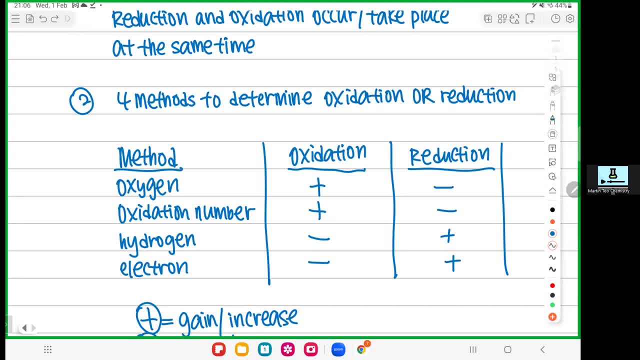 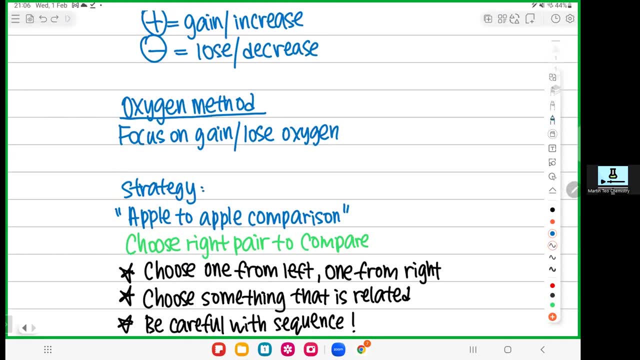 No point? okay, No point. I rather go super slow, but you can understand. Now let's go on with hydrogen method. Hydrogen method is very, very rare in SPM, Not popular, okay, Not popular, but if you understand the oxygen method, 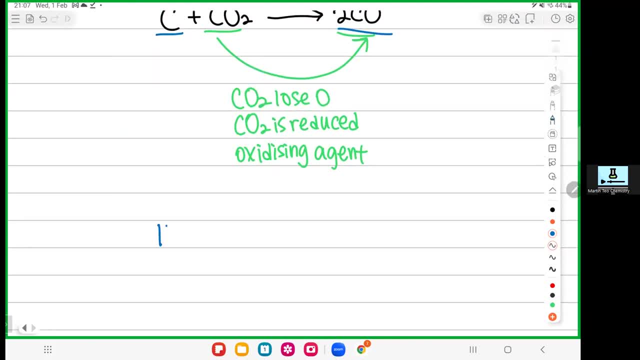 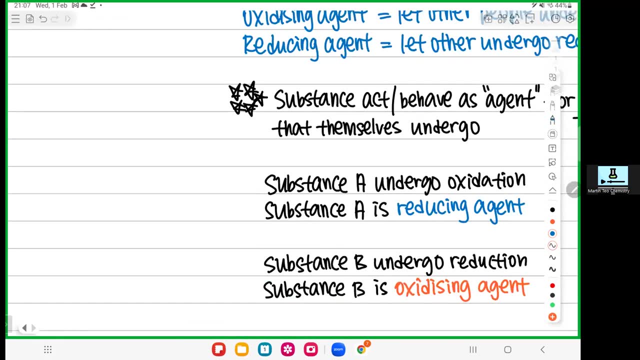 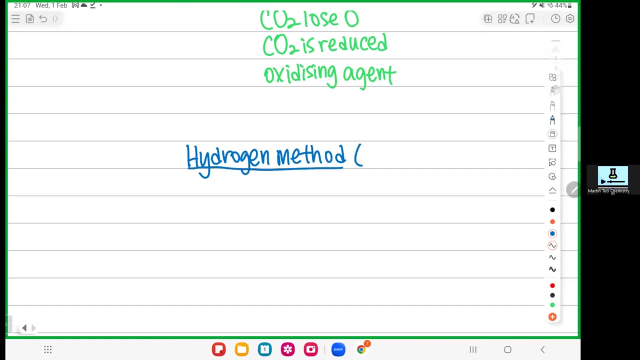 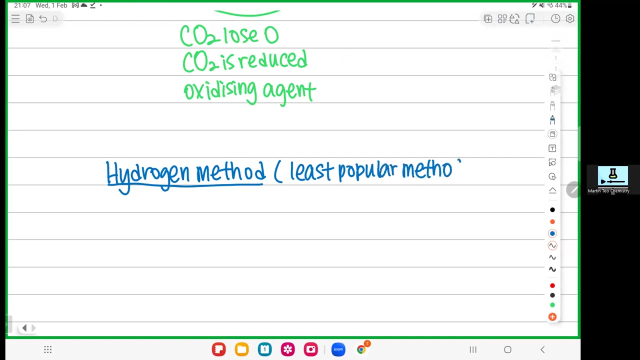 you shouldn't have a big issue with the hydrogen method. okay, Hydrogen method, you follow exactly what oxygen method will do. okay, You just need to focus now on hydrogen, okay, Okay, Hydrogen method is the least Most popular method among four. 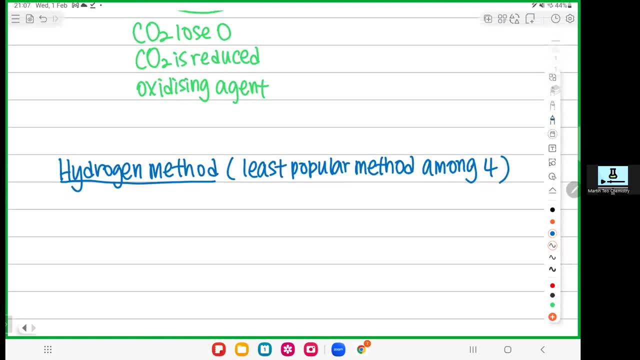 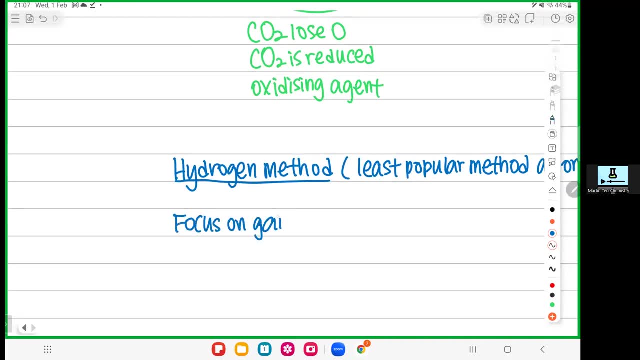 So we have four methods. The least popular one is hydrogen method. okay, So same thing. now We just need to focus on whether you gain hydrogen or whether you lose hydrogen. okay, So if you understand the so-called oxygen method, you shouldn't have a big issue. 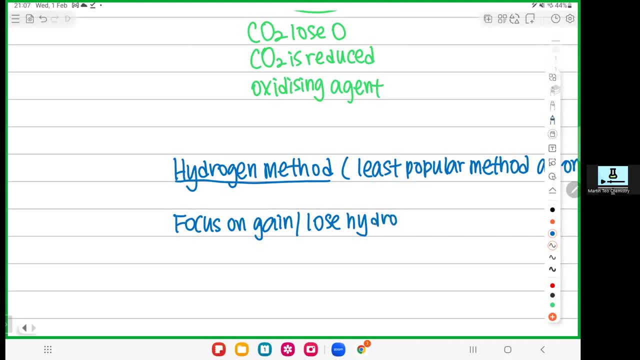 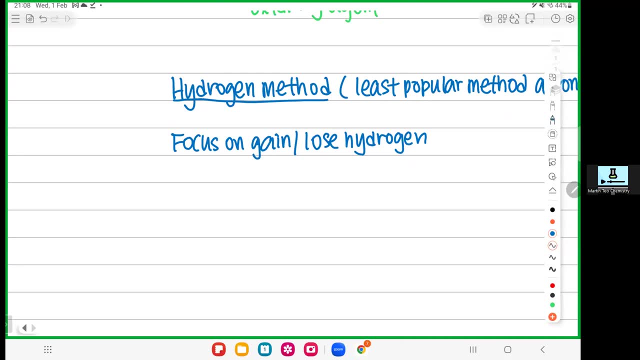 You shouldn't have a big issue at all when it comes to the hydrogen method. okay, Let me show it to you. Let me show it to you now. all right, So how to do the hydrogen method. How are we going to do the hydrogen method? okay. 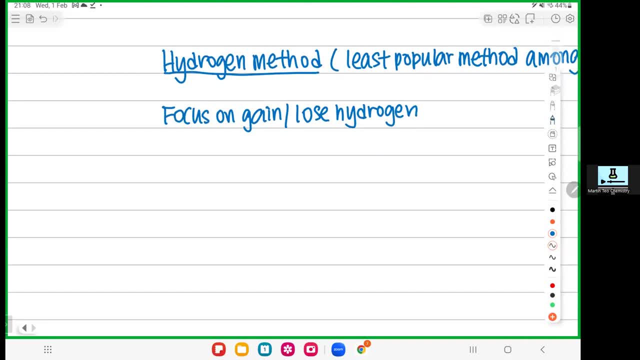 So let's see, okay, We will use two examples. Okay, I'll use two examples also to do the demonstration. okay, I'll do the demonstration here, okay. So let's say the first example, I'll show you one example and then I'll show you one K-Bud question, okay, 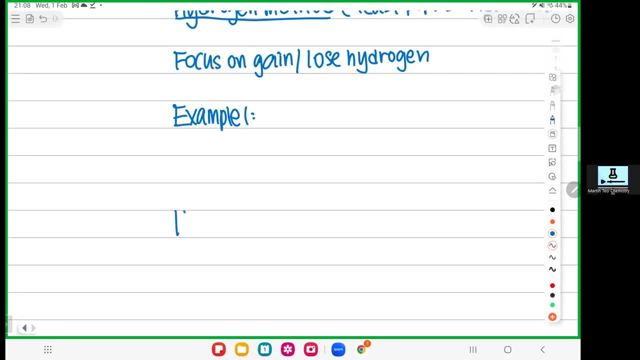 Okay. So example number one: let's say H2S, hydrogen sulfide, react with chlorine, so that you become hydrogen chloride and you become sulfur. So same thing. Now we just want to focus on hydrogen. okay, We just want to focus on hydrogen. 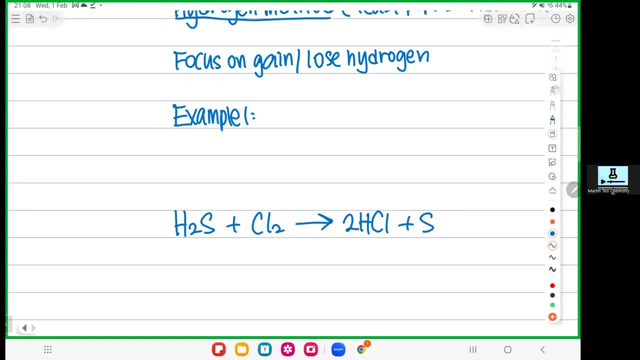 Just now we focused on oxygen, Now we focus on hydrogen. as simple as that. okay, All right, So same thing. First of all, choose the apple first, Always choose one apple on the left, Always, always. begin with one apple on the left first. 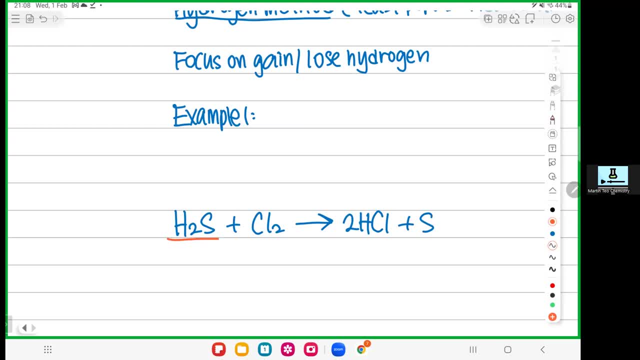 One apple on the left. So which apple you want to compare with the right-hand side here? Sulfur, Why don't you compare this one? okay, Why don't you compare this one? You see, this fellow got 2H. 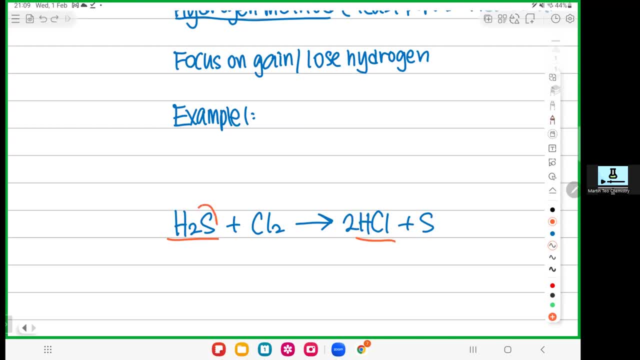 This fellow got 1H. Looks good, But here the sulfur. why all the sulfur become chlorine Cannot matter. There's no way sulfur become chlorine, or instead it becomes something else. Doesn't make sense. So if H2S, H2S and S at least make sense, but why? 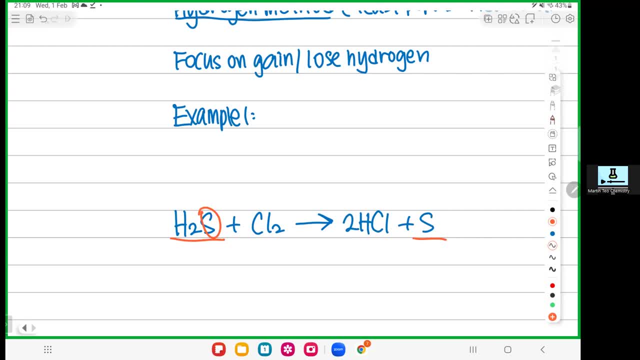 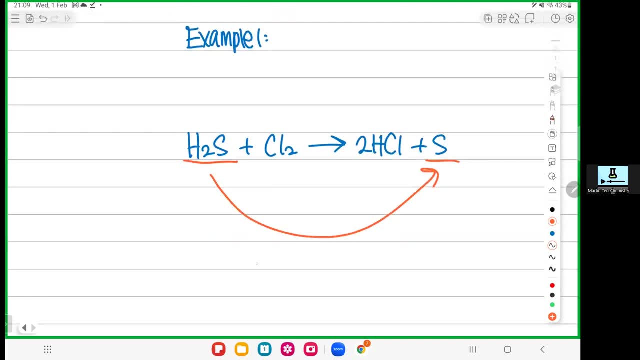 Got sulfur, got sulfur. Then you can see this sulfur sticking with 2H. This sulfur got no hydrogen. So from here, obvious no. So you can see that from left to the right-hand side the H2S lose hydrogen. 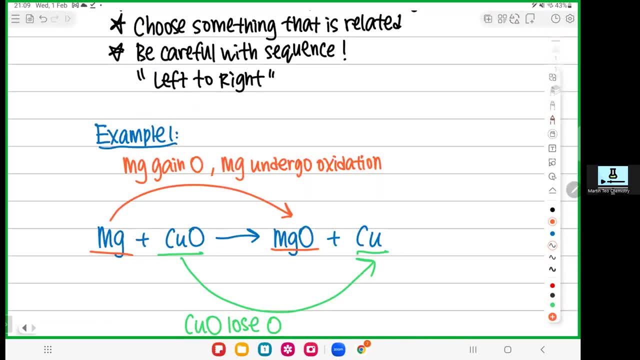 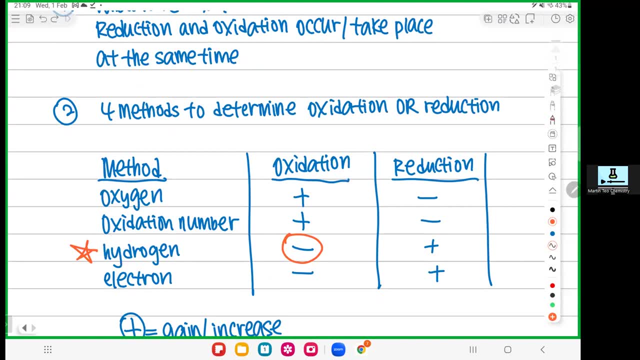 Okay, Now look at hydrogen method that we learned earlier on today. So if you look at hydrogen method, when you lose the hydrogen, it's oxidation. So tabalic Hydrogen method, exactly tabalic of oxygen When you gain oxygen oxidation. 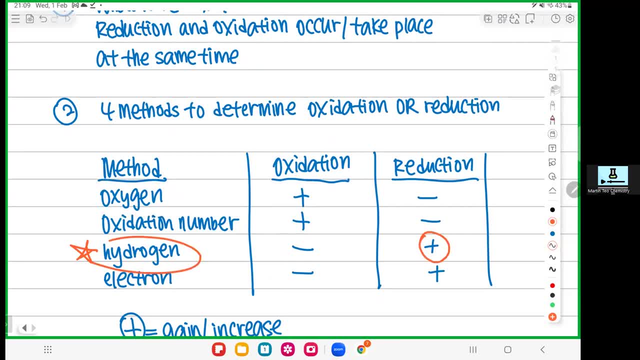 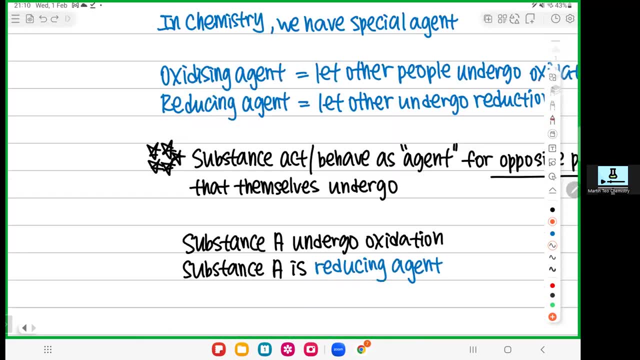 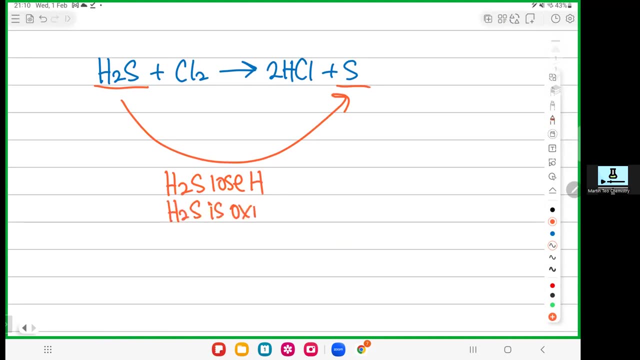 Now hydrogen tabalic. When you gain hydrogen reduction, So hydrogen and oxygen, exactly tabalic, Exactly tabalic, All right. Opposite: So when hydrogen sulfide lose oxygen, so you undergo oxidation, All right. If you're not sure, just refer to the table. 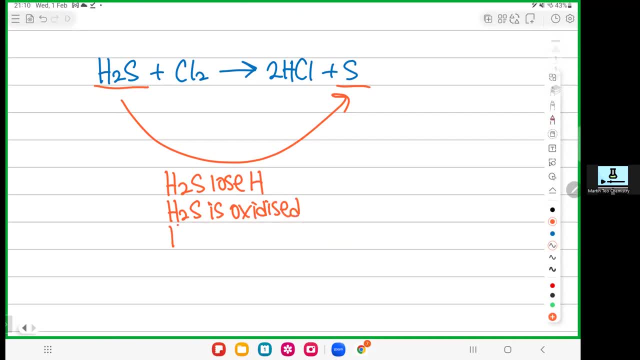 Just refer to the table. So when you undergo oxidation, same thing: You'll be the opposite agent, So you will be reducing agent. Okay, All right. So now another apple to apple comparison. So choose another apple: chlorine. Another apple is HCl. 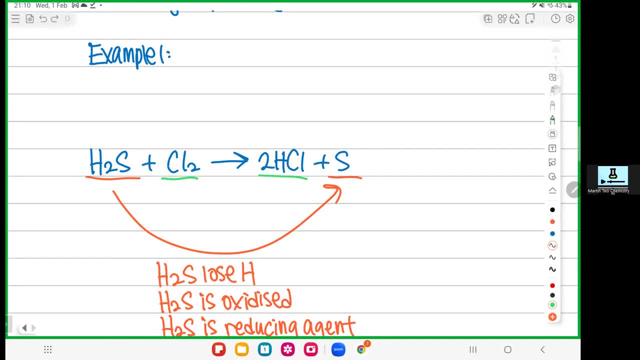 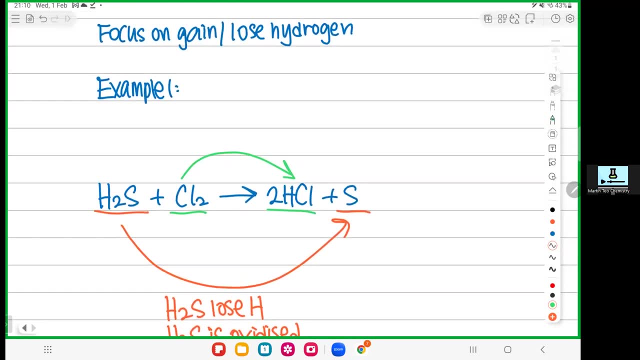 Does it make sense? Makes sense. ma Here the Cl got nothing. Here the Cl got hydrogen. So you can see already, On the left-hand side the chlorine don't have hydrogen. On the right-hand side, the chlorine got hydrogen. 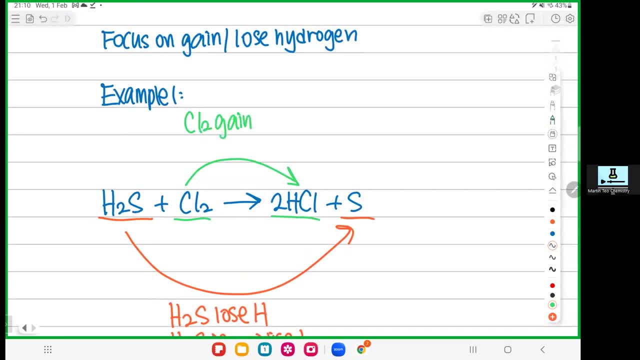 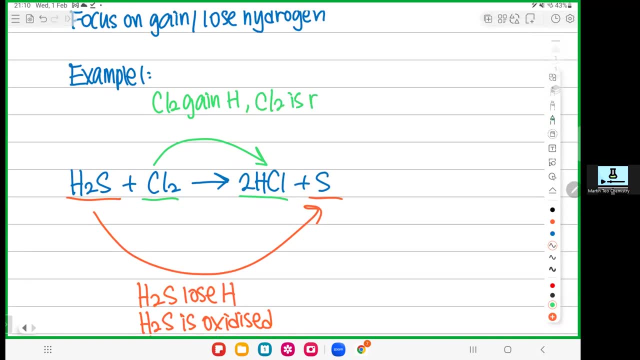 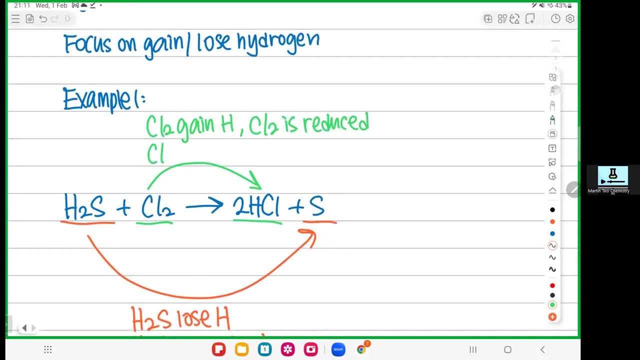 So you can see. look The chlorine here gained hydrogen. So when you gain hydrogen, chlorine undergo oxidation. Okay, Reduction, isn't it? Remember- refer back to the table: Gain hydrogen means reduction. So when you undergo reduction, which agent you are? 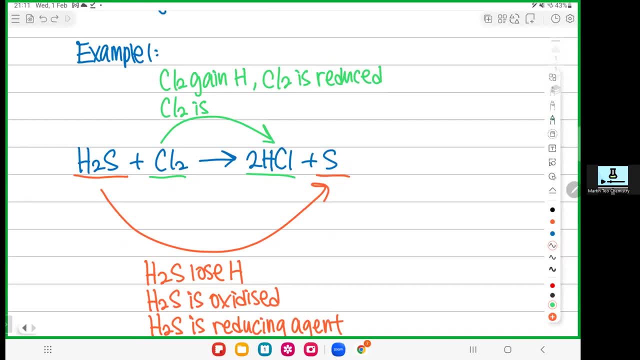 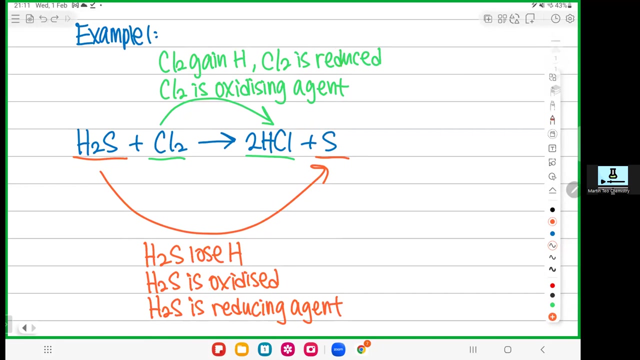 Opposite. So when you undergo reduction you are the opposite agent. So you are oxidizing agent. End of story. Is this a redox reaction? Yes, Because I have reduction, I have oxidation, Redox. Okay, So when oxidation and reduction process happens at the same time, then it is a redox process. 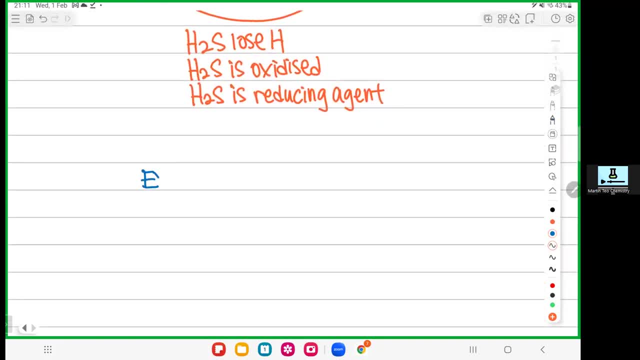 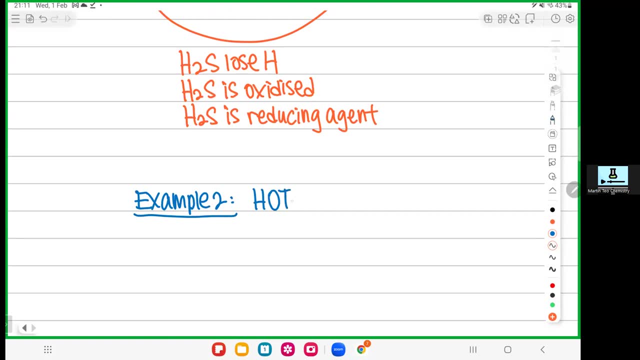 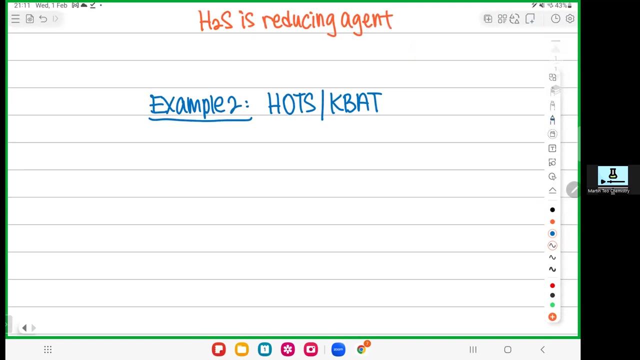 Okay, Let me give you another example. Let's have a look. Okay, So here is the problem. So you have hydrogen in Bm, The Mahiran Perficir Aras Tinggi. Okay, So higher order thinking, critical thinking question. 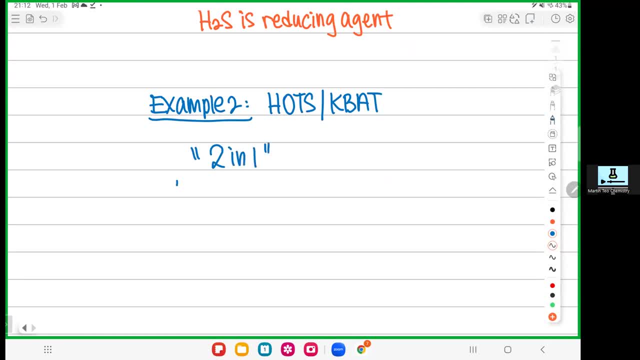 Okay, So how am I going to make this question become a K-Bud question? Okay So, K-Bud question, they can do something called two in one. So two in one means that they can combine oxygen method. They can combine the oxygen method as per the oxygen method. 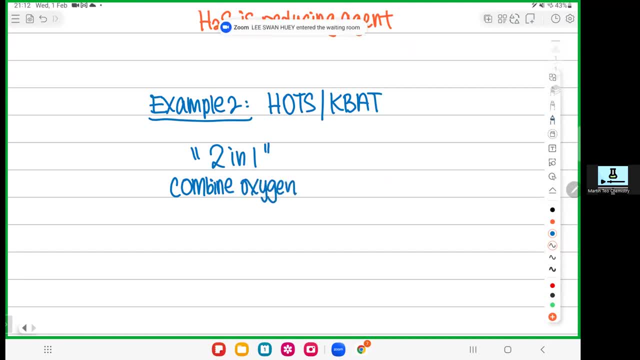 So two in one means that they can combine oxygen method. They can combine the oxygen method as per the oxygen method, Okay, as well as they can combine hydrogen method. so this is special because just now, if you remember, all the example we use is purely oxygen method or purely hydrogen method. but now they can make 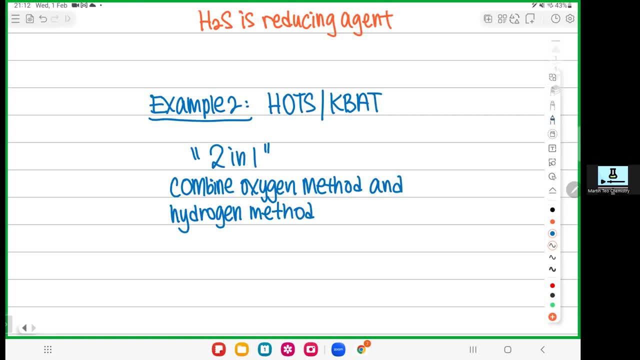 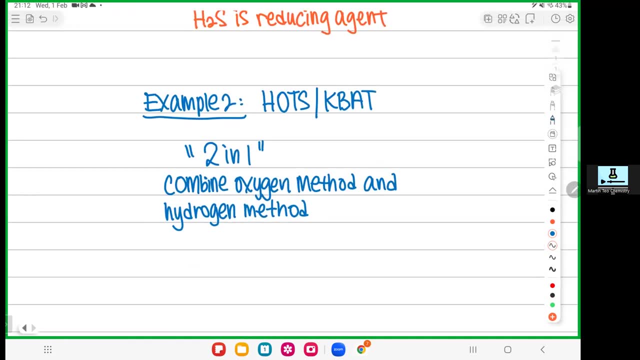 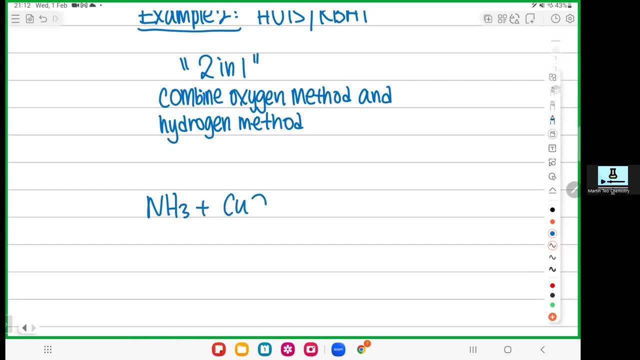 it become a k-butt whereby we will use both two method all come in together. no worry, no panic, just do as usual. just do it as usual, okay, all right, let's say we have this: ammonia react with copper oxide, become a nitrogen gas, water and copper. okay, so no worry, okay, just follow my. 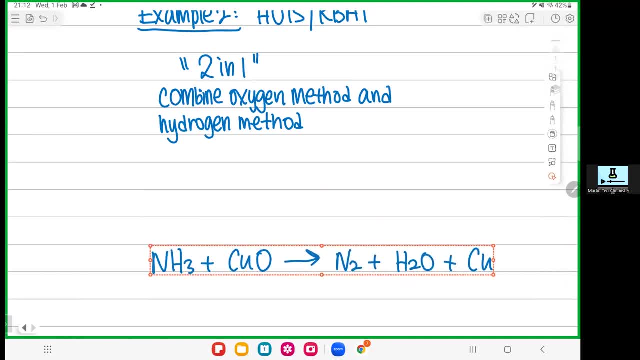 my lead. okay, i'll lead you. i'll teach you what to do. so, first and foremost, before you do apple and apple comparison, don't be so excited yet. always, always make sure when you have a chemical reaction, the first ever thing you need to do is what balance it always remember. 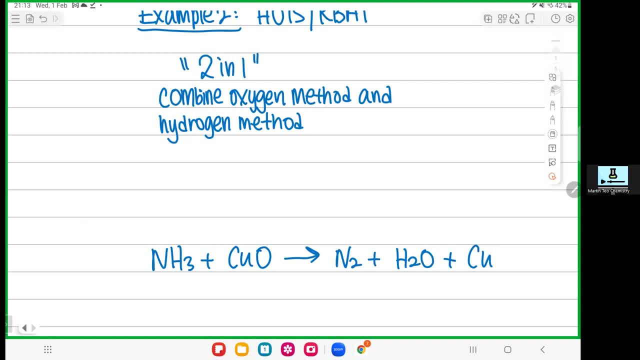 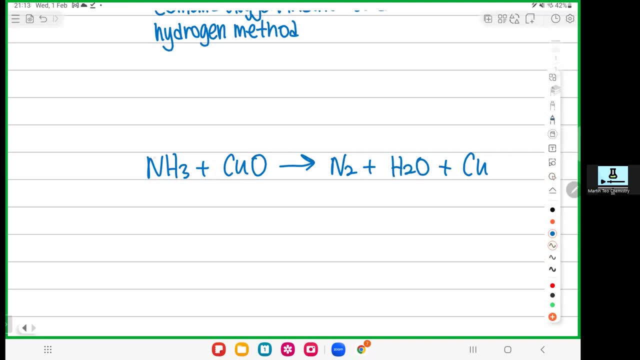 whenever you get a chemical reaction, just balance it before balance the equation. don't ever do your apple and apple comparison. okay, so i balance it quickly. yeah, let me, let me balance it. two, three, three. that's right. two, three, three, three. yeah, so you can balance yourself. 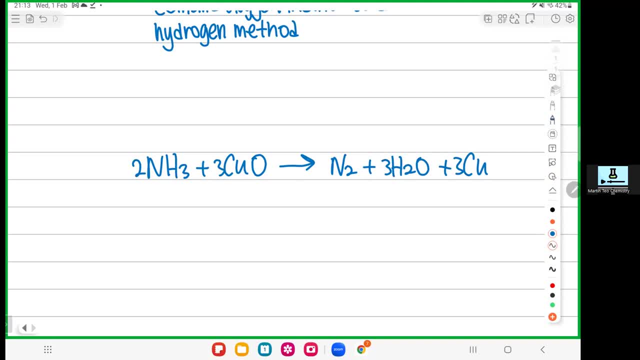 so now let's choose the apple to compare, let's choose the apple and apple to compare. so let's say, i choose one apple on the left. okay, so we choose one level on the left. so tell me, guys, this apple on the left i should compare with who? 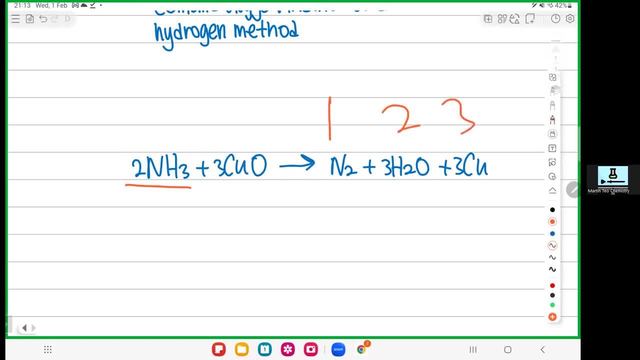 one, two or three. if i choose ammonia on the left, i should compare with who? one, two or three, okay, very good. okay, very good, i should compare with number one. yeah, i should compare with number one. uh, make sense, this nitrogen sticking with hydrogen, this nitrogen not sticking with hydrogen. 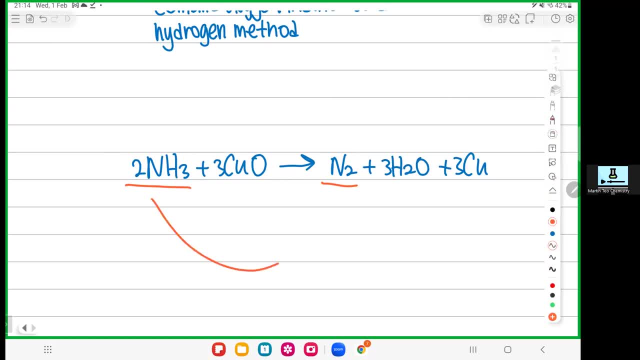 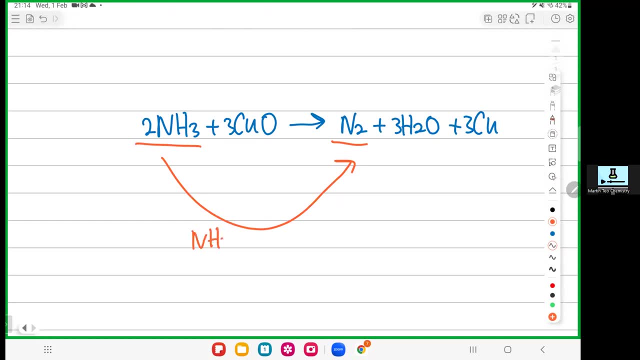 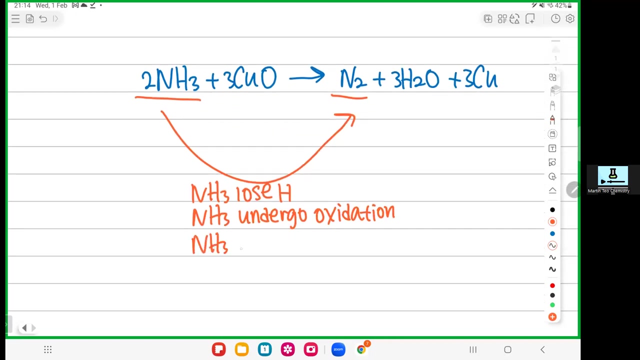 so obviously you know which method you need to use: hydrogen method, isn't it? so ammonia is actually losing hydrogen. so, loose hydrogen, what process is happening? oxidation, right, loose hydrogen is oxidation process. when oxidation process take place, you will be the opposite agent. you are reducing agent. okay, you are reducing. 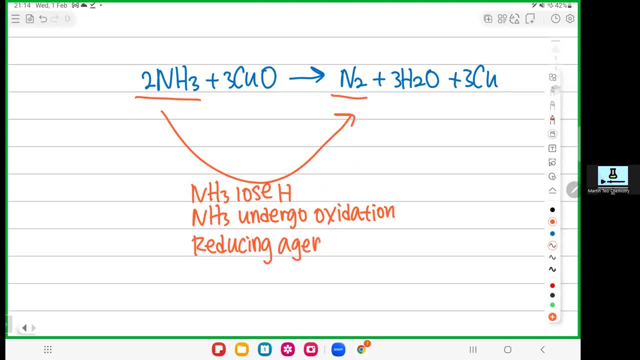 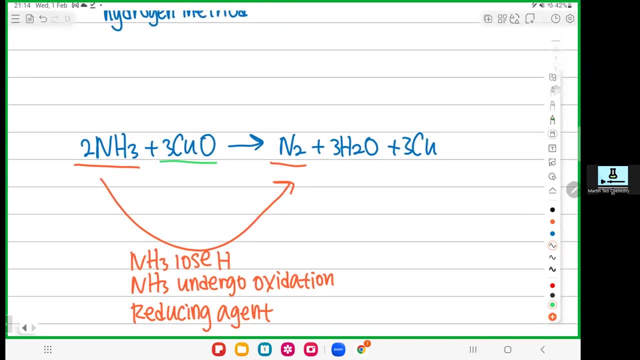 agent and of storing. now let's choose another apple to do comparison: green apple copper oxide. now i want to compare with who? one or two copper oxide, who i compare one or two? okay, let me see the chat box first. okay, very good, okay, duncan, haida, zoe, eliza, ying chi, cynthia. 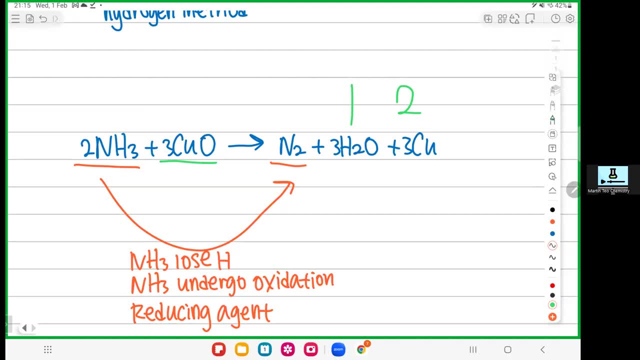 jianni, okay, xing ning, okay, very good, compare with two. so that's what i say. you must know which apple you should compare. that's the most and basic thing. okay, you choose the right apple. you won't get wrong, la right, unless you're callous. so, copper, so come to here. okay, remember, left to right, not right. 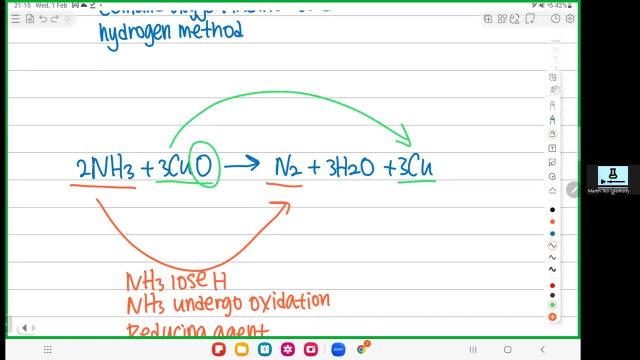 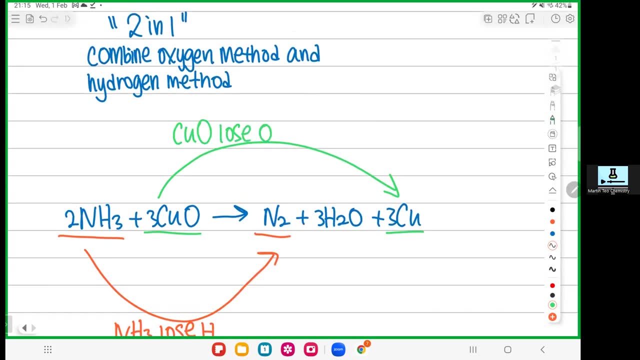 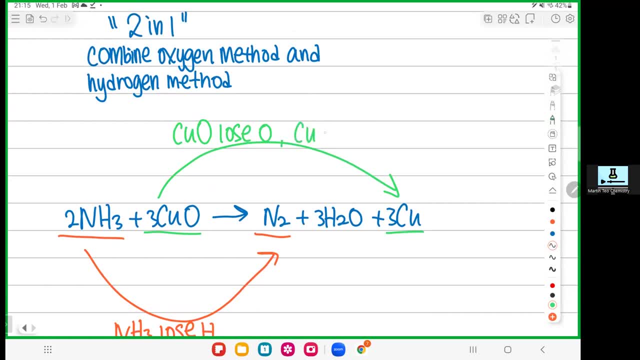 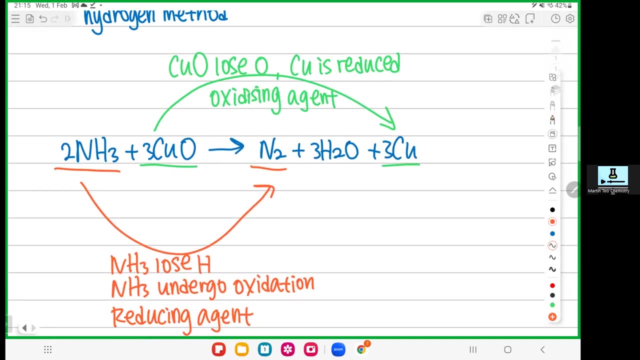 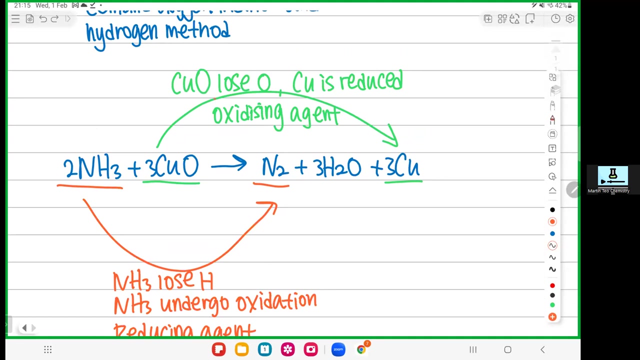 oxygen method. lose oxygen is reduction, isn't it okay, reduction. so when you undergo reduction, you are opposite oxidizing agent. okay, that's it all right, simple as that. so you see, this one, i not even need to purposely do it. you see, this is hydrogen method, this is oxygen method. i not. 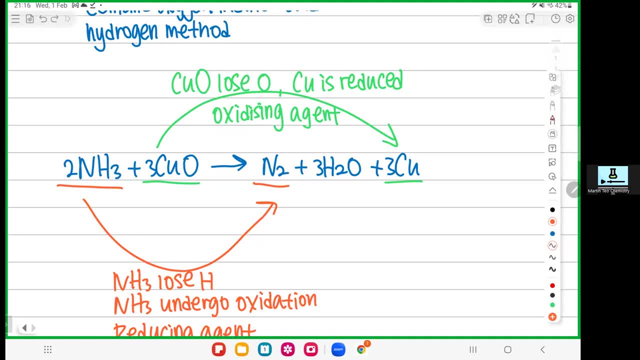 even need to purposely think about it, i just choose the right apple. i see, hey, this one, the oxygen disappear oxygen method. in this one, the hydrogen disappear, hydrogen method. i not even need to purposely memorize, i follow the flow naturally. i follow the flow naturally and i get. 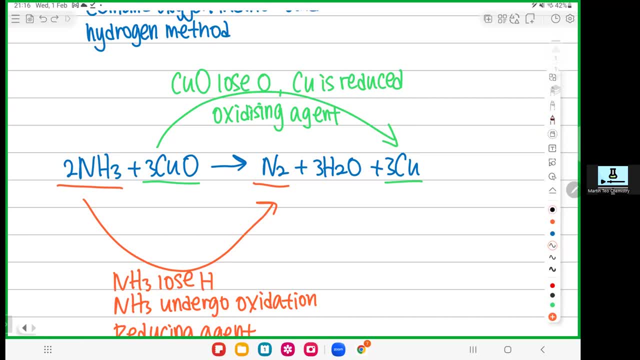 answer already as simple as that. there's. some people will say: mr martin, this fellow, we haven't used well this copper oxide, nothing more. well, just now, i only tell you you need to choose one apple on the left and compare with the apple on the right. i didn't say you must use all the 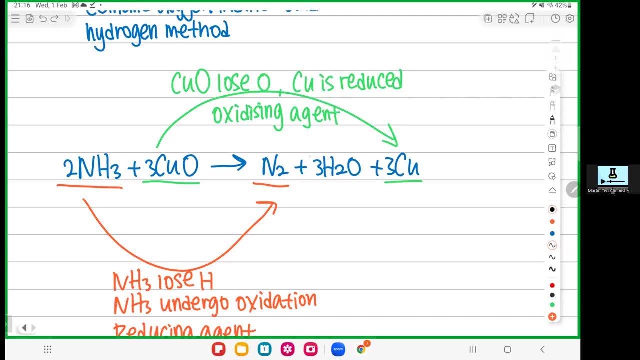 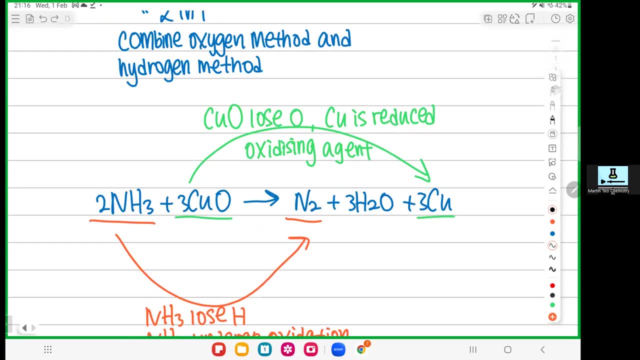 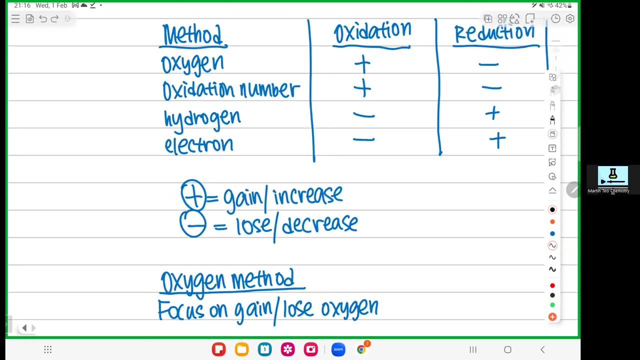 apple, right? uh, some of the apple. you don't want to use it. it's okay, not to say you must use all the apple one, it's okay, all right. so with that being said, we are all done with hydrogen method. we are done with hydrogen method already. okay, so the pace is quite good so far. so we have managed. 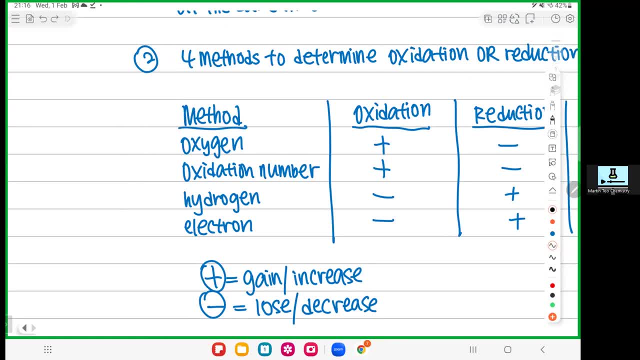 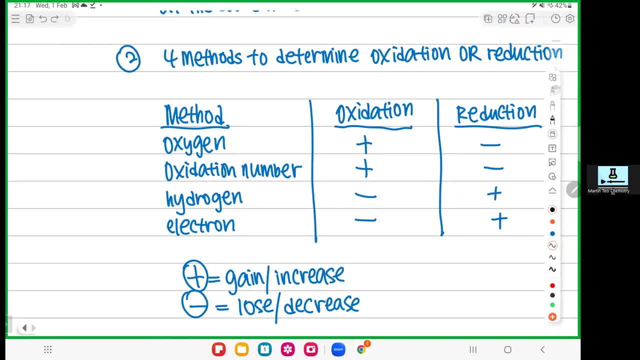 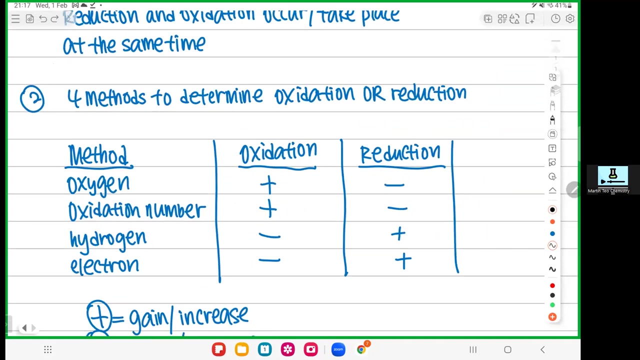 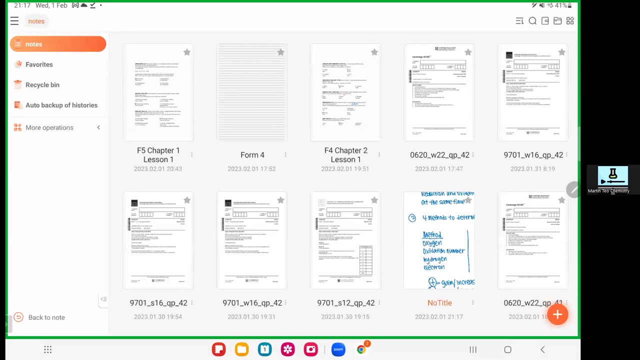 to complete two methods. okay, guys, let me know in the chat box how's everything. how's everything okay, not very hard, not very hard. can i? okay, can do la, all right, so not very hard, okay, it's actually doable okay. it's very, very doable, okay. so if you really understand, you follow the logic. 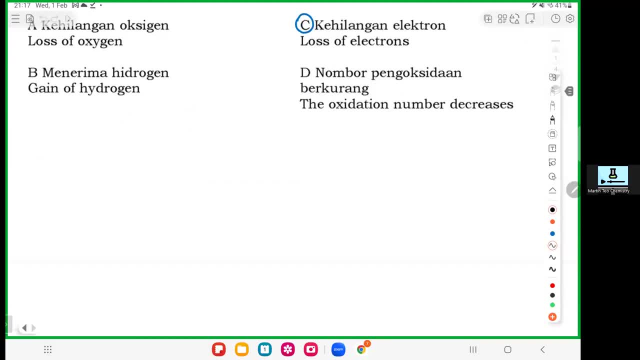 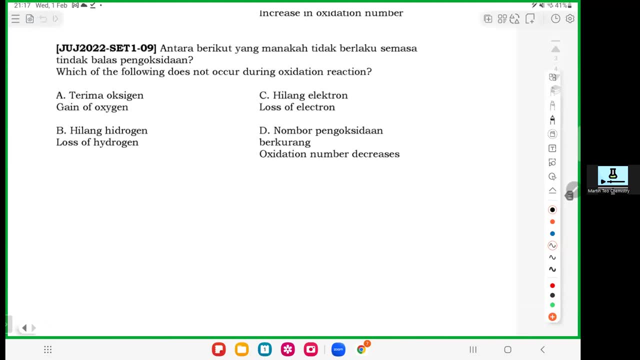 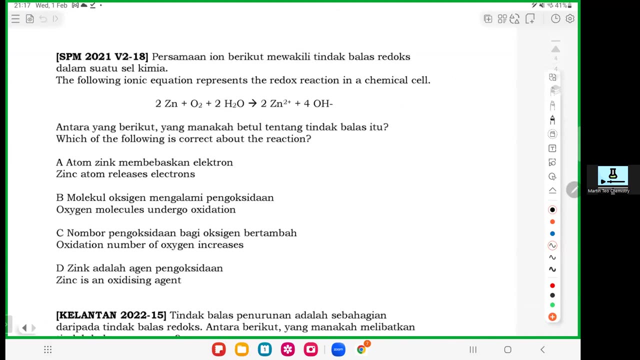 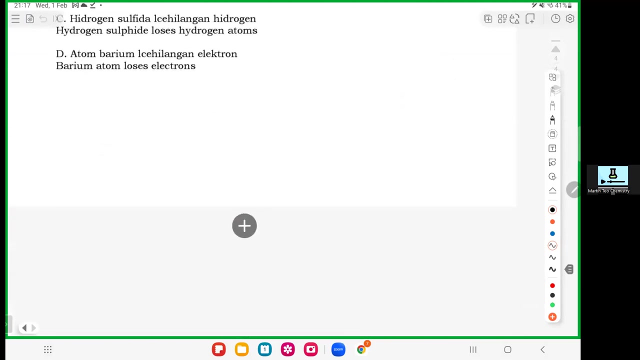 it's not that hard, okay, all right. so let's see. okay, any questions i can do with you. okay, any question here. all right, so, okay, here, here, here here. okay, this one oxidation number later, okay, okay, all right. so now i'll teach you the third method, which is the. 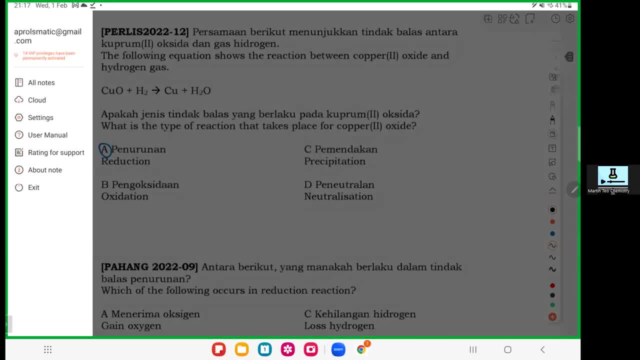 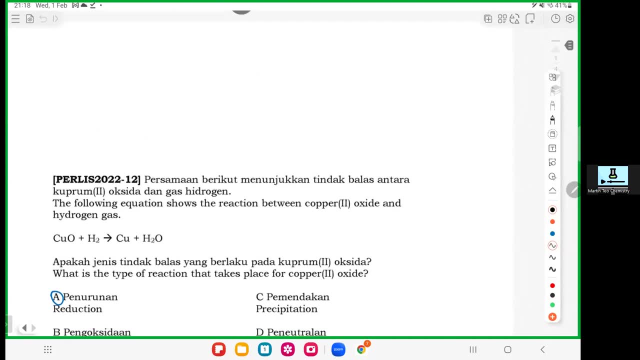 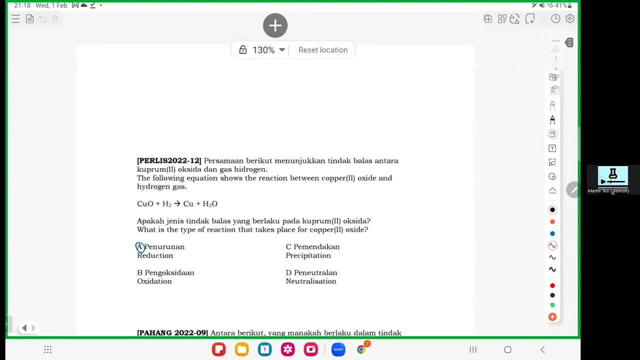 most tricky method, okay, which is a super, super technical method. okay, we will try to finish it very slow. if i cannot finish today, never mind, okay, i'll finish it next week, okay, but this is very important. that's why i'm going to go very slow, huh, okay. so now let's do it. 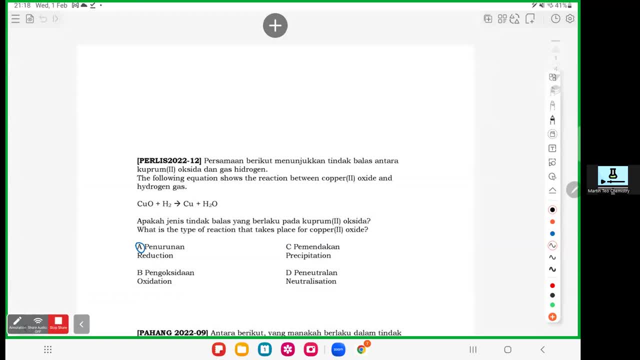 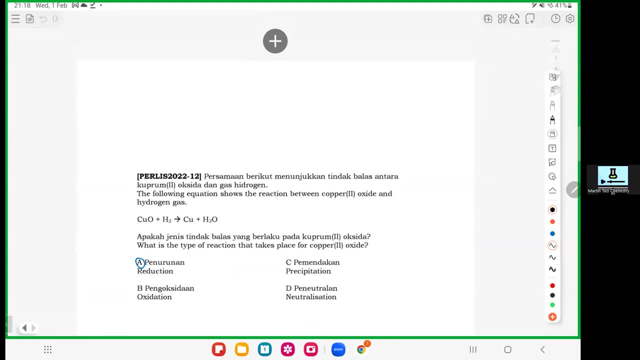 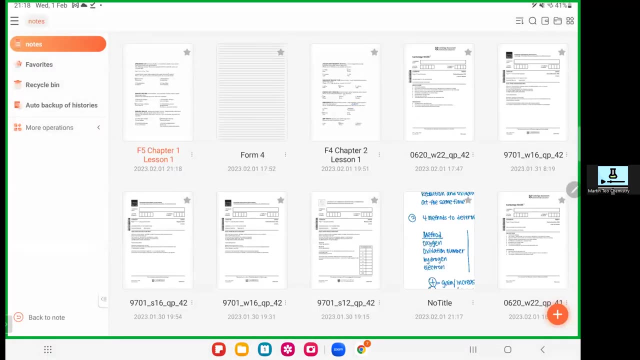 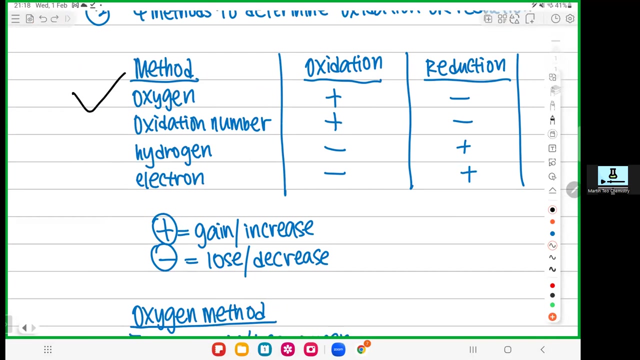 okay, okay, okay, this is very, very technical. okay, i want to, hopefully, okay, i can. i can teach in a way that most of you can understand. if, let's say, after this, you still don't understand, you can watch back the playback of the video. if you still don't understand, feel free to ask me anytime. yeah, don't be shy, ask. 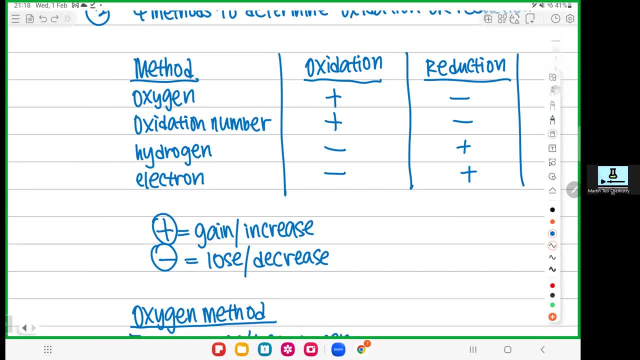 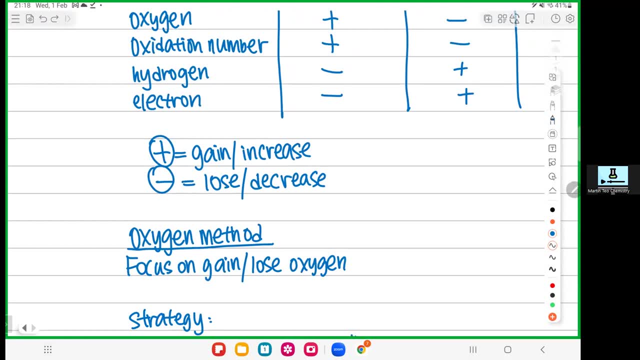 me. please ask me if you're not sure. okay, so now we have completed these two easy methods, so now we are moving toward to these two hard method. so i won't touch electron method, for sure today. right, i will only touch oxidation number method. okay, so this is very, very technical. okay, i want to hopefully. 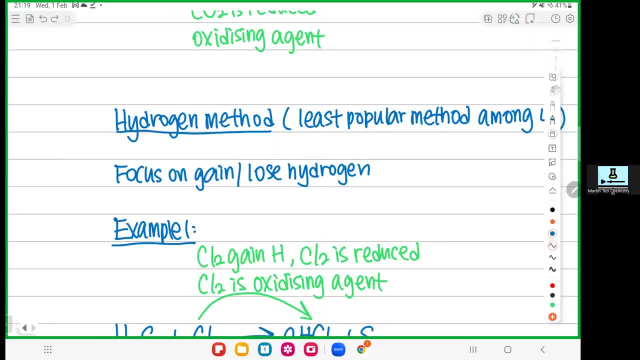 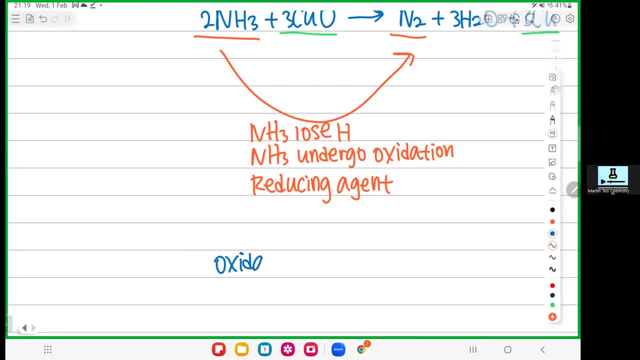 ask me if you're not sure. so now let's look at the heart method already. yeah, so the heart method we need to learn is called oxidation method, oxidation number method. okay, so oxidation number method. okay, this is a very popular method in spm. super duper, popular, super duper. 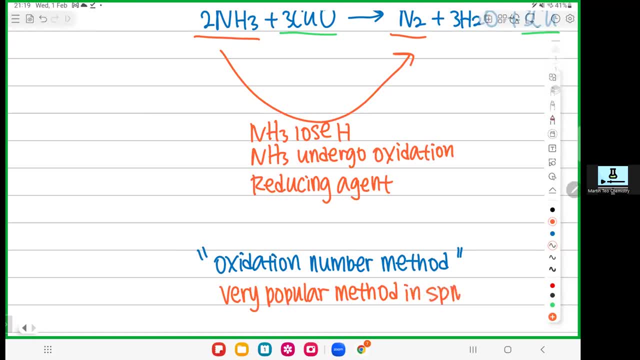 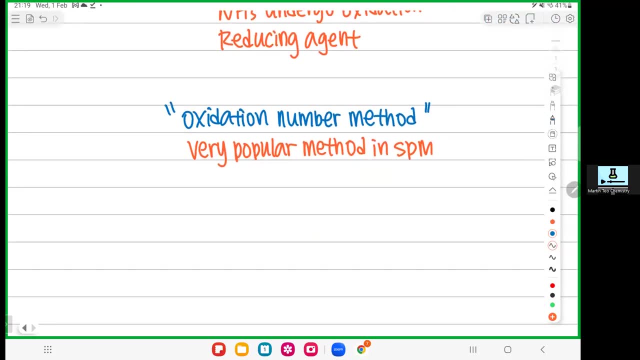 popular in spm, uh, okay. so when you come to oxidation number method, okay, so i will teach you two things that today. i want to teach you a few things first. okay, first of all, i want to teach you this: okay, there are total four rules to determine the oxidation number. okay, so you need. 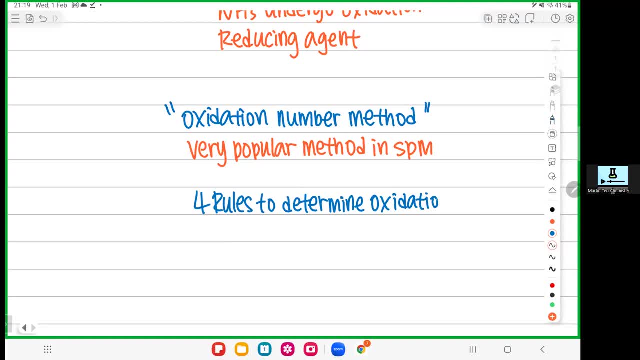 to know what is oxidation number and how to get it. how are we going to find the oxidation number for a substance? okay, hopefully, in about 20 minutes time, whenever i give you a substance, you will be able to tell me the oxidation number for that particular substance. i repeat, uh, hopefully in 20. 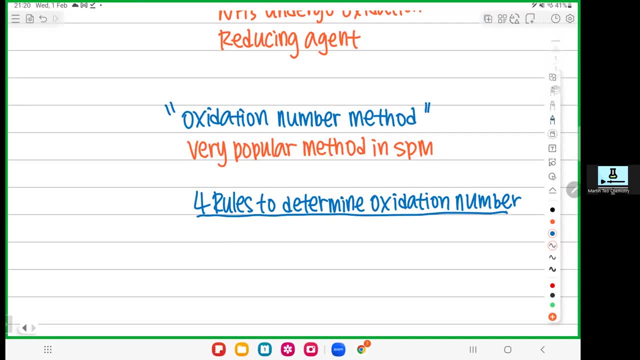 minutes time. okay, whenever i give you the oxy, i give you a substance, you will be able to tell me, okay, what is the oxidation number of that particular substance. okay, so let's start. okay, so there are total four rules. okay, i will go through one by one. i will gonna give you a lot. 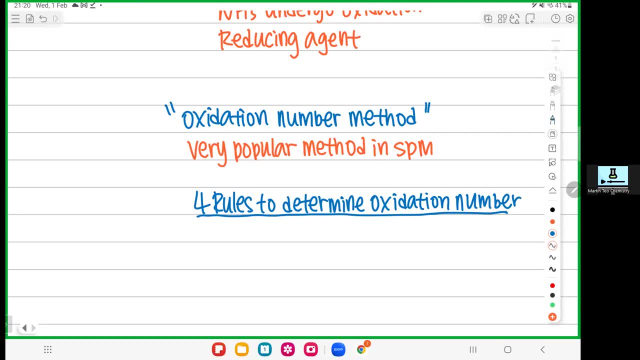 of examples so that you can apply. you can apply whatever things that i want to tell you now. okay. so, rule number one: okay, the rule number one. okay, just a moment, just one minute. okay, all right now. so why oxidation number method is so popular? okay, why oxidation number method is so popular? because oxygen number method can use for all the cases. 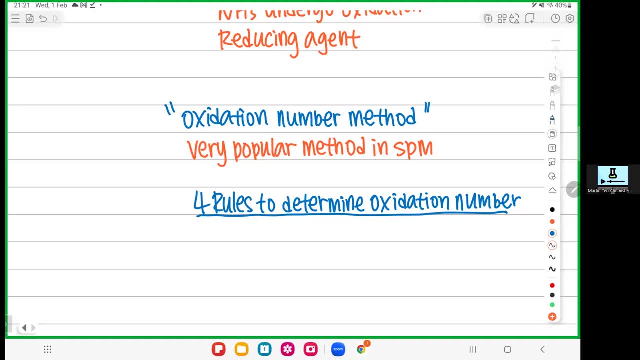 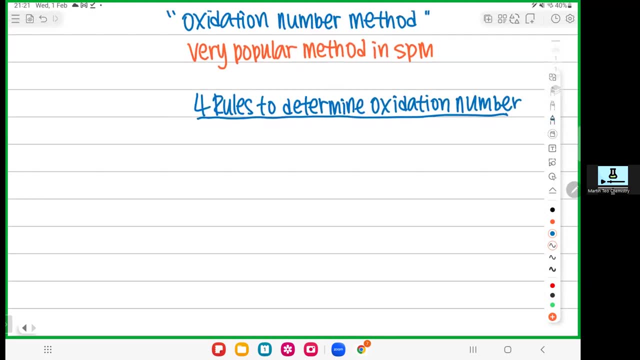 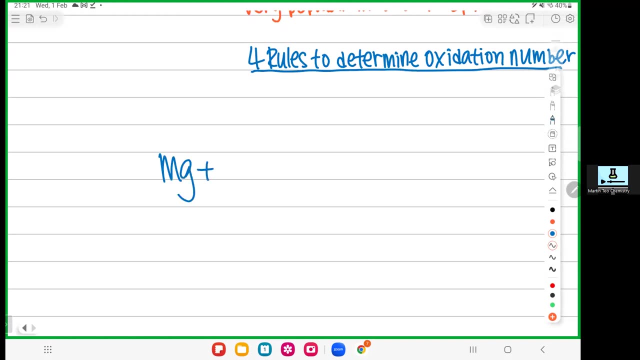 every single case can use. okay, like oxygen method: can only use if the question got oxygen. hydrogen method: can only use if the question got hydrogen. let's say: you see, guys, let's say i give you something. it is magnesium plus. okay, uh, uh, this magnesium plus uh. 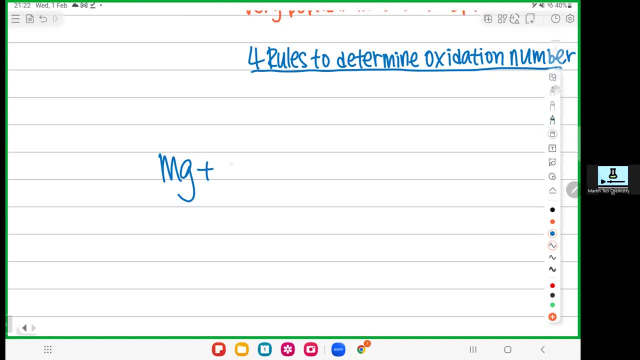 hydrochloric acid become magnesium chloride and hydrogen, or maybe i'll go for another one. okay, let's say this one: sodium plus chlorine becomes sodium chloride. do you think we can use oxygen matter in this question, yes or no? can we use oxygen matter in this question? 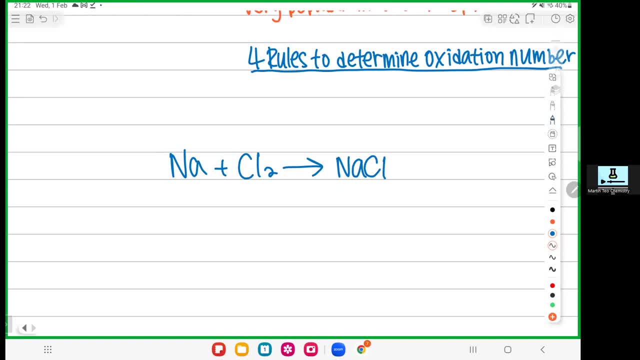 no right, okay. can we use hydrogen method in this question? yes or no? can we use hydrogen matter in this question? no, right, you see that. so oxygen and hydrogen method, they are quite easy, but they has they have a weakness. okay, many, many case cannot use if the question don't have oxygen, if the question don't have oxygen. 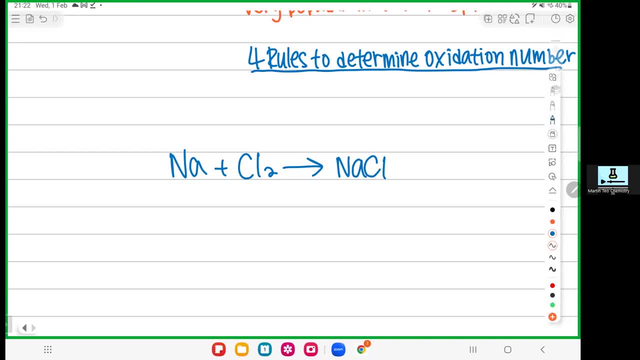 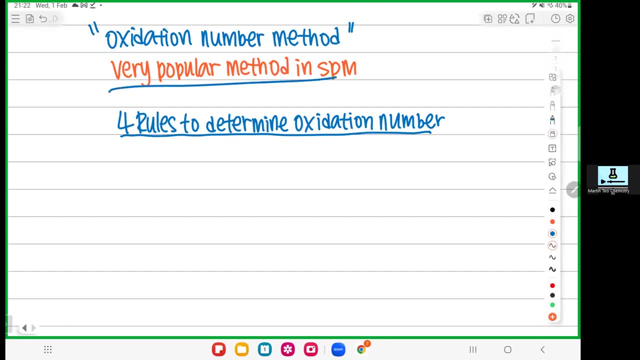 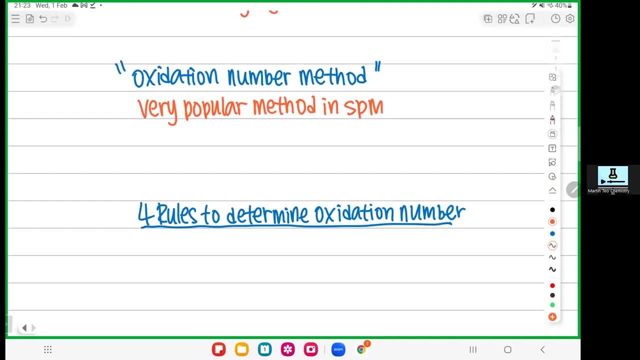 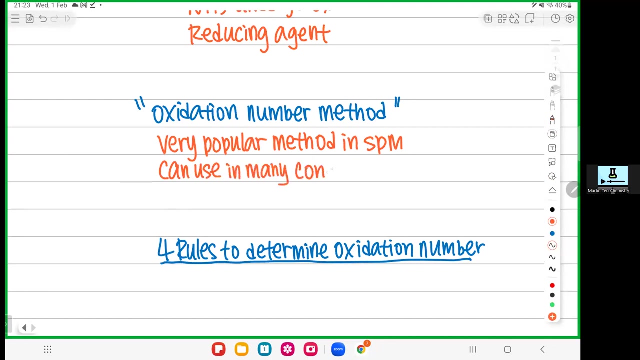 that cannot use already. okay, mixed well your skin. okay, you can use in all situations. okay, because you open your mouth, you can use it. uh, take a drink, you can use it outside. okay, because that matters. okay, because you can use it in all situations. okay, you can use in many conditions or many situations. 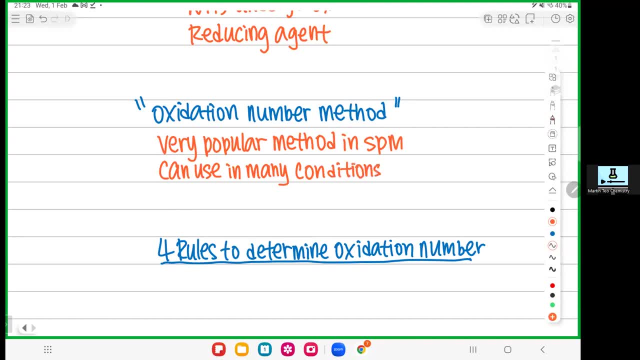 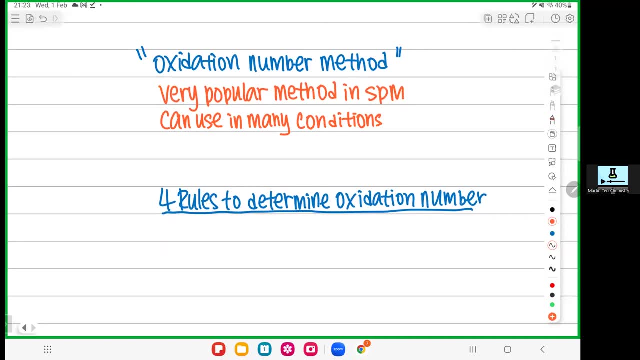 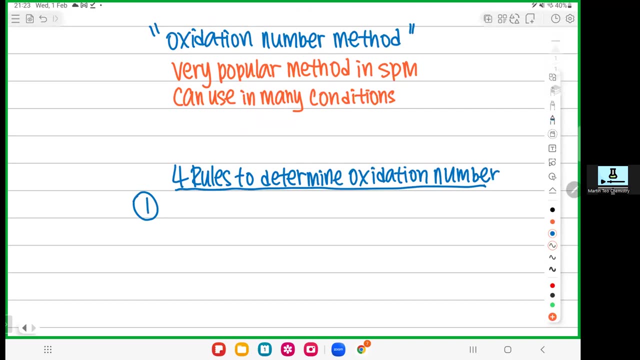 no matter the question got oxygen or not, no matter the question got hydrogen or not, oxidation method can be used. okay, you can use oxidation number method. okay, so let's look at rule number one. okay, rule number one. you need to know that the oxidation number of: okay. the oxidation number for element: okay, oxidation number for element. 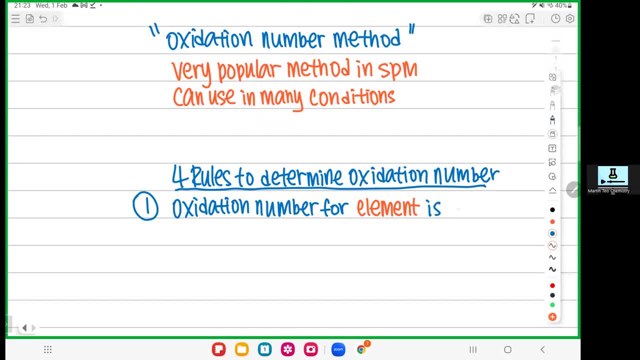 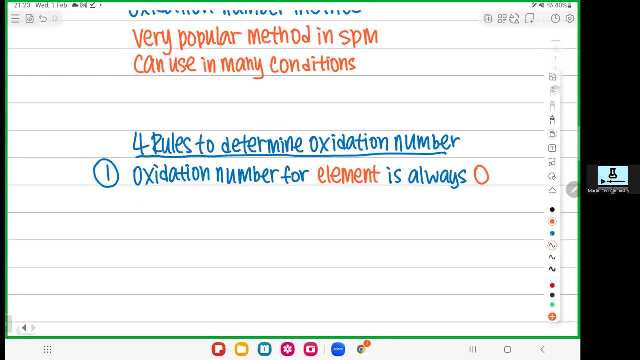 okay. it's always always zero, so oxidation number for elements is always always zero. Allow me to ask a simple question here. Allow me to ask a simple question here, guys, Anyone of you here don't know what is element. Anyone of you don't know what is element If you don't know what is element. 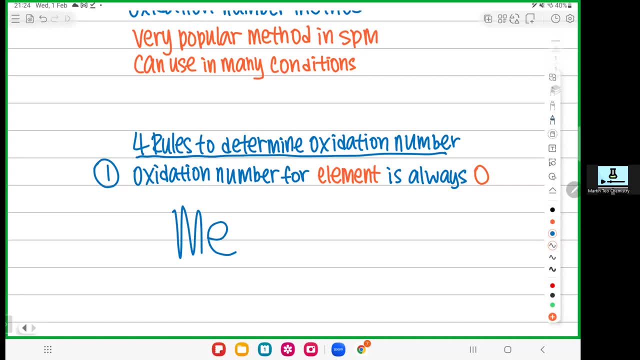 can you type me? If you don't know what is element, can you type me for me? M-E. Okay, let me teach. okay, Element is something you learn in from 4, chapter 2.. Okay, from 4, chapter 2 are element. So what? 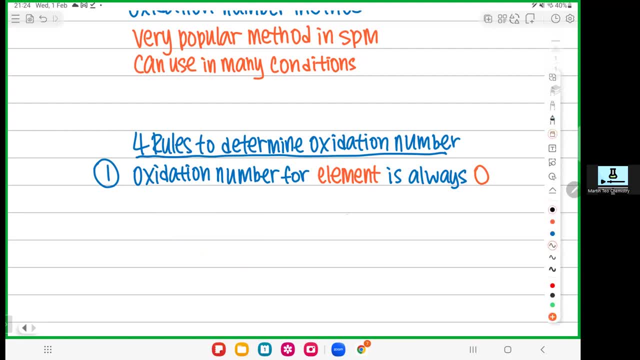 is element. Element is referred to anything that is made of one species. okay, So anything that is only made of one species. Okay, what do you mean? one species? okay, For example. let me give you a few examples. okay, 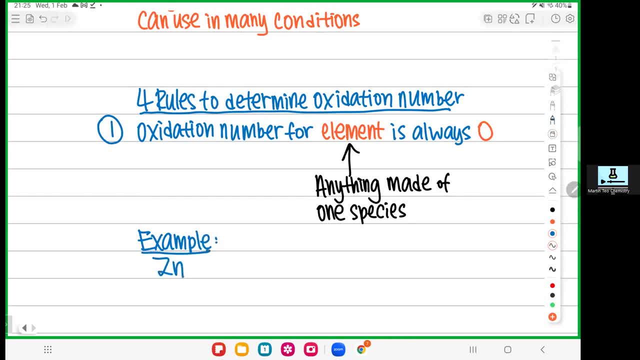 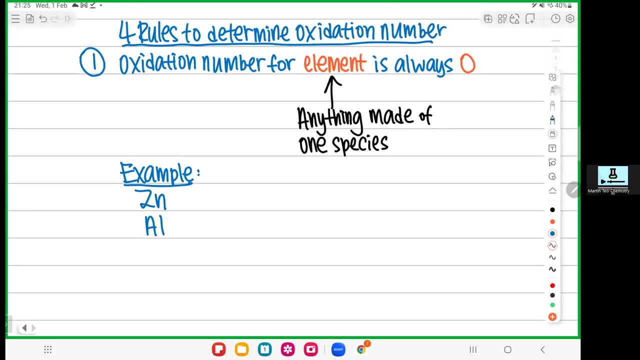 Zinc is an element, because only one species, right, Only one type of substance here. zinc Aluminium is only one type of substance: Aluminium, only nothing else. So it's one type of substance, One species only is element O2, oxygen. 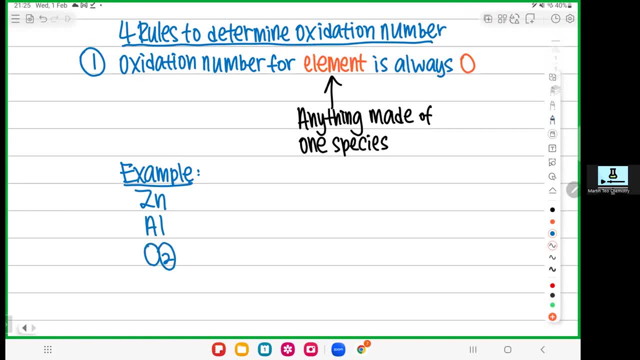 Don't get cheated by 2. Although you have 2 filler, but both of them are O, They are same species, right? Both of them are O. You only have one type, One type of substance, So they are element, Let's say sulfur. 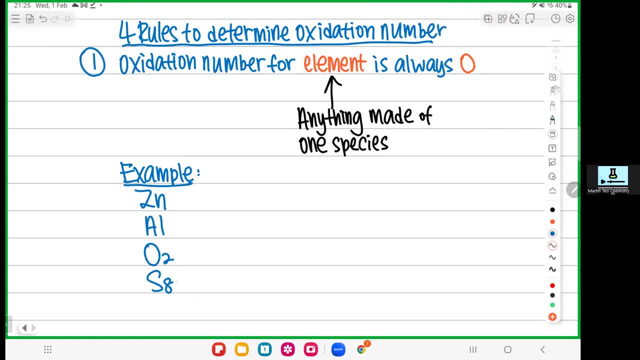 S8.. Don't get cheated by number 8. Although you have 8 filler, but all the 8 substance, all the 8 substances, they are sulfur. All of them are same species, So they are element. So, as long as you have, 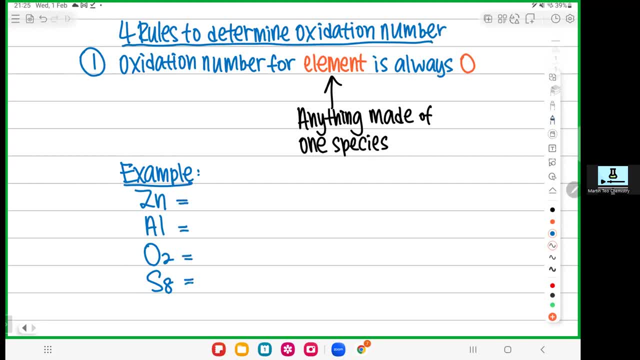 element. all their oxidation number is 0.. Okay, So when you have element, the oxidation number is 0.. So you all must know what is element: Anything that is made of one species only, So that is element. So, guys, 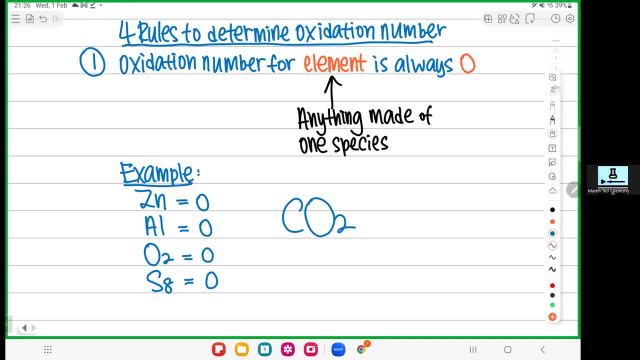 carbon dioxide: is it element, Yes or no? Carbon dioxide: is it an element, Yes or no? No, ah, Because you got carbon, you got oxygen. you have 2 elements, You have 2 species, So you are not element. 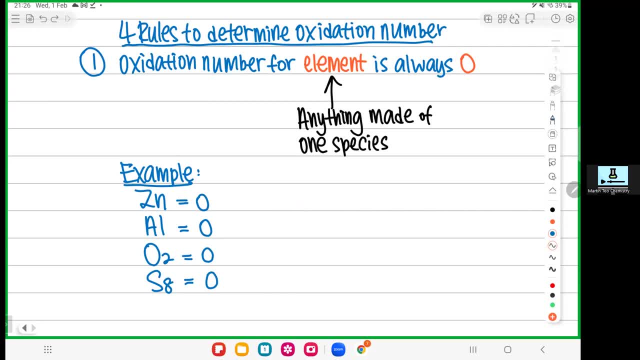 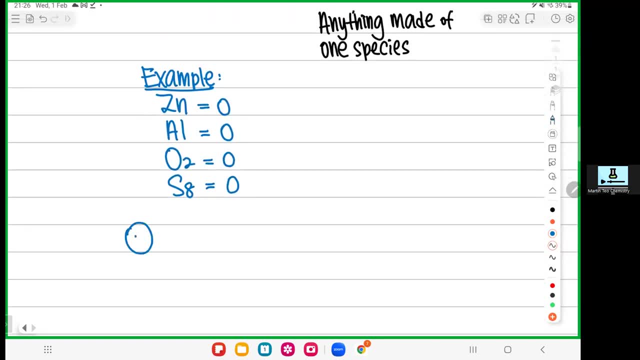 Alright, So element must have only 1 species. Okay, So that's it. So if you have element, the oxidation number will automatically become 0.. Okay, Rule number 2.. Okay, Rule number 2, ah, Okay. 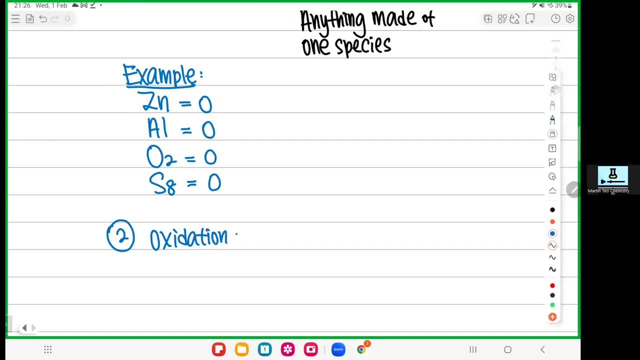 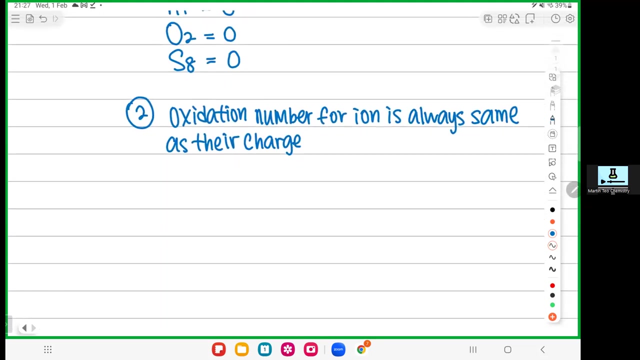 Oxidation number for ion. it's always same as the. ah, Okay, Charges, Okay. Oxidation number of ion is always same as their charge, Okay. So what is ion? Anything got charge. So if you know anything, got charge the. 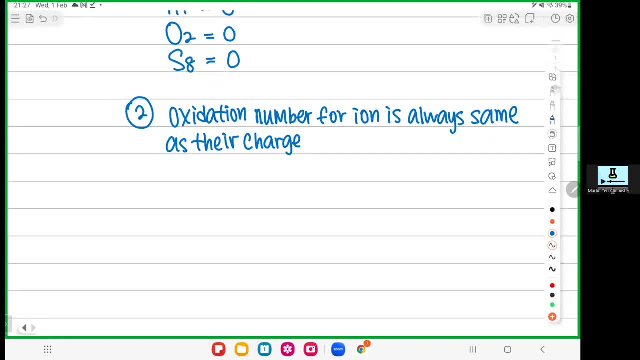 oxidation number is exactly same as their charge. Example: you have Na plus. Is it ion? Yes, because you got charge. So Na plus got charge is ion. So for ion the oxidation number is same as the charge, So it's positive. 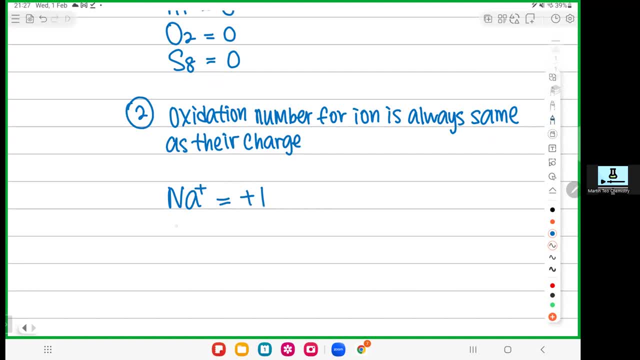 1. Okay, So let's say aluminium, Al3, plus What is the oxidation number. Copy back the charge Plus 3. So, guys, here you have to be very careful. ah, Here you have to be very careful. 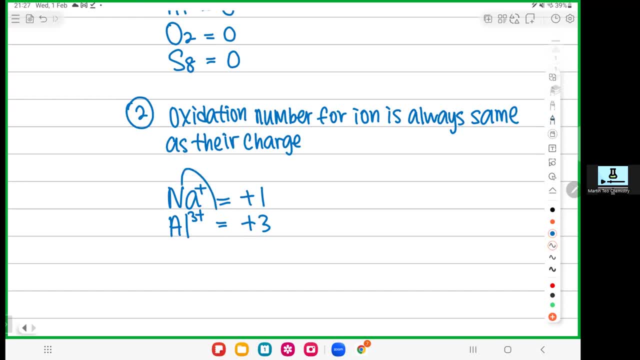 When you go for charge in chemistry, when you write charge, ah, you write the number, then only the sign. Isn't it Like oxygen O2 minus? You don't write O minus 2.. You write the number first. 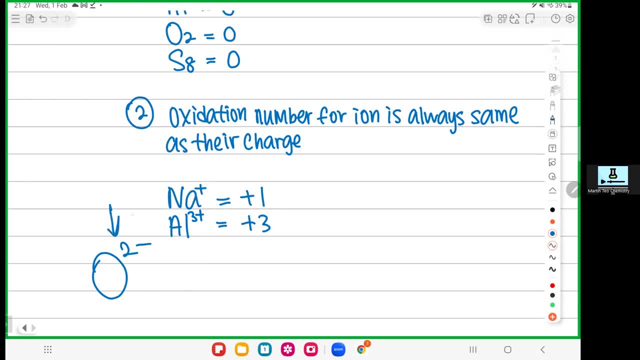 Then only the charge. So charge: you always write number, then only the sign. But when you come to oxidation number, just like normal number, you must write the sign first, then only the number. Okay, So please be careful. ah, So if I ask you, 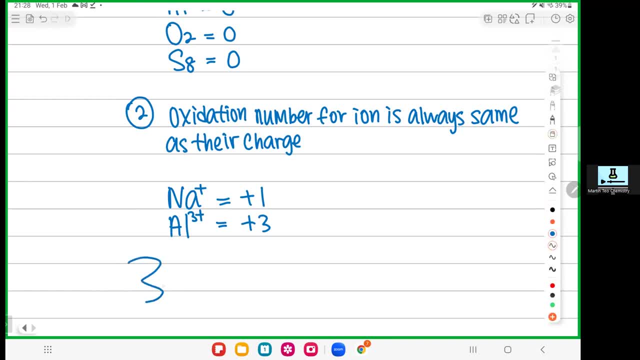 what is the charge for aluminium 3 plus? What is oxidation number for aluminium Plus 3.. So there are some small difference. Okay, So let's say O2 minus, What is the charge? 2 minus? 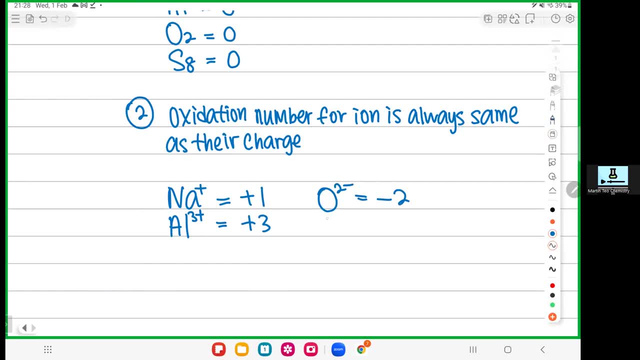 What is the oxidation number Minus 2.. Cl minus: What is the oxidation number Minus 1.. Okay, So make sure you know it. Nitrogen N3 minus. What is the charge? 3 minus. 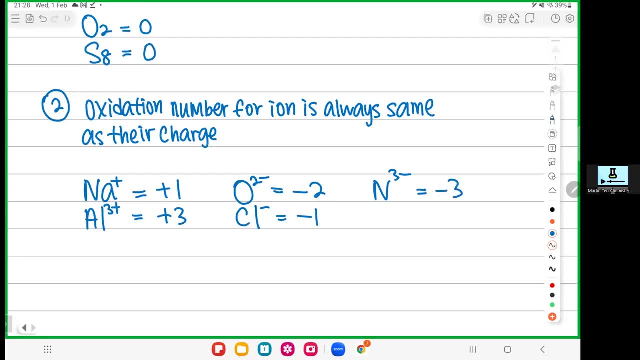 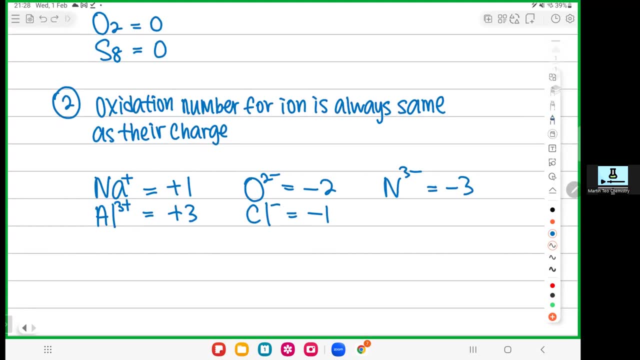 What is the oxidation number Minus 3.. So, guys, can you please let me know in the chat box, which is very important: Do you guys know the difference between charge and oxidation number? Do you guys okay with it? So the arrangement. 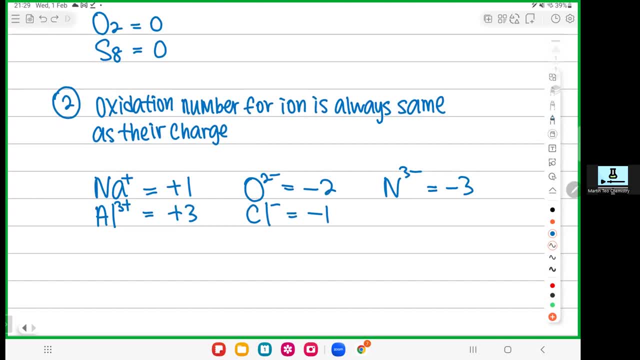 the arrangement is slightly different: Charge 3 plus Oxidation number plus 3.. Okay, And this is very important, because when you do mathematics, when you do mathematics, normally you don't show the sign right, Normally you don't show. 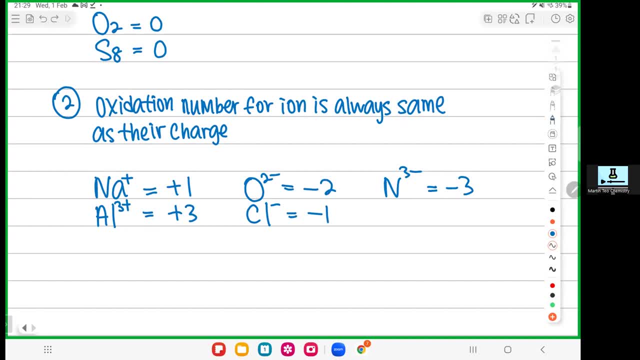 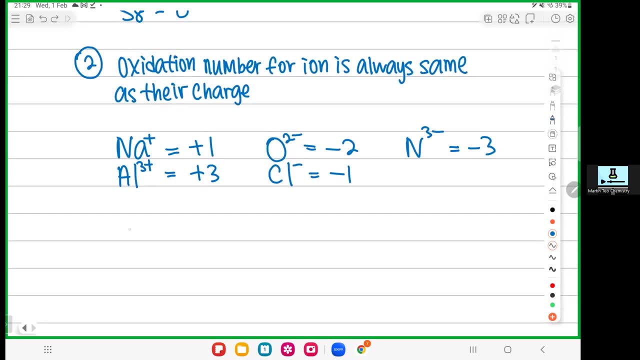 positive sign, isn't it? But when you come to oxidation number, you must show the sign, no matter it's positive or negative. Okay, So this is a tips. Okay, You must show the sign for oxidation number, No matter. 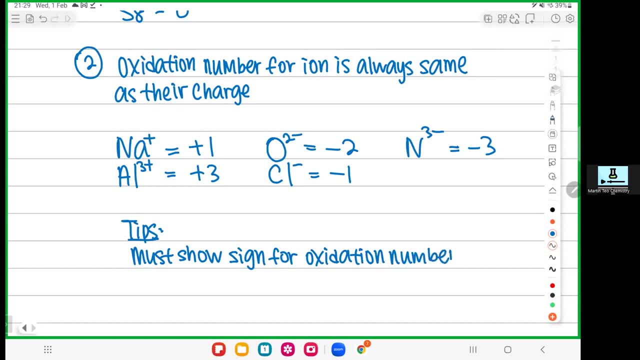 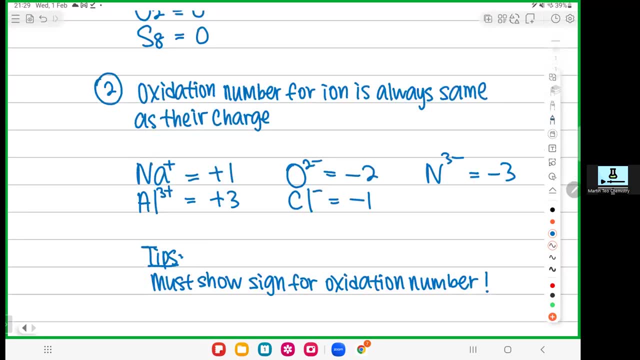 it is positive or negative, Because in mathematics normally we don't show the positive sign, but not for oxidation number. Oxidation number: you must always show the sign. Okay, This is rule number 2.. So now let's look at rule. 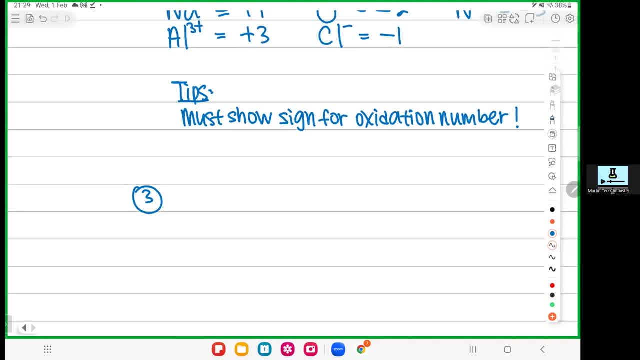 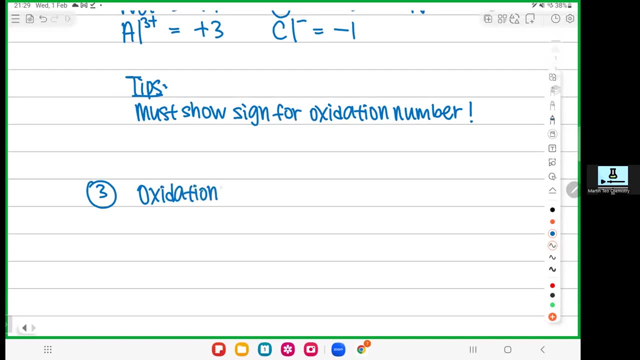 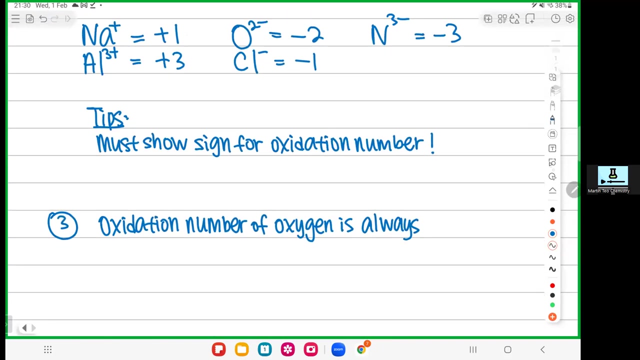 number 3. Okay, So rule number 3. Okay, So now we go for oxygen. Oxidation number of oxygen is always always negative. 2. Okay, Oxidation number for oxygen is always always negative. 2. Okay, Let me change. 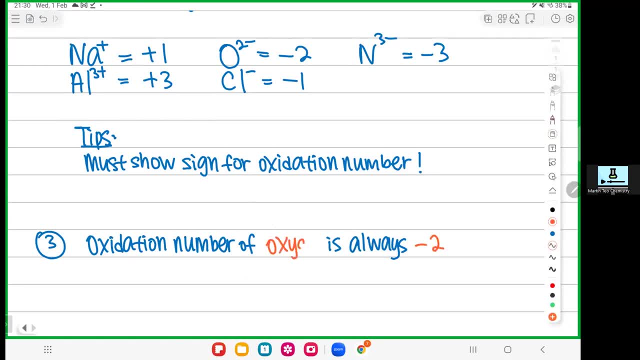 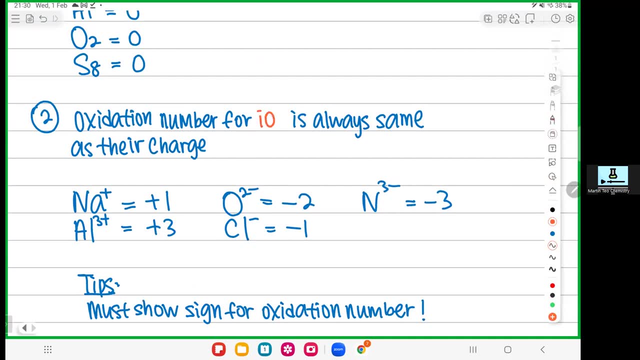 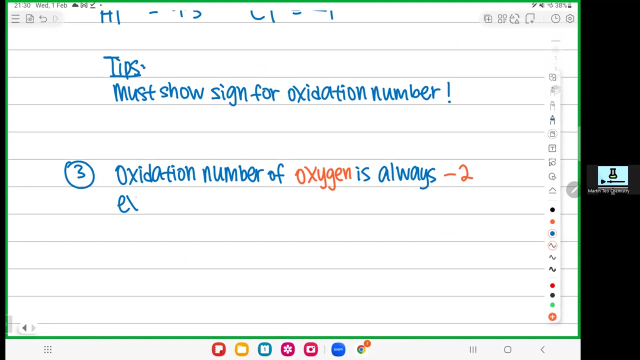 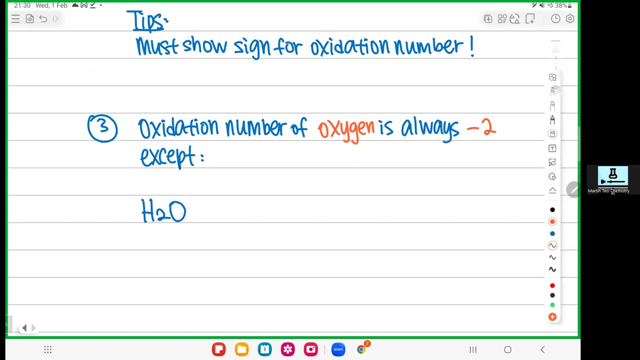 a bit Alright. So the red color is important. Okay, So oxidation number for oxygen is always negative, 2, except a few special case which I'll show later. Okay, Let's say water. Water got oxygen. So the oxygen. 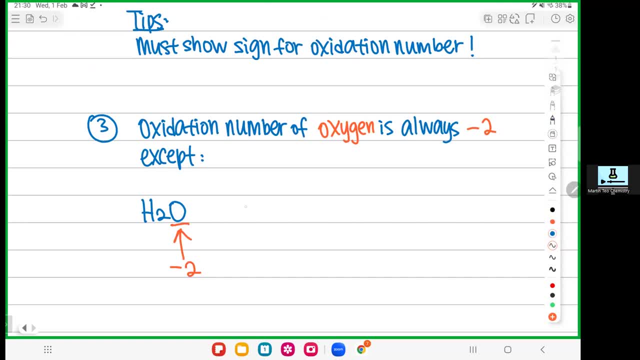 here is negative 2.. Magnesium oxide got oxygen. Oxygen- here is negative 2.. Okay, So let's say we go for something that looks weird: Carbon dioxide. Carbon dioxide got oxygen. So the oxygen here is minus 2.. 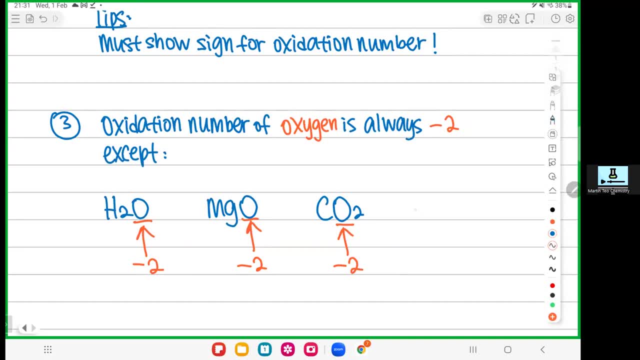 Okay. So let's say aluminium oxide. Aluminium oxide got oxygen. You don't bother how many oxygen it has, You don't bother, you have 1 oxygen, you have 2 oxygen or you have 3 oxygen, Don't bother. 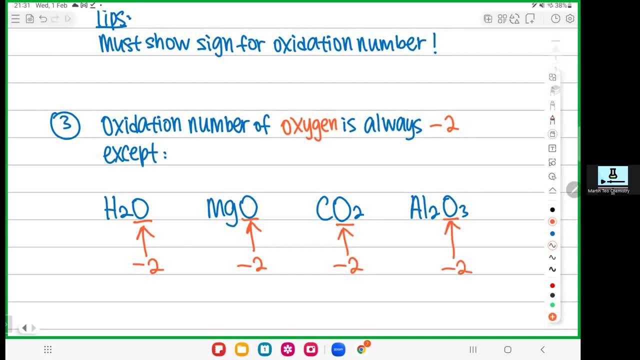 All the oxygen. the oxidation number is minus 2.. That's it. The quantity of oxygen, not important. No matter you have 1,, 2,, 3, or 11 oxygen, it doesn't matter. All the oxygen, the oxidation number. 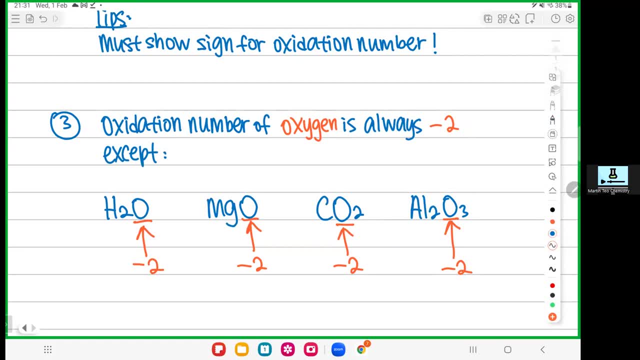 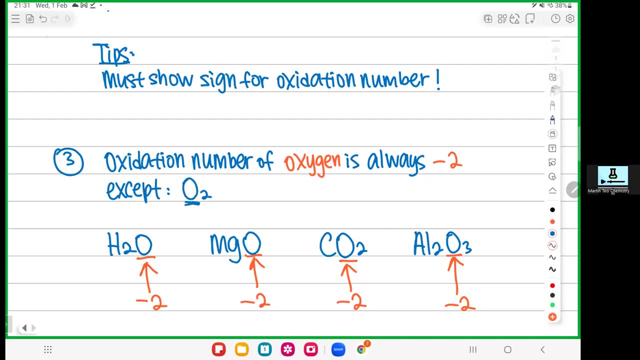 is negative 2.. That's it. So you have 2 special case when you have O2.. When you have O2, what is the oxidation number? O2 only have 1 species, right, So it's element. So that's what we learned today. 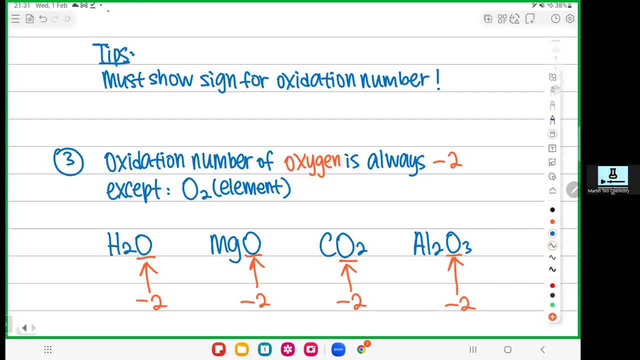 Element: what is the oxidation number? Guys element: what is the oxidation number? We learned just now in rule number 1.. Very good, 0.. Okay, O2, although you have O but it's not negative. 2, because O2 only have. 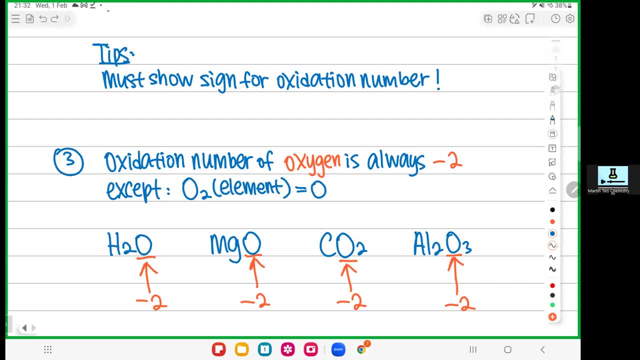 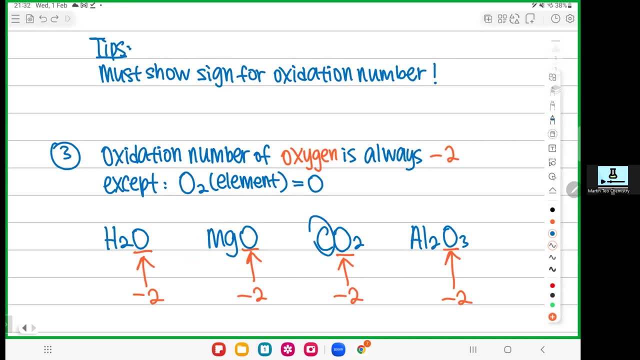 1 species, So it's element Element is 0.. You see just now all the O here combined with something else, The O combined with H, The O combined with MG, The O combined with C, The O combined with aluminium. 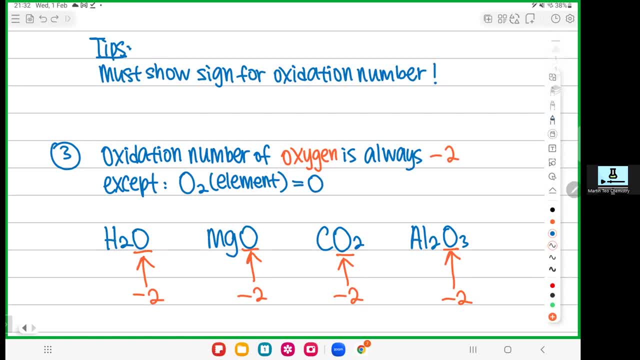 So all these, they are not element. Okay, So when you are not element, the oxidation is always negative, 2. But if the oxygen only come alone, if the oxygen only have 1 species, you are element, Then you are 0.. 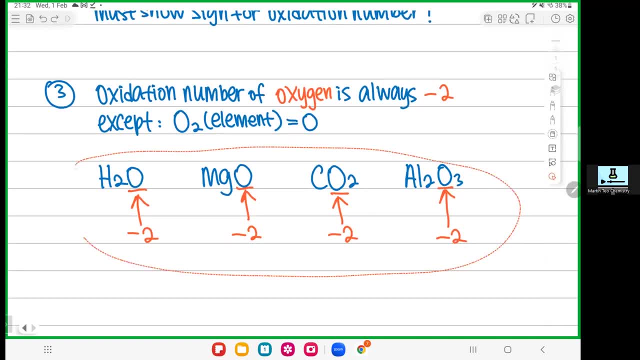 Okay, So you have to be very, very careful. Okay, That's it. Another one which is super rare. They seldom ask in exam For the past 25 years. they only ask 3 times For the past 25 years. they only 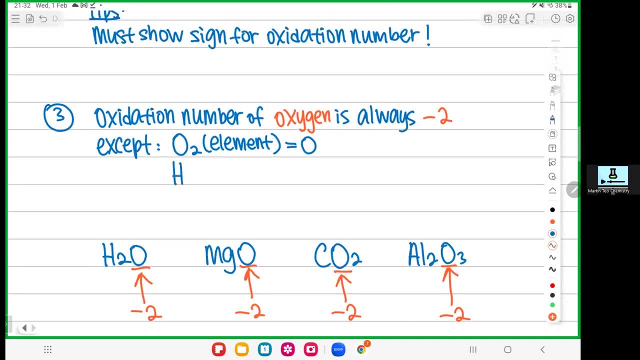 ask 3 times, So not very important- Which is H2O2.. So H2O2, the name is called hydrogen peroxide. If you cannot remember the name, doesn't matter, Doesn't matter. So H2O2, just. 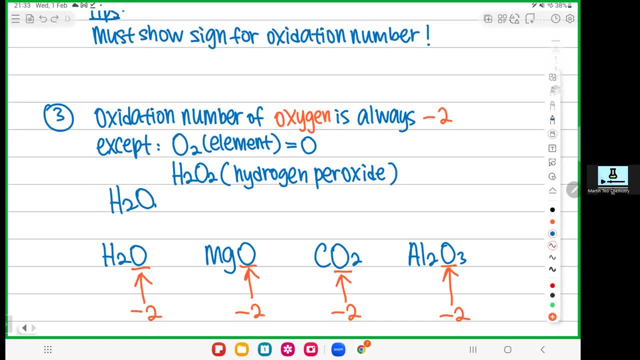 like a water. Water got 1 O. This is water with 1 more O, 2 O. That's it Okay. Hydrogen peroxide: just a normal water with 1 extra oxygen. If you cannot remember the formula, if you cannot remember the, 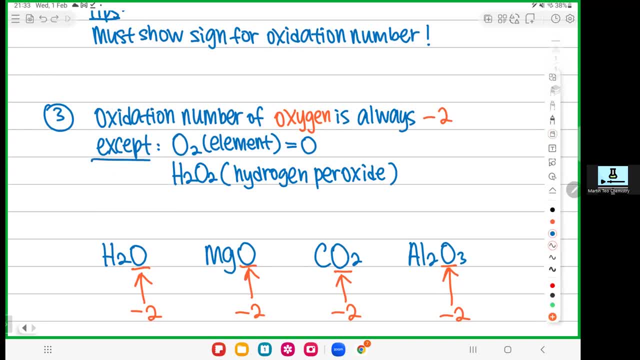 name doesn't matter. So in H2O2, this is another special case- In H2O2, the O, here it's negative 1.. Okay, The O here is negative 1. Other than that, oxygen is. 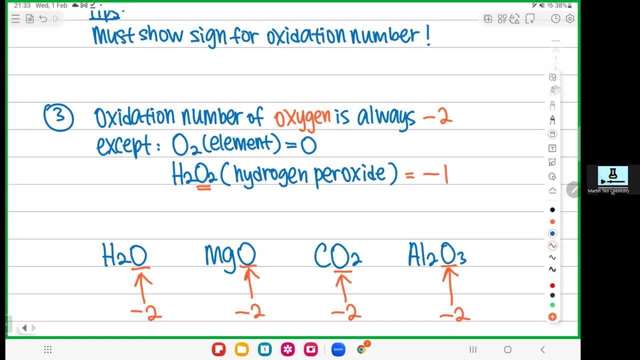 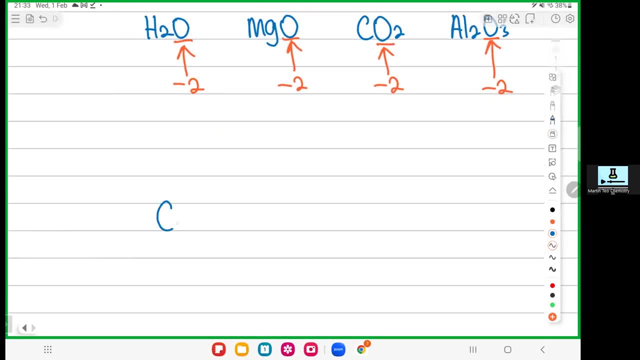 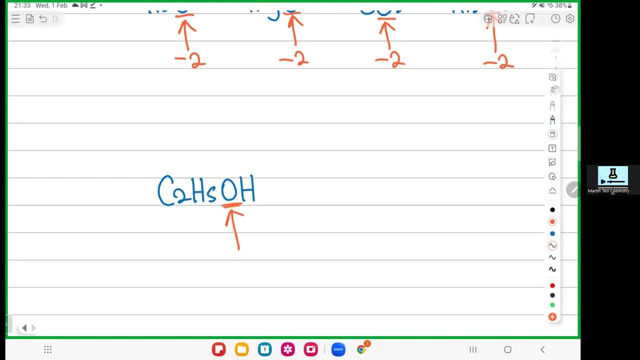 always, always, always negative: 2. Okay, Other than that, oxygen is always, always, always negative. 2. Okay. Example: Let's say C2H5OH. Okay, So this oxygen? what is the oxidation number? This oxygen? 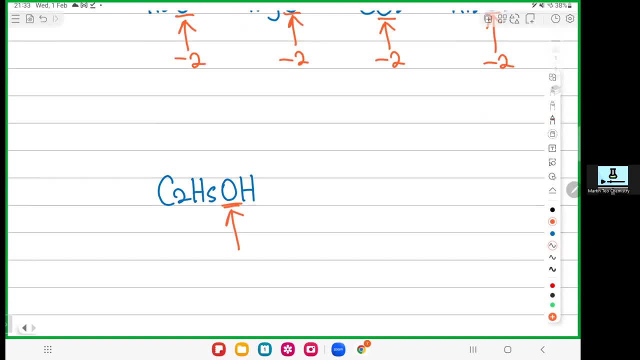 what is the oxidation number? Somebody type in for me. Very good, Not negative 2, right, Because this is not the special case. This is not the special case. Okay, let's say another one. Okay, All right. Zinc. 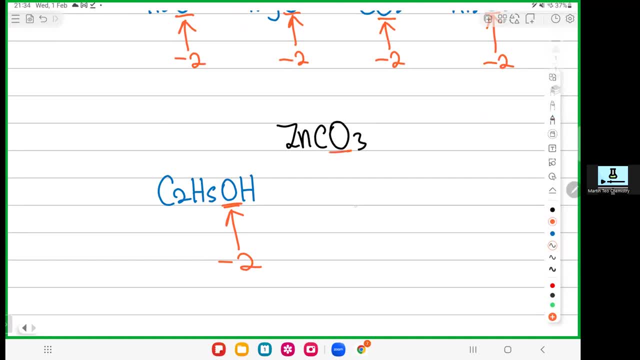 carbonate. Wow, We have 3 oxygen here. So this oxygen, what is the oxidation number? What is the oxidation number for this oxygen? Very good, Negative, 2.. Okay, what if I have this O3? O3, called ozone. 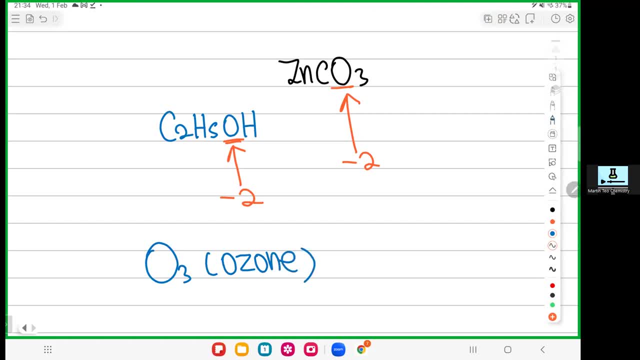 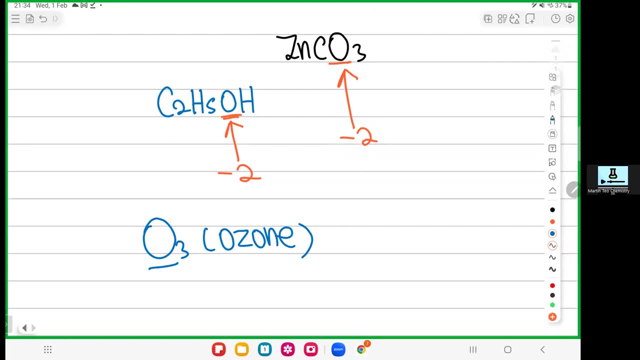 Not in the syllabus, Okay. But what if they ask you what is the oxidation number for the O in the O3? O3. Fantastic zero. Why? Because only got O, only one species. You are element. So when you only 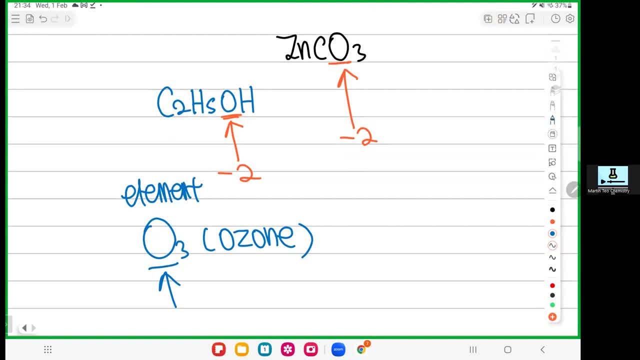 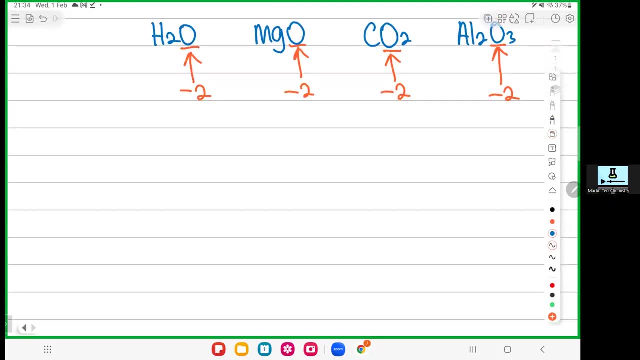 have one species, you are element When you are element zero. As simple as that. Yeah, So very good. Okay. So, guys, seems that you guys have some good ideas. So if anyone already get lost, if you 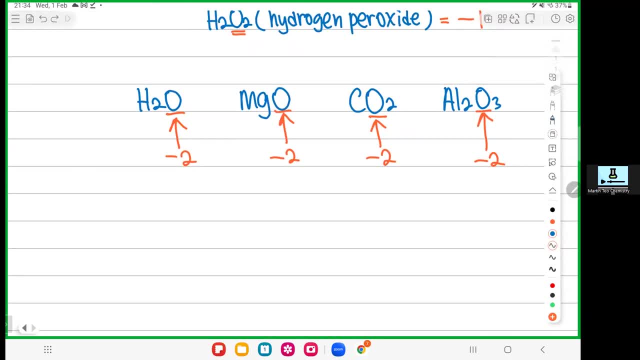 already get lost. if you cannot follow, can you type an X in the chat box? If you cannot follow already, you feel very confused. you can type the X, Okay. Okay, No worry, We are going to the last rule and that is. 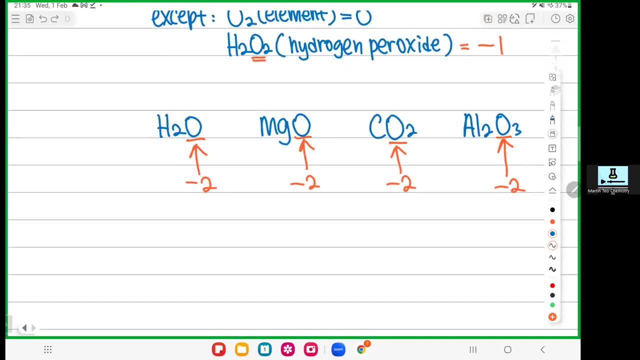 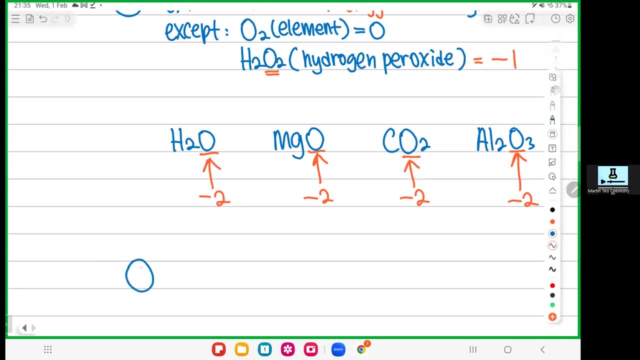 the last thing for today. Okay, I'm not going to put too many things for you, or else you just cannot take it. Okay, I'm not going to put too many things for you, or else you just cannot take it, Okay. So let's look at rule. 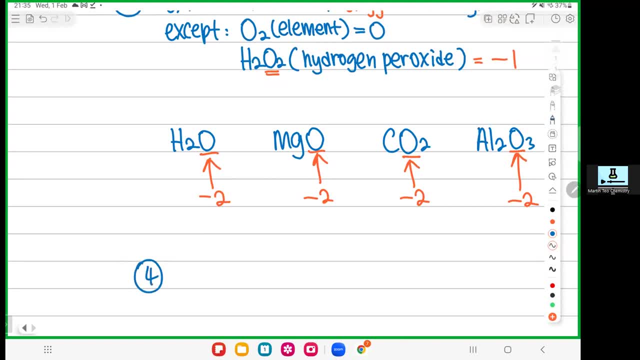 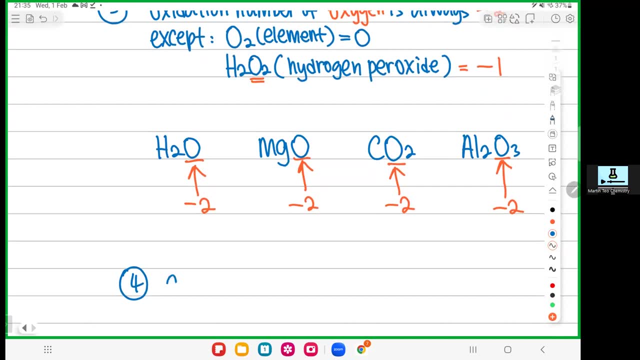 number four, which is the last rule already. The last rule already. yeah, So the last rule that we can see is this. The last rule is this: Okay, Oxidation number. Oxidation number for hydrogen. Just now we have oxygen. Now we look at hydrogen. Hydrogen, the oxidation number is always always positive one. Hydrogen is always always positive one, except, again, two special cases. Okay, The two special cases I'll talk about, But let's look at the normal. 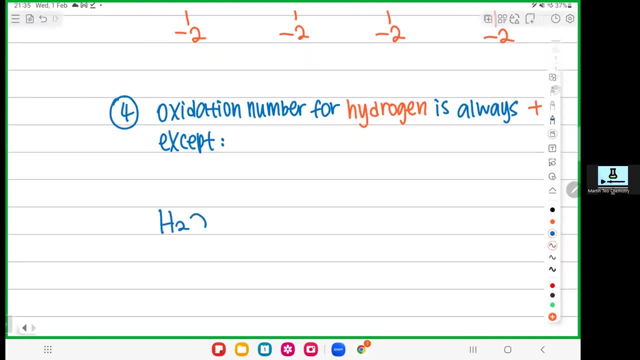 cases. Let's say normal case: water, Water. do you have hydrogen? Yeah, So the hydrogen here it's plus one. You see, it doesn't matter how many H you have, As long as you have H, you have plus one. 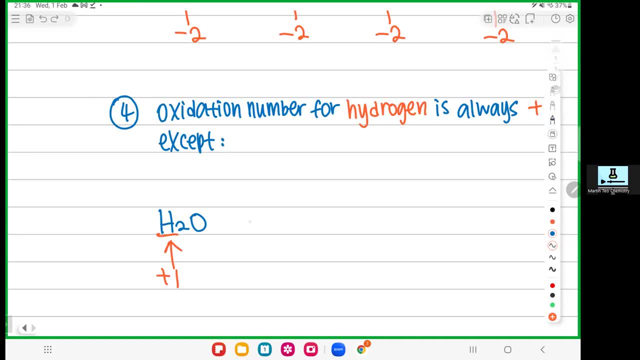 So let's say we go for something different. Okay, Let's say we go for sulfuric acid. Sulfuric acid also got hydrogen, right. All the hydrogen here is plus one. Let's say we go for hydrochloric. 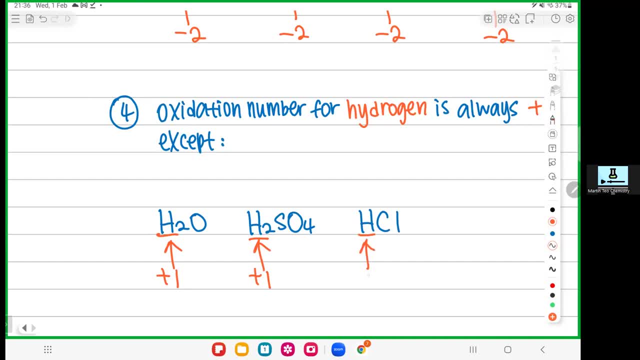 acid, Hydrochloric acid also got hydrogen, right. So it's plus one. Okay. So let's say we go for some very weird substance. Let's say we go for some other weird substance. Let's say we go for CH3,. 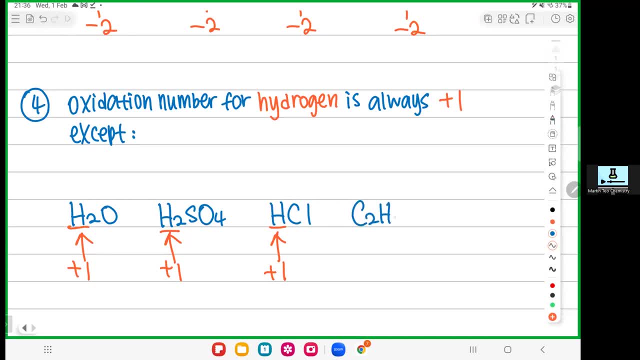 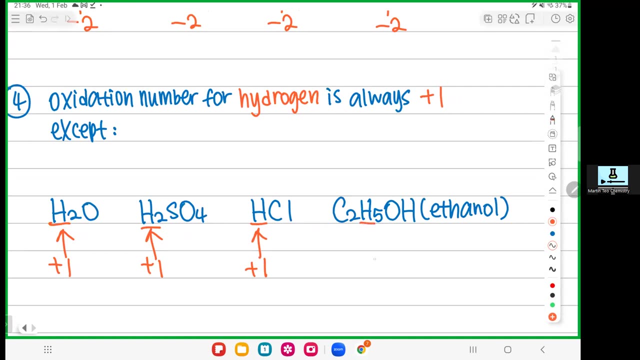 C2H5OH. So this fellow is ethanol. You will learn this in your Form 4, Form 5, Chapter 2.. So this fellow is an alcohol. So this fellow got hydrogen, This hydrogen also, plus one, This hydrogen. 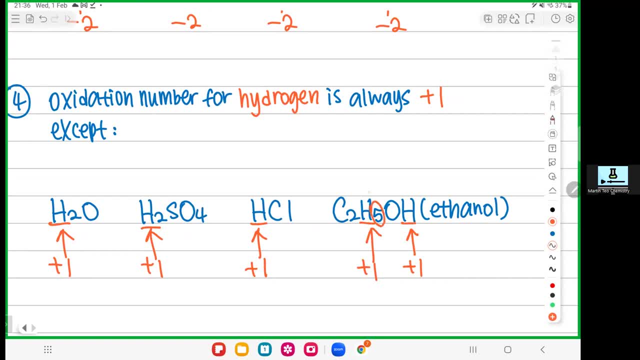 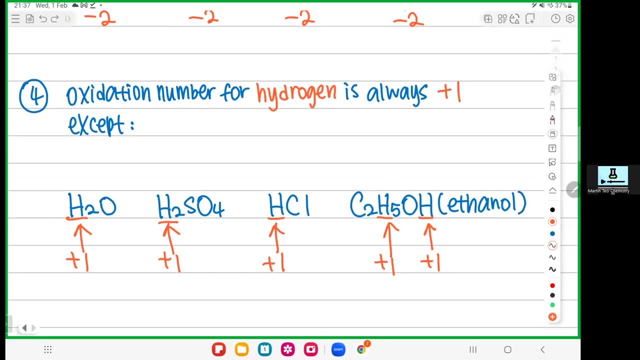 also plus one. Okay, No matter, here got five hydrogen or here got one hydrogen, don't care. As long as you have hydrogen, it's plus one. That's it Very easy. Hydrogen always plus one, Oxygen always minus two, except special case. 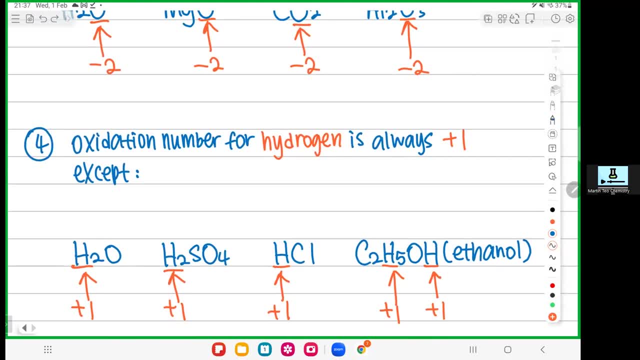 Okay, So what is the special case we have? The first special case is H2. Hydrogen gas. Hydrogen gas, again, not H2. Both of them are H, Only one species. So you are element Again when you have element. 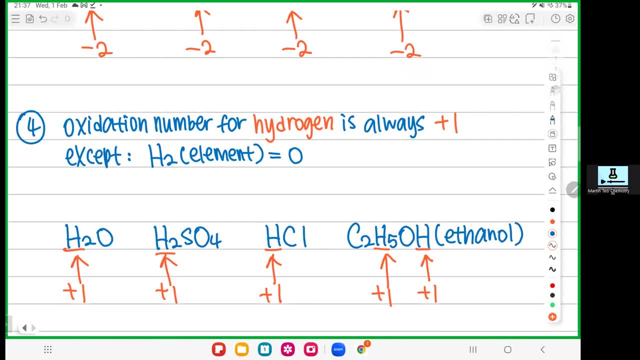 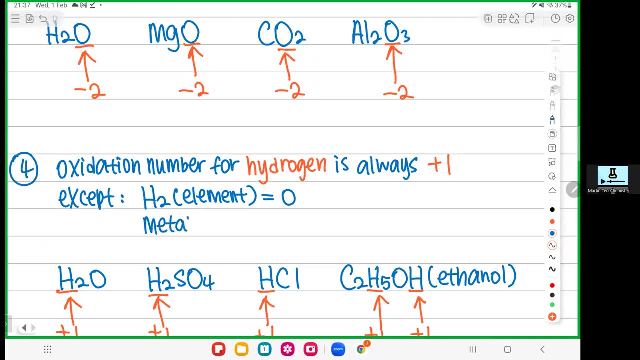 it is zero. You know when you have element, you are zero. Another special case, which is super, super rare- in exam as well- which is called metal hydride. No need to memorize: Metal hydride means metal. 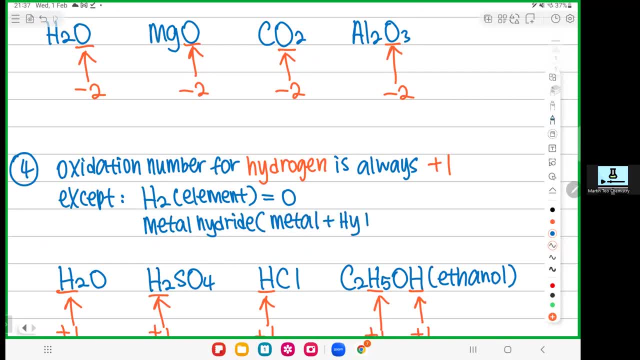 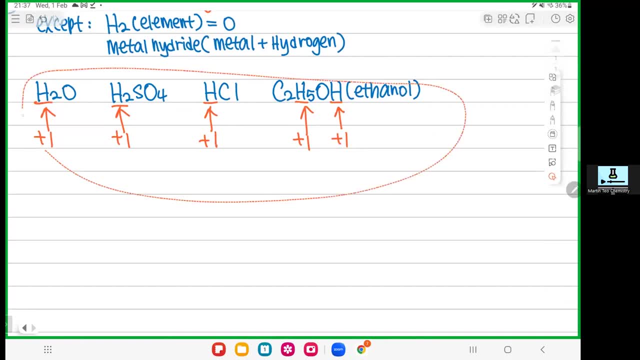 combined with hydrogen. When metal combined with hydrogen, you get metal hydride. Okay. So when you have metal hydride, okay. So like this: okay, Let's say we have a change color. I use green color. 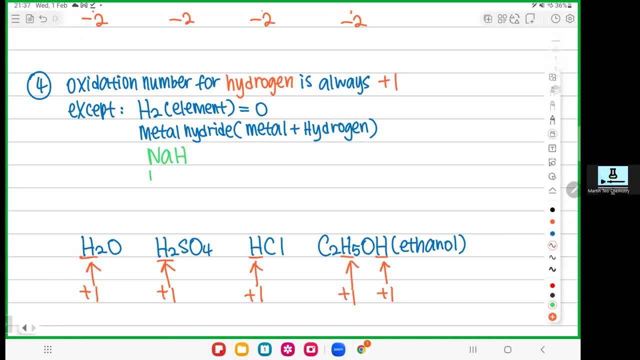 Sodium is a metal combined with hydrogen. Magnesium is a metal combined with hydrogen. Aluminium is a metal combined with hydrogen. So when you have metal combined with hydrogen, you call it metal hydride. So in metal hydride, 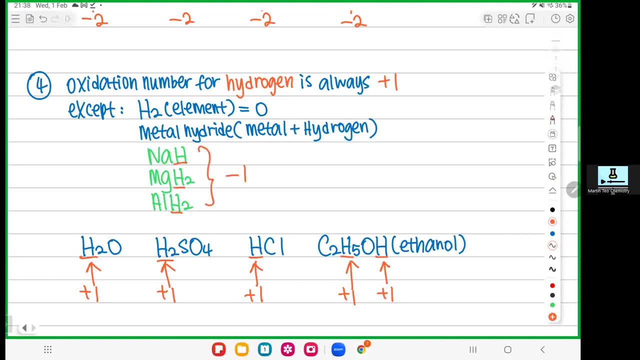 all the hydrogen here they are minus one. Other than that, hydrogen always plus one. No worry, This one is super, super super rare in exam, Super super rare in exam. So it's good to know, It's good to know, But the chances 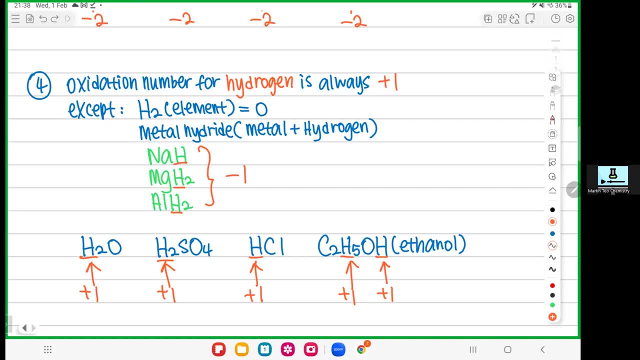 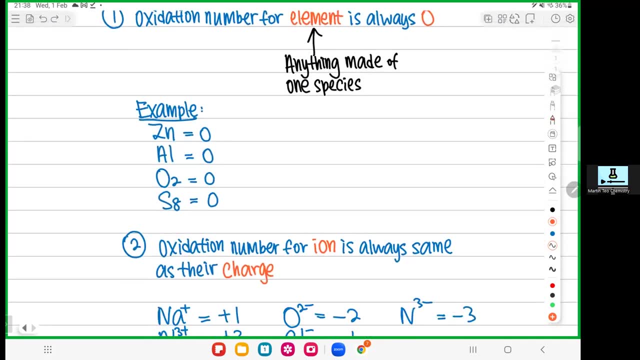 to be tested is super low, Very, very low. Okay, So by using these four rules now, you can get majority of the oxidation number. Okay, You can get majority of the oxidation number already. So now let me show you using 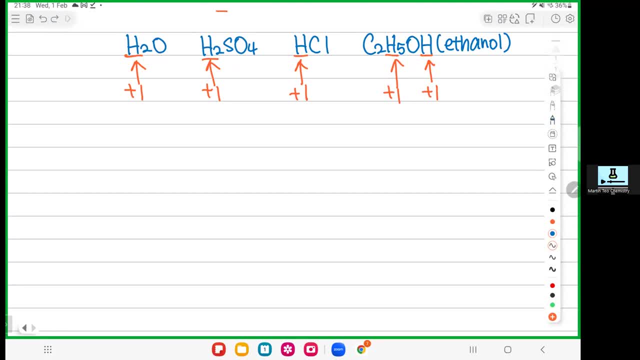 two examples: how to use the oxidation number to do the apple to apple comparison. So let me use two examples to show you how to use the redox, So how to do the apple to apple comparison by using this so-called oxidation number method. Okay, I start with easy one first, 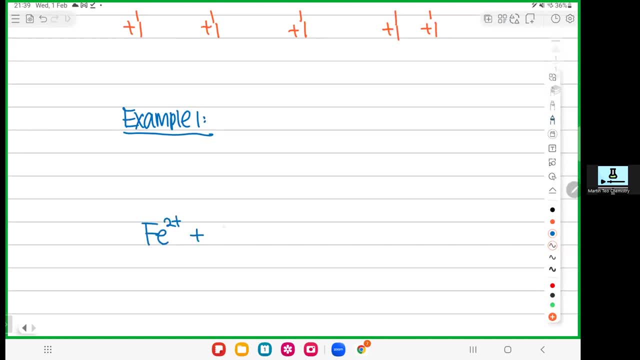 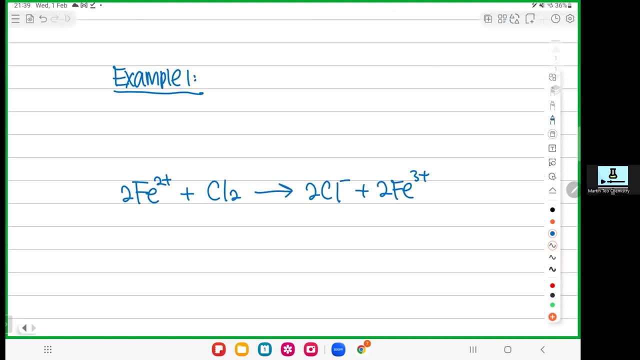 Fe 2 plus fluorine become 2 chloride. This one put 2.. This one put 2.. Fe 3 plus: Okay, So no need to memorize, Just show you only Okay. So now let's say you have this question, Can we use? 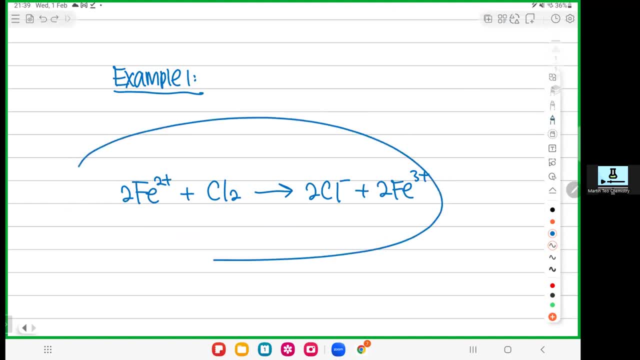 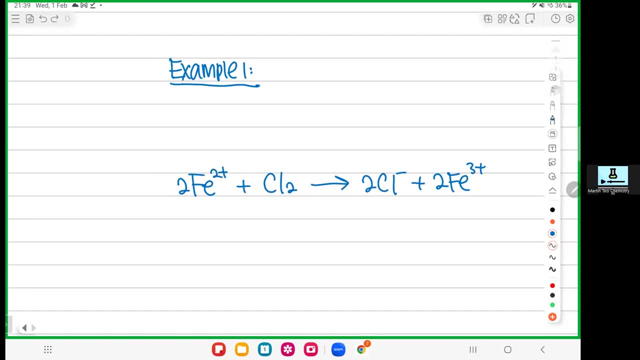 oxygen method? No, There's no oxygen at all. Can we use hydrogen method? No, There's no hydrogen at all. So now we have to use oxidation number method. So when you want to do oxidation number method first and 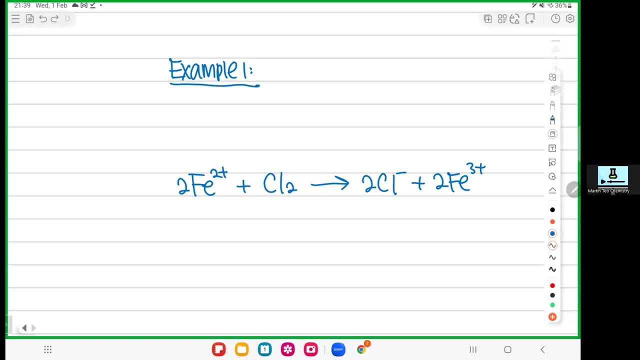 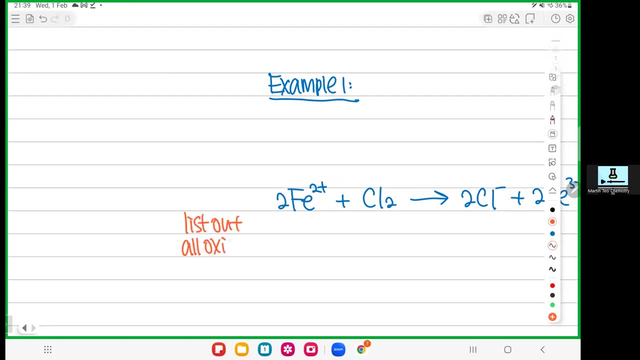 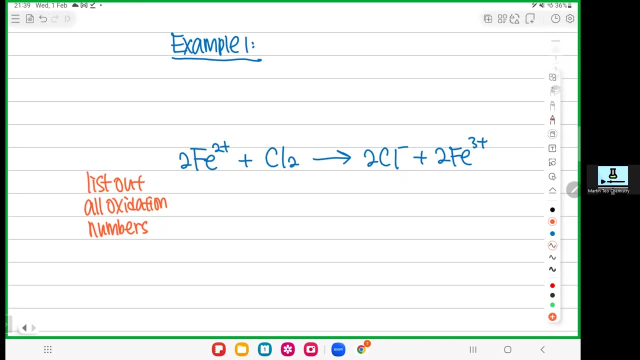 foremost. first of all, you need to list out the oxidation number first. First of all, please list out all the oxidation numbers. You need to list out all the oxidation numbers, Okay, On the left and the right. So can we do it together? So what is? 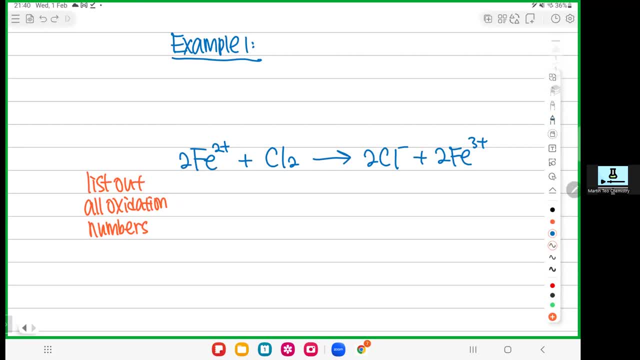 the oxidation number for Fe 2 plus here, Guys, what is the oxidation number for Fe 2 plus? Anyone can type in the chat box and let me know: Okay, 2, 2, wrong Plus 2.. Okay, So some people. 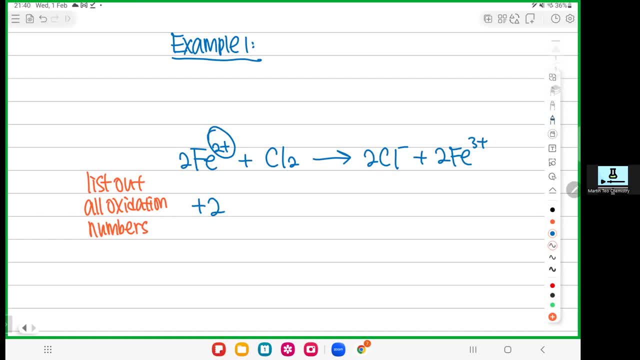 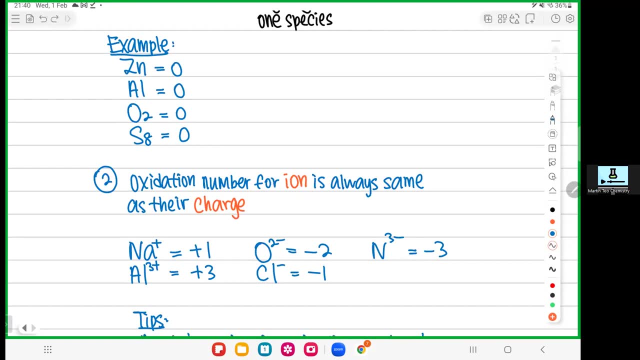 answer 0, wrong, Why This fellow got charged When you got charged. you are ion, So ion the oxidation number. copy the charge rule number 2.. So there are many of you type only 2, which is wrong. 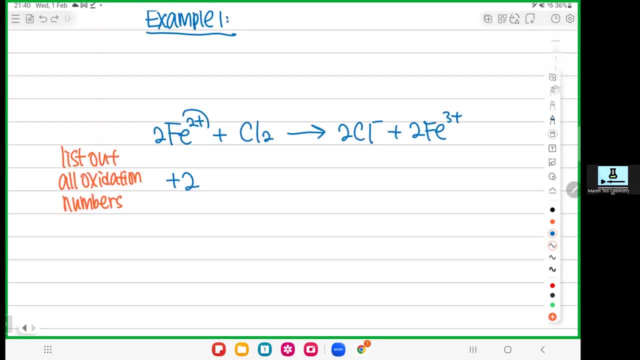 Remember I say what Oxidation number always need to type the sign. You must put the sign even though it is positive. So it is positive 2.. It is positive 2.. Alright, So not 0. Why it's not 0? Because you. 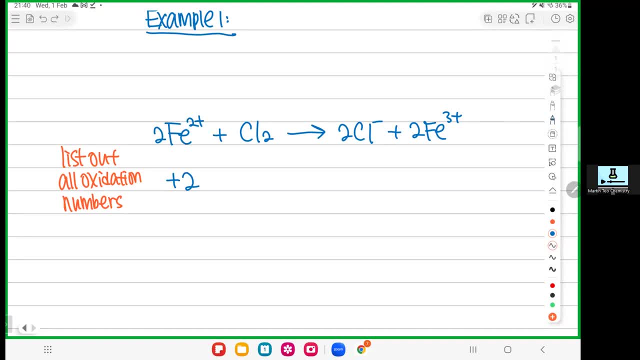 got charged. When you got charged, you are ion. When you are ion, the oxidation number must follow back the charge. Okay, Alright, Next one. What is the oxidation number for the chlorine here? What is the oxidation number for the chlorine here? 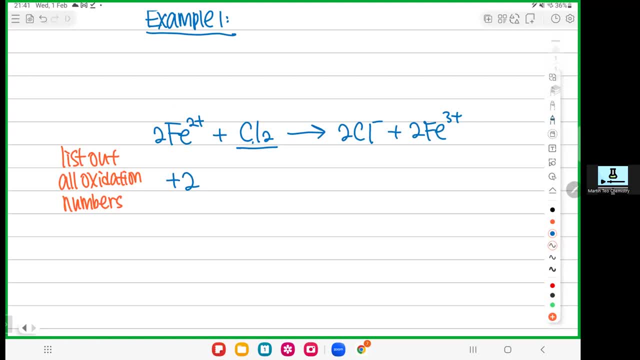 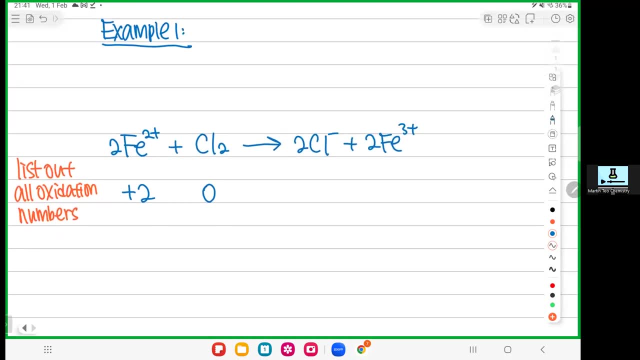 Okay, Very good. 0., Because this chlorine is one species element, So it is element. Element is 0.. Rule number 1.. Very good, What is the oxidation number for this fellow Chloride? What is the oxidation? 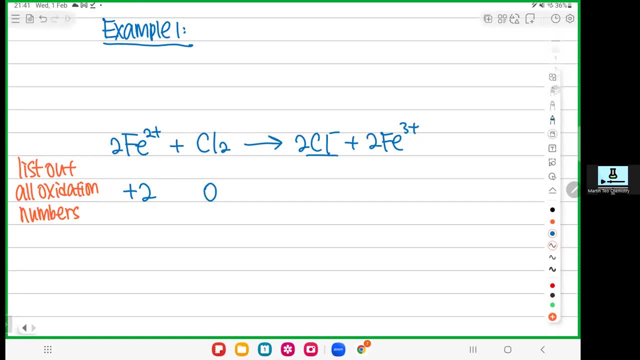 number for chloride here, Fantastic. Negative 1. Remember when you have charged you are ion. When you are ion I will copy back your charge. Negative 1.. Okay, So some people say, Sir, I got 2 in front, No need. 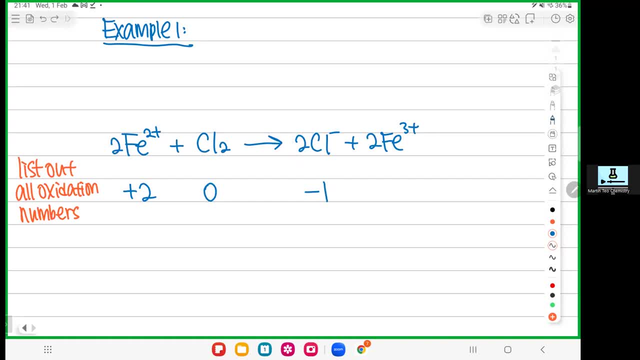 to times 2.. No need Remember I say what. All the number in front only for balancing purpose. All the number in front only for balancing purpose. So what is the oxidation number for Fe3+? So this fellow got charged. 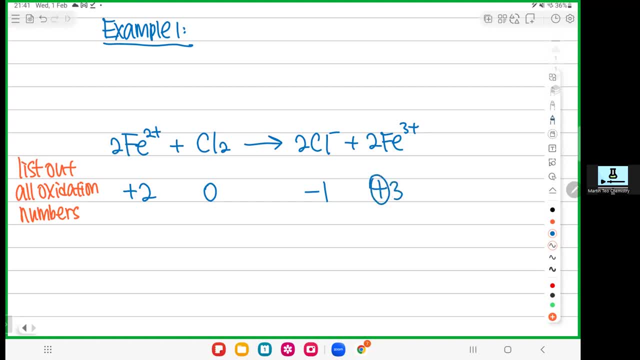 Oxidation number. copy the charge Plus 3. Must put the plus. If you only put 3, it's wrong. Remember oxidation number must always show the sign, despite it is positive or negative. No matter it's positive or negative. 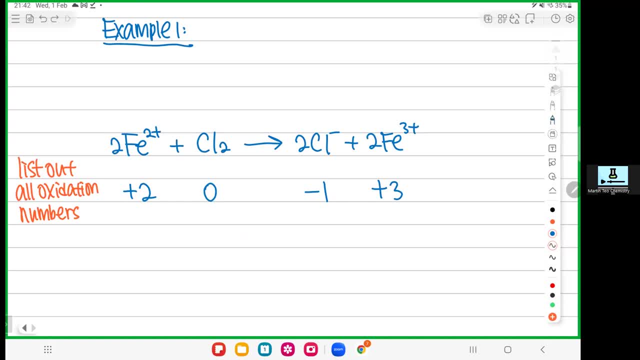 you need to show the sign, Very good. So once you list out the oxidation number, then only you do your apple to apple comparison, Then only you do your apple to apple comparison. So let's do it, Okay. First apple. 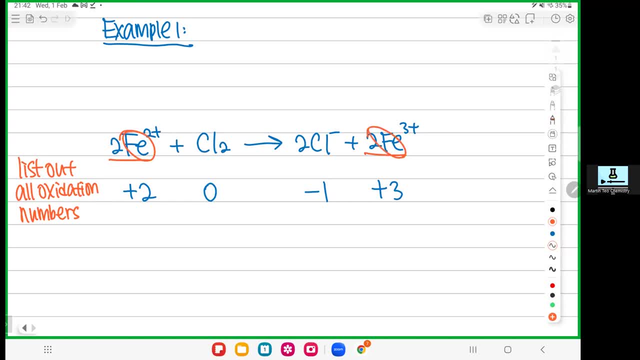 Fe2+ compared to Fe3+, because you can see something in common, right. So plus 2 to plus 3, what you can see Oxidation number: plus 2 to plus 3.. So oxidation number we don't say gain or 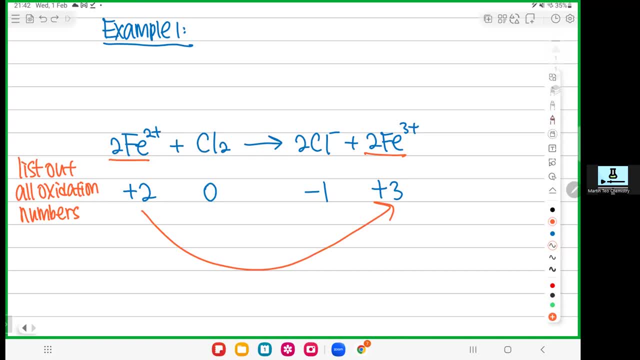 lose one Oxidation number number. you don't gain or lose. You don't say: I gain a number, I lose a number. No, You can say: you gain oxygen, you gain hydrogen, you lose oxygen, you lose hydrogen. So 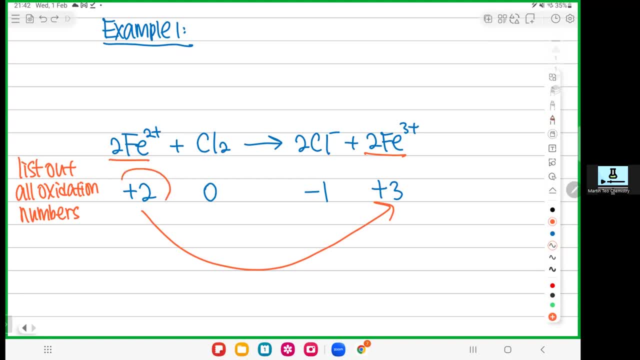 oxidation number. normally we use increase or decrease. Plus 2 to plus 3, increase, So oxidation number increase. Now ON stands for oxidation number. Okay, Oxidation number increase. So according to the oxidation number method that we learned, 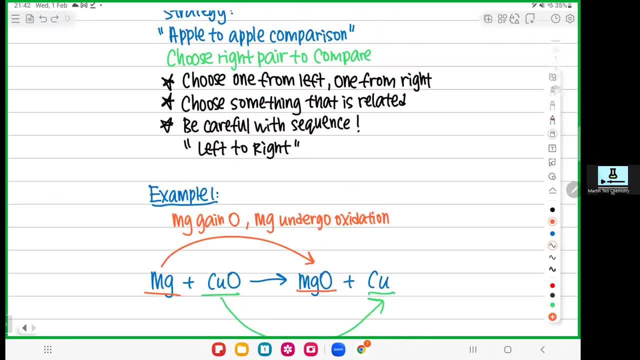 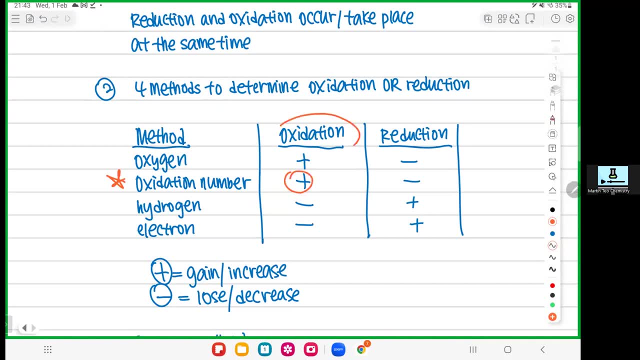 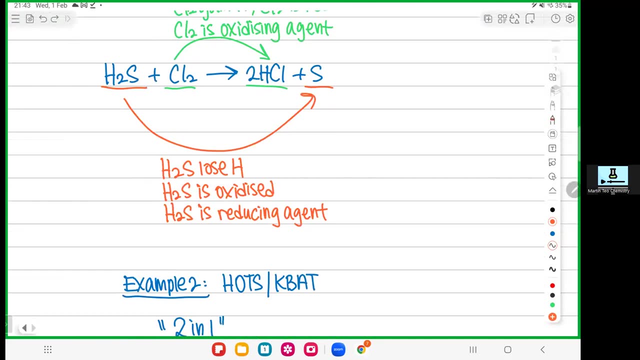 earlier on today. look back: Okay, According to oxidation number method, When the oxidation number increase means plus. So it is oxidation process, Okay, So you know already, Okay, What happened. So it undergo oxidation process. So when you undergo, 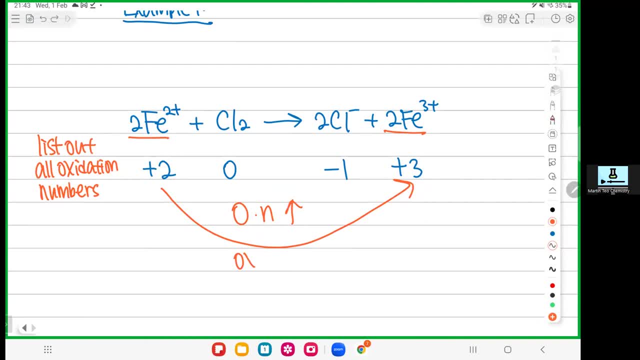 oxidation process. who undergo oxidation process, This fellow FE2+. So FE2+ undergo oxidation process. When you undergo oxidation process, FE2+, it is opposite reducing agent. Okay, So next one Another apple to apple comparison. 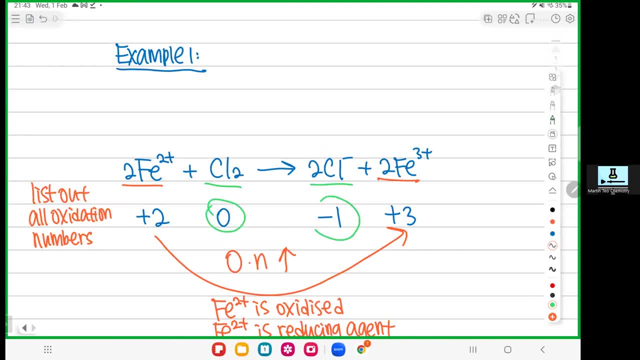 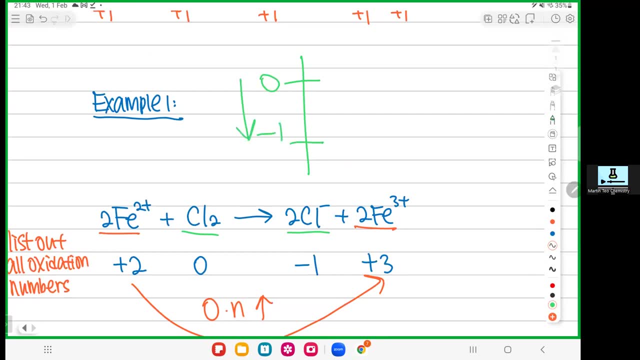 So this apple, compared with this apple, obviously 0 to negative 1.. What happened? Number decrease right According to number line: 0, negative 1. Decrease, right. Okay, So you can see the. 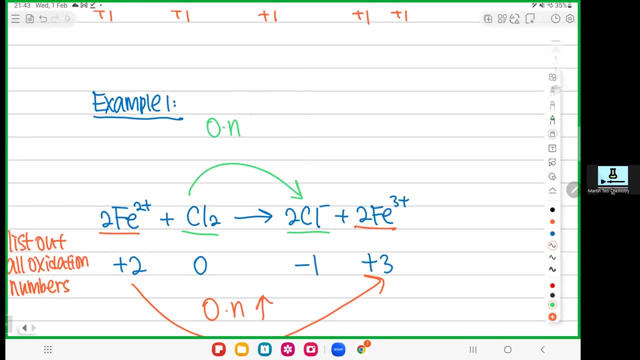 oxidation number decrease. So oxidation number decrease means reduction. So who undergo reduction? This fellow Chlorine undergo reduction. So when chlorine undergo reduction, you will be oxidizing agent, You will go opposite. As simple as that. Okay. 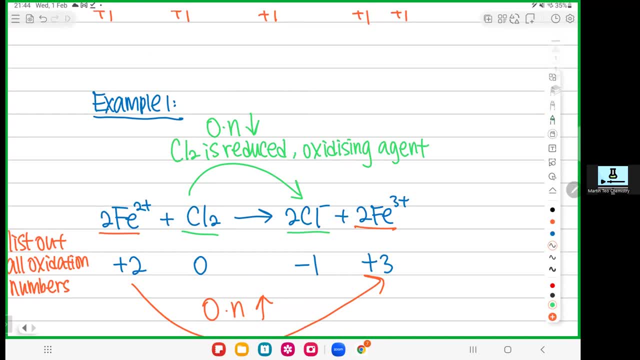 So guys, let me know in the chat box: are you okay with oxidation number method? so far Not very hard, isn't it Okay? I mean okay lah, Not very hard, Okay Now what if I increase the difficulty? 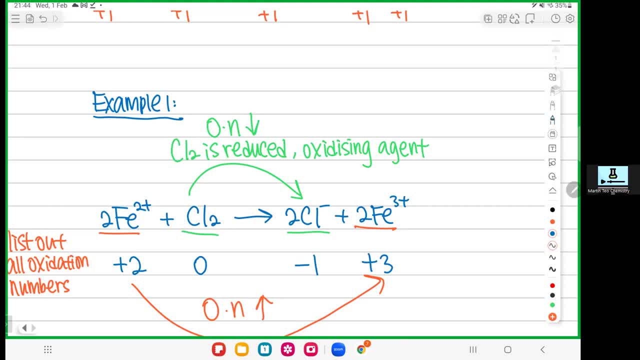 a little bit Okay. So let me see. Okay, Haida is all the agent on the reactant side. Yes, All the agent here will be on the left-hand side here, Because you always compare left to the right right, So you always. 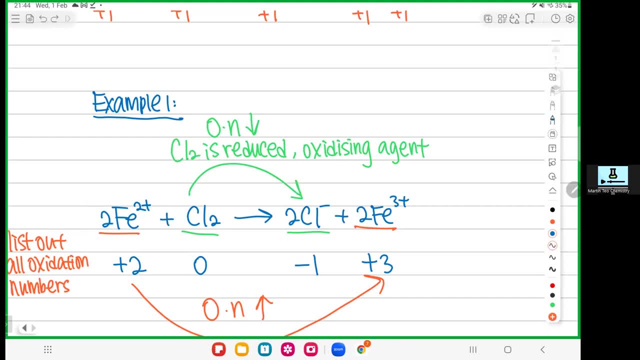 focus on the left. So all the agent, oxidizing agent, reducing agent- they are always on the left. It's never on the right, Because you never compare right to the left. Okay, So that's why you always focus on the left, All right. 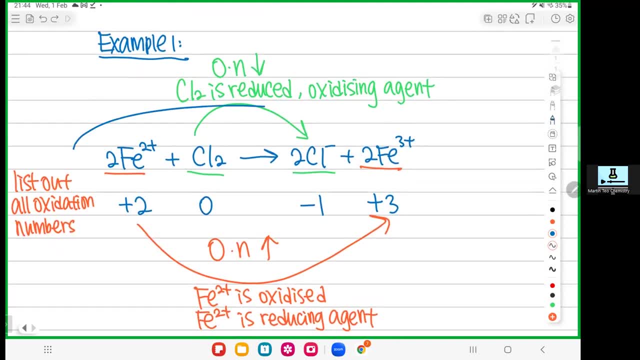 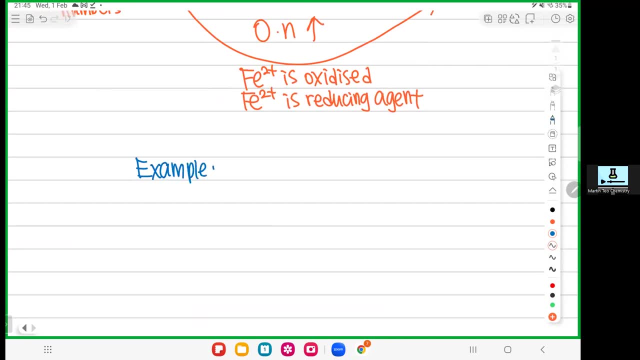 Good question, Haida. Okay, Good one, All right, So now. this is very straightforward, Okay. So now let me show you how I can make it a little bit more confusing. Not hard, Just slightly more confusing. 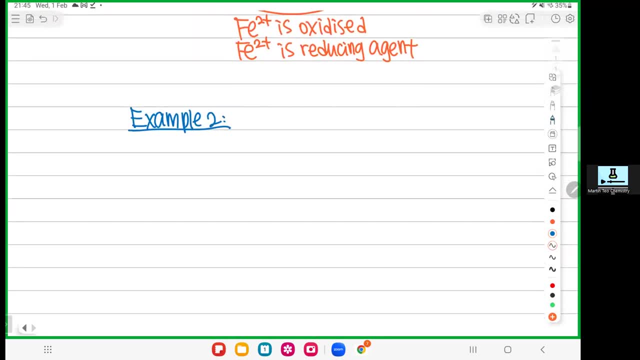 Just slightly more confusing. Okay, Just look at this And then we do two past year question, Then we are all done with today. Okay, Give me 10 minutes. Okay, Give me 10 minutes to finish off with today's lesson. Yeah, All right. So let's say we have. 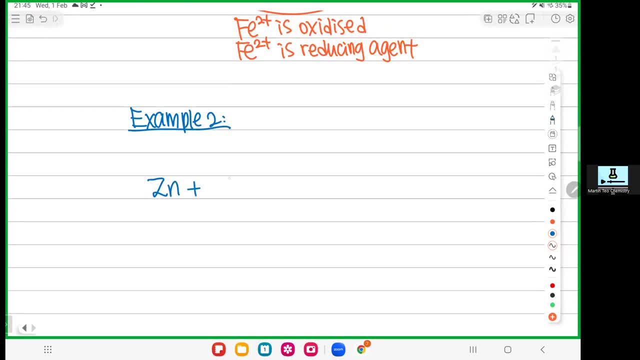 zinc, And then we have bromine, And then we have zinc bromide. Okay, So let's do it. Okay, Let's do it Okay. So zinc and bromine become zinc bromide. Okay, Now. 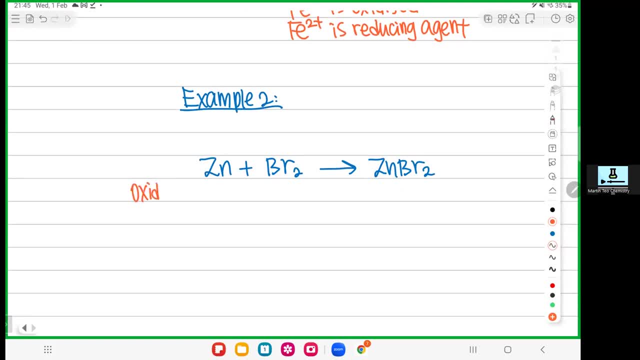 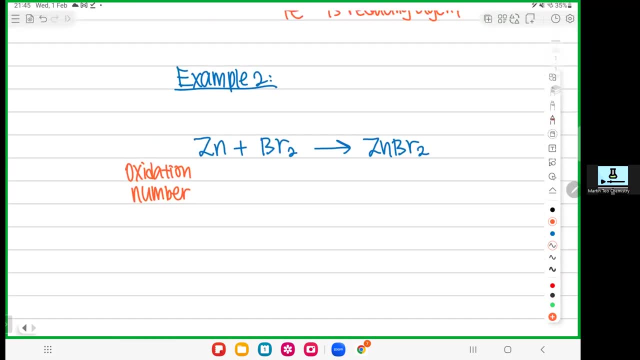 can we first list out the oxidation number? So let's list out the oxidation number, And I would like to ask you all to help me with this. So what is the oxidation number for zinc? Anyone can help me. What is the oxidation number for zinc? 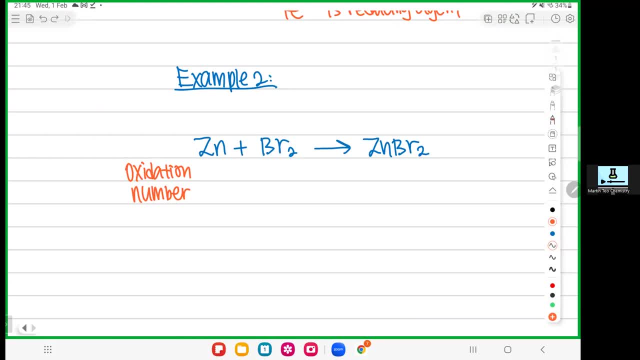 Okay, Zero. Okay, Not plus two. Okay, Yingqi, Not plus two, Because you only get plus two when you have charge. You don't have charge at all. So if you don't have charge, you are not an ion, You have only one. 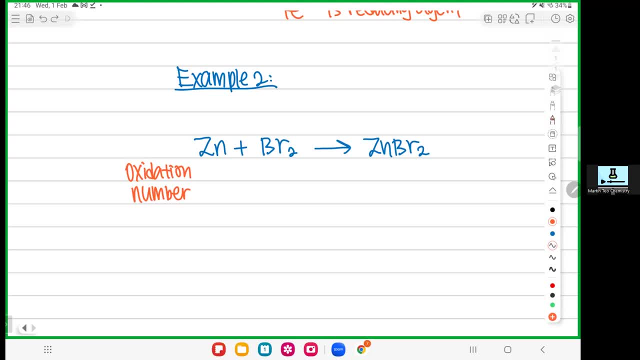 species. You are element, So its element should be zero. Okay. So anyone can tell me what is the oxidation number for bromine? Anyone? Bromine? Okay, Very good, Zero, Because the bromine only got one species right. 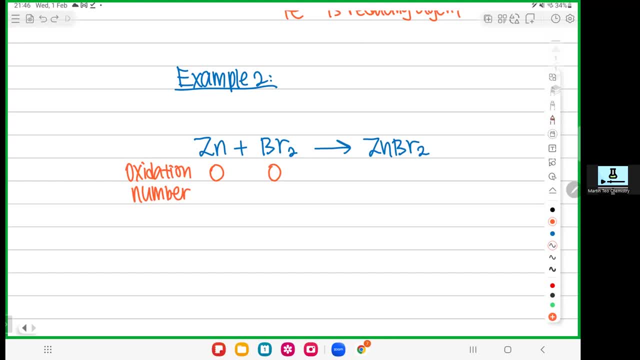 You only have Br, nothing else. So you are element. So when you are element, you are zero. Very good guys. Come on to the last one. What is the oxidation number for zinc? on here, the right-hand side. 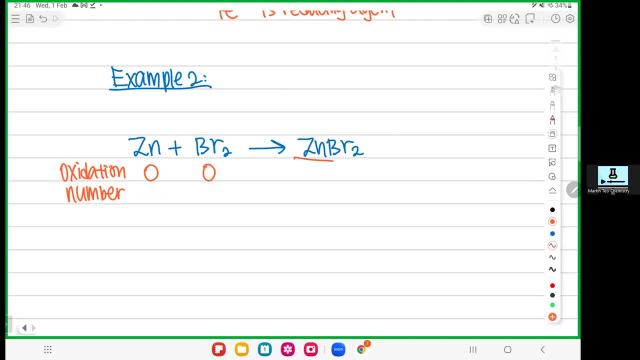 What is the oxidation number for zinc on the right-hand side? Okay, I saw two plus I saw zero. Any other answer? Zero plus two. What else? Plus one Plus two? Okay, Now listen carefully, Listen, listen, listen, listen. 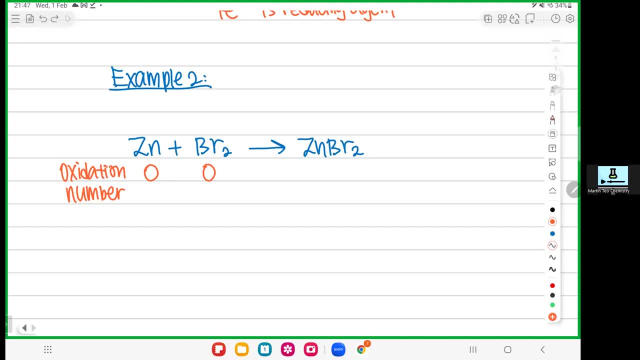 listen carefully. I say five times so important, Listen carefully. So the zinc here can it be zero? No, You are zero when you are element. Is the zinc one species here? No, Zinc combined with Br: you have two species here. 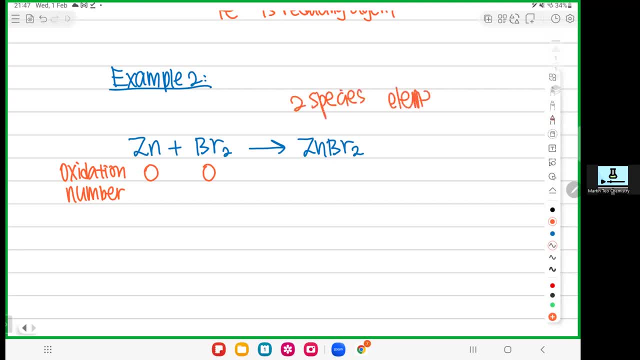 So when you are two species, you are obviously not an element, So it cannot be zero. Do you know the charge of zinc? Yes, They purposely don't show you the charge, but you should know it. Zinc bromide. 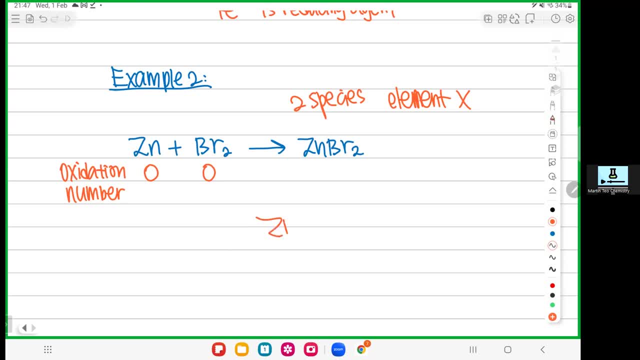 Okay, Do we know what is the charge for the zinc? Yes, Zinc is Zn two plus, isn't it? You learn this back in your form. four: What is the charge for bromide guys? Br. what Minus. 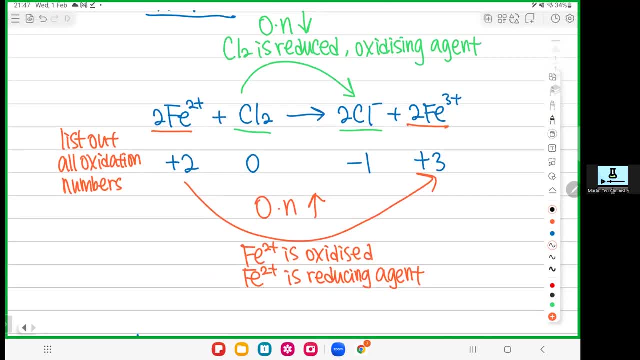 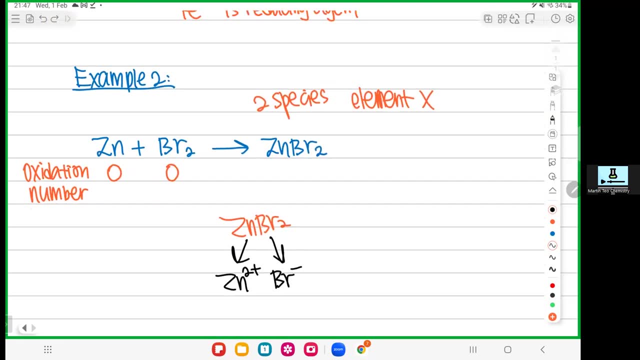 right, Hold on, Okay, So you don't expect they will spoon feed you give you the charge every time. No, Sometimes, which is most of the time, they are not going to give you the charge which you have to find. 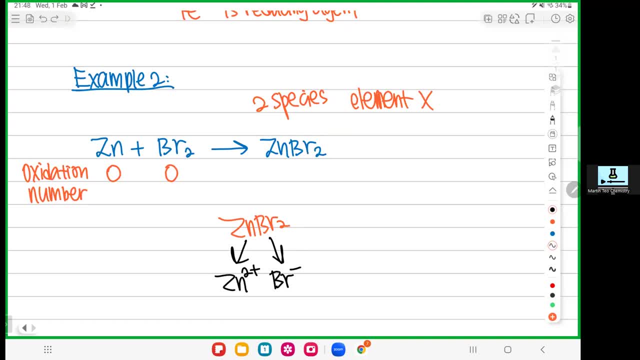 it out yourself. You have to find it out yourself. So zinc bromide is made by zinc, Zn two plus bromide Br minus. So when you know the charge of zinc, can we go for the oxidation number? Yes, 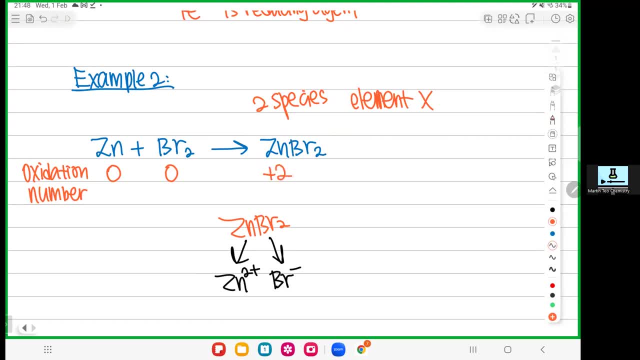 The charge and oxidation number is the same Plus two, not two plus Oxidation number. the charge come ahead of number. What about the bromide? So, bromide, we know. it is Br minus. So Br minus, Br minus. 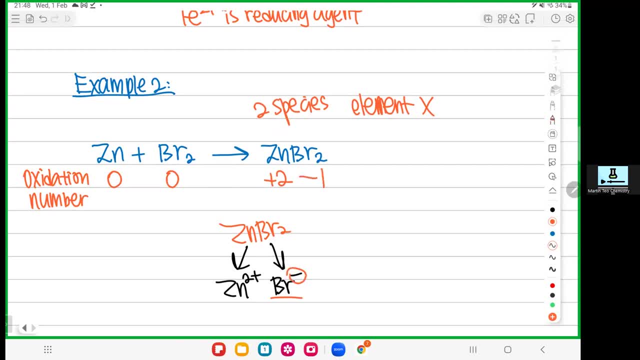 oxidation number. copy back the charge: negative one: Okay. So guys let me know in the chat box: are you okay with the listing of oxidation number? If you are okay, type okay. If you are not okay, type X. 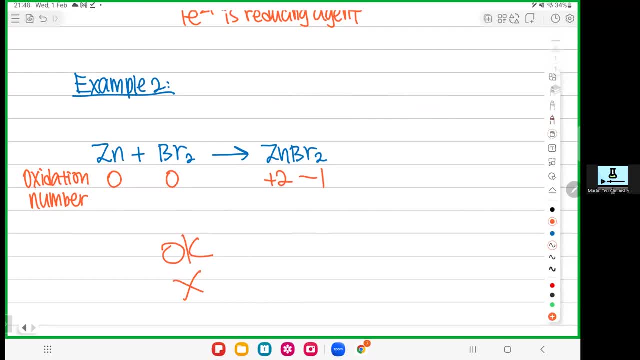 This is very, very important. Okay, This is very, very important. Okay, I want to make sure everyone is okay, Because this is exactly how the question will be tested in SPF. This is exactly how they ask the question for SPF. 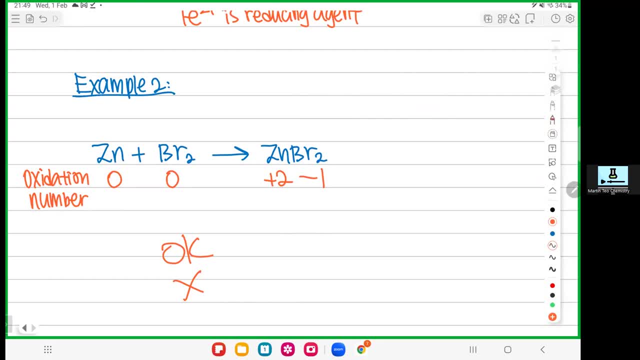 Okay, They are not going to give you all the charge one. You have to find it out yourself. Okay, Good huh, Okay, So after you list out the oxidation number, then you can do your apple to apple comparison. oh, So, let's. 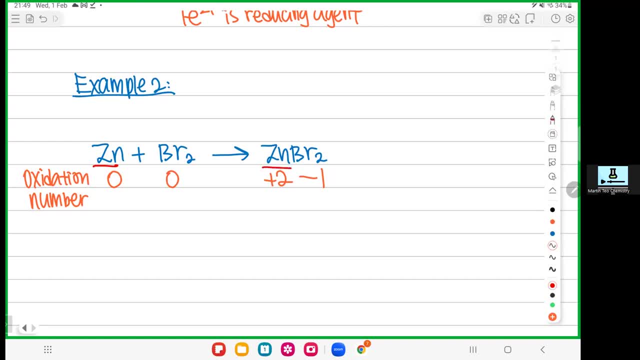 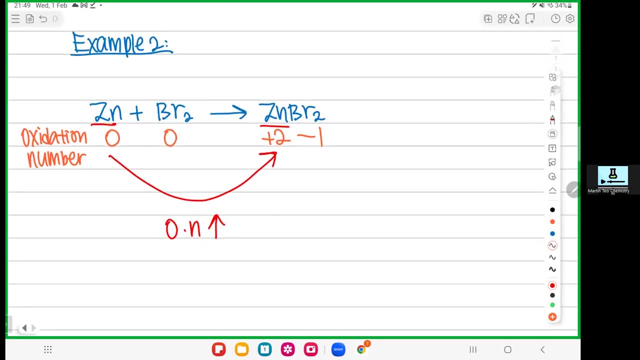 look at it: Zinc. compare with zinc la Pro, not Zero to plus two. oxidation number shoot up right, So oxidation number increase. according to the table we learned today, Oxidation number increase is oxidation, So zinc. 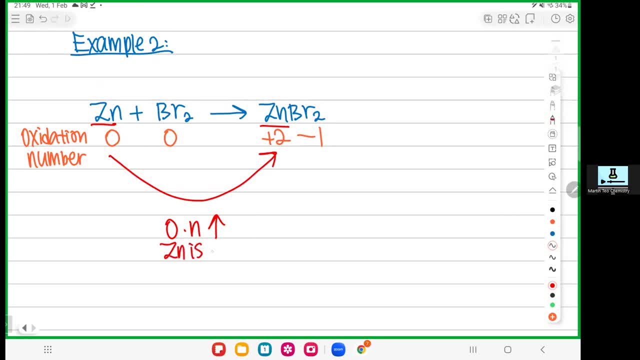 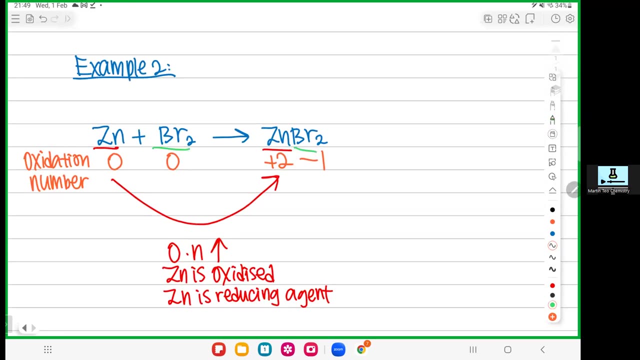 undergo oxidation. So when zinc undergo oxidation, zinc will be the opposite thing: reducing agent. Okay, So let's do another apple to apple comparison, which is the bromine Bromine. compare with bromine, la Apple to apple ma. 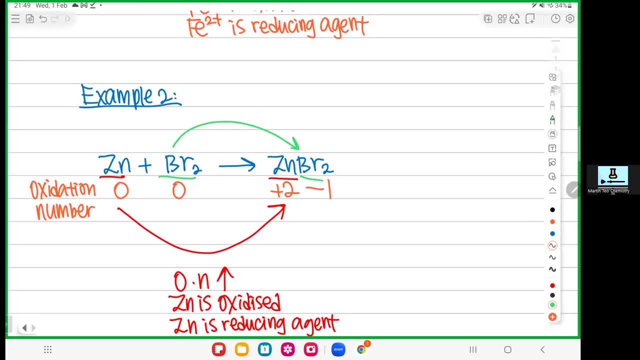 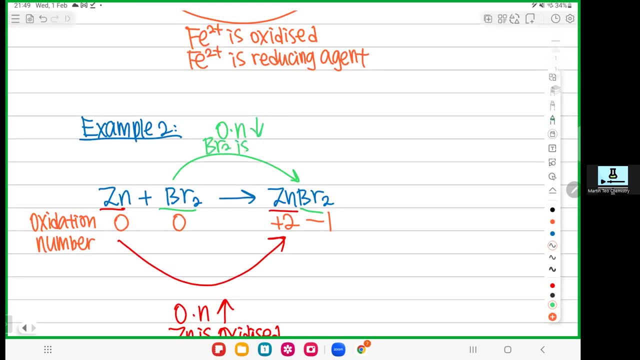 Zero to negative one, Zero to negative one, the oxidation number went down, decreased, So oxidation number decreased. So this fellow bromine undergo reduction, isn't it Okay? When oxidation number decrease is reduction. So when undergo. 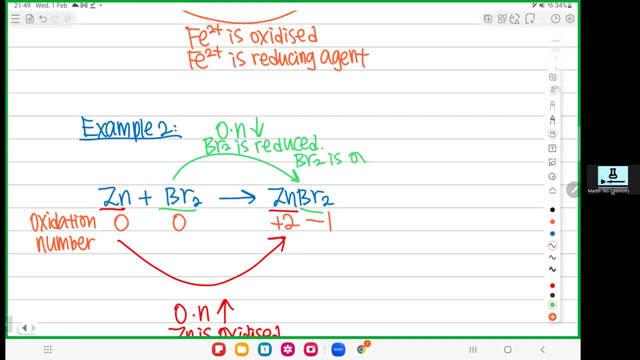 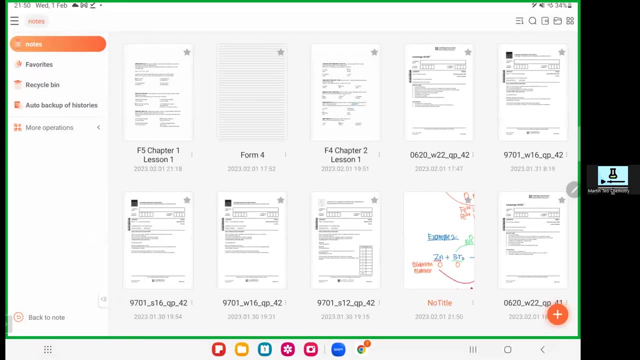 reduction. so the bromine, it is our oxidizing agent. That's it, Okay, So that's exactly how it works, Okay, So, to finish off with today's lesson, so let me show you the trial exam paper. Let me show you the trial. 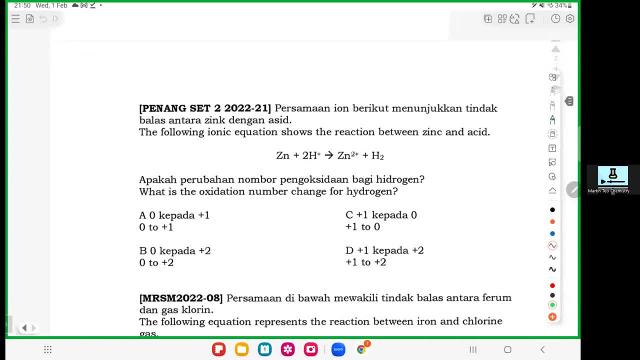 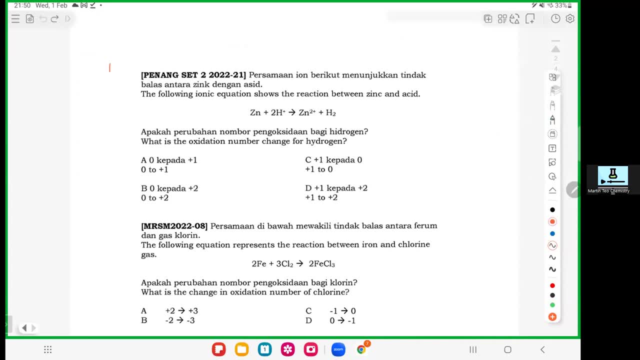 exam paper so that you can see exactly how to apply. So I will do two questions for you With you, then we were all done with today's lesson. So one question from Penang, one question from MRSM. Okay, Right. 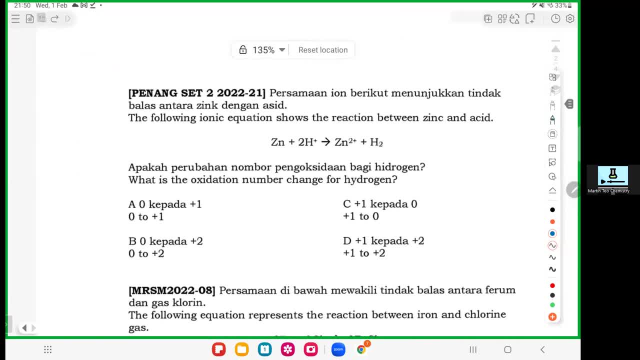 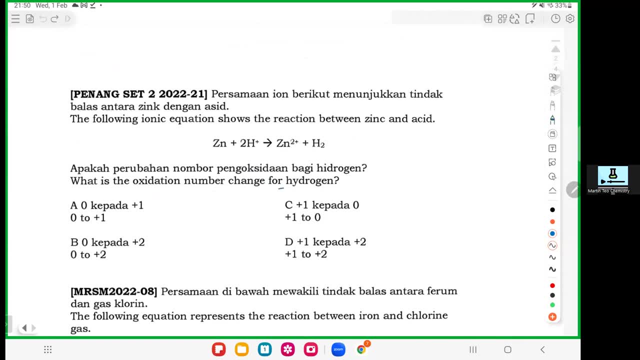 Both are trial exam questions, which are good quality questions. So, first of all, what is the oxidation number change for hydrogen? So hydrogen, they only ask hydrogen. focus on hydrogen on the left and the right So hydrogen can release out the oxidation. 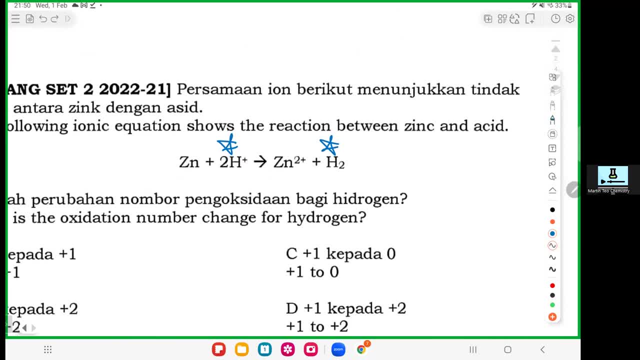 number, Okay. on the left-hand side: H+. So H+ got. charge is ion. When you are ion oxidation number, follow the charge plus one, Okay. So what is the oxidation number for hydrogen on the right? This hydrogen only. 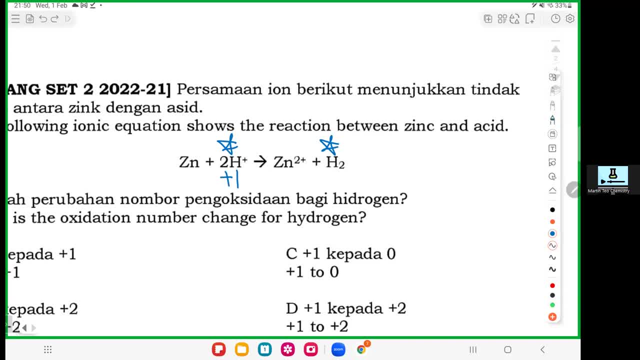 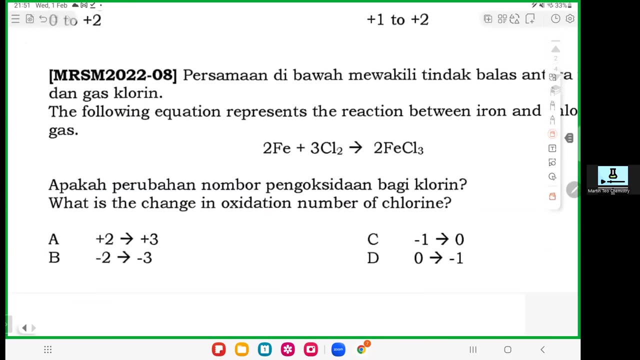 have one species is element. Element is zero, isn't it Remember? Element is zero, Okay, So plus one to zero, As simple as that. Plus one to zero. Answer C. Yeah, Answer C, Next one, Okay. 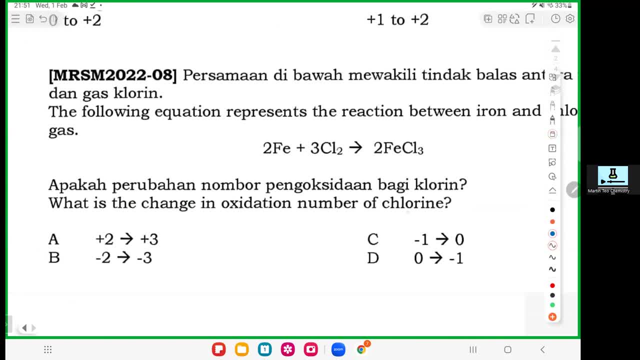 What is the change in oxidation number for chlorine? So chlorine only focus on the Cl here. So on the left-hand side, the chlorine here. Anyone can tell me what is the oxidation number for chlorine on the left? On the left, what is the oxidation number for chlorine? 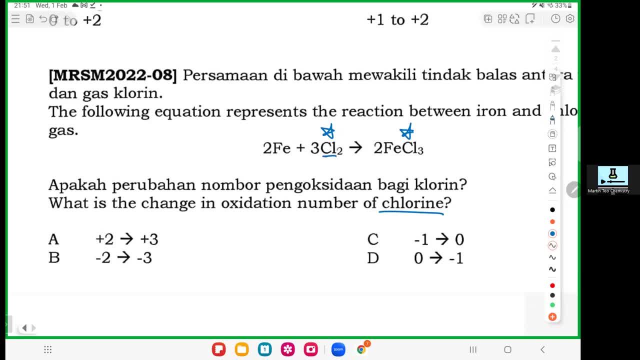 Very good. Zero Because the chlorine here only have one species, only got Cl, nothing else. So it's element Element is zero. Okay, now anyone can tell me what is the oxidation number for chlorine on the right-hand side? 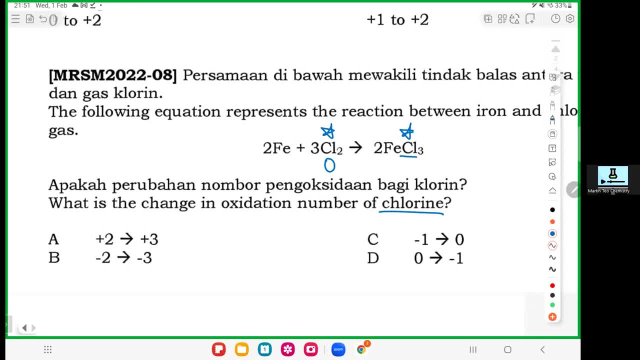 Well done, Venisha Yingqi, Shaila, Joey Jaya, Annie, okay, Eliza Yixuan, Very good. Negative one: Cheng Yi, not one minus minus. one One minus is the charge. 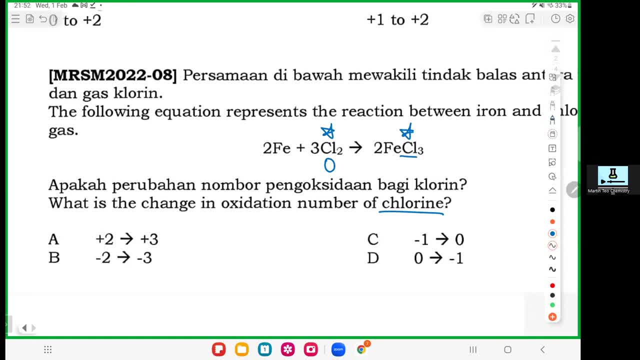 Oxidation number is minus one. Remember oxidation number. the side must come in front of the number, So please don't mess up charge and oxidation number. Is it okay, Cheng Yi? Can I All right? Okay, so. 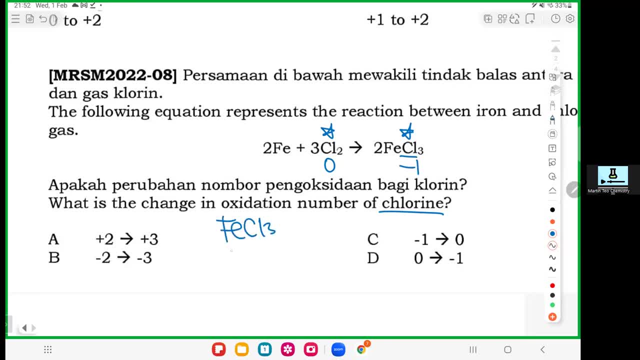 negative one, Because we know FeCl3 is made by Fe and Cl. We know the Cl, the charge is minus. Very good, Okay. so it's what? Zero to minus one. Zero to minus one, End of story, Okay. 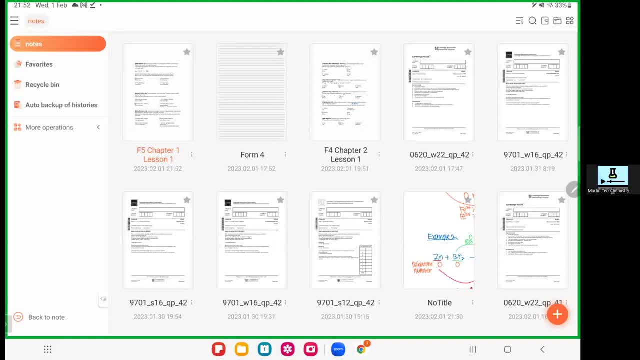 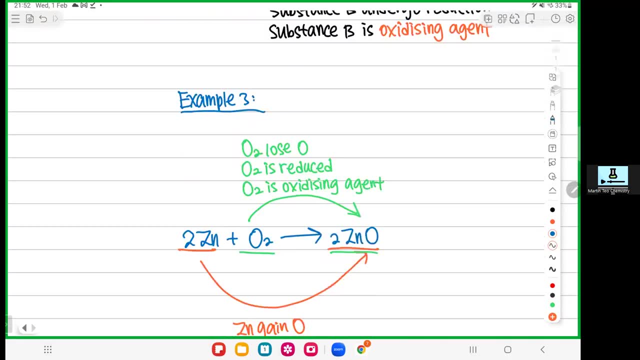 So, with that being said, with that being said, we are all done with whatever thing we need to learn today, So let's take one minute to do a summary. So, today, what we have learned Today, we started with the first chapter. 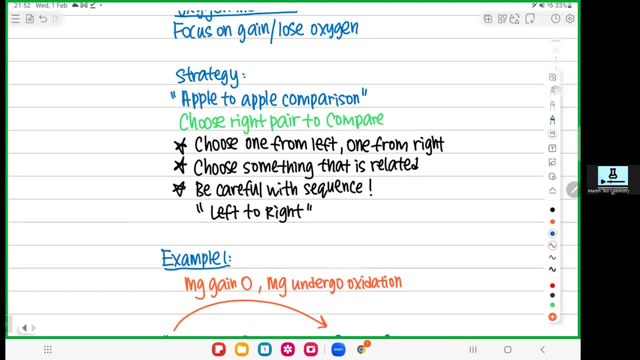 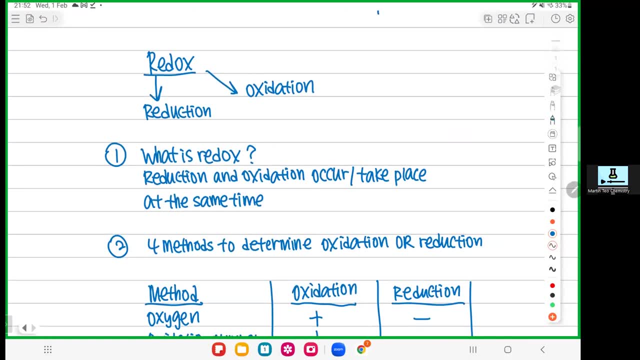 of your Form 5, Chapter 1.. The longest chapter. We will spend four months. Four months in this chapter alone. If we are faster, maybe three months. Okay, All right. So you need to know what is redox, Oxidation and reduction. 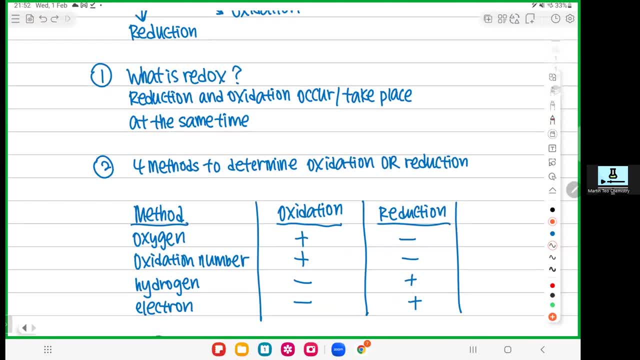 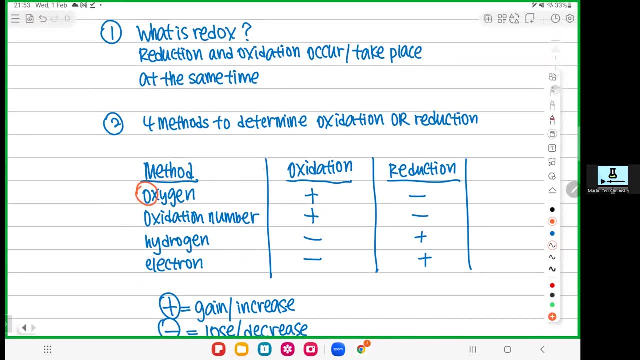 these two processes must happen at the same time. Okay, So you have four methods to find out. the chemical reaction is oxidation or reduction. So make sure you know the four methods and how to memorize. Same letter put plus. Different letter put minus. 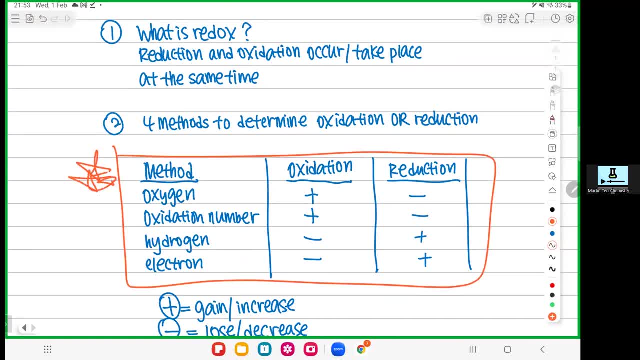 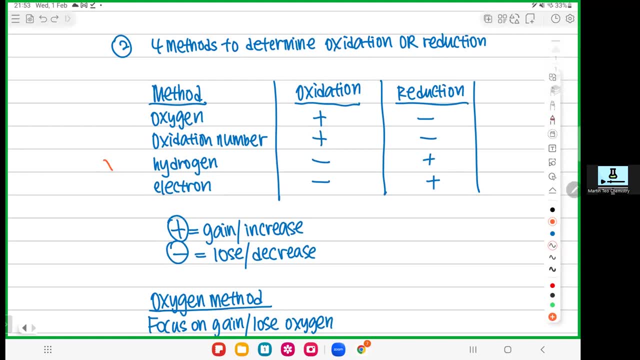 Okay. So this table is super, duper important. You must know this table, So make sure you know. Today we learned oxygenation, Today we learned oxygen method, Today we learned hydrogen method And today we learned oxidation number method. 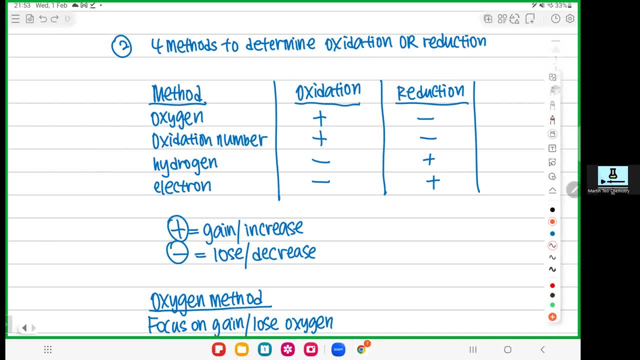 which is good. Okay, All right. So you must be able to do apple-to-apple comparison. Do the apple-to-apple comparison, which is very important. Choose one apple on the left, one apple on the right. You cannot compare left and left, Cannot? 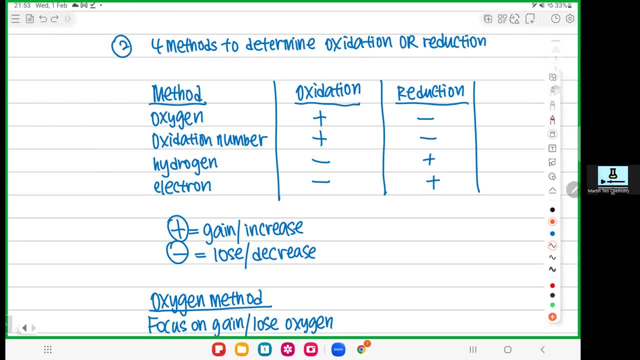 You cannot compare right and right, Cannot Must be left and right. Okay, Sometimes some apple you will compare two times. Sometimes the same apple you will compare two times. Sometimes some of the apple you don't compare at all. 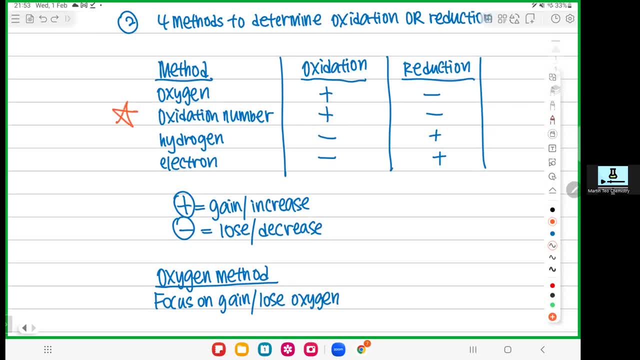 which is okay. Yeah. And the most important one is oxidation number method, Because this is super popular in SPF. So you must know four rules. Rule number one: if you have one species, you are element, your oxidation number is zero. 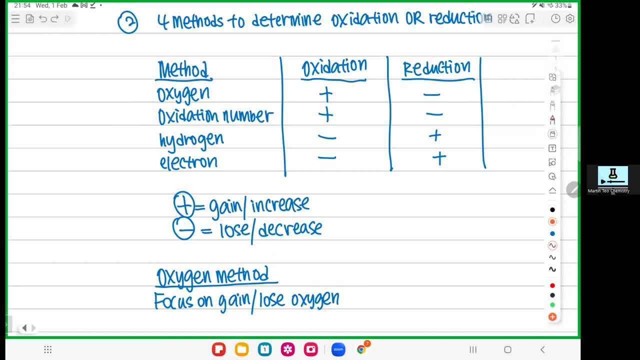 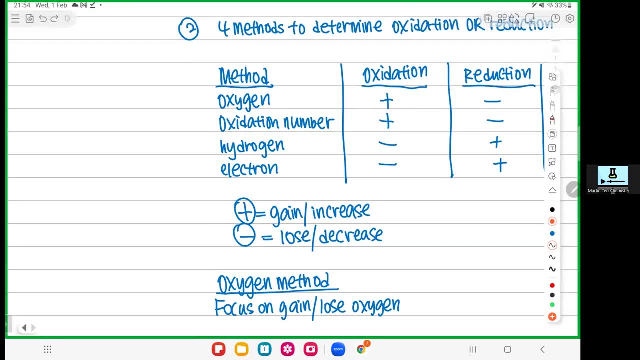 Rule number two: if you have charge, you are ion Oxidation number of the ion same as the charge. Rule number three: if you are oxygen, your oxidation number is always negative. two, except you are O2, which is element, or you are H2O2, hydrogen peroxide. 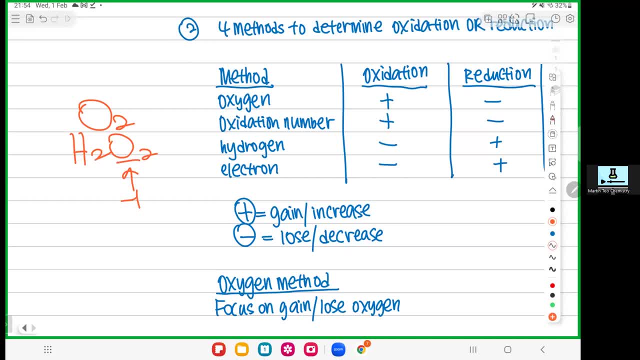 If you are hydrogen peroxide, the O is negative one. Rule number four: oxidation number of hydrogen is always plus one Special case: when you are H2, hydrogen gas, you are element, so zero. When you have metal combined with hydrogen, you are metal hydride. 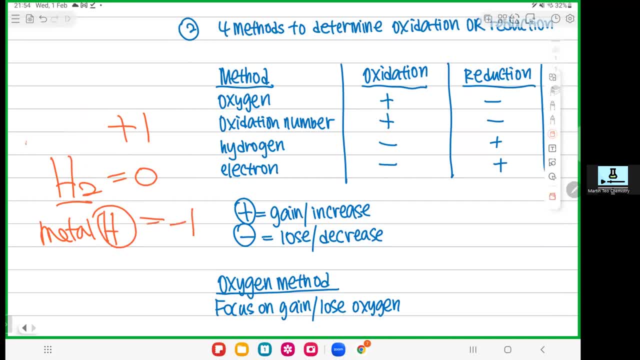 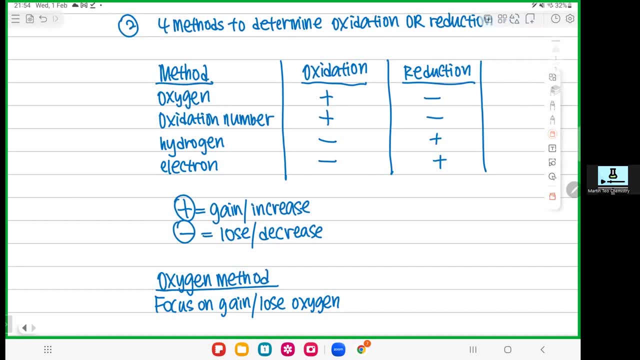 The hydrogen here is negative one. Other than that hydrogen, always always positive one. Okay, so I need your feedback. So, guys, can you please let me know in the chat box how's everything for today? How is it? Okay, not very hard, isn't it? 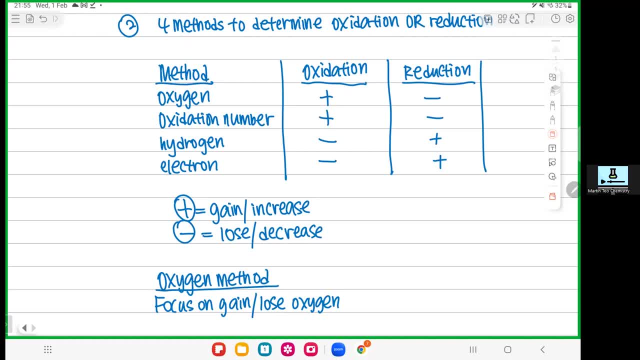 Okay, you follow the steps. You follow exactly the steps I told you. you will be fine. So, for the first few lessons, I'm not going to give you a lot of information. I'm not going to give you a lot of information. 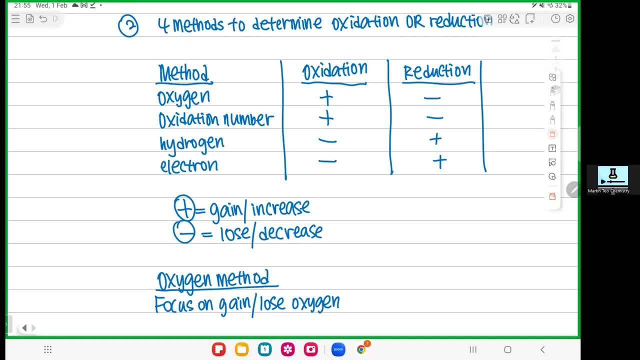 I'm not going to give you a lot of information, But after that I will let you to do tutorial. I'll give you three to five questions for you to do, Not too much that make you very stressed. but you must always do some question one, okay. 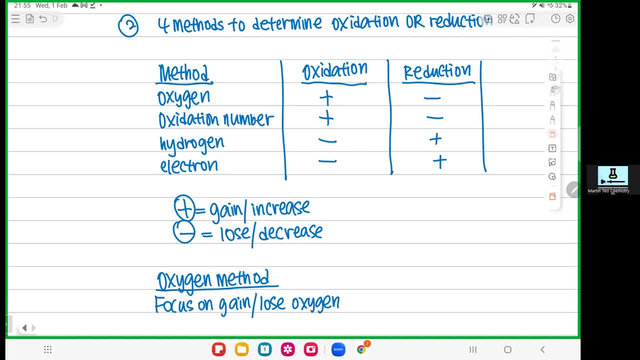 Because I know if I'm not giving question it's very hard, that you will take initiative and do on your own very hard. So I'll give you a few questions just to help you, to really test your own understanding. okay, But not for today, okay. 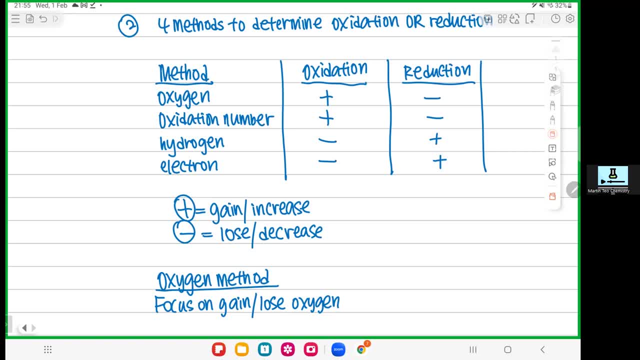 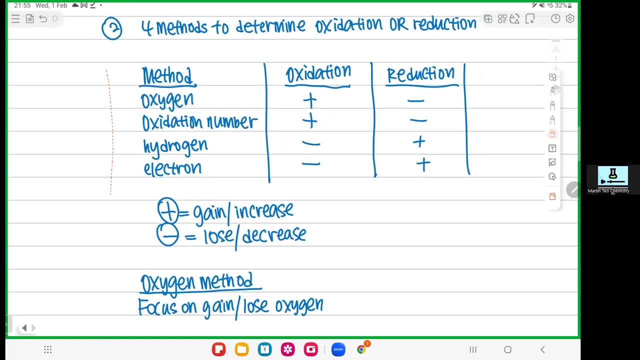 After three to four more lessons, then only I start to give you a few questions. as you know, your homework or tutorial, okay, So you see, this is the way that we will learn in your home five, We learn something, and directly.